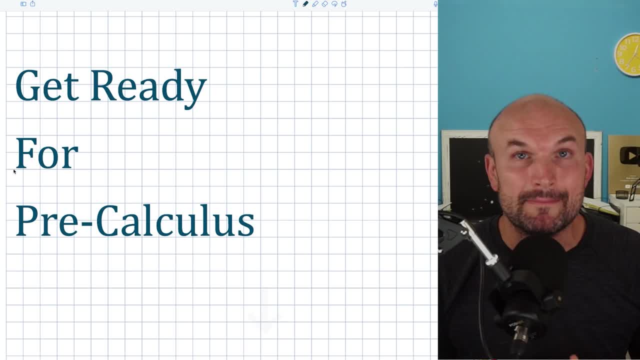 understand that you might be looking for something in particular. Therefore, I do have all of the topics and questions timestamped down below. Also, for you overachievers, I have some bonus content that you can take advantage of If you want to go ahead and download the worksheet. 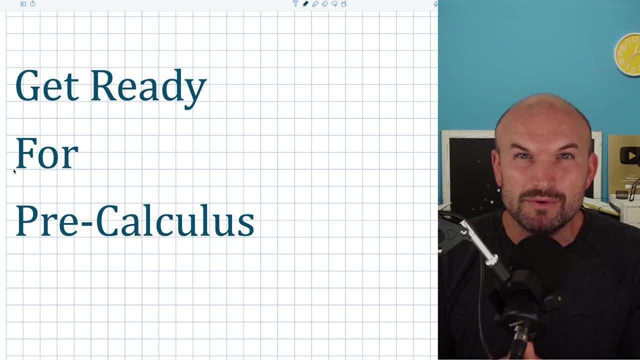 that I worked through on this video. then go ahead and check out the link down below As well if you want to go and try a diagnostic test to kind of see how really well prepared you are for pre-calculus. I'll make sure that information is provided, as well as information regarding my get. 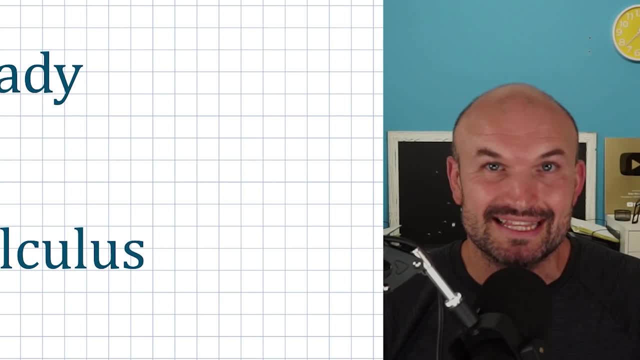 ready for pre-calculus course, where I go much more deeper into the content that we're going to touch on today to really get you prepared for pre-calculus And if you're not really sure if pre-calculus is right for you, well, 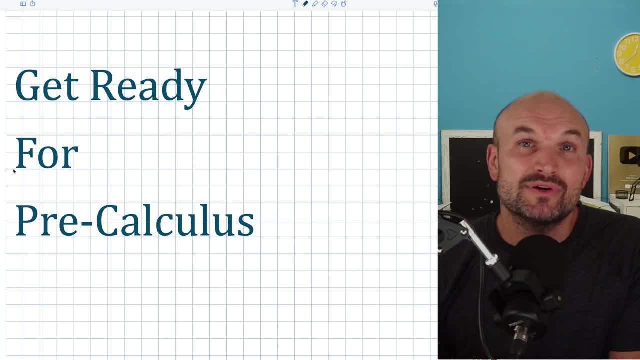 obviously you can go ahead and check out the link down below And if you're not really sure if pre-calculus is right for you, well, obviously this video is going to help prepare you for taking pre-calculus- what exactly pre-calculus is, as well as how you can ensure that you are. 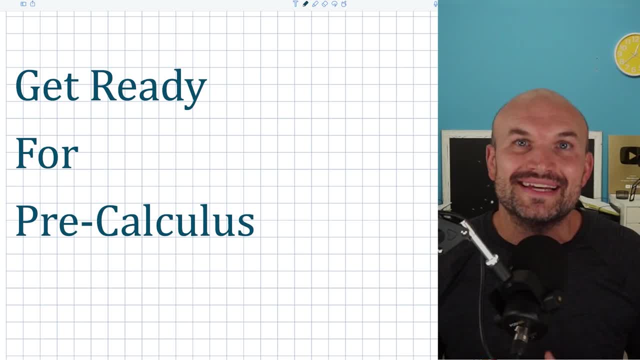 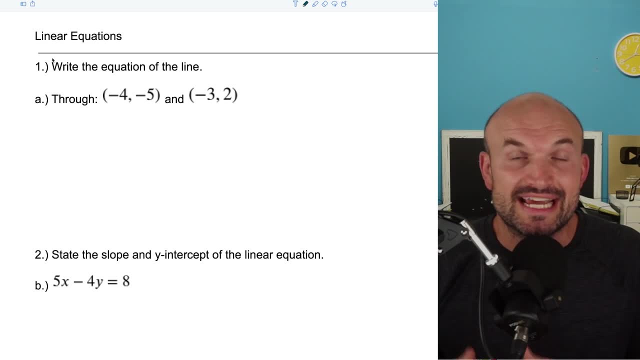 going to be successful. All right, that's enough of that. Let's go and get into the good stuff of getting ready for pre-calculus. All right, so one of the first topics that I want to kind of talk about for this video is linear equations, because that's really going to be a foundational topic. 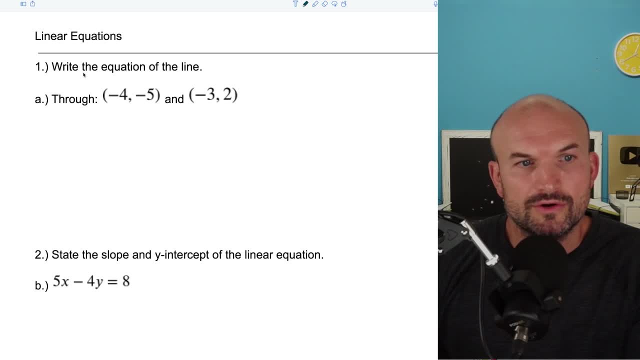 that, I think, is just going to be really important for you to know. So let's go first go through, like writing the equation of the line. So in this case we're given two points. And just remember, when we're given like two points, we can always label these points as like X? Y and X Y. But to 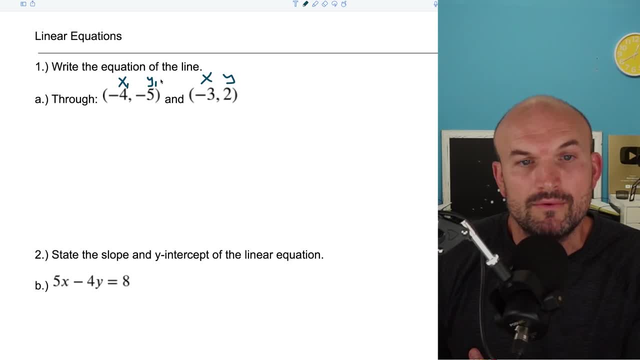 differentiate them. we're going to use subscripts, So I can say like this is X1, Y1, and this would be then X2 and Y2.. So to write the equation of the line now, there's a couple of different ways we. 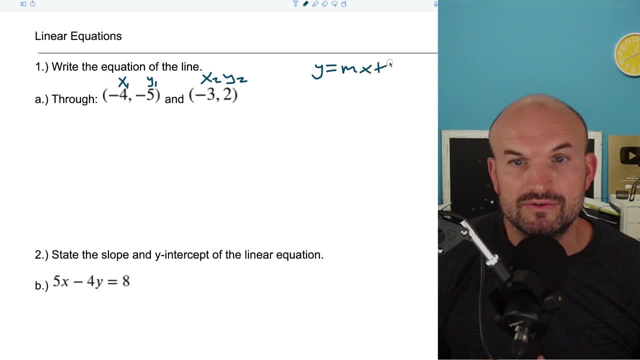 could write the equation of the line right. We could write it in slope-intercept form: Y equals MX plus B, or we could also do it in point-slope form. I will say kind of like: point-slope form is one that is probably more common in, like pre-calculus and calculus, So it is going to be. 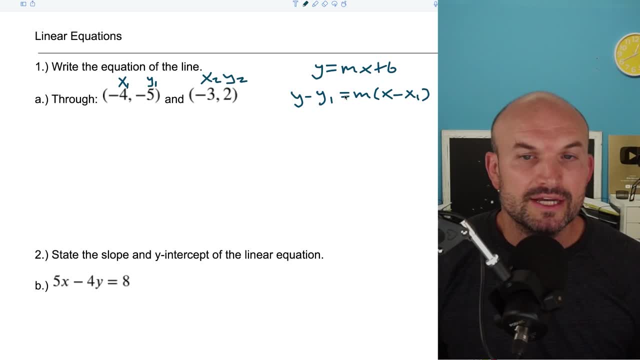 really helpful to make sure that you can go ahead and be able to write the equation in really kind of both forms. And now, the one thing that's kind of in common for both of these is, besides the Y and the X, but there's also the M, And remember, M represents the slope. Now, if you're given two, 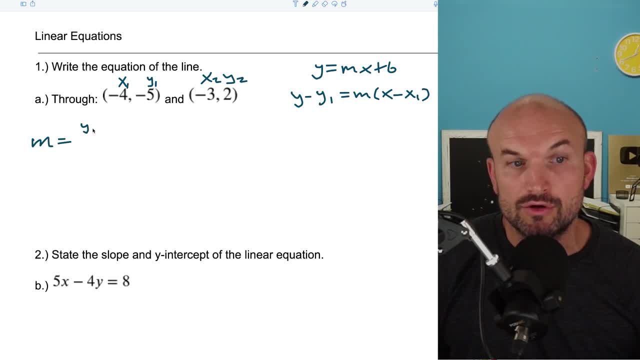 points, you're going to need to find the slope, And so it's important to remember the slope formula, which is going to be a Y2, a minus a Y1,, all over a X2 minus an X1.. So, if we want to find the slope, 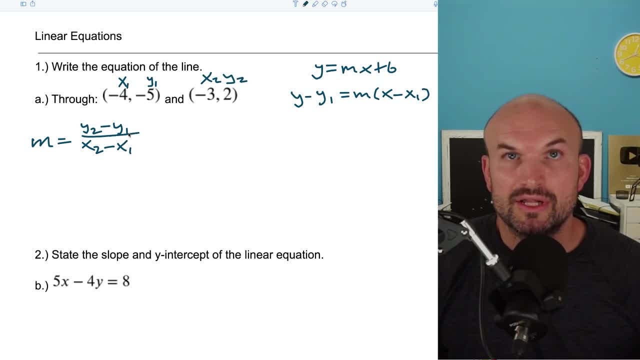 between these two points or of this equation of the line, then we need to go ahead and plug in our values. So what I'm simply going to do here is do a 2 minus a negative 5.. And then over here, a negative 3 minus a negative 4.. Now notice that I use parentheses here, And this is really. 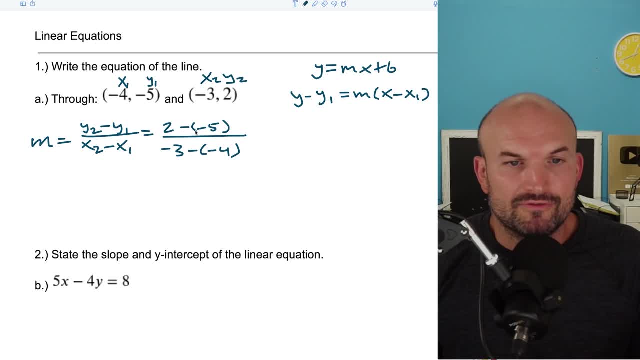 important because a lot of times students will just kind of subtract terms here and they'll forget about using parentheses and therefore they get the problem wrong. So when I do this I have a minus, a negative. So 2 minus a negative 5, that's actually going to be a 7.. And over here, 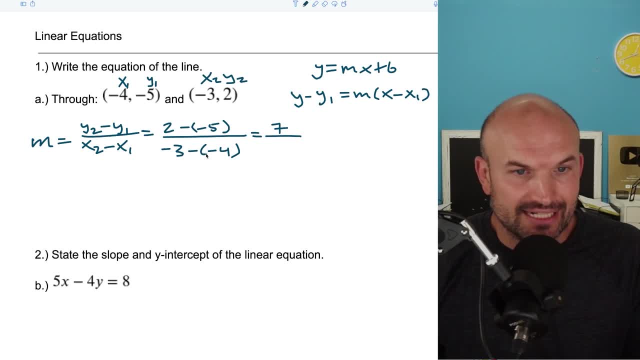 I have a negative 3 minus a negative 4.. Well, again, that's like adding right. So it's like a negative 3 plus 4, which is just going to be a positive 1.. 7 over 1 is just going to be now a 7.. 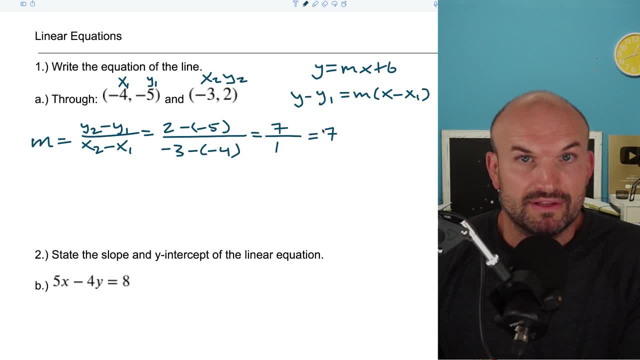 So now we know what the slope is, Now we would need to be able to figure out the equation of the line. So I'm going to go ahead and plug this into my point slope form And again, I'm going to plug a X1 and a Y1 into that equation as well And therefore we can just find that, find the equation. 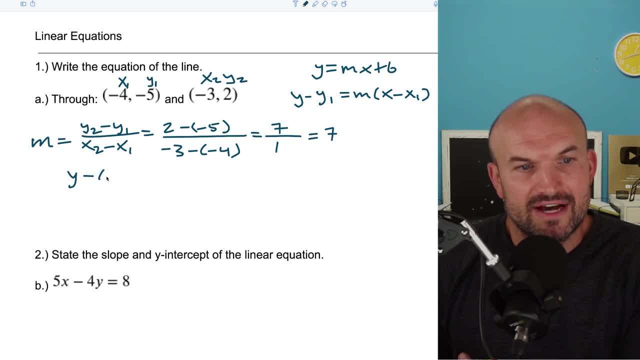 of the line. So what we'll have here is a Y minus a negative 5.. Again, I'm going to use my parentheses here. It's going to equal to a M, which is going to be a 7. And that's going to be an X minus a. 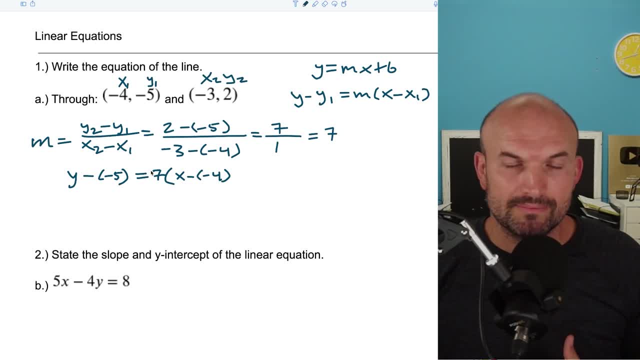 negative 4.. Okay, Now that's the equation of the line that's in point slope form. Now I do recognize teachers, or your own teacher might want you to put in slope intercept form, So let's go and practice that. Notice, actually I got a quote Make sure you use whenever you open a parentheses. 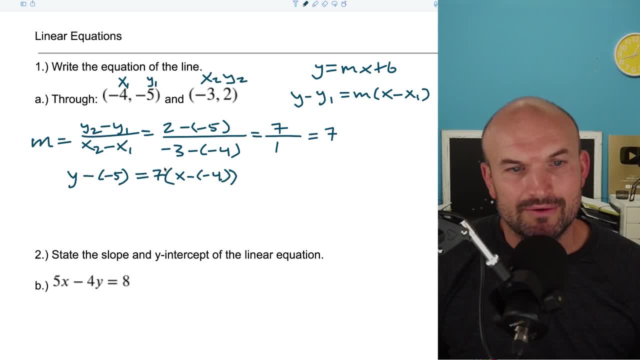 make sure you also have one closed, All right. So let's go ahead and simplify this. We are going to have to apply the distributive property here And this becomes a. Y plus 5 equals a. let's see, that's going to be a 7X And that's going to really be a positive 28,. right, Because minus. 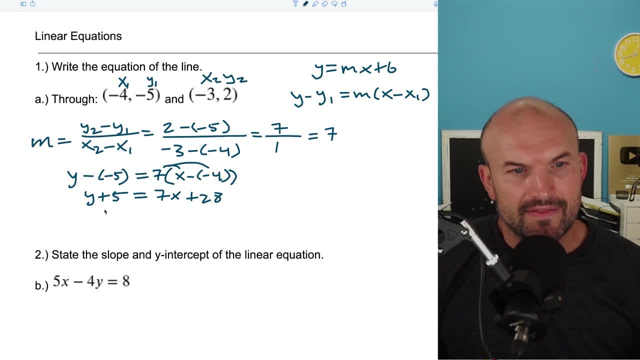 a negative, so it's a positive 4.. 7 times 4 is a 28.. And then now, just to go ahead and simplify this, I can subtract a 5. So I get Y equals a 7X minus a 23.. Okay, And I think that's what we were asking. Yep, So that's. 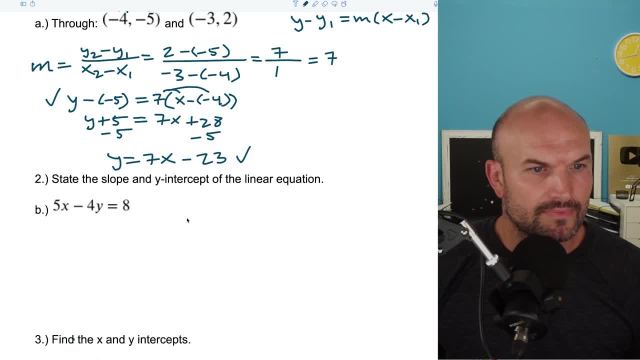 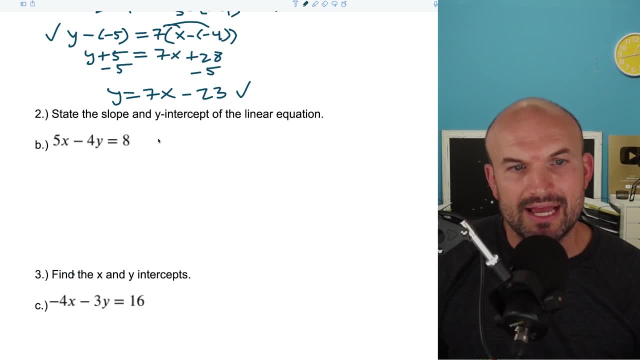 another equation of the line from on there. All right, The next question is saying state the slope and the Y intercept of the linear equation. So there's a couple of different ways we can do this. You know, when we have an equation that's in Y equals MX plus B, form, right Like the slope. 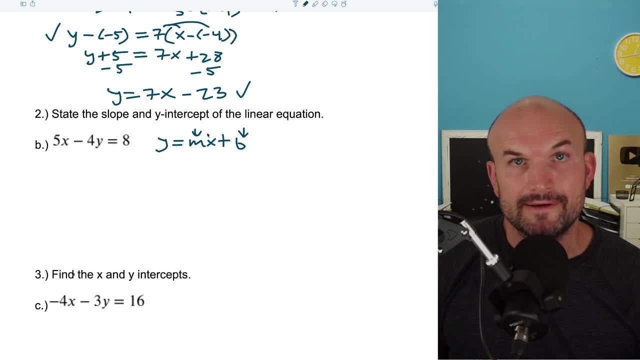 is kind of easy. That's your M and your Y. intercept is going to be your B right. So you know kind of straightforward. So the first way, I'd kind of say that it's important to be able to do this. 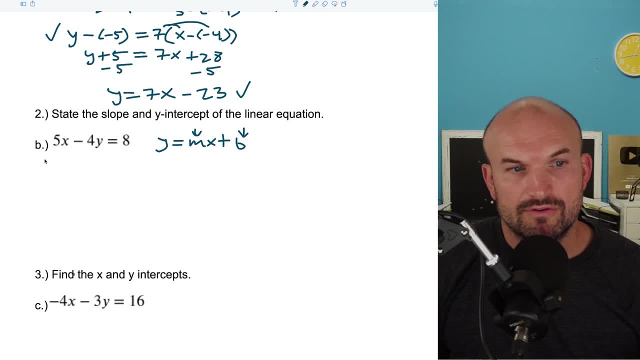 is just to kind of rewrite this in slope intercept form. So to do that, we're just going to solve for Y. So what I'll do is I'll subtract a 5X on both sides and that's going to leave me with a negative. 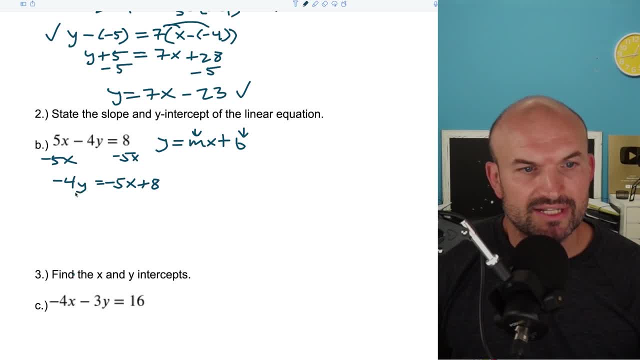 4Y equals a negative 5X plus an 8.. Now I can divide by a negative 4 on both sides and I get a Y equals. Now it's really important that you make sure you remember to divide the negative 4. 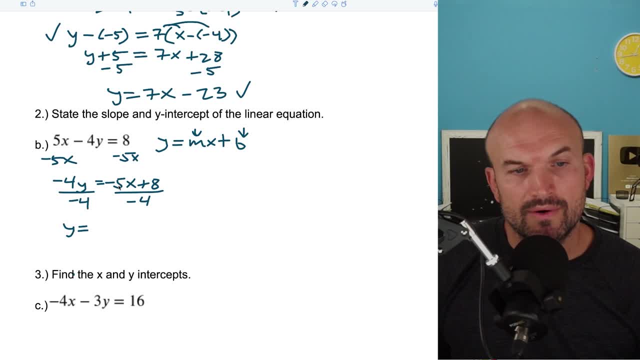 into the negative 5X, as well as a negative 4 into the 8.. So a negative 5 over negative 4, it's going to be a positive 5, 4s X And an 8 divided by a negative. 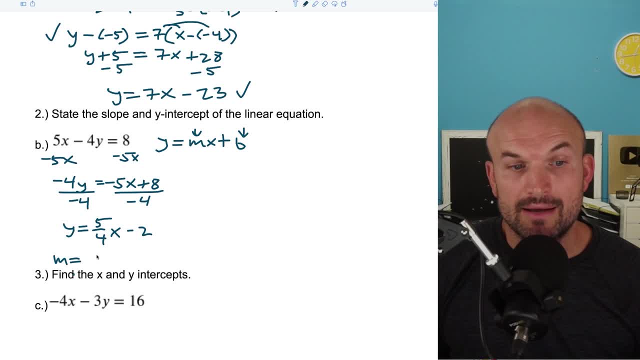 4 is just going to be a negative 2.. So therefore, we can say: our M, which is our slope, is going to be a 5- 4s And our Y intercept, which is our B, is going to equal a negative 2.. Now there's another. 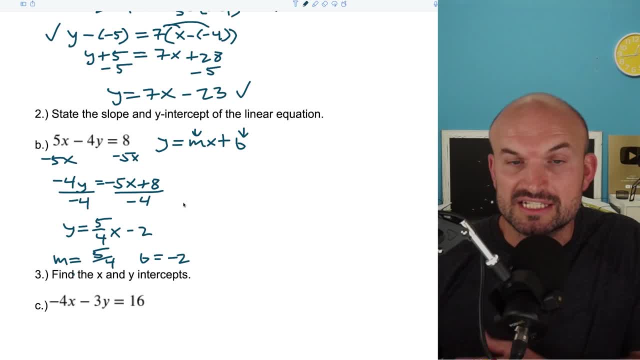 way that we can be able to do this, which, you know, I kind of want to be able to make sure I can explain this, because it's going to kind of help us for further problems down the road, And not so much really about the slope. The slope is just kind of like a little trickier. This is what 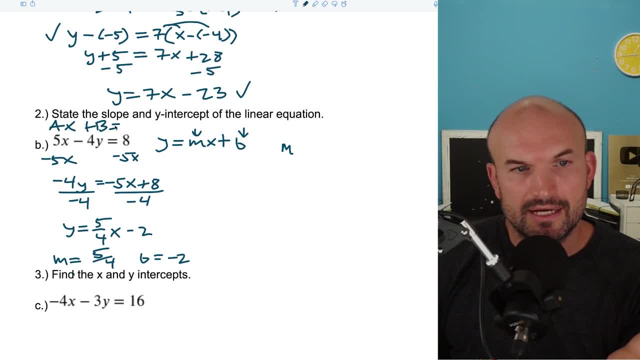 we call in standard form. If you have AX plus BY, that's sorry, BY is equal to C. Actually I don't know why, I'll just go ahead and delete that. So that's a BY is equal to a C. So how can? 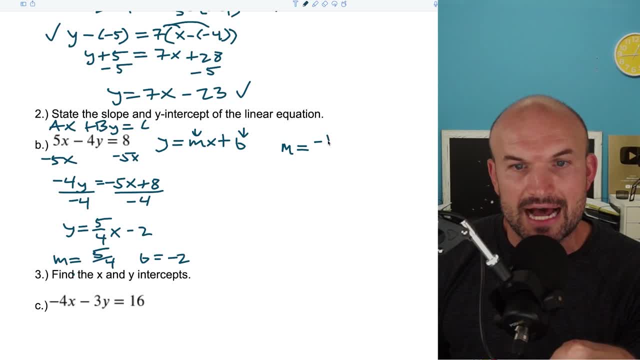 you write the slope. Well, a nice thing to know about the slope is: M is equal to the opposite of our A over B. So all I simply need to do here if I want to just kind of find the slope I actually didn't need to solve for Y- All I simply need to do is take my opposite of my A. 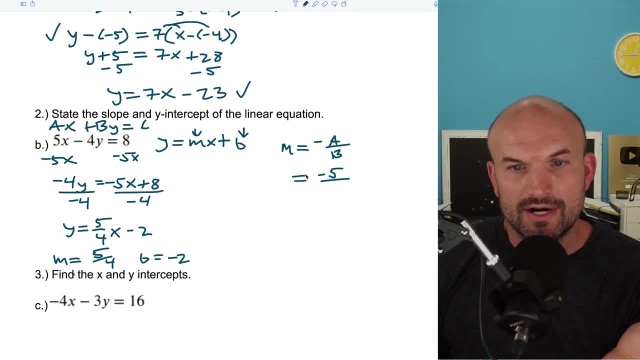 which in this case would be a 5, right, So this would be a negative 5 over a negative 4.. Well, negative 5 over negative 4 is what A 5- 4s. And is that the slope that I figured out? Yes, it is. 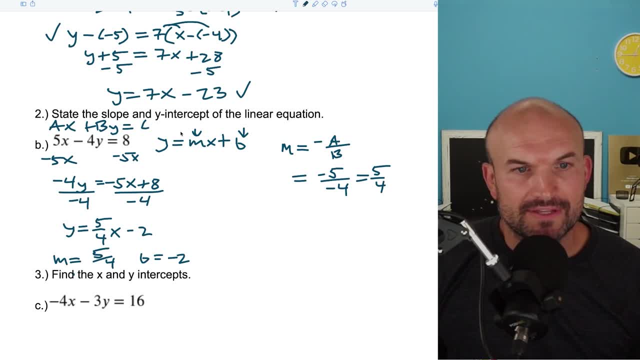 So that's just kind of a way to do it And I'll see you in the next video, A little helpful kind of tip hopefully, to help you out there. The other thing I want you to understand is the Y intercept. When you're trying to find the Y intercept, that's when X is equal, 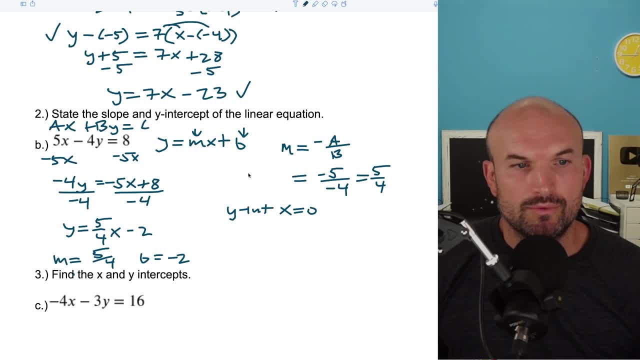 to zero. So, again, we don't really need to actually solve this for Y. What we simply can do is- or I mean from the beginning- is just plug a zero in for X and that's going to be a zero. 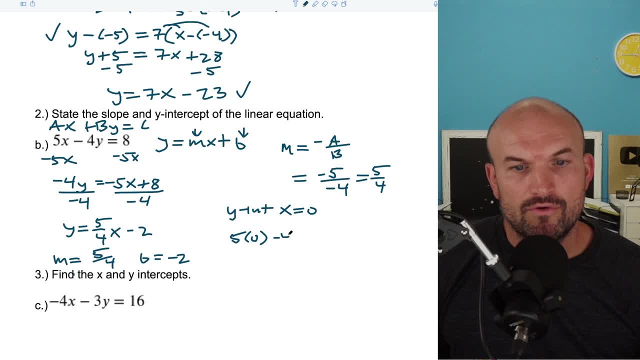 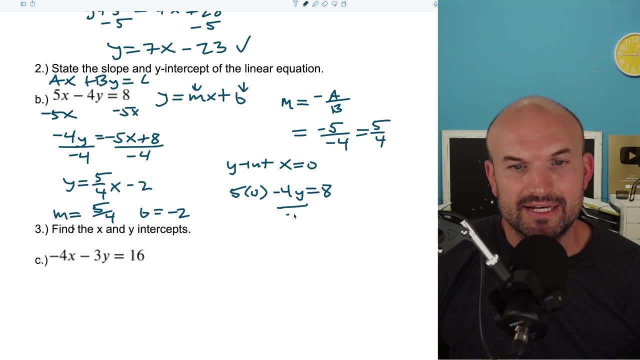 what? five times zero- And that's going to be minus a 4Y is equal to an eight, right? Well, again, obviously, now that just goes to zero, right? So therefore you'll have: you can divide by a negative four on both sides and you get Y equals a negative two, which, again notice- is the. 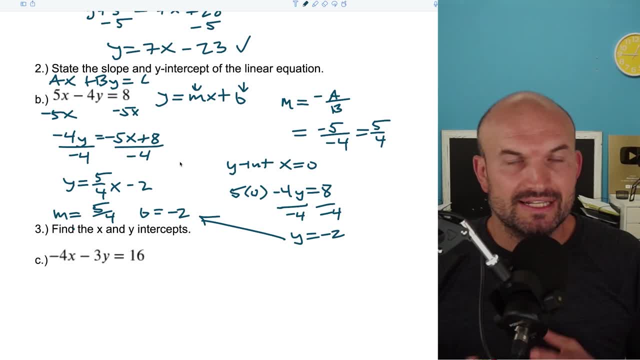 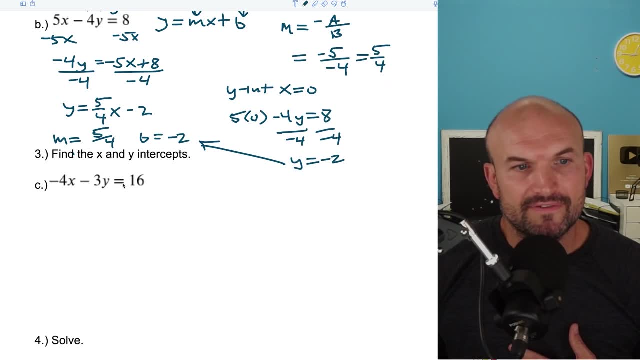 exact same thing we did when we had it in slope intercept form. So I just want to kind of give you those alternatives. And the reason why actually, I think it's really important to recognize that is because if in the next example it says: find the X and the Y intercepts Well. 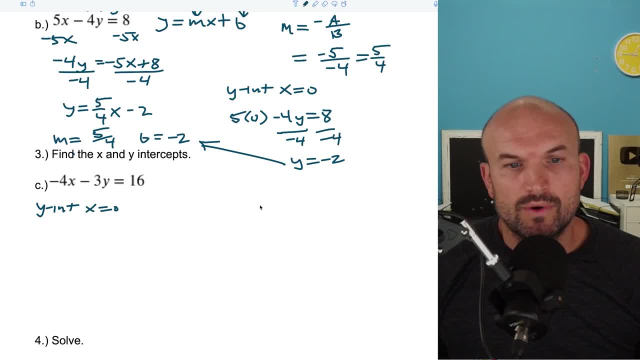 the Y intercept was when X is equal to zero. So what do you think is going to happen when we want to find the X intercept? Well, it's just going to be the opposite, right? X intercept is Y is equal to zero, And that's a really important concept. 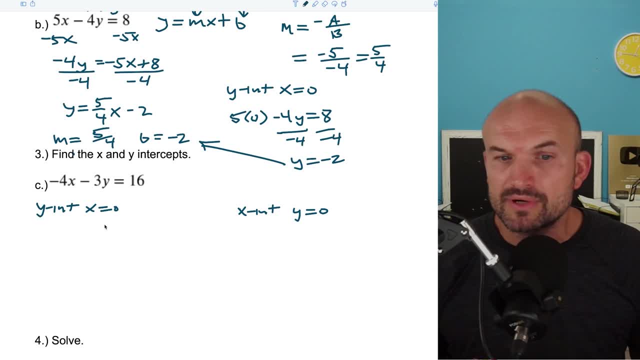 To know for precalculus, because this is going to come up over and, over and over again, because in precalculus we're going to be dealing with a lot of different functions that are going to come up. So you're going to want to make sure you know how to find the X and the Y intercept. 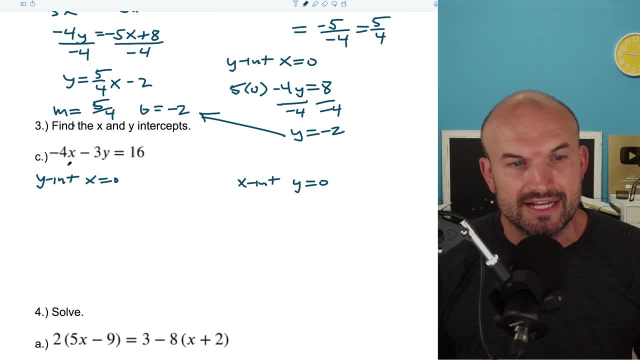 no matter what type of function we have And no matter what this is going to be that rule that you're going to want to pay attention to- that If the Y intercept X equals zero, the X intercept Y equals zero. So in this case, all we're simply going to do now is just plug a zero in for X and 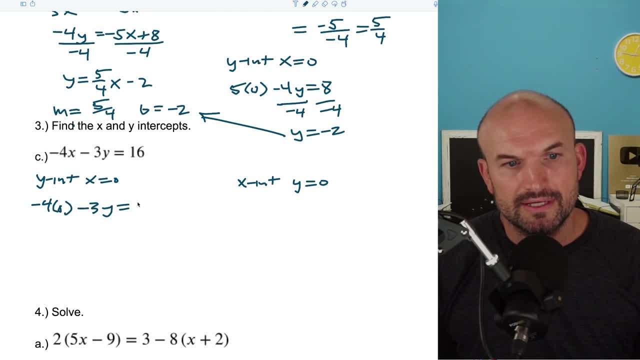 then solve for Y, right? So therefore, that's going to be a three Y equals a 16.. And now let's just go ahead and solve Negative: three Y equals a 16 divided by negative three. divided by negative three, Y is going to. 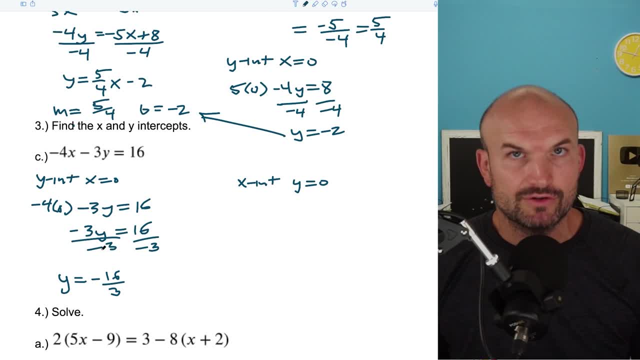 equal a negative 16 thirds. Now, if you wanted to graph this, a lot of times students will be confused Like, how do I graph a negative 16 thirds? So a lot of times, what I think it's always helpful is just so you can just rewrite it as a mixed number. Now, as far as an answer goes, 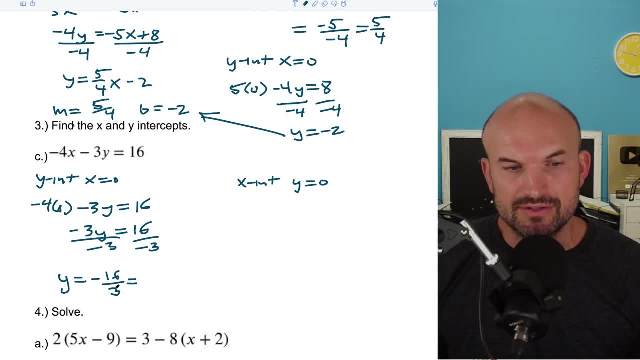 I'd prefer it as an improper fraction, but I just want to kind of show you like you could also just rewrite this as a mixed number. Three goes into a 16.. Forget about the negative right. We already know it's a negative value. Three goes into 16, what? 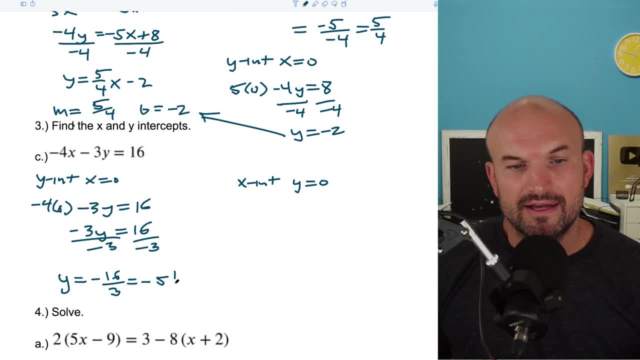 Times right And then we have a remainder of one, So that's going to be a negative five and one third. That would be a little bit easier to graph- negative five units and one third- than a negative 16 thirds. So just make sure you can kind of recognize that, because a lot of times when 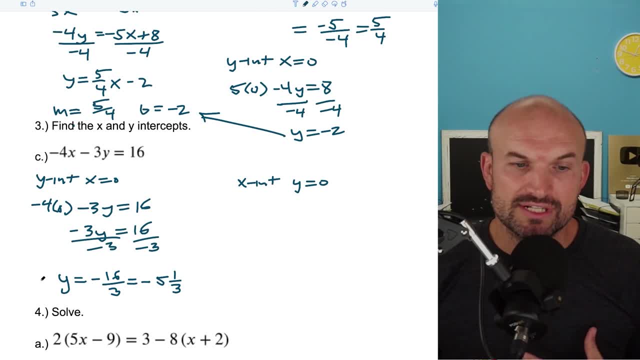 we do want to find the intercepts, we need to plot them. So it's I think it's kind of important to understand: how do you plot something that's going to come in as a fraction? Now, for the X intercept, Y equals zero. So we're going to basically do the same thing. We're going 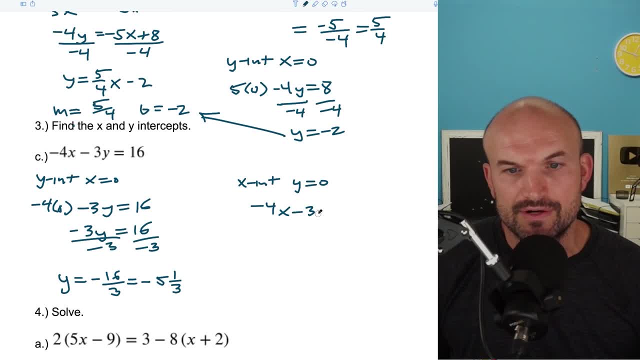 to negative four: X minus a three. I replaced the Y with a zero right And therefore that's going to be a 16.. So therefore, now I'm left with a negative four. X equals a 16 and divide by negative four on both sides, And when I do that I get X equals a negative four. And again, just remember guys. 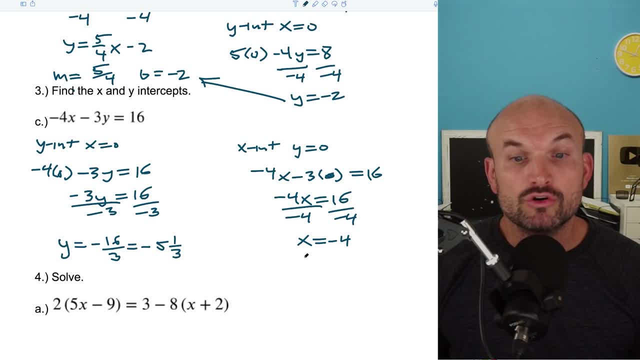 like. these are coordinate points, right? These are the plot. These are the values that cross on the X and the Y axis. So you could also rewrite this as a negative four common zero. And you could also write this one as a, let's say, a zero, negative 16 thirds, right? So just remember, those are. 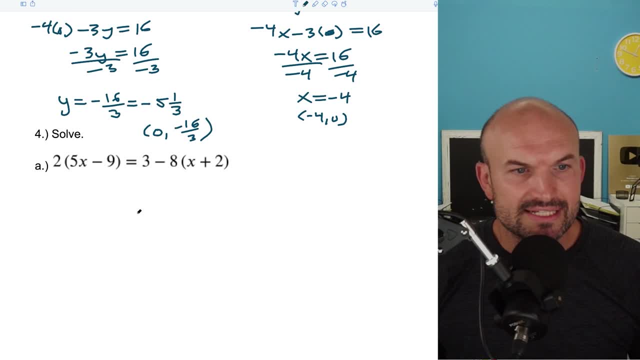 coordinate points on a graph. All right. The next thing um we're going to look at is just kind of going back through some like linear equations, And I think it's just really important to you know, remember, how do you solve an equation Like that's going to. 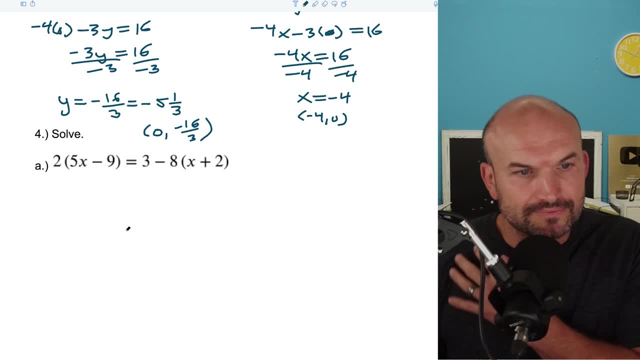 come up time and time again. we're going to be, you know, moving variables around. So in this example- just recognize: here we have parentheses and we have variables on both sides- The first thing I'm going to want to do is get rid of the parentheses, And the way that I'm going to do that. 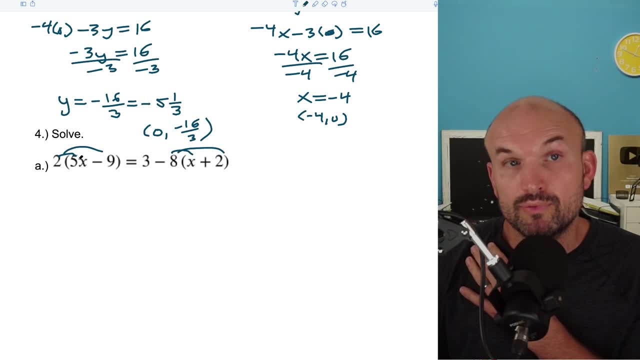 is by using a distributive property. So I'm going to multiply my two through both terms inside the parentheses, as well as a negative eight- Now remember that's a negative- is attached to that eight, So don't multiply by an eight. You've got to make sure you're multiplying by a negative eight. 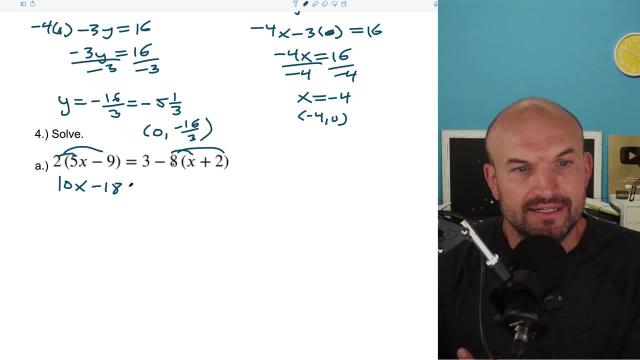 So when I do this, I'm going to get a 10 X, and minus an 18 is equal to a three. Now, this is going to give me a negative eight X and negative eight times Um. a positive two is going to give me a. 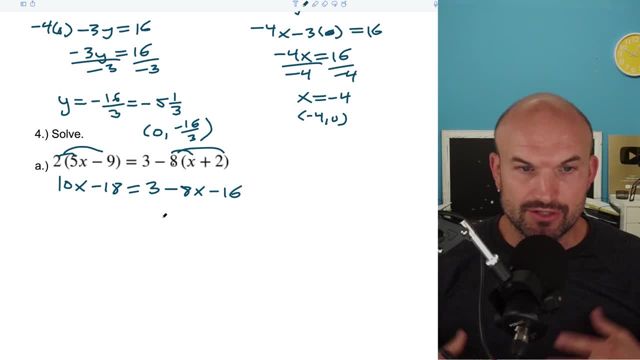 negative 16.. All right, So now I have an equation with no parentheses or grouping symbols. That's good. Now I want to get my variable to the same side. Typically, I always like to get my variable on the left-hand side, or at least make the coefficient to be positive, In this case. 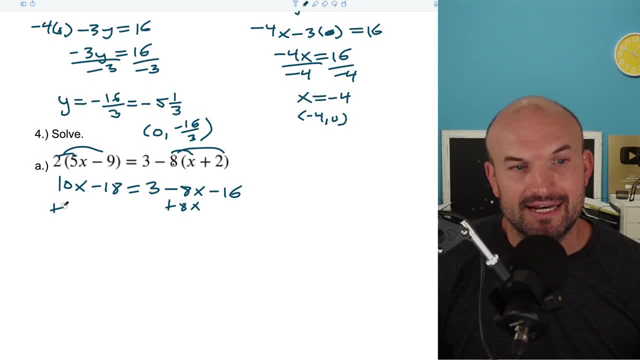 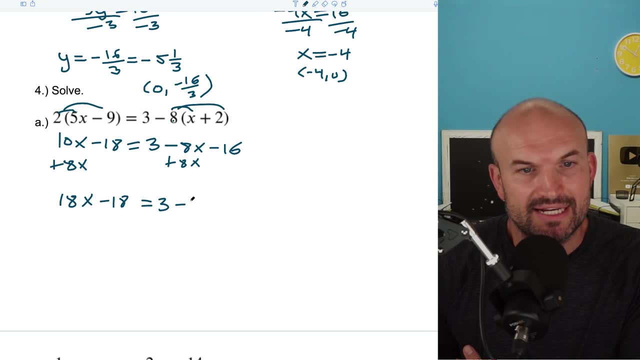 both are going to be true when I add an eight X to both sides. So I add an eight X to both sides. All right, That's going to give me a 18 X and that's going to be minus 18.. Um, that's going to equal a three minus a 16.. Okay, Now I can. 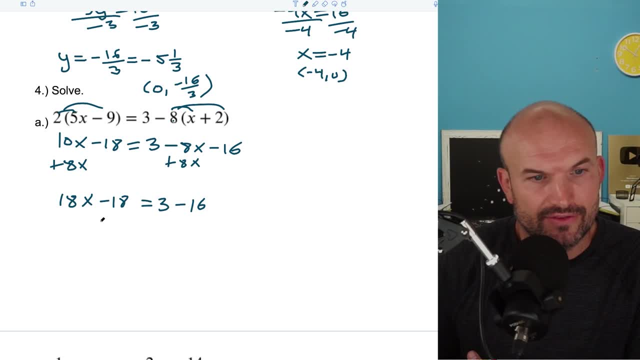 go ahead and simplify it to a negative um 13.. And so therefore, then I'll just go ahead and solve for my eight X, So I'll go ahead and add a 18 on both sides. So this is technically going to give. 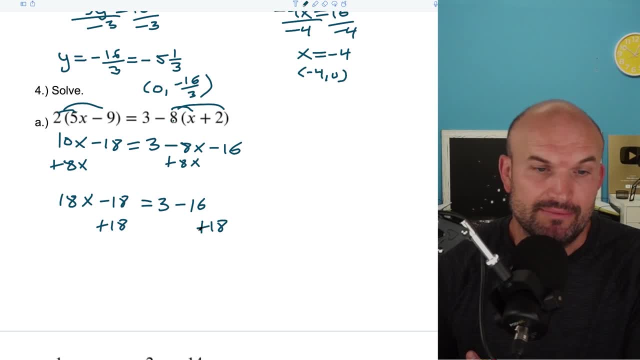 me a negative 13 and then plus an 18, right, So that's going to give me a negative 13, plus 18 is going to give me a positive five. So I have an 18, X is going to equal to a five, And then I can just 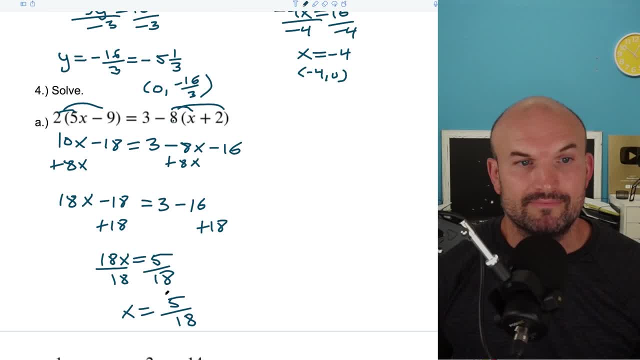 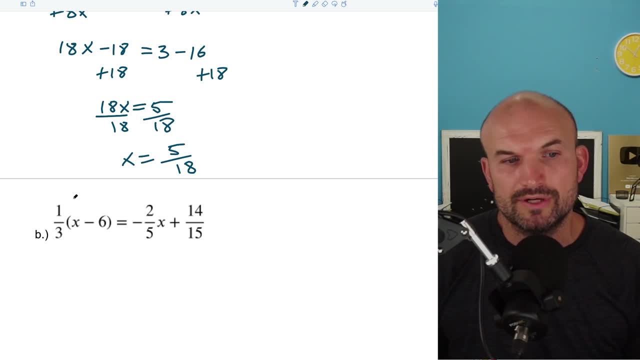 go ahead and multiply it And now I get an X is equal to a five over 18.. So now, next one, we have a little fraction. So basically the same kind of idea and concept. we're just now going to be dealing with fractions. So again, we want to get rid of the group example, So I'm going to go ahead and 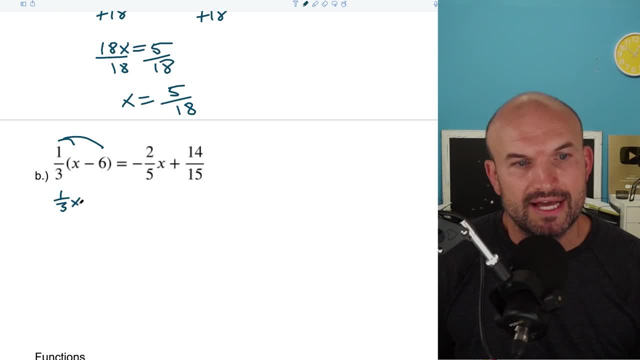 multiply my one third times everything inside of there. So therefore that's going to give me a one third X. now one third times a six, or negative six, right? So a lot of students will get confused with the fractions. So just remember: all fractions you can rewrite are all numbers You can rewrite. 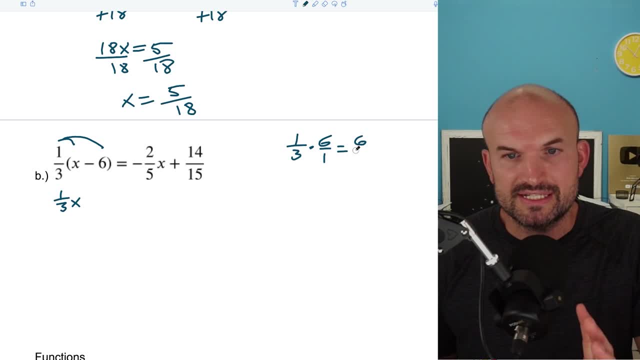 as a fraction, right, So you're multiplying fractions, you multiply straight across. So this is going to be a six over three, which is just going to equal a two, but again that's a negative six. So therefore that's going to be a negative two, And then we're going to have a negative two fifths X plus a 14. 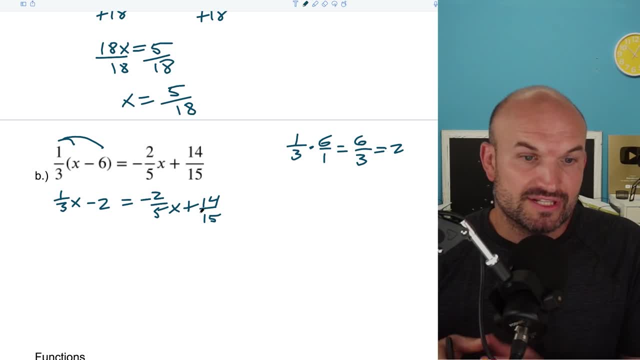 fifteenths. Okay, So again, we want to get our fractions, you know, to the same side. right We are. we got to get, I'm sorry, our variables to the same side. So what I'm going to do is I'm. 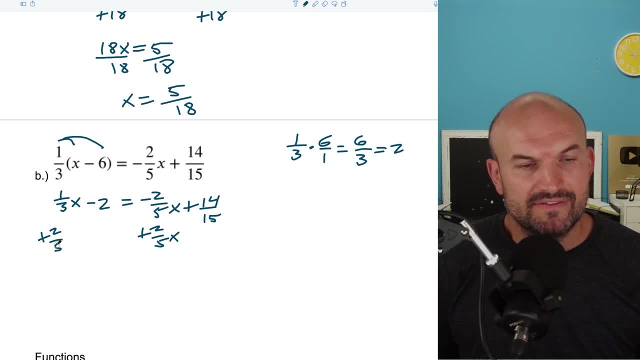 going to add a two fifths X to both sides, Okay, So I have a two fifths X plus a one third X. So again, remember, when you're adding variables you got to add the coefficients. So basically, what I have is a one third plus a two fifths, Like, and we got to. 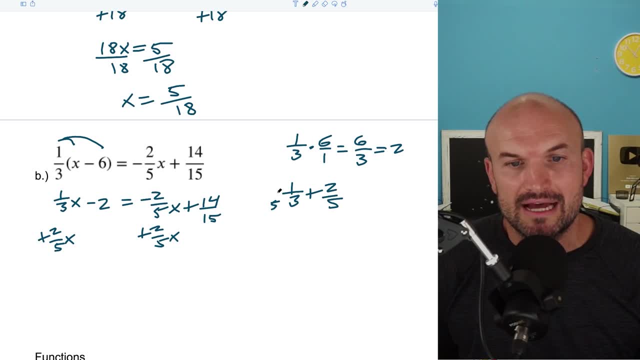 remember how do we do that? Well, we got to get a common denominator And in this case, the common denominator is going to be the product of our denominator. So I'm going to do that on the top and the bottom, And when I do that now, I'm going to get a five over 15 plus a six over 15, right? 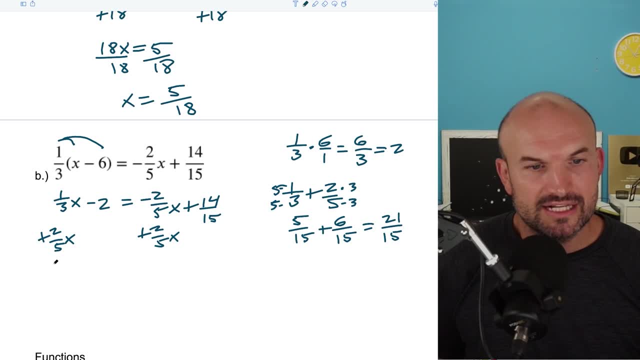 So that's going to give me a 21 over a 15. So that's going to be a 21 over 15.. And again, that's an X right Minus two equals a 14. 15.. Okay, Now what I need to do is go ahead and add a two to both sides. So now we need to somehow 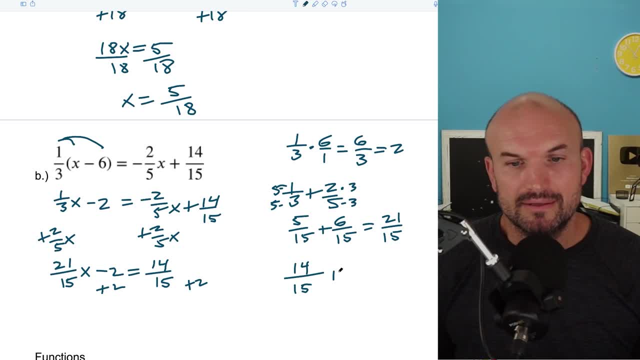 figure out. well, how do you add a fraction for like 14,, 15 plus two, right? Well, remember, two can be written as a fraction. And then we just want to be able to write the common denominator, right, Which is going to be a 15.. So I'll multiply by 15 on the top and bottom, And when I do that, 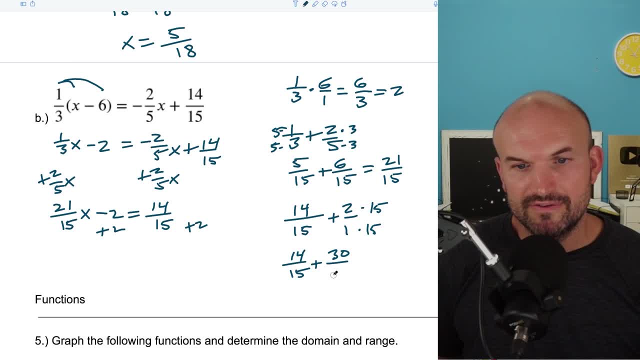 I get a 14, 15 plus. what a 30, 15 and 14 plus 13. It's going to be a 44- 15.. Okay, So now I have a 21, X. all over 15 is going to equal. Now this adds up to a 44 over 15.. Now the cool thing. 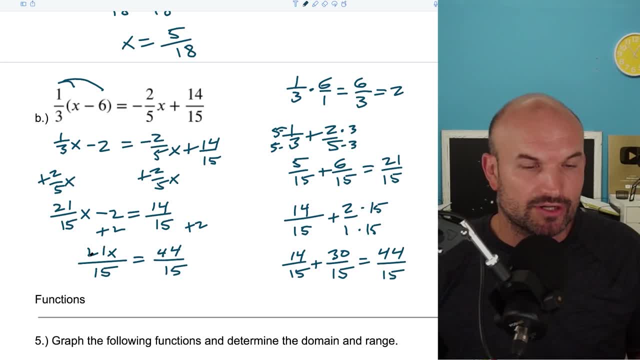 here is um the cool thing since my two, since I have an equation, whenever your equation- that are both divided by 15, you can actually just eliminate the denominator 15, because the first step we would do here in solving this algebraically would be multiplied both sides by 15 to get rid. 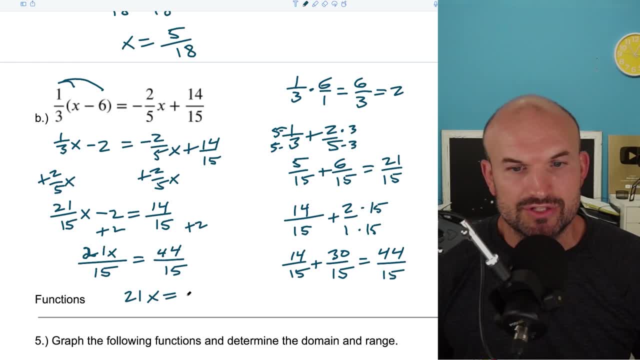 of it. So therefore I can just rewrite this equation as 21 X is going to equal a 44. And then now I'll just divide by a 21 on both sides and I get: a X is equal to a 44 over a 21.. 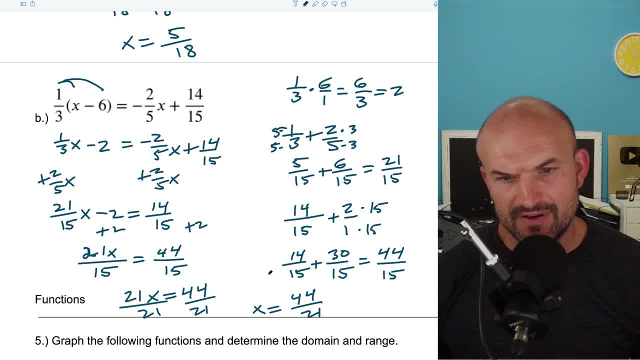 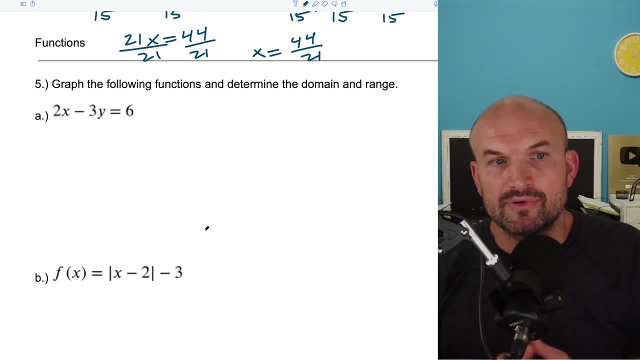 And yep, So see if there's anything else that would go ahead and simplify, but I'm not seeing anything that would All right. So now we're going to get into functions, and functions is actually a topic inside of precalculus that we're actually going to expand upon what you've learned. 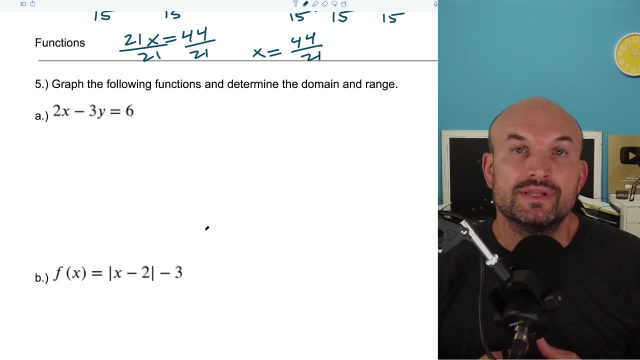 in algebra one and algebra two. So this is actually some really really important information. The linear equations was really just kind of like that Foundational stuff, making sure you remember like a line and all that kind of stuff, But for functions. now we're actually going to get into some really good, like meat and potatoes of what 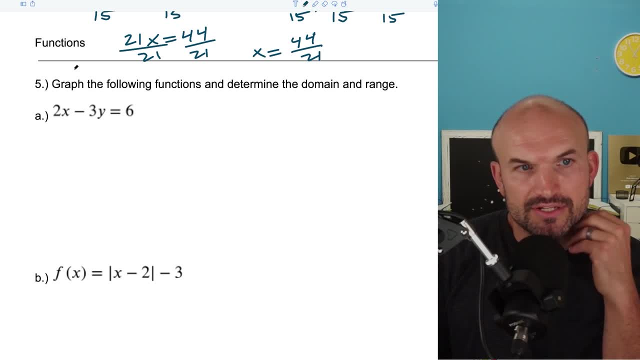 you can expect um coming into precalculus. So, um, for these questions we're going to graph the following functions and determine the domain range. So when I want to graph a line, I usually just like to rewrite this in slope intercept form. Okay, So Y equals a, MX plus B. All right, So to be. 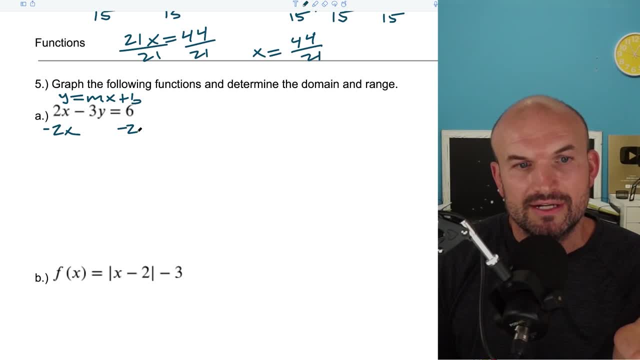 able to do that again. we're just going to basically solve for Y. So I'm going to subtract this negative two. So it's going to be negative two. I'm going to give it a value of zero, two thirds. So if you kind of go through the um, just kind of go through the process here to make 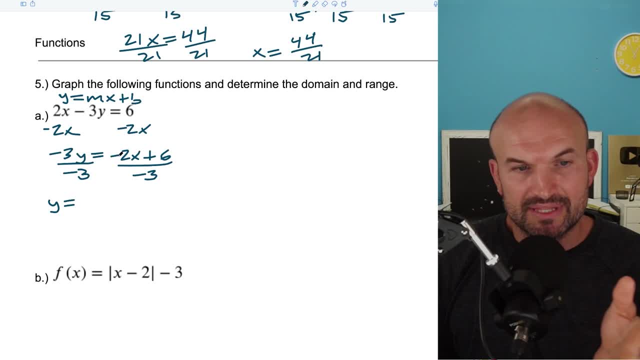 sure that you are not going to be making any mistakes and you remember everything, and everything is kind of like automatic. So remember this negative three is going to divide into both of those. So therefore, that's a two thirds. um, that's gonna be two thirds X minus two. Therefore, my 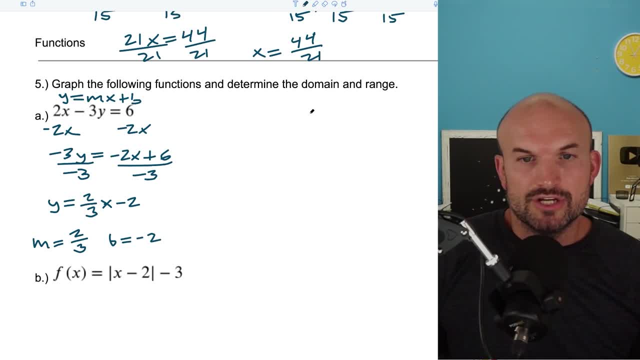 slope in this case is going to be a- two thirds, and my B, which again is my Y intercept, is going to be a negative two. So we need to graph this and then we need to determine the domain and range, create a nice little xy-intercept. 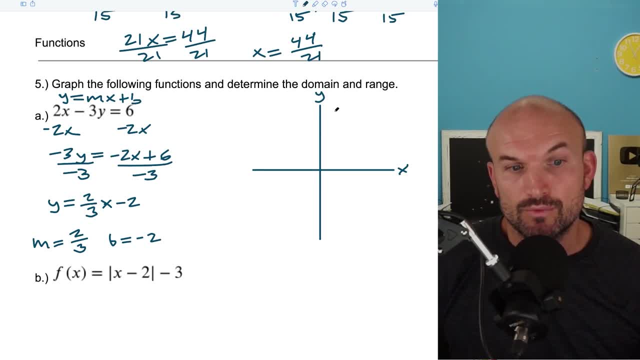 Remember, this is your x-intercept, That is your x-axis, That's your y-axis. So whenever you're graphing a line, you're always going to graph the y-intercept first. So we're going to go down to negative 2. 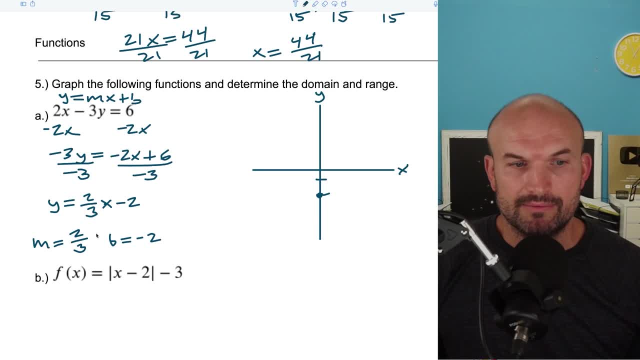 and make a nice little dot, And then we're going to go ahead and follow our slope to another point. Remember, you only need two points to be able to graph the equation of a line. So the slope is that rise over, run the change in the y. 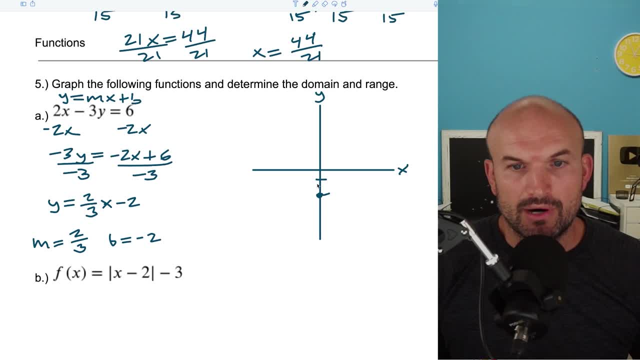 over the change in the x. So to graph this, those 2 thirds, I'm going to go up 2, and then to the right, 3,, 1,, 2,, 3.. Now remember when you have a positive slope. 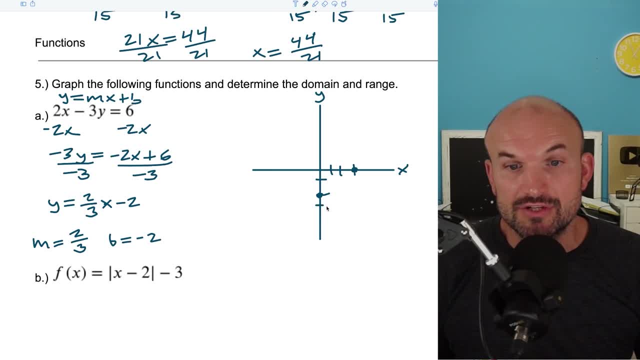 you could also have a negative 2 over a negative 3, right, So you could actually also go down 2 and then to the left, 3, 1,, 2, 3.. Either way, you can see that all these lines or all. 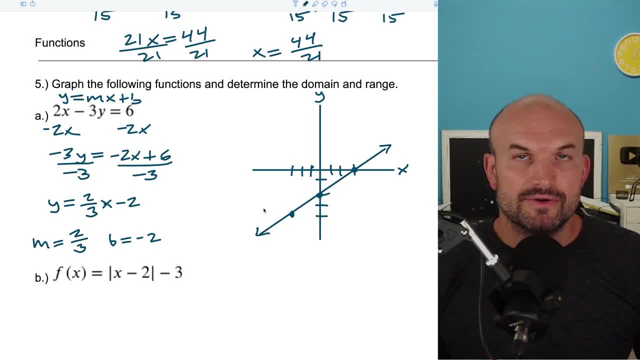 these points are going to rely on this exact same line. So now let's go and identify the domain and the range. So remember, the domain is a set of all x values that make up your graph. So you can see, this graph is continuously expanding. 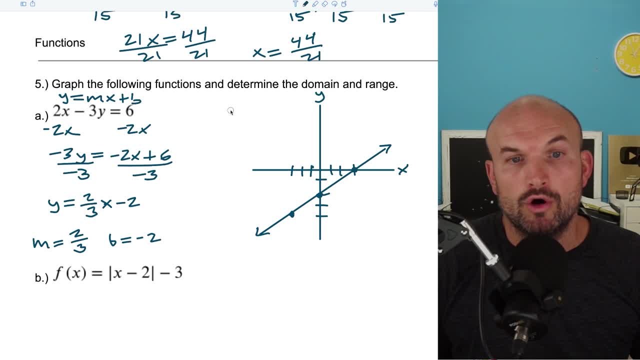 to the left as well as to the right. So the domain is going to be what we call all real numbers. So a couple of different ways we can write the all real numbers. Obviously, in precalculus we get pretty heavy into interval notation, but that's. 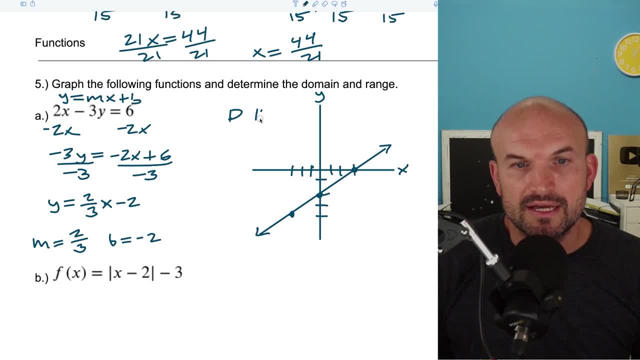 something I want to deal with in precalculus. So for right now I'm just going to use this r with the double line here to represent my all real numbers. You can also use interval notation like negative infinity is less than or equal to x, which 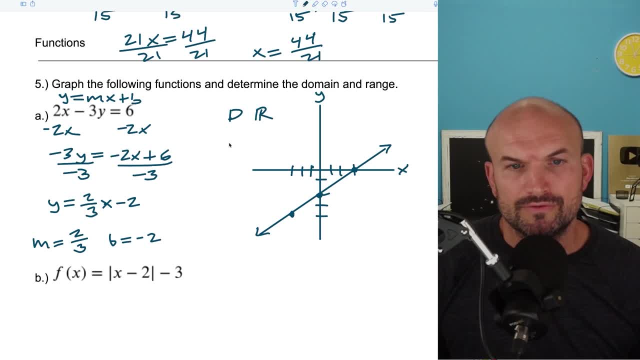 is less than or equal to infinity- And I'll go through some of that interval notation as well- And the range is the set of all y values that make up the graph. And again you can see that this graph is continuously expanding down as far as up. 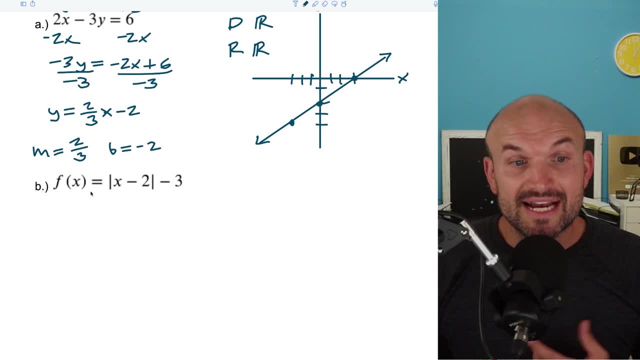 So the range is also going to be all real numbers. All right now. the next function that's really important is going to be this absolute value function. Now, to understand this absolute value function, it's kind of really important to understand what the parent graph looks like. 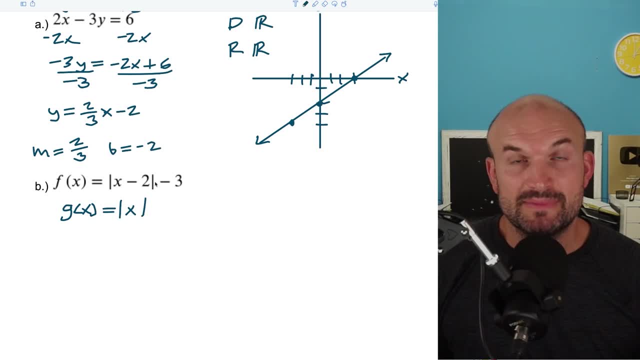 And so let's just call the parent graph here g of x, And that's just going to be absolute x, So that's going to be without any transformations. So if you remember from your study in algebra 2, we kind of looked at this graph. 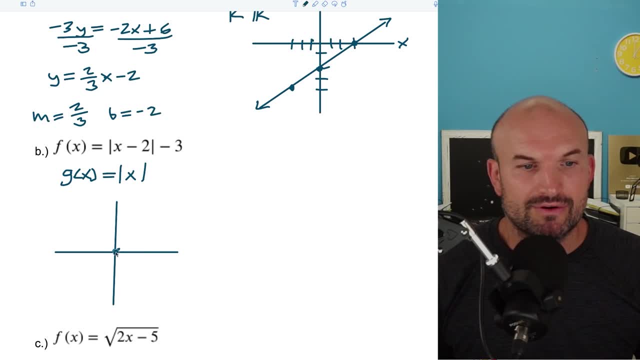 And this graph took the shape of what we call the v-shaped. So what the graph did is it looks something like this And it went over that way And it had this nice little point at the origin, which we call the vertex, which is at 0 comma 0.. 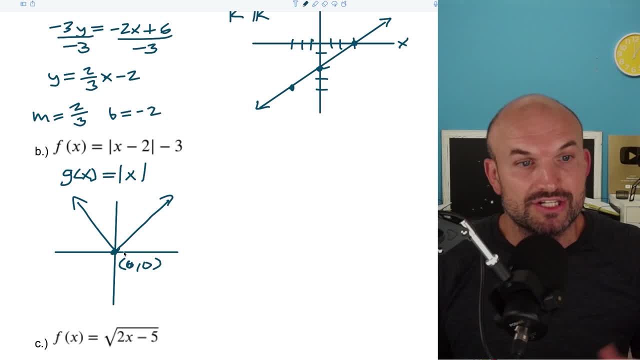 Now, before we kind of understand the transformations or what the new domain and range is of my function f of x, let's go ahead and make sure we understand what exactly the domain is of this function. So the domain, remember, is the set of all x values. 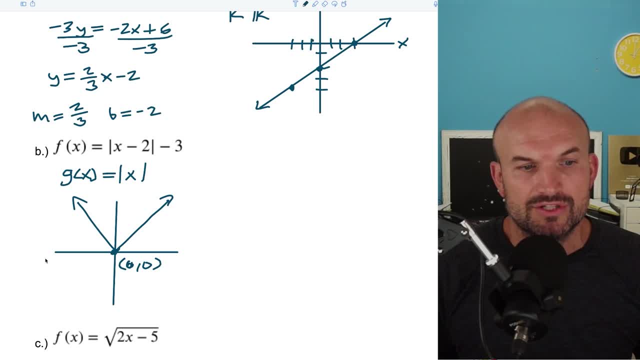 that make up this graph, And you can see this graph is expanding to the left as well as to the right, So my domain here is again going to be all real numbers. However, my range does not expand infinitely down as well as 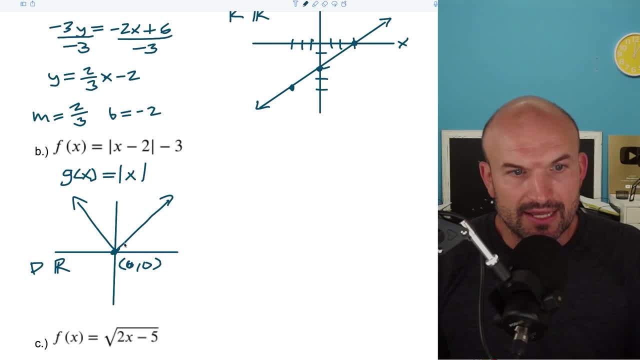 infinitely up. Right, You can see, the lowest point that my y value goes is going to be 0.. Right, It doesn't go below 0.. So my range in this case is going to be, for all y values that are greater than or equal to 0. 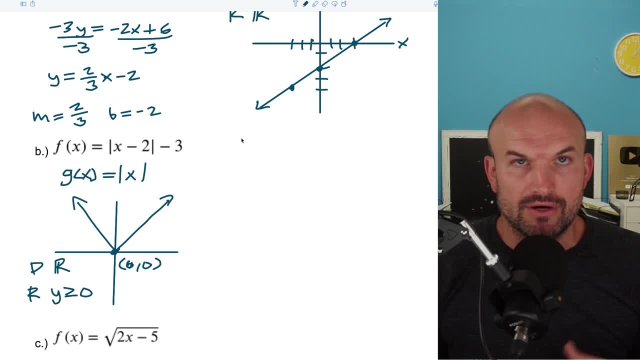 Now we need to understand well what is this negative 2 and what is this negative 3 doing. So one of the things that we probably talked to- or hopefully you talked about- in algebra 2, was looking at the transformations, Right. 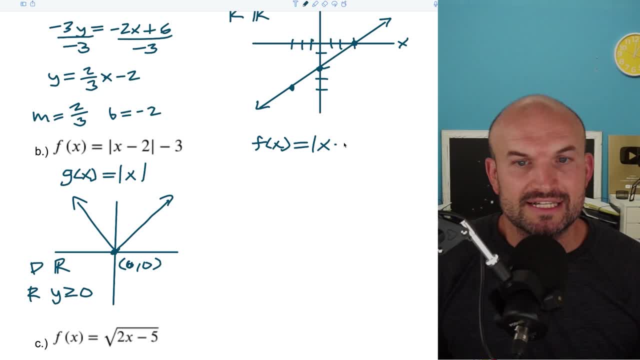 So f of x equals- you might have been familiar with this- x minus h and then plus k. And how did those impact our function? Well, remember, h was your horizontal transformation and k was your vertical transformation, So a lot of students will get it confused. 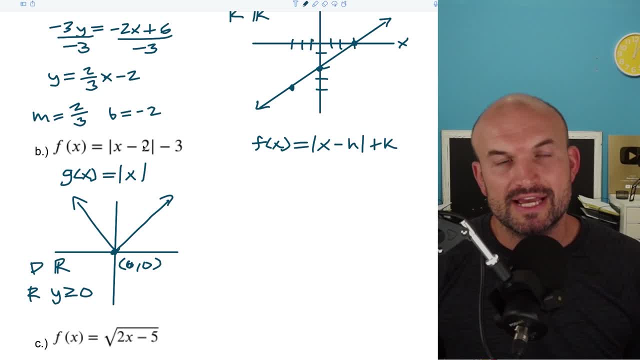 If you recall, if you go to x minus 2, they'll say, oh, that's to the left 2.. And actually it's the opposite. You're actually going to be moving to the right 2.. So what I'm going to do, the reason why it's important to know. 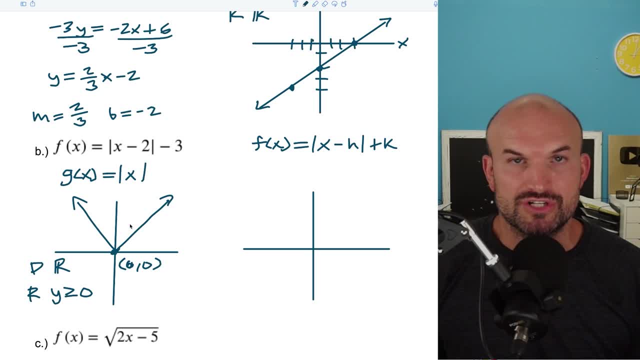 this one point is, rather than trying to graph multiple points of my function, I can just take the one point I know and apply the transformation. So that's going to be shifted two units to the right, And then this negative 3, which is my k. 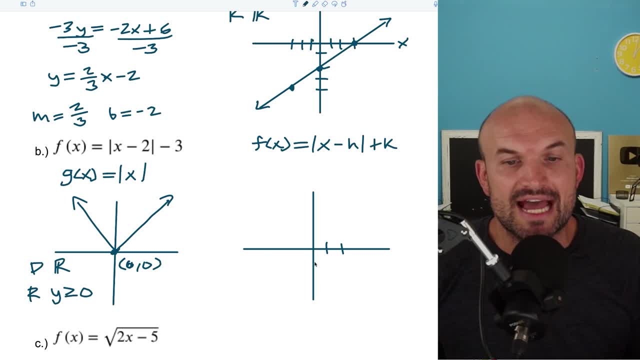 is going to be your vertical translation. Now, when this is negative, you actually are going to go down that many units. So in this case, that's going to be going down three units. So now what I'm going to do is just kind of do my slopes. 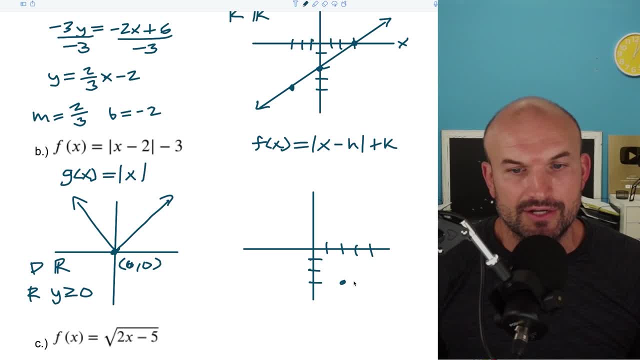 You remember that's over 1, up 1, like on either direction, Right? So I can just kind of go like over 1, up 1,, over 1, up 1.. And I can do the same thing in this direction going from there. 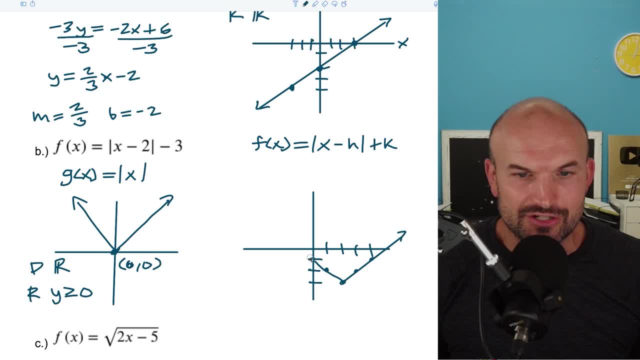 So you don't really need to be perfect. It's perfectly fine Like there's no stretch or compressions, And again, for this video, I'm not going to be as overly concerned right now as far as your shape of the graph. 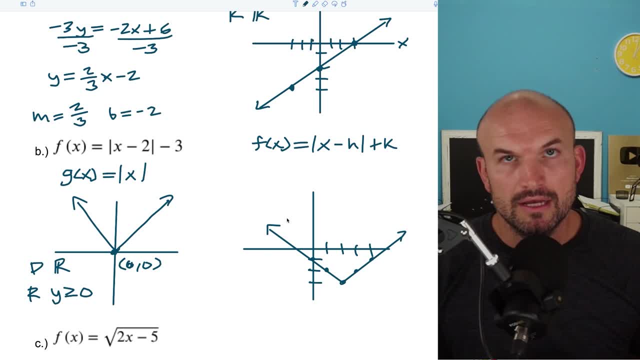 The main thing I want you to be able to understand is how to apply your transformations, and then also what's going to be the new domain and range. So what you can see here is, though this graph got shifted two units to the right. 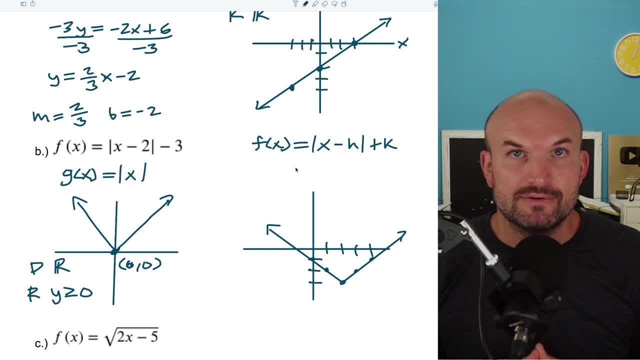 and then three units down. Now what's important is, this graph already had a domain. that was all real numbers. So when I shifted this graph left or right, did anything change with the domain? And the answer is no. So the domain in this case is still. 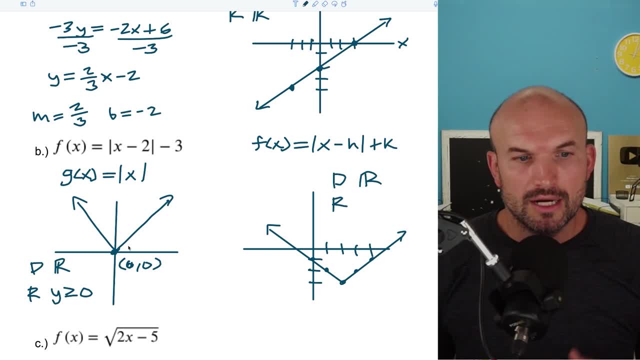 going to be all real numbers. However, what about the range? Previously, the range only went as low as 0. But now, when I shift this graph down three units, you can see now the lowest point of this graph is going to be a negative 3.. 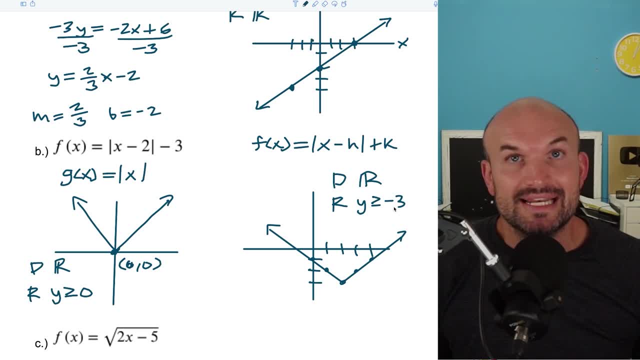 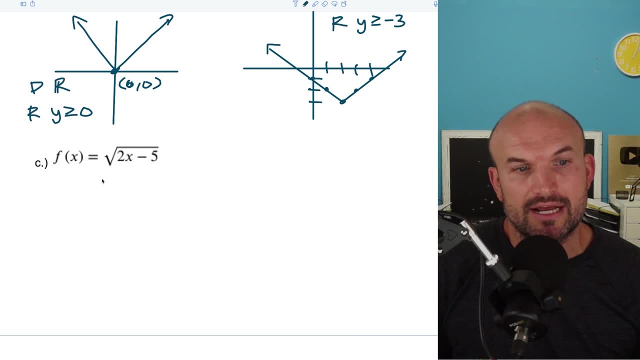 So my range now is going to be: y has to be greater than equal to a negative 3.. OK, now in the next function here we have a square root function. So again we need to understand what this parent graph is going to look like. 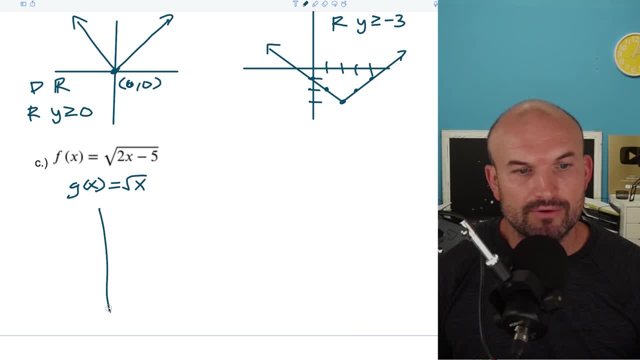 So g of x is going to be the square root of x And hopefully, if you remember, in algebra 1 or maybe even algebra 2, this graph is going to look something like this. So again, let's understand what is the domain and range here. 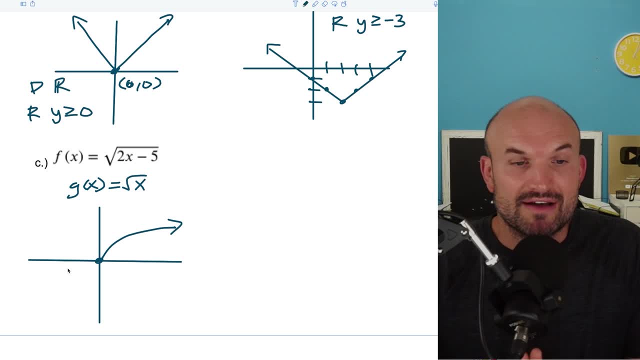 Now, here you can see that the domain or the set of all values that make up this graph is not expanding infinitely to the left and to the right. My domain is only x values that are greater than or equal to 0.. Notice, that's a filled in dot. 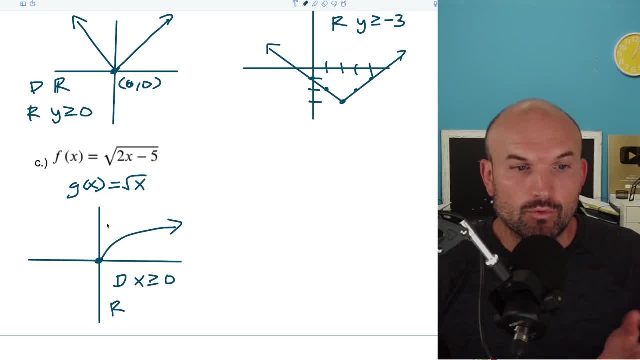 That's why I use the equal to, And my range is exactly the same. The y values that make up this graph are all greater than or equal to 0. So y has to be greater than or equal to 0. So it's just really important to recognize. 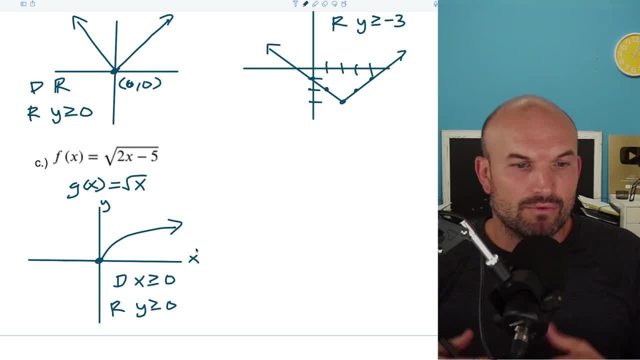 that they have the same domain and range. But again, one's for x values, one's for y values, right, OK? so a big mistake that students will make- and this happens all the time in precalculus, because this comes up time and time again. 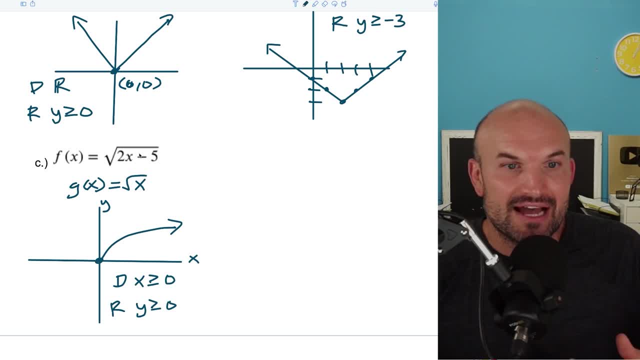 is. students will say: oh, 9 is 5, right, That's going to be OK. it's not left 5, right, It has to be right 5.. But that is incorrect. It's actually not going to be right 5.. 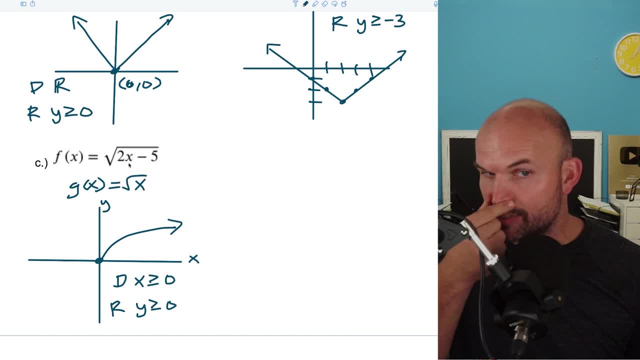 So what we need to understand is we have this 2 here And what that 2 is actually doing is horizontally compressing the graph. Now again, I'm not really going to be concerned about is your graph looking perfect, But I need you to understand that- that horizontal compression. 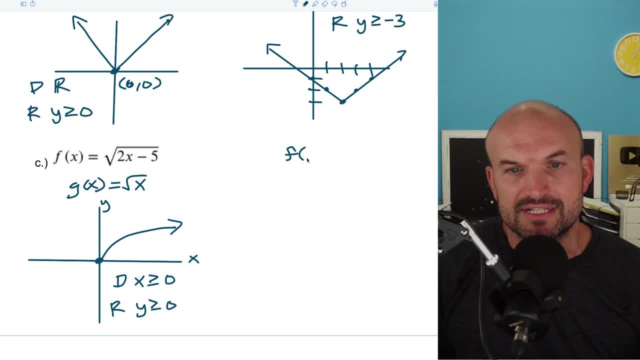 is happening And the way that the reason why it kind of looks is one thing we kind of talk about here- is your transformations of general functions And so going away from the h and the k which we use for quadratics and absolute value functions. 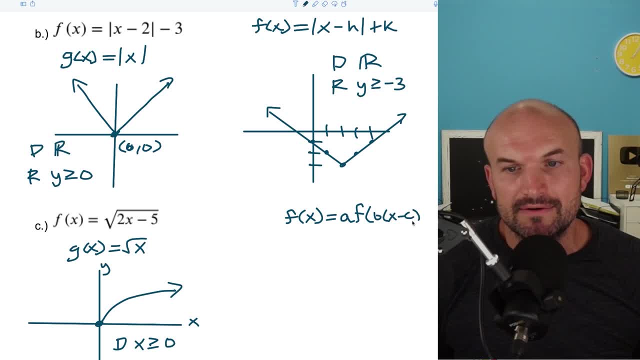 another thing that we kind of look at is your b times x minus c plus a, d. OK, And I kind of ran that off the side so I'll make sure I include that over here. But the really important thing is I want you to understand is your c. 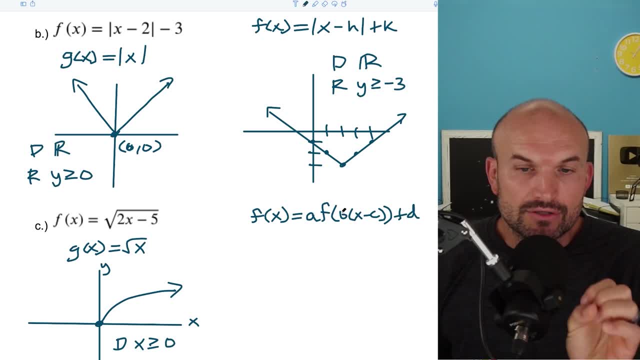 or this horizontal transformation only makes sense when your horizontal compression is being factored in. OK, It's not factored out. So you can see here, this 2 is not factored out, right, It's just 2 times x minus 5.. 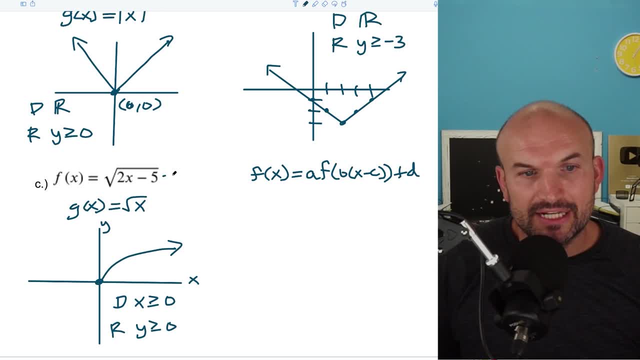 So to actually apply the proper transformation here, what I simply need to do is I need to factor out the 2 from the 2x, as well as from the 5.. So when I do that, what I'm going to be left with is a 2. 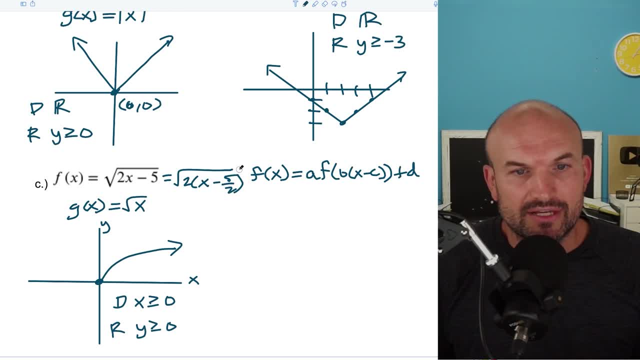 times x minus a 5 halves. Now a lot of times students will get confused here and they say: how did you do that? You can't factor out a 2 from 5.. 2 does not divide into 5.. 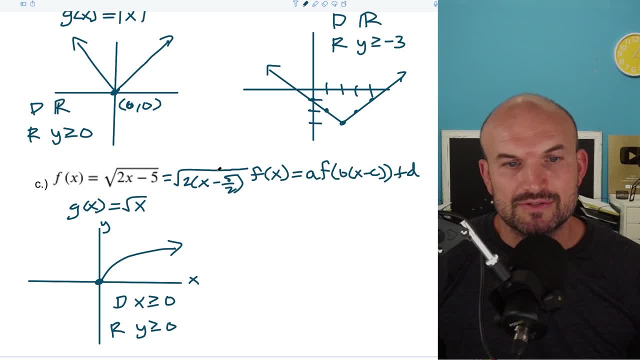 And you're right, It doesn't at least evenly. However, notice what happens when I check my work. 2 times x is 2x. 2 times a negative 5 halves is going to give you a negative 5, right. 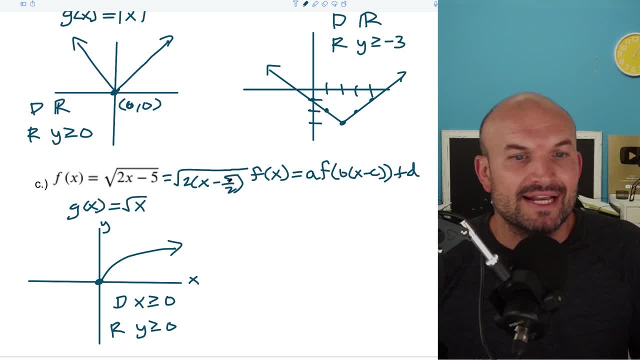 So when you're factoring out something that's not divisible, you can just rewrite it and leave it into that factored form. So now we need to understand, like all right, what are these transformations then? that's happening here, Like here's the graph. 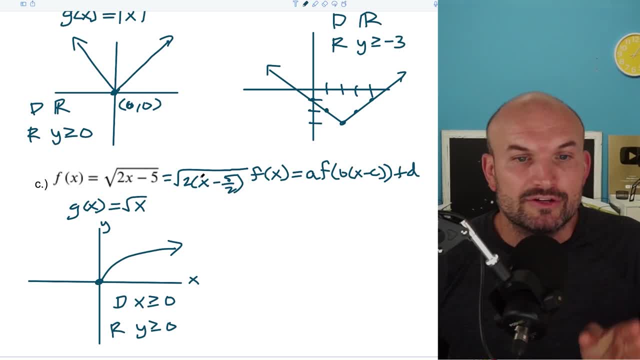 So now my graph is not shifting 5 units to the right, Do not make that mistake. The graph is shifting 5 halves to the right. all right, Now again going back to that one problem, if you remember, in linear equations, 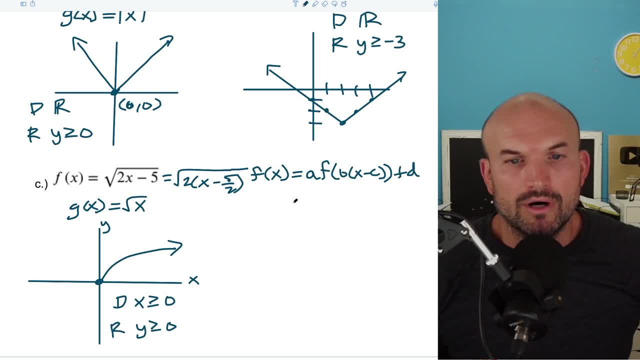 like: how do you graph something when it's a fraction? Well, just remember, like 5 and 1,, 5 halves, right. We can rewrite that as a mixed number: 2 divides into 5, what 2 times with a remainder of 1.. 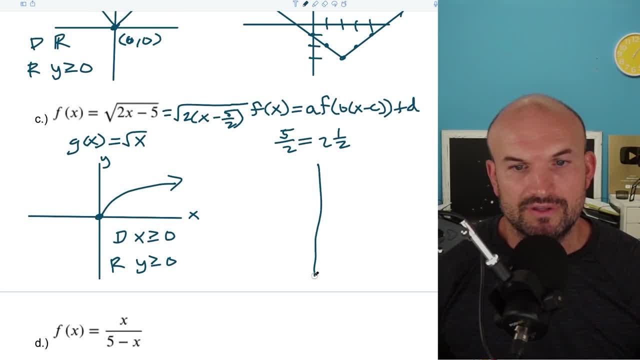 So that's going to be 2 and 1 half. So let's go ahead and graph what this graph would look like. So, again, I'm going to go ahead and draw this graph here. So there's my graph. It's being shifted over. 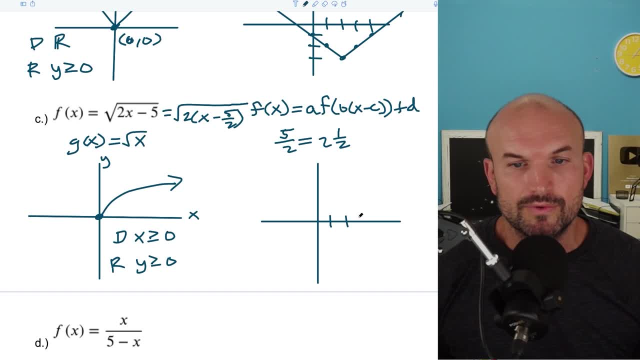 This point is being shifted over 2 and 1 half units, So 1,, 2, 3.. So 1, 2, and we'll go like 2 and 1 half. Now again nothing's happening vertically, right. 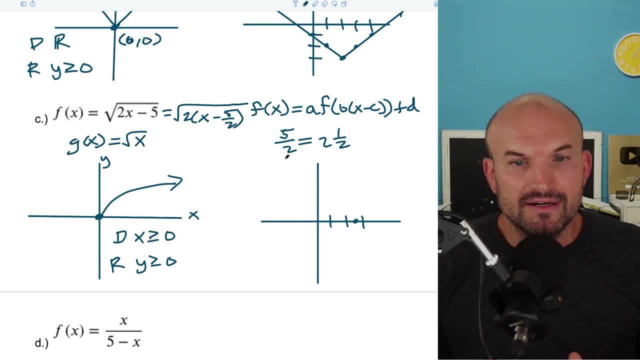 I'm not adding or subtracting anything, So the graph is going to stay there. Now you could say the graph is being horizontally compressed, right? So it's going to kind of look, maybe horizontally smushed. But again my main point I'm trying to make. 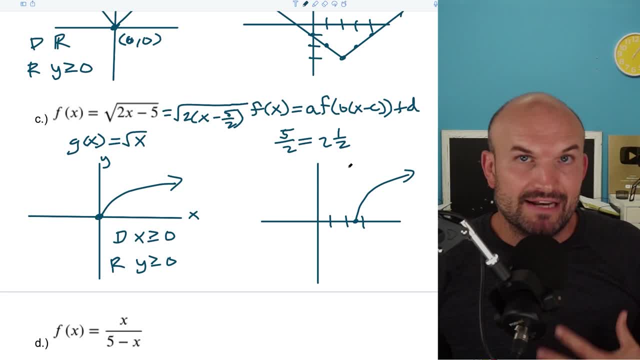 is if it's smushed or if it's stretched. it doesn't really matter. The domain of this graph is still going to exactly be the same. Now the domain again is: how far left does the graph go? How far right is the graph going? that is making up the graph. 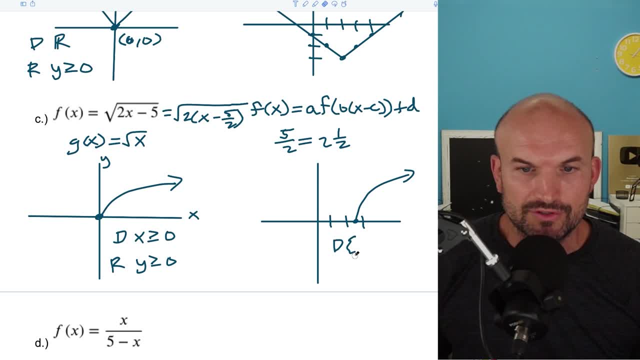 And in this example you can see that the graph- I don't know why I did the interval notation here, I'm just going to leave it as an inequality is going to be all x values that are greater and equal to a 5 halves. 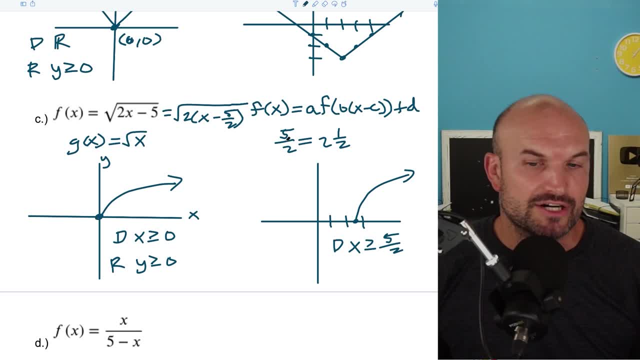 And again, you can use a mixed number, but I prefer to use the improper fraction. OK, Now, as far as my range goes, the range is unchanged. The only thing that happened was a horizontal shift, right? So when you just have a horizontal shift, 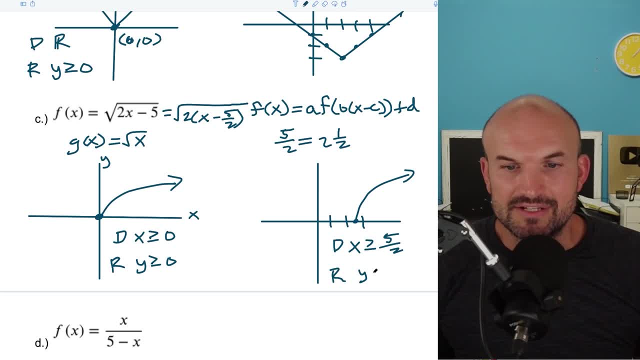 the range is going to be what it originally was, which is going to be all y values that are greater than equal to 0, right, The range is only going to change when you have a horizontal or when you have a vertical change. that was going on. 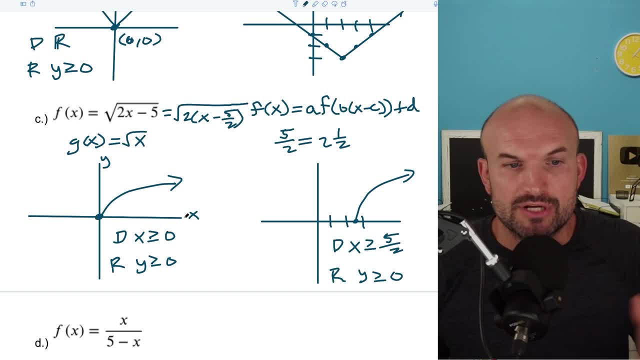 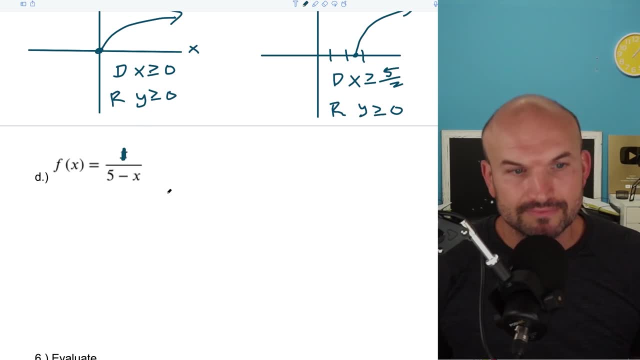 Since there was no horizontal change, it was only horizontal. Since there was no vertical change. I'm sorry, it was only horizontal. The range just remained the same, And that's actually supposed to be a 1, so that is incorrect. 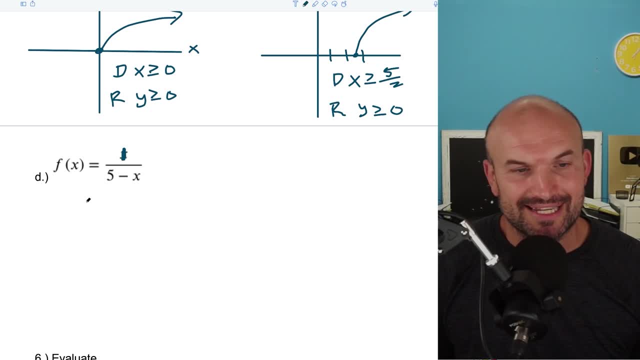 So the last one I want to do- and the reason why I know it was a 1 is because I was expecting we're going to get into rational functions here later. but g of x equals a 1 over x, So it's important that students also 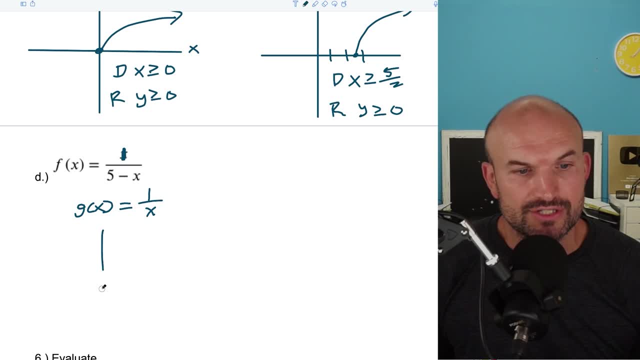 recognize this function, which we call the reciprocal function. So if you kind of remember this one, this is going to be a pair of hyperbolas And again, the important thing here is that we have some asymptotes right. So this is that one function that we kind of introduced. 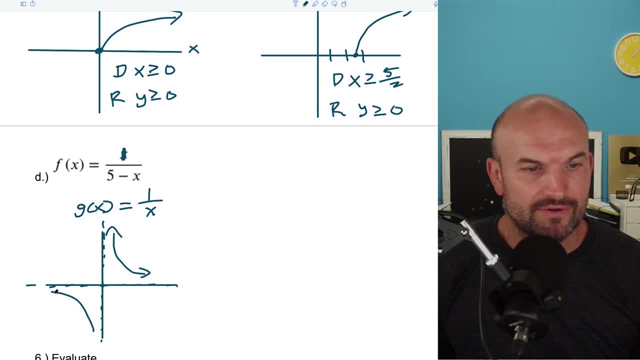 with asymptotes And the graph looks something like this going in from there. Now again, this is again another problem where you can see we actually have a b in front right. So if you were to actually rewrite this, you could rewrite this as a negative: 1 times x plus 5.. 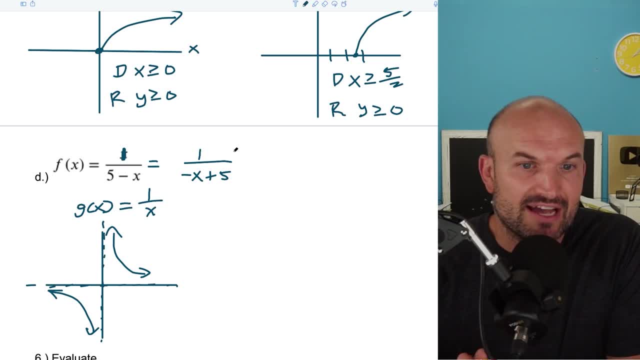 And again you can see that we have a horizontal transformation: that plus 5, but again we have this b. So what we simply need to do now is actually factor that out. So I'm going to factor out a negative. That's going to give me an x minus 5.. 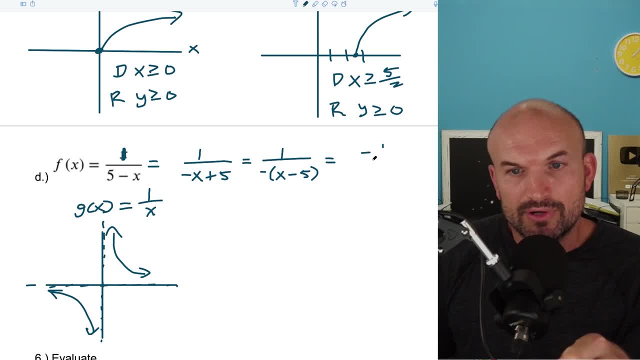 Now, as far as this negative, you can leave it in the denominator or you could also put it up top. There's a lot of different ways we could go ahead and write this problem Now, if you put it in the bottom or on the top. 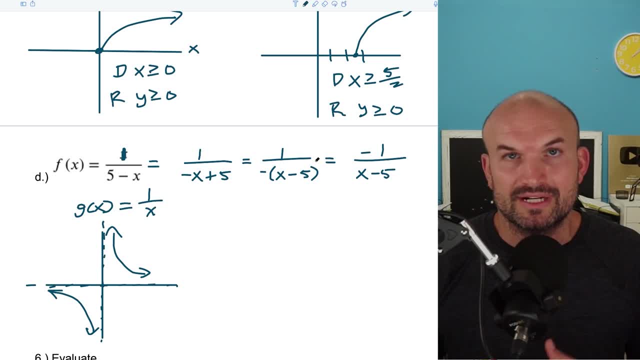 it doesn't really matter. I don't want to get into the weeds because this is again something we're going to deal with more in depth in precalculus. But if you had it in the bottom, then that's going to be a reflection about the y-axis. 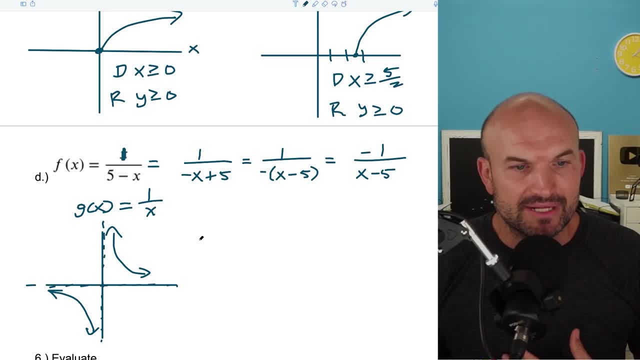 And putting it up top is going to reflection about the x-axis. And again, it doesn't matter, because if you look at this graph, this is what we call an odd function- If you reflected about the y or if you reflect about the x. 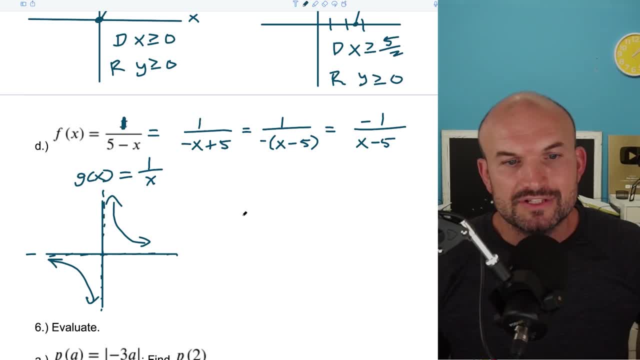 you're still going to get the exact same reflection. So you're going to get the exact same reflection. So that's going on okay. So that's kind of an important thing. I'm just going to put it up top because that's typically how I like to see it. 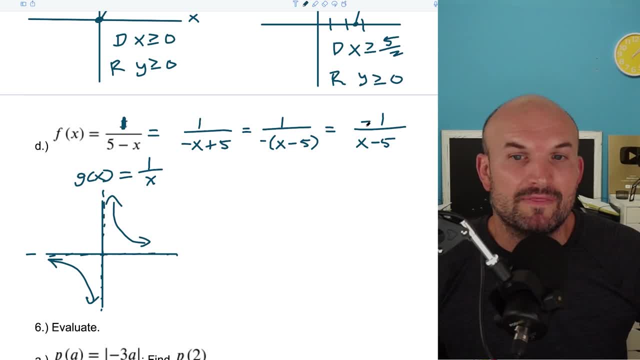 So what's going to happen is now: this graph is being reflected about the. remember, there's a reflection that's going on, right? So the graph is being reflected about our x-axis. okay, So I'm going to flip this graph about the x-axis. 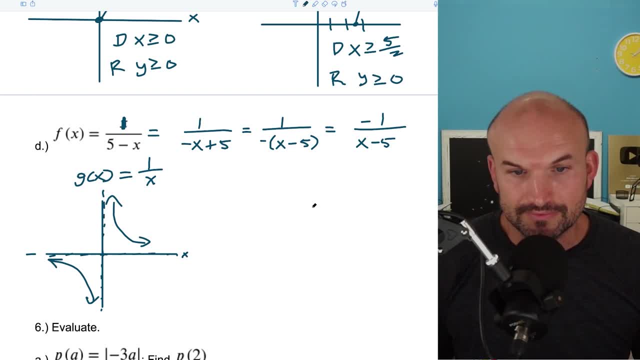 and then what else do we have Now? we're shifting the graph five units to the right, So let's go ahead and graph what this graph is going to look like, So I'm going to draw. my asymptote, though, is being shifted right. 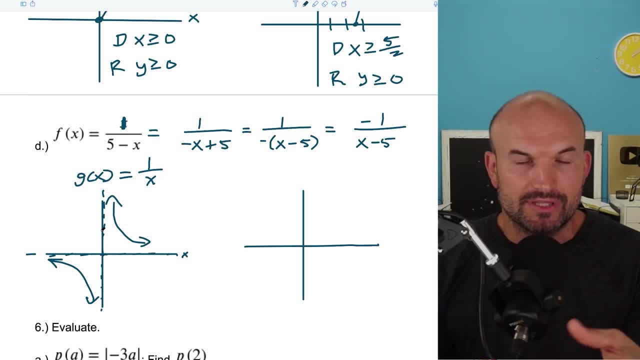 So in this case, our points, or at least the things that we're going to apply with our transformation, are going to be our asymptote. So one, two, three, four, five, I'm going to draw this new vertical asymptote. 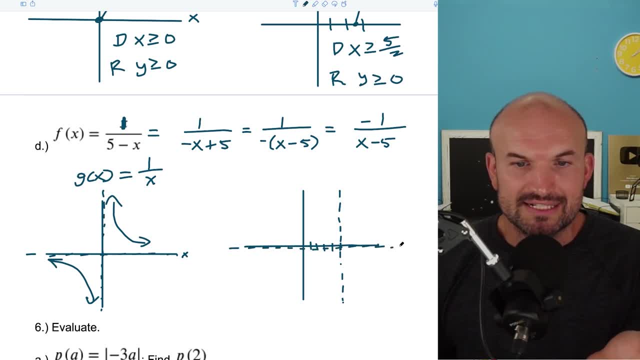 Now the cool thing is, you know, up and down horizontally or vertically. my vertical asymptote didn't change right. The only thing that really happened was we were doing a horizontal shift, So now I just need to graph the reflection of this graph. 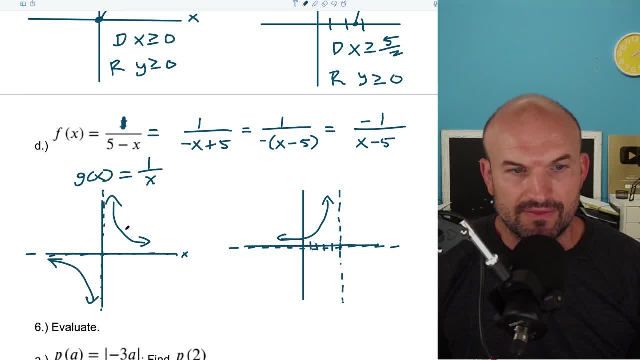 which means it's going to basically be flipping: So this goes up here, that goes down there. So the graph is going to look something like that. Now let's go and talk about the domain. Now, as far as the domain, I'm not going to write this in interval notation. 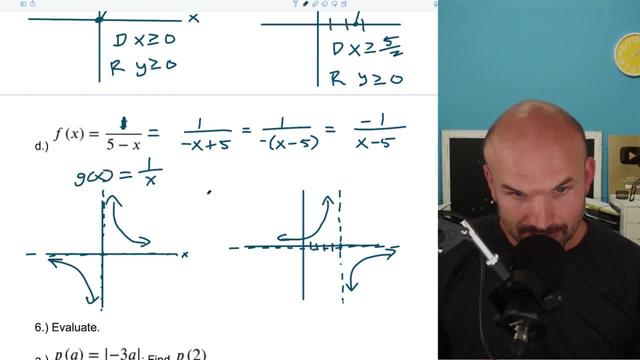 because that's usually really confusing for students. I will just kind of do a. I'm just going to kind of do a set notation for this. So the domain it looks like it's going to be defined. Looks like this graph is expanding to left and to the right. 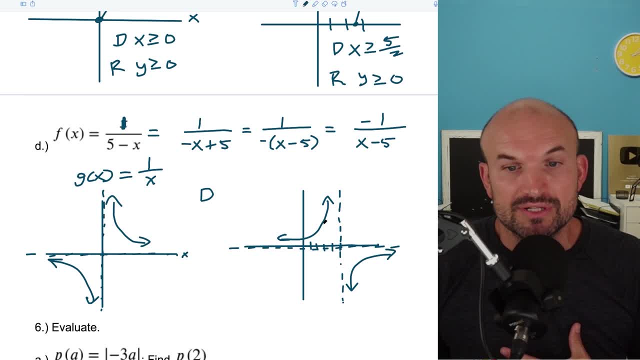 for all values except for the asymptote. So it's really true for all real numbers, except for when x equals five. So my domain, I'll say it's going to be true for all real numbers such that x cannot equal a five. 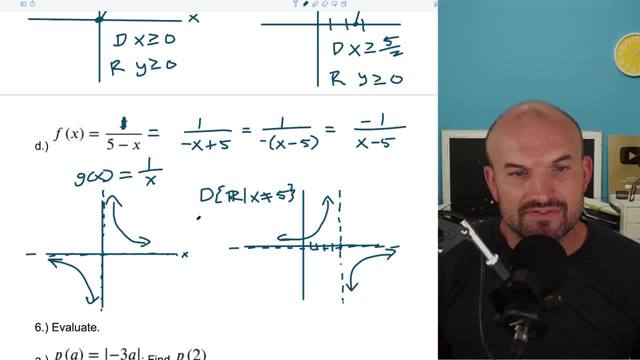 And why can I equal five? Well, because that's a vertical asymptote, All right. Now, as far as the range go, we kind of have the same thing right. It doesn't look, it's not defined at your horizontal asymptote. 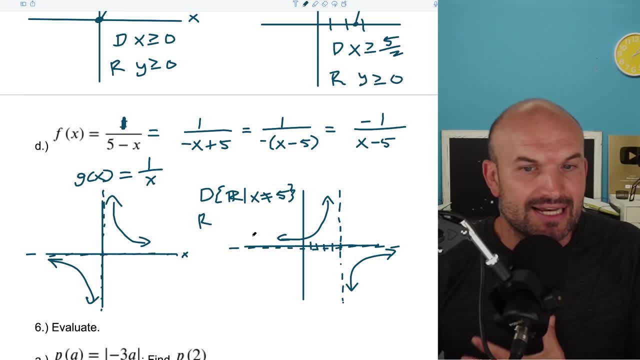 It looks like it's approaching that value from the left and from the right, but it's actually not crossing at any one of those values. So, again, the y coordinates that make up this graph is going to be all real numbers, except y cannot equal zero. 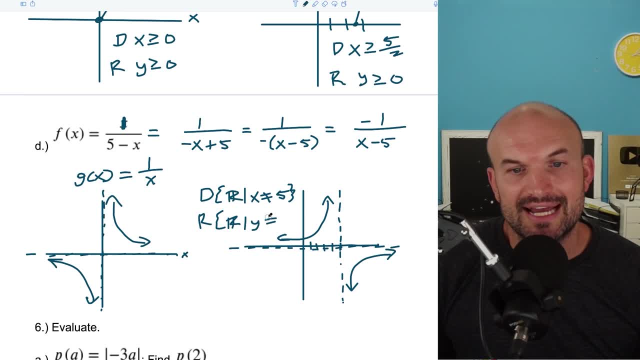 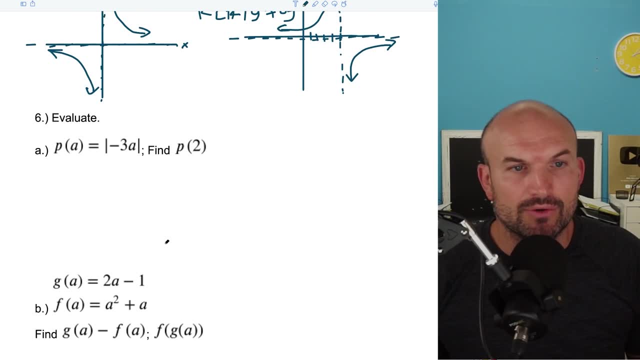 So I'll go ahead and write this as all real numbers, such that y cannot equal a zero. All right, So now let's go and get into the functions. Hopefully that was a good kind of little review of at least domain range, And like the graphs. 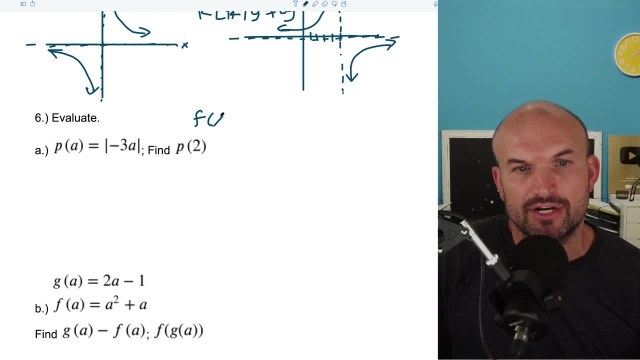 now the next thing is like the function notation, And just remember function notation. you know we have an f of x equals a rule, right? So the f is really just going to be the name, X is going to be your input value, right? 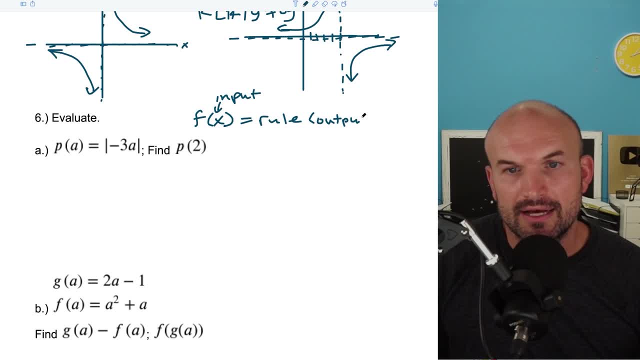 And your rule is also sometimes called our output, right? So remember, the input is going to be like your domain, The output from the rule is also going to be your range. Just kind of make a connection between those two. But one thing that's going to come up again and again: 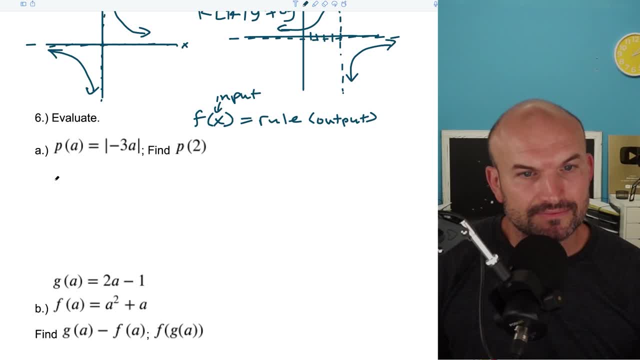 is going to be evaluating, you know, for our functions. So in this case, if I say p of 2, what I basically want to do then is be able to say: all right, well, what is the value of the function at 2?? 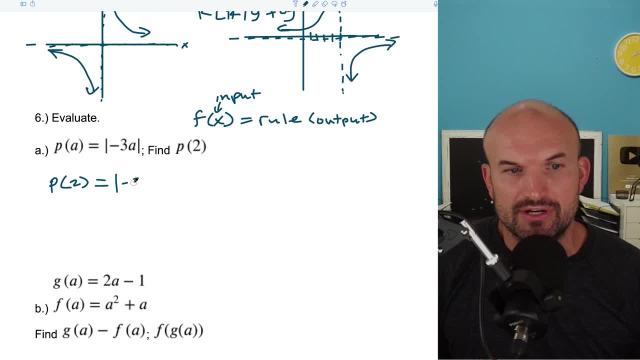 So what you're simply going to do is, whenever you see an a, you're just going to replace that with a 2. So I'll have a negative 3 times 2.. OK, so negative 3 times 2, that's. 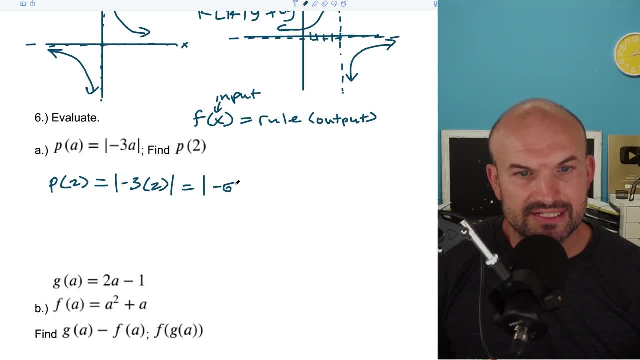 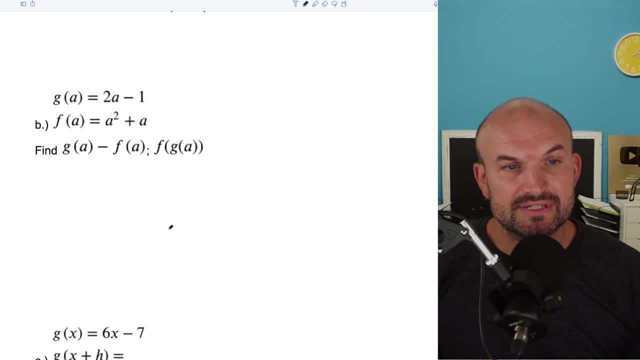 going to be absolute value of a negative. let's see a negative 6,, right, And the absolute value of a negative number here is just going to equal a positive 6.. The next thing we can do is like operations. So you just remember like we can also add, subtract, multiply, divide operations. 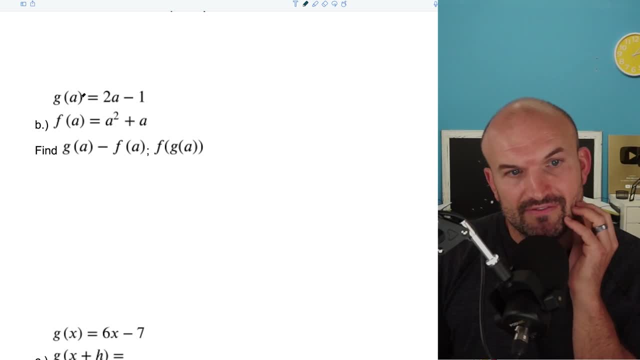 As well as compose operations. So in this example I have g of a, which is 2a minus 1, and f of a, which is an a squared plus a. So how would we subtract them? So you know, if you just kind of rewrite this, 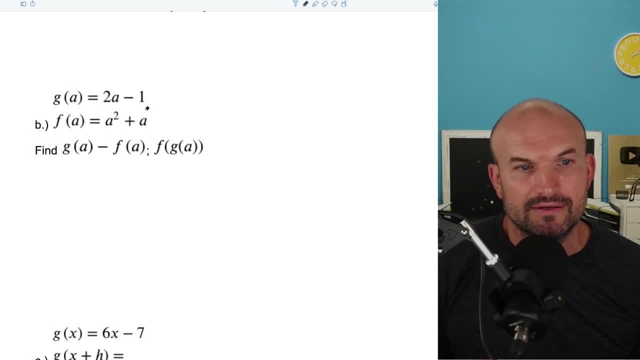 well, really, g of a is equal to a 2a minus 1,, right? So what I can do is I can just replace this with a 2a minus 1, and then minus an f of a, which is what. 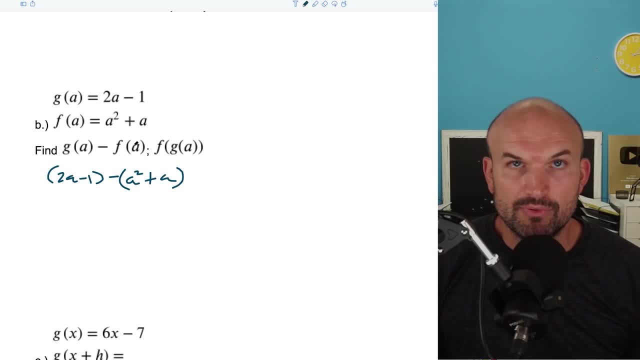 A squared plus a. OK, now again, it's really important to notice. I'm using parentheses here, Because again, you're not subtracting the a squared, you're subtracting an: a squared plus a. So what I'm going to do is, before I 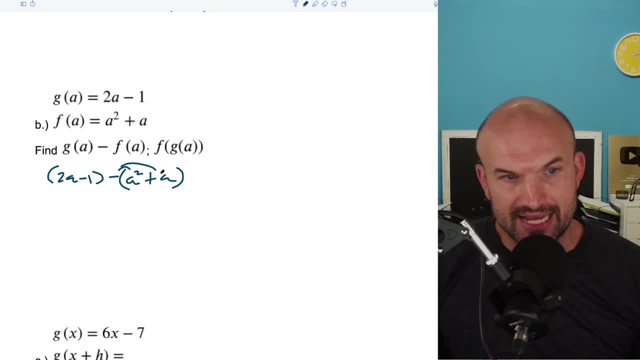 do any work, I'm going to get rid of my parentheses by distributing this negative Over here. I don't really have any operations that's being applied to this, So therefore I can actually just drop these grouping symbols. So therefore I have a 2a minus 1.. 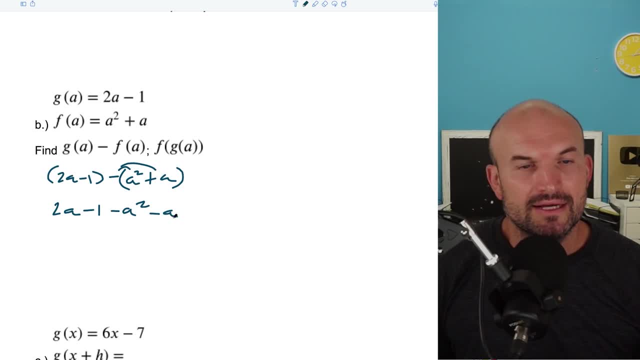 This would be a minus an a squared and this would be a minus an a. Now, in this case, what you can simply do is just kind of rearrange everything, So therefore everything's kind of grouped together. So this would be a negative a squared plus 2a, minus an a minus a 1, OK. 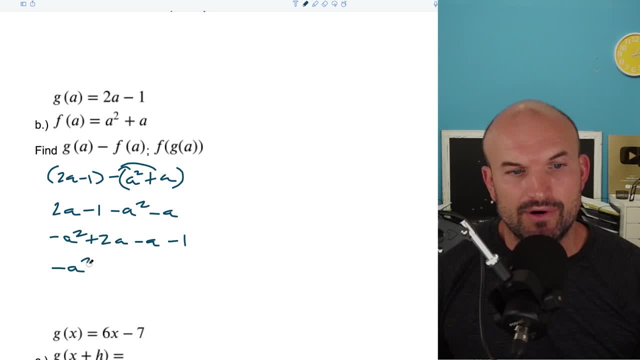 And 2a minus 1 is just going to be an a. So therefore I have an, a squared. Let's see that's going to be what: a plus a minus 1.. Now, composition is kind of a fun one. 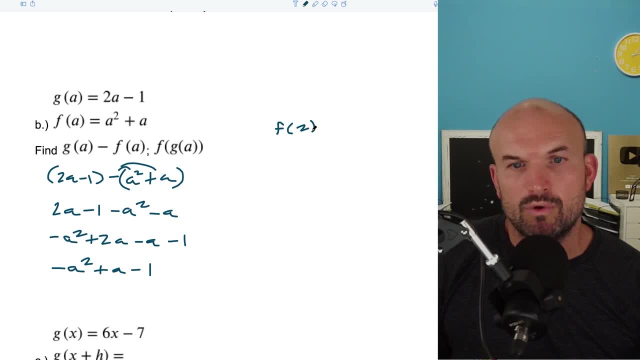 Because if you think about this, like if I did f of 2, what would that be? Well, f of 2 is just going to be now a 2 squared plus 2, right, 2 squared is going to be a 4 plus 2, which is equal to a 6.. 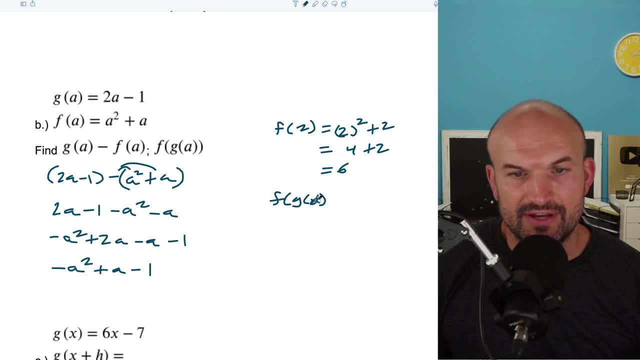 So if I said: what is f of g of a? Well, I'm sorry, g of a, not g of x, then what would you do? Well, then you'd say, all right, well, I'm just going to do. 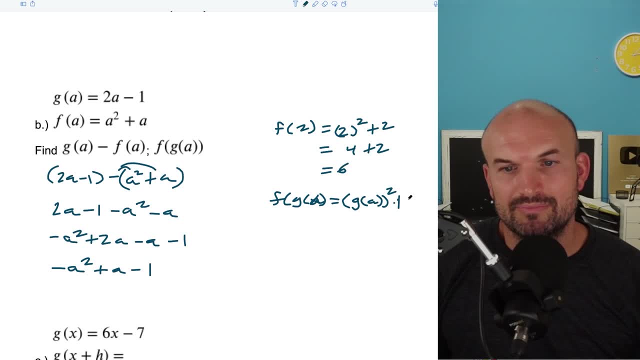 a, g of a right quantity squared plus 2.. Like whatever is as your input value, that's just simply what you're going to plug in to your function, right? So I mean it's like it doesn't make any difference. 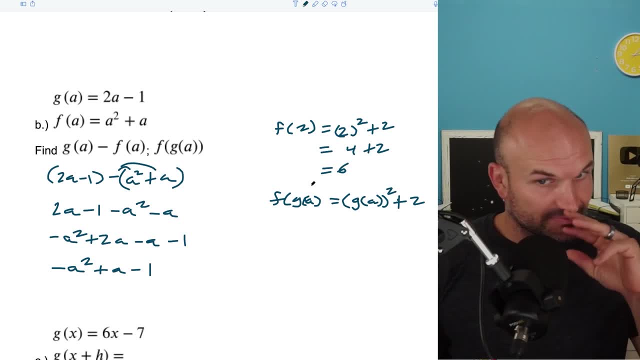 It doesn't matter whatever you're putting into your input value. Now the cool thing is, though, we actually know what g of a is right. We are given g of a. g of a is 2a minus 1.. 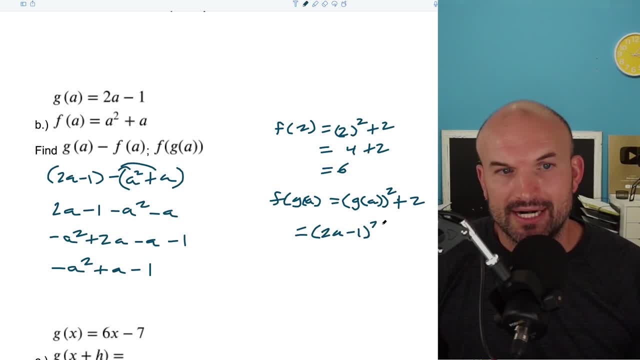 So therefore, that's equal to a 2a minus 1 quantity squared right, And then we're just going to be adding a 2, right, Or what was this? f of g of a. So f of g of a, or it was f of a. 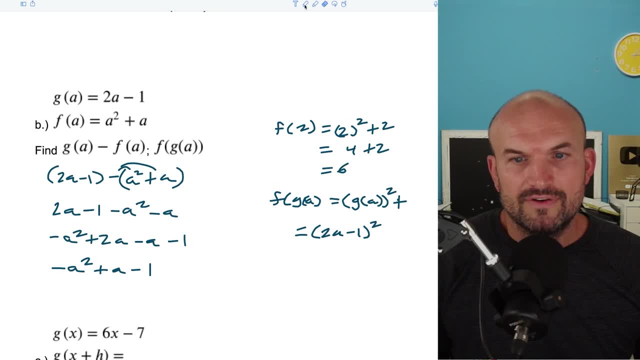 I'm sorry that would be incorrect over here. This would be a g of g of a squared plus a g of a. There we go OK. so then a plus here is going to be what g of a is, which is a 2a minus 1.. 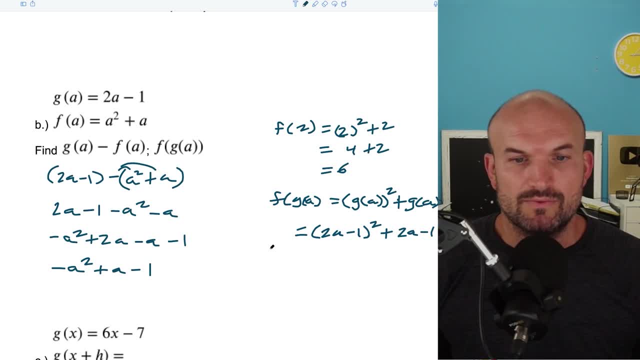 OK, so now we need to remember well, how do you multiply out a 2a minus 1?? Well, remember, 2a minus 1. squared is a 2a minus 1 times a 2a minus 1.. 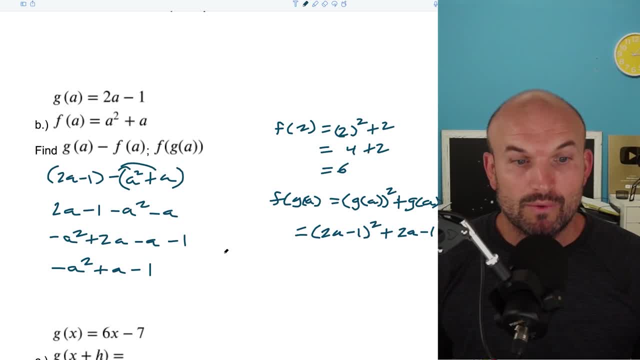 Do not distribute that squaring to both those terms, So what we actually need to do is multiply that out. So this is actually going to look like a 2a minus 1 times a 2a minus 1 plus a 2a minus 1.. 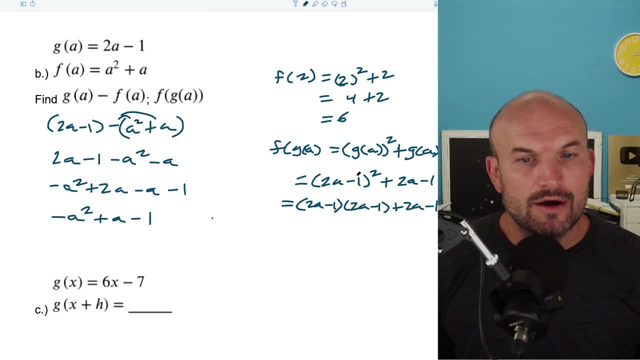 OK. so very important that we have that kind of organized. And now what we can do is just go and apply your distributive property here and multiply every term by every other term. I'll kind of move this to the left: 2a times a 2a is a 4a squared. 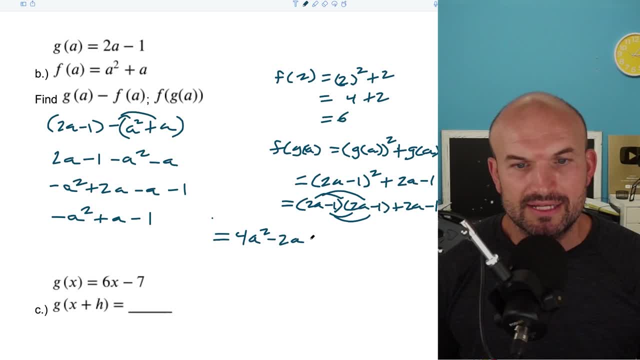 2a times negative 1, so that's a negative 2a. Negative 1 times 2a is going to be a negative 2a And negative 1 times negative 1 is going to be a positive 1.. 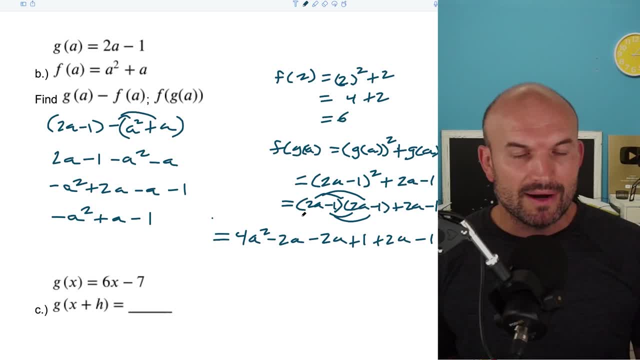 And that's again plus a 2a, minus 1.. OK, so now I can kind of group my terms. Notice how this negative 2a and this positive 2a, those are going to add to 0. They don't cancel out. 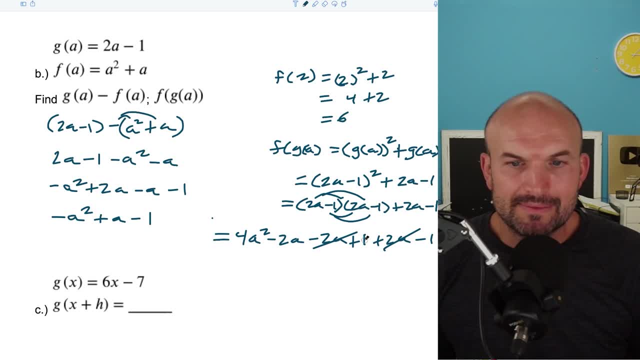 They just add to 0. But that's why I'm kind of drawing the line here. The same thing's happening with the 1 and the negative 1.. Those are going to add to 0. So, therefore, I'm going to be finally left with a 4a squared minus a 2a. 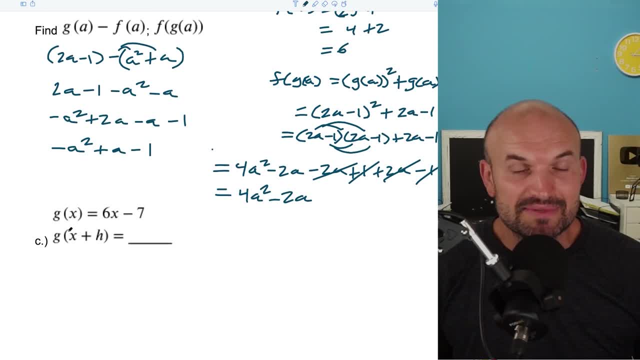 In the next example. now we're just going to do the same thing, But you can see, sometimes it can even get more confusing, right? What if I have this expression x plus 8?? So again, like do the same thing. 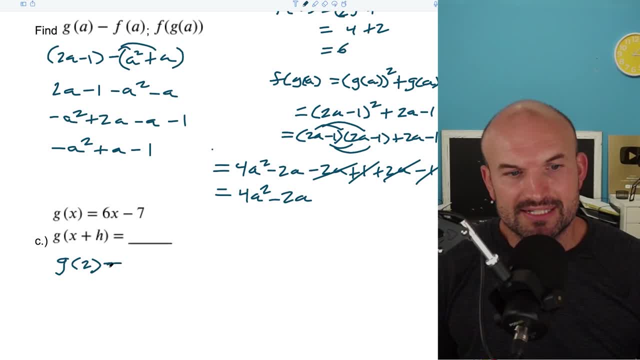 Like g of 2, what would that be? Well, if I said g of 2, then you do 6 times 2 minus 7, right, And so 6 times 2, that'd be a 12 minus a 7, which is just going to equal 5.. 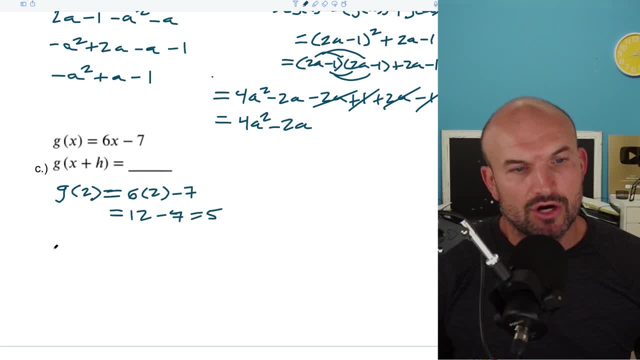 And if I said: what about g of h of x or g of whatever? So what if I did a g of a x plus h? Again, just follow the process. You plug in a x plus h in, for your input variable in this case is x. 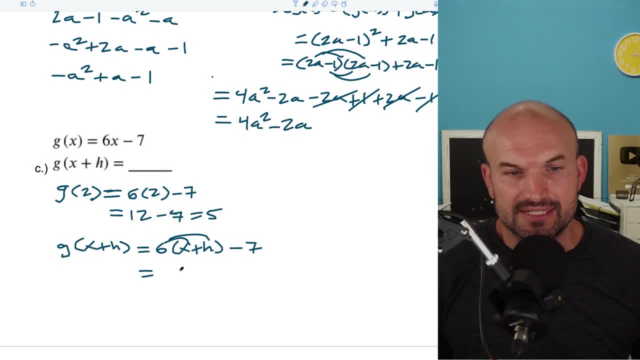 That's going to be minus 7.. Now, in this case there's really nothing else. I'm going to be able to kind of simplify here: 6 times x is a 6x. 6 times h is going to be a 6h. 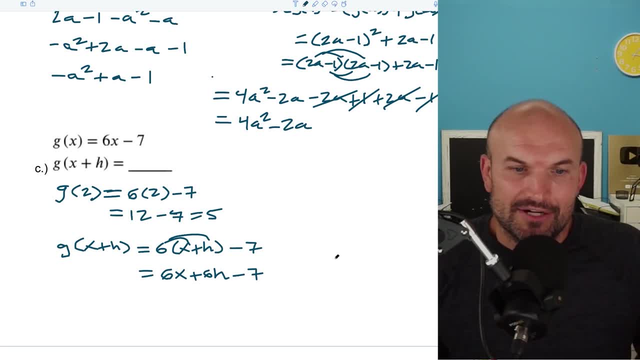 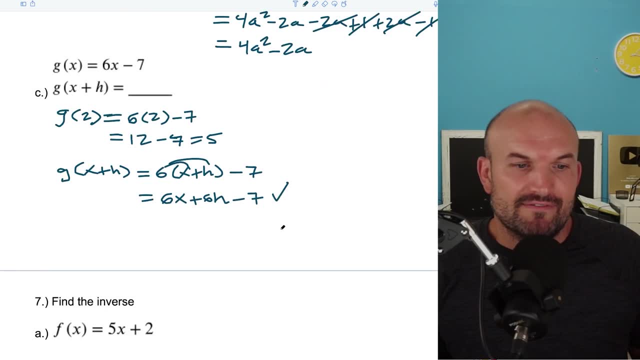 And then that's going to be a minus 7.. And that's kind of basically it. Like we have multiple variables, it's just basically being able to apply that operation or just being able to apply substituting a value. that's going to be most important. 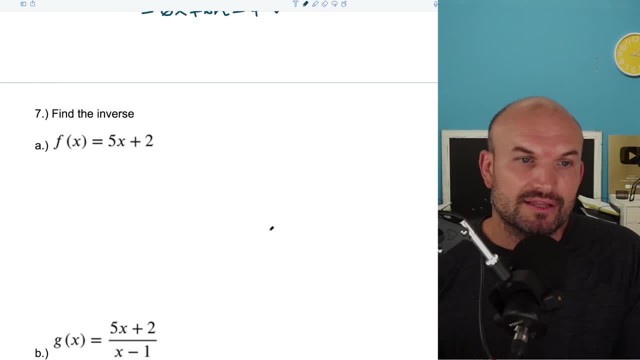 Now, another thing that we're actually going to spend a lot of time going further on in precalculus is finding the inverse. But I think it's just really important to kind of go through the findings, Finding the inverse algorithm, just to kind of remember, because you know it is something. 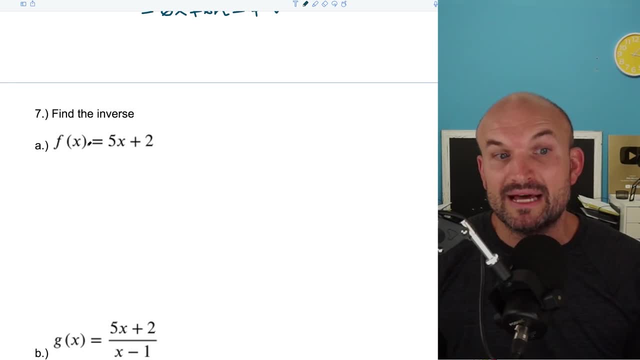 that we talk about a little bit in algebra too. that's going to be beneficial for you because in precalculus we'll go through much more deeper kind of examples. So the important thing here to find the inverse is just replace your f of x with a y right. 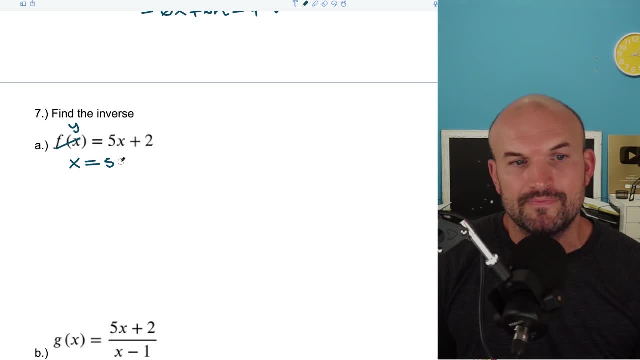 And then what we're going to do is we're going to be swapping the variables, So x is going to equal a 5y plus 2.. And now you're going to go ahead and solve for y, So I'll go ahead and subtract the 2.. 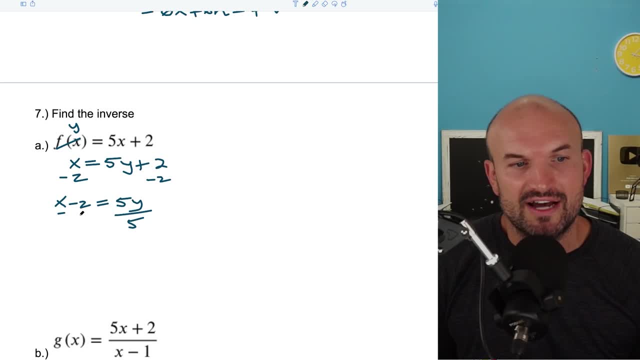 So I have: an x minus 2 equals a 5y, And then you divide by 5.. Okay, And you can say y is going to equal a x minus 2 over 5, right Now, again, this is the inverse right. 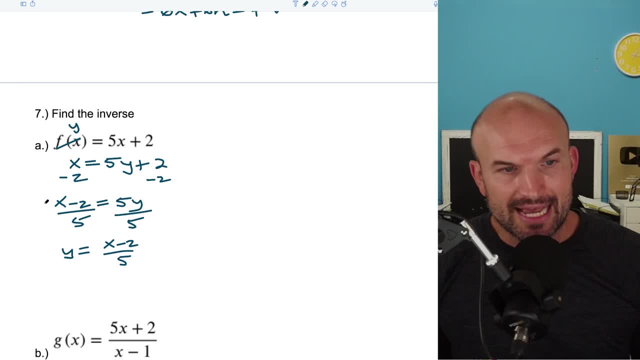 So we can rewrite this using like our inverse notation, And you can write that like negative 1 if it was an equation of y, Or you could also just say like f of inverse of x, So this little negative 1 up top, And then you could leave it like this: 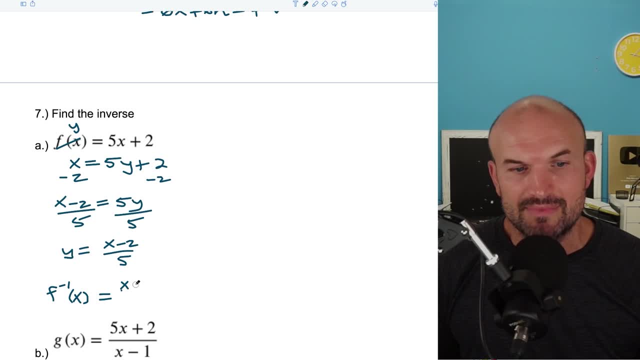 Or you could also distribute the 5 to both of these terms. right? You could leave this as a x minus 2 over 5.. You could rewrite this as a x over 5 minus a 2 over 5.. Or a lot of times. the preferred way we'd write this is a 1 fifth x minus a 2 fifths right. 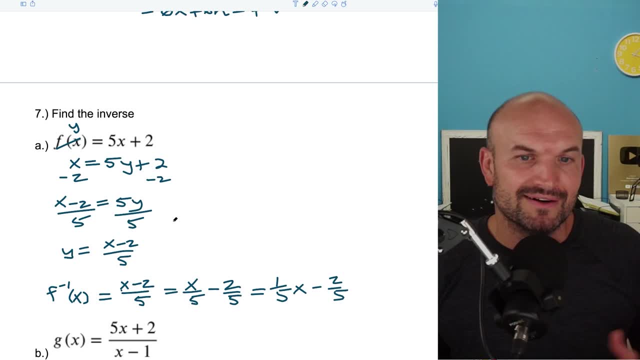 And you could write the slope and the intercept from there. Remember, a graph and its inverse are reflected about the y equals x line And that's why we swap those coordinate points. Also, the domain and the range, if you remember, are swapped in that case. 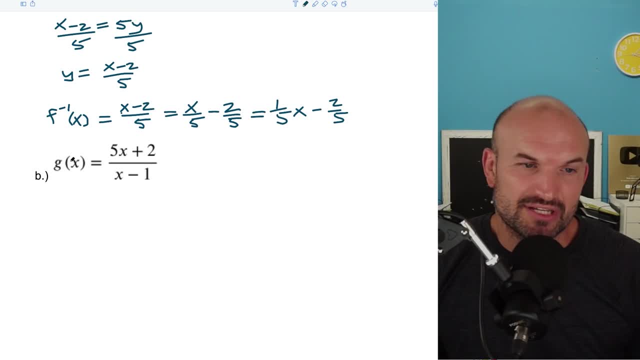 So this is a really important problem. You know it actually comes up in pre-calculus a lot, But I figured it'd probably be a good one to kind of cover here Just again to kind of work through that algebra right. 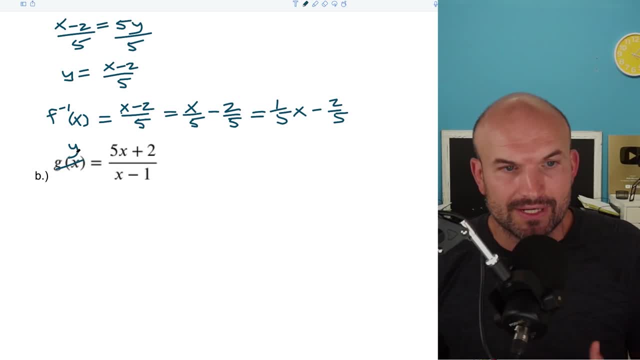 You replace g of x with g of y, Right, You replace g of x with y, And now what we're going to do is swap our variables, So x equals a 5y plus 2 over a y minus 1, OK. 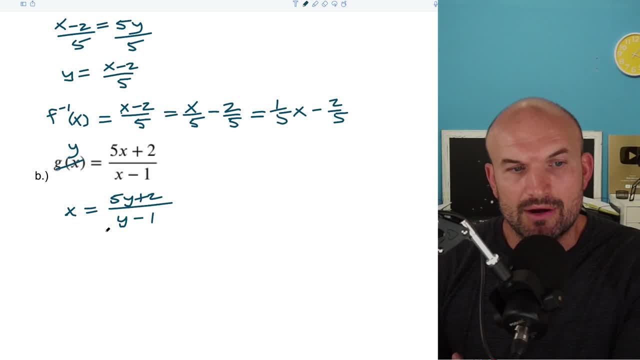 Now what we need to do is go ahead and solve for y. So how do we do that? And the reason why I wanted to cover this is because this is just really important. as you're getting prepared for pre-calculus, This kind of like solving technique just comes really in handy. 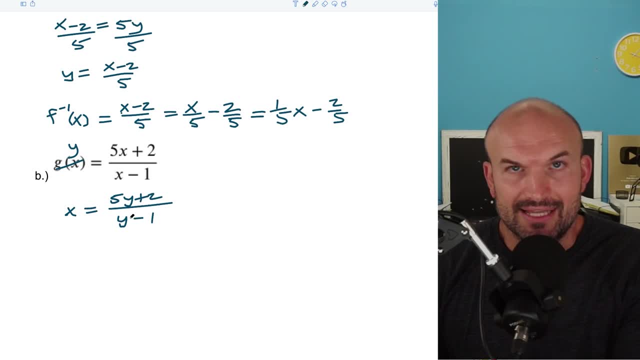 So if I have two y's- one's in the numerator, one's in the denominator- and I can't divide them out or anything, what I need to do is get this y off the denominator. So I'm going to do that is by multiplying it by y minus 1 on both sides. 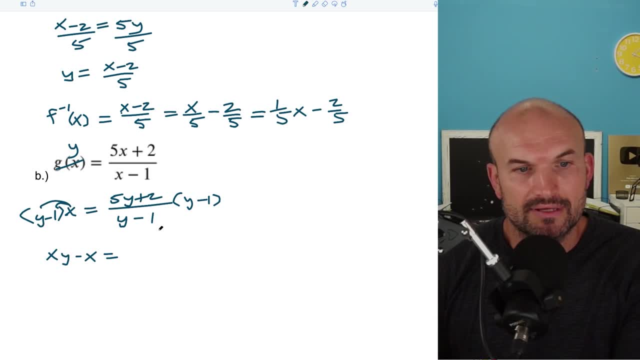 Then I'm going to go ahead and distribute here, So I'll have a xy minus an x and those are going to divide out. So that's now going to leave me with a 5y plus a 2.. Now again I need to solve for y, right? 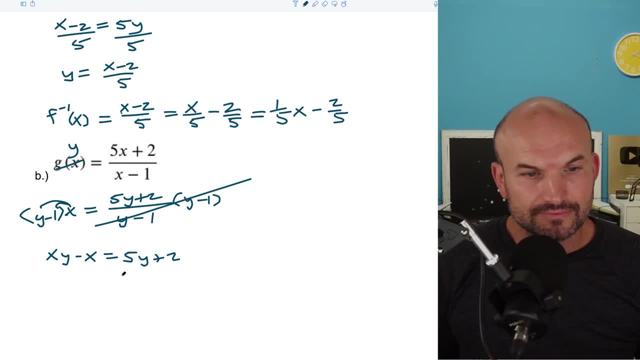 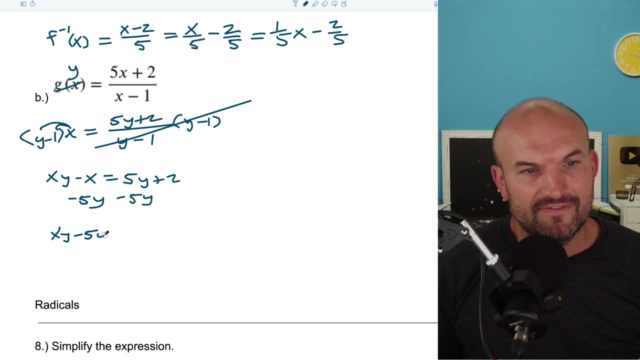 So I need to get all my y's over to the same side. So what I'm going to do is I'm going to subtract a 5y on both sides. That's going to give me a xy minus a 5y, And then I will minus. x equals 2.. 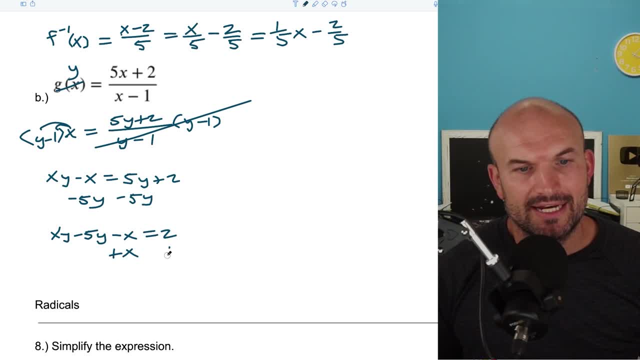 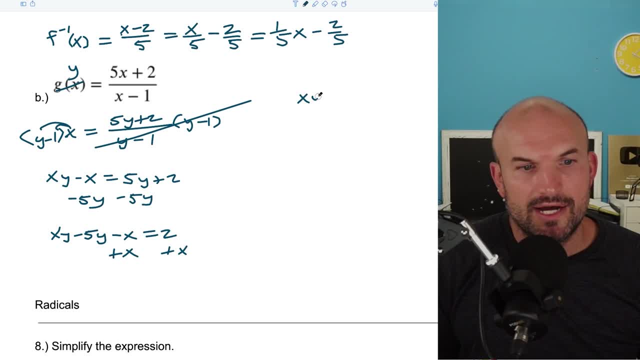 So now I have a- this is right over here- a xy minus a 5y equals a x plus 2.. OK, now again I need to solve for y, and I have two of them And I can't combine them right. 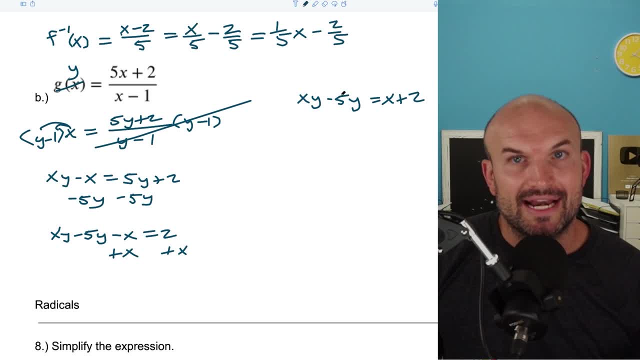 Those are not like terms, so you can't combine those two. You can't divide out the y. That's not going to work. So what you're actually going to do is factor out the y. See how these both share a y. 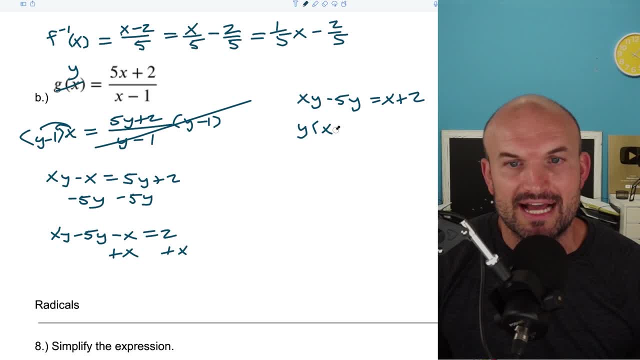 You can actually factor that out. So when you factor out that y, you're going to be left with an x minus a 5.. Now you can solve for y by dividing by an x minus 5.. And now you get the equation of y equals a x plus 2 all over a x minus 5.. 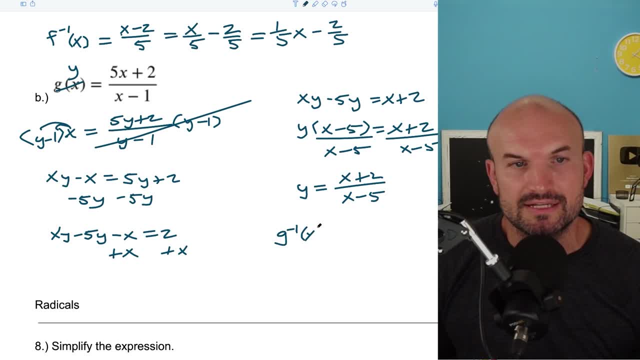 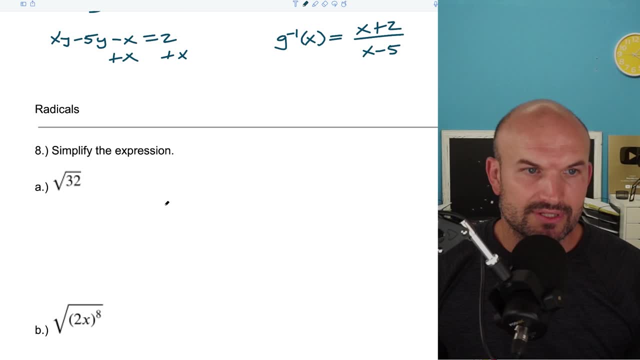 And then you can rewrite it in inverse notation. So g inverse of x is equal to a x plus 2 all over a x minus a 5.. All right, now let's go and talk about radicals. So again, radicals is pretty important in precalculus. 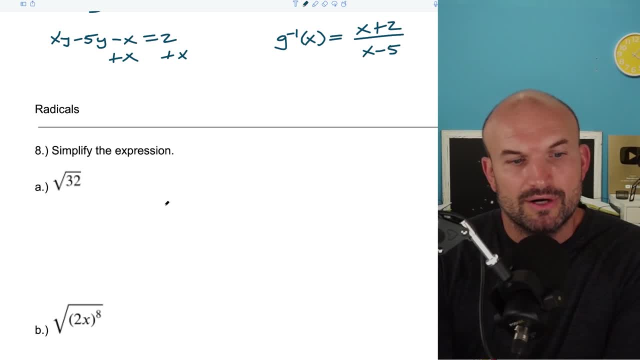 They do show up quite a bit. So it's really important to make sure we know how to simplify them and kind of apply some operations with them. So first of all, let's just kind of practice on simplifying the expression. There's many, many different ways we can simplify an expression or a radical expression. 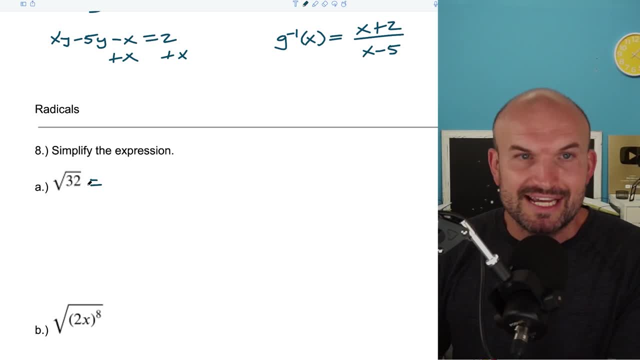 I think the most important thing is to recognize, rather than using prime factorization or some of the stuff we do in algebra 2 is really to kind of rewrite this And we're looking for what number multiplied by itself is going to evenly divide into 32.. 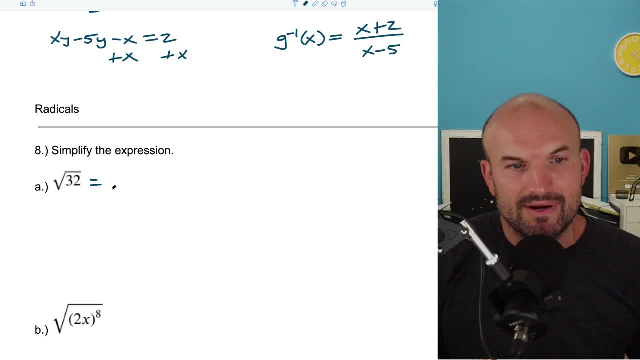 Basically, what we want to do is take 32 and divide it into 32.. So what I recognize here is I can rewrite this as a 16 times 2, right? So you want to find square numbers that evenly divide into what we call our radicand. 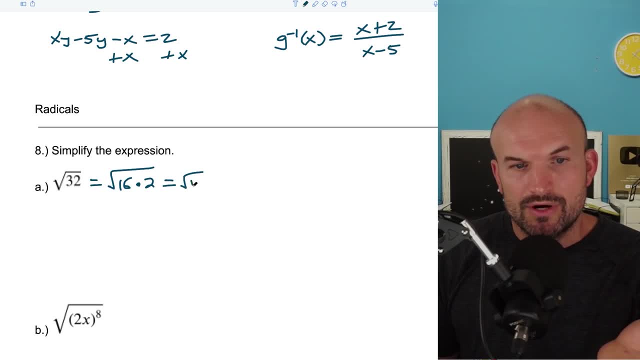 The reason why that's important is because, again, we can break this up into a square root of 16 times a square root of 2, right, That was the rules of logarithms, or rules of radicals. allow us to break up a radicand. 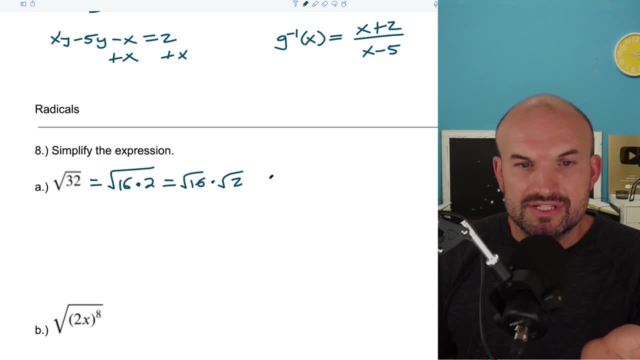 like that. So now I can take the square root of 16, right, The square root of 16 is just going to be a 4.. I can't take the square root of 2, so I'll just leave that as a 4 times the square root. 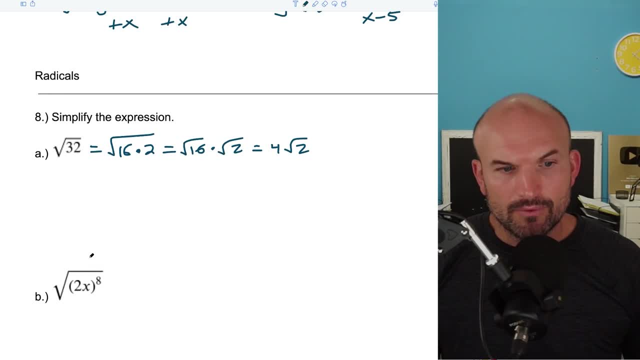 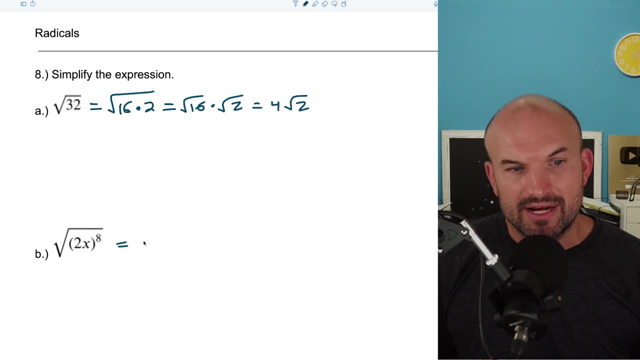 of 2.. Now, in this case, a couple different ways. we can also do that. Remember, we can always rewrite radicals as rational powers. So in this case, what I would simply do is I would go ahead and rewrite a square root. 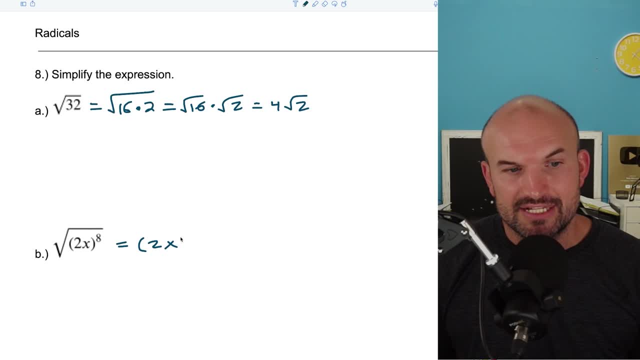 as raised to the 1 half power. So, therefore, I can rewrite this as a 2x raised to the power, And then I can rewrite that as raised to the 1 half power. Now, what my rules of radicals, or rules of rational powers, just tell me to do is whenever. 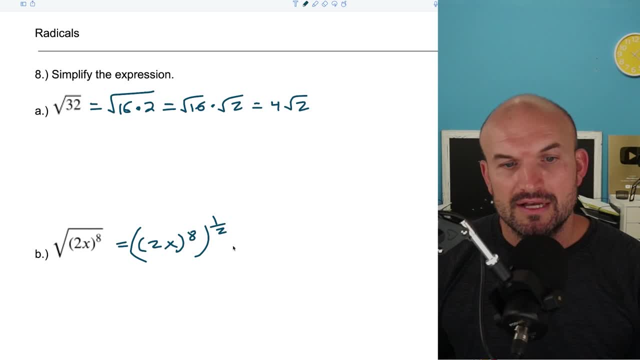 I have an exponent raised to another power. I can just multiply those powers. So therefore this is the same thing as a 2x 8 times 1. half is going to be to the fourth power. Now it's really important, though. you can't distribute your power across addition. 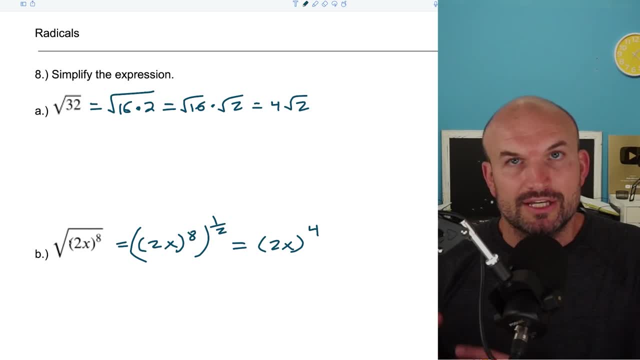 If you remember that polynomial, remember we had the 2x minus 1,, I believe, squared. You can't distribute that power across addition or subtraction, but you can go ahead and distribute a power across multiplication, Because basically the way that this reads is a 2x times a, 2x times a 2x times a 2x. 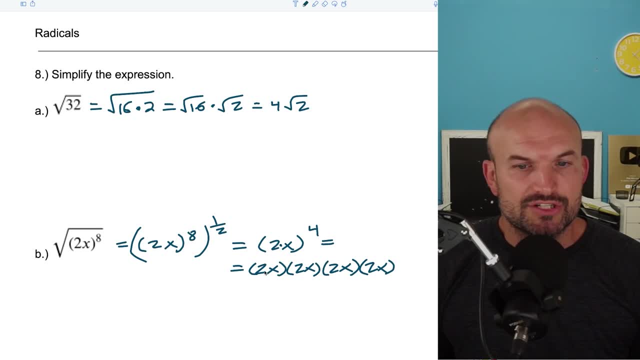 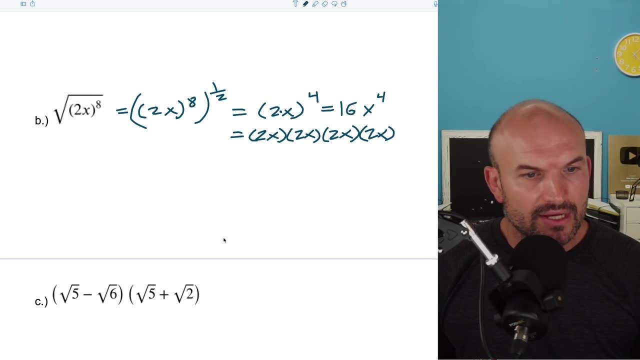 okay, Okay. So when I take 2, you know what is 2 times 2 times 2 times 2?? Well, that's going to equal a 16x to the fourth power. The next thing is like: what about when you multiply binomials? 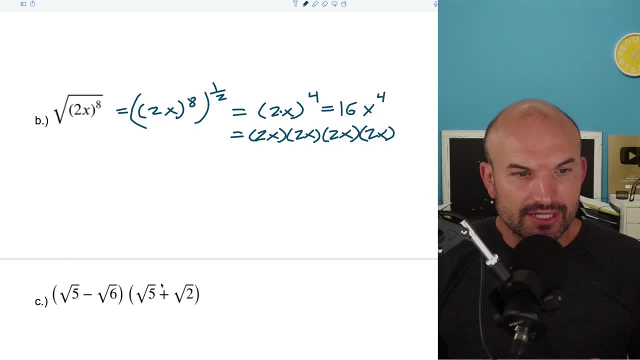 And remember, multiply binomials. you could use like the FOIL acronym, or you can supply distributed property, Like everything needs to be multiplied by everything. And again, when you're multiplying radicals, as long as they have the same index, like 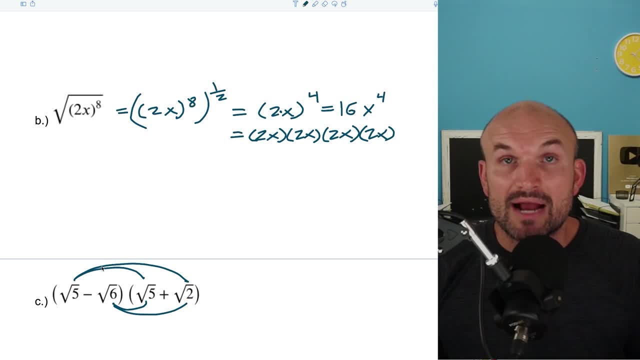 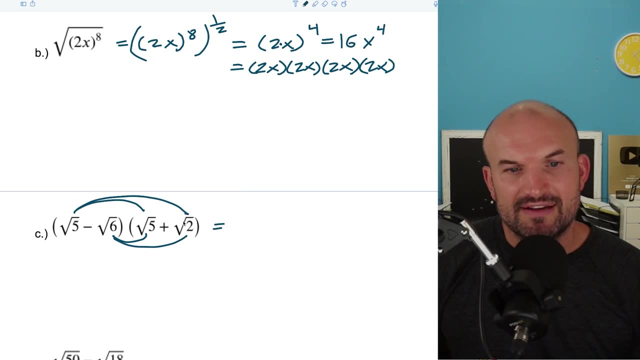 square root, or cube root, or fourth root. you can go ahead and multiply the radicands, which is the numbers or the expressions under the radicals. Okay, So let's just go on and work this step-by-step here. So square root of 5 times square root of 5 is going to be the square root of 25.. 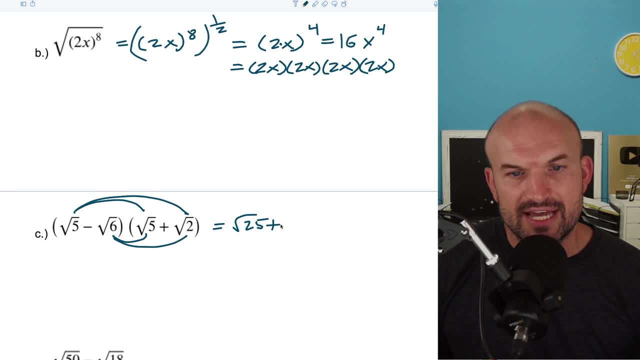 Square root of 5 times the square root of 2 is going to be a square root of 10.. Okay, We have the negative square root of 6 times a square root of 5.. So that's going to be a negative square root of 30.. 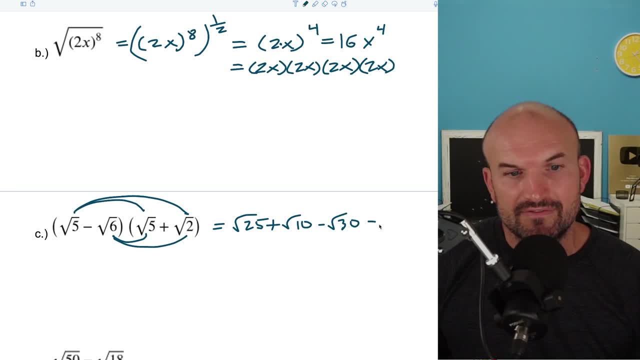 And a negative square root of 6 times a square root of 2.. That's going to be a negative square root of 12.. Now, obviously you could simplify square to 25, like from the onset. but now let's just kind of work left or right. 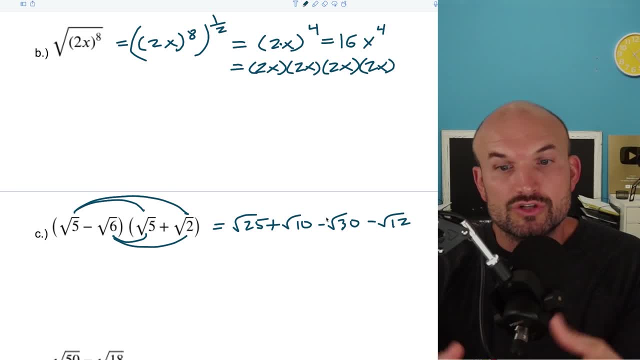 Okay, And again from that original problem, I want to look for square numbers that evenly divide into our radicands, So I don't need to do that. 25 is already a square number, right? So that's just equal five plus the square root of 10.. I can't do anything with that, So I'll just leave. 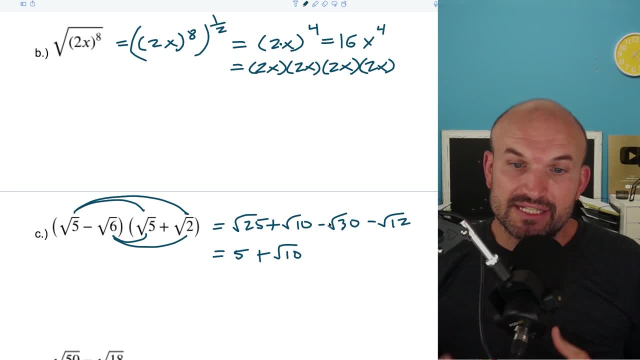 that. there Now the square root of 30, like what square numbers would possibly divide into 30?? Well, I have four which doesn't go into there. Nine, nope, 16, nope. So there's really nothing. 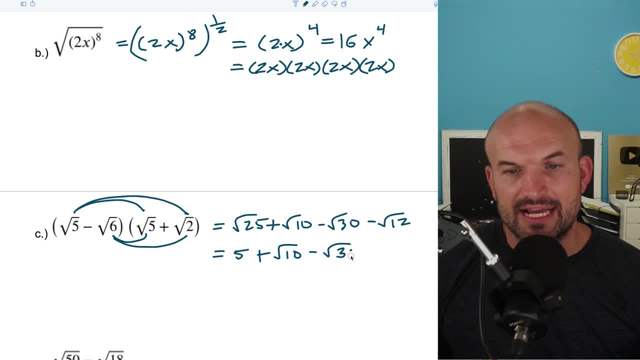 I can do to simplify this, So I'm just going to leave that as a negative square root of 30.. However, when you look at the square root of 12, you can say that four does evenly divide into that right. So I can rewrite that as a square root of four times a three, And then the square. 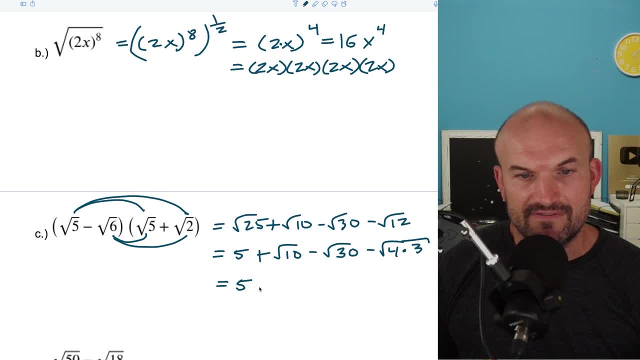 root of four, here is going to be a two, So I can finally write this out as a five plus a square root of 10, minus a square root of 30, minus a two square root of three. And again, I cannot combine them, Like when you're multiplying radicals. when the index is the same, you can multiply your. 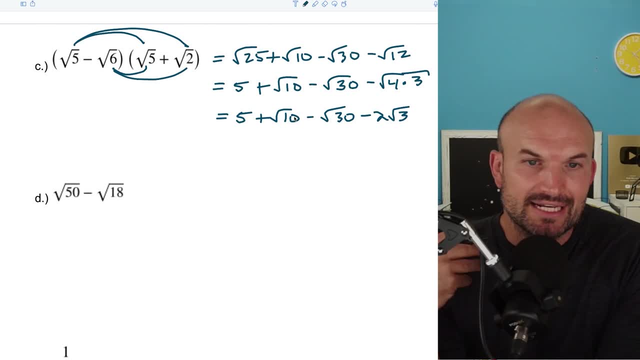 radicands. It's okay if they're not exactly the same, So I'm just going to leave that there. But when you're adding or subtracting, they have to have the exact same index as well as the exact same radicand for you to be able to combine. So in this case we have subtraction right, You see. 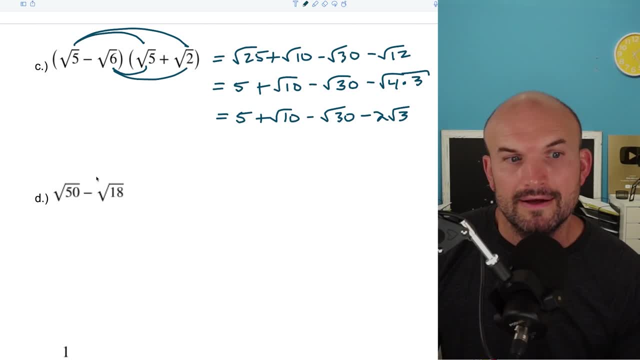 that, hey, you can't subtract these. right, They both are square roots, That's good, But they have different radicands, So we're not going to be able to subtract them. However, one thing we can do is simplify them, And again we want to look for what square numbers evenly divide into these. 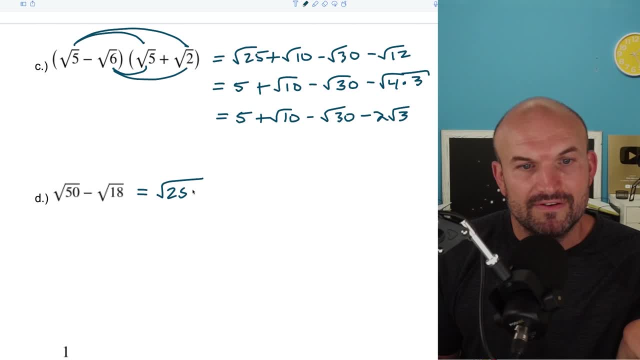 radicands. And when I do that here, what I have is a 25 times two. Okay, And that's going to be minus a nine times two. Well, what's cool? here I can take the square like I can break this up. right, That's a 25 times the square root of two, right? Just remember those. 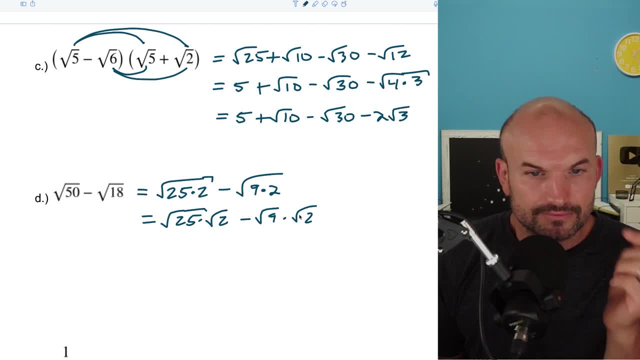 rules of radicals, That's going to be a square root of nine times a square root of two. Okay, So the square root of five is going to be a five square root of two, And the square root of nine is going to be a three square root of two. Okay, So now onto the next one. we have one divided by 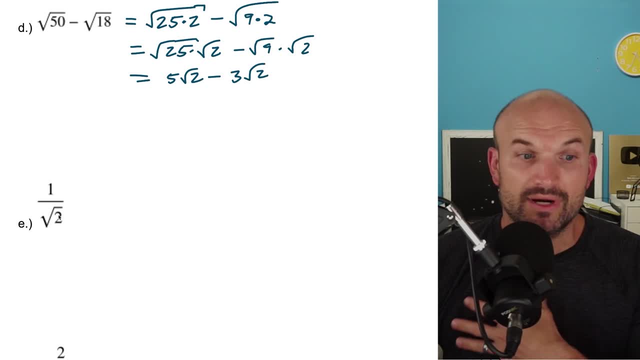 square root of two. So a lot of times in expression and breakout because we're going to want to have a radical in the denominator. So to do that, what we're going to do is rationalize the denominator, Because the reason why that's going to happen is square root of two times square root. 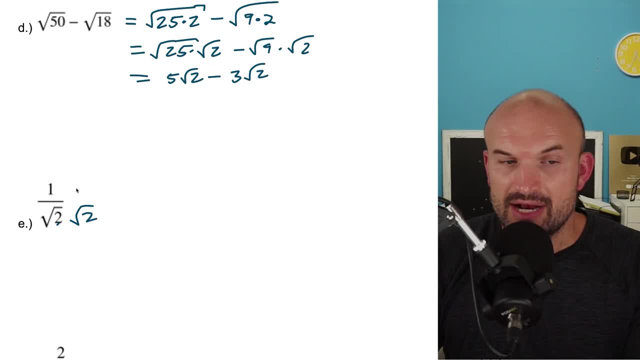 of two is square root of four, which is going to be two, So therefore we're not dividing by a rational number. It's really important, though, whenever you're rationalizing the denominator, make sure that you multiply by the square root of two, in the numerator as well as in the denominator. 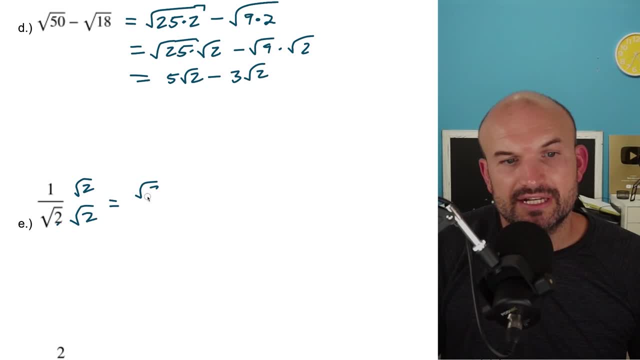 because that's going to produce what we call an equivalent fraction. So, therefore, this is going to give us the square root of two over again two. So just make sure that we can go ahead and simplify, just make sure you multiply that square root of two in the top and the bottom. Now one of the 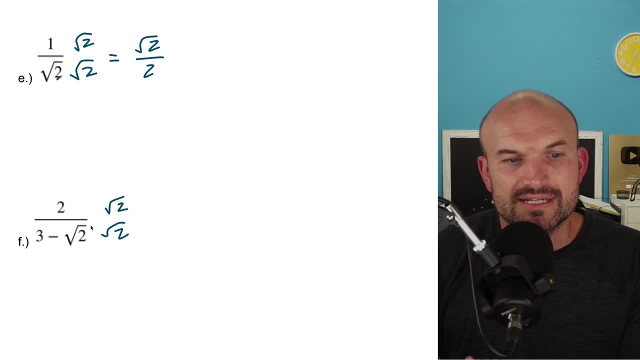 students will do? is they see a problem like this and say, oh, we just do the same thing again? Well, no, because again, by distributive property, you have to multiply the square root of two into the three and the negative square and the negative square root of two. So, even though you 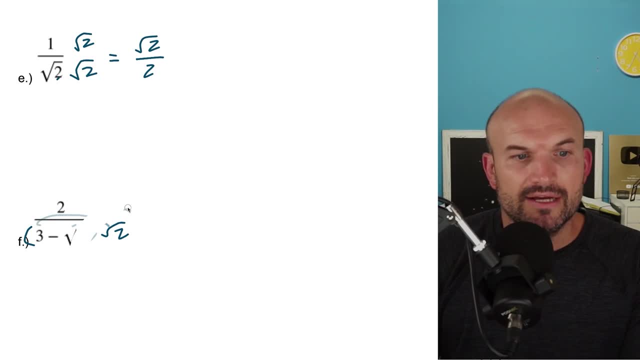 get rid of the radical here. you're not going to get rid of it when you're multiplying it by three. So what we need to do in this case is actually multiply by the conjugate. So three minus the square root of two has a conjugate of three plus the square root of two, And what we're going to 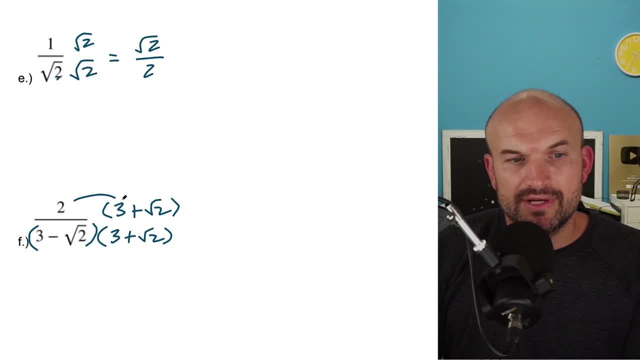 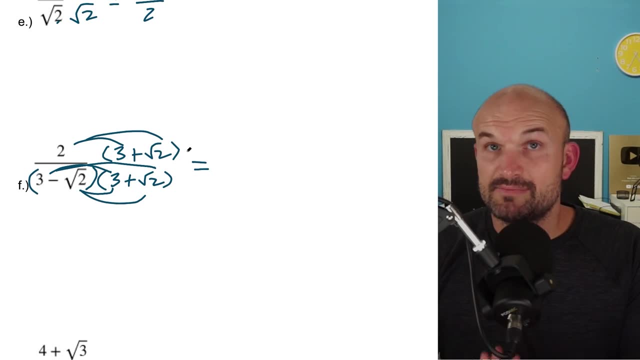 do is, again, we're going to multiply that on the top as well as on the bottom. So here I'm going to go ahead and apply FOIL right. So we're going to multiply everything, times everything. So let's go ahead and then like, expand this out and see what it's going to be. So two times three. 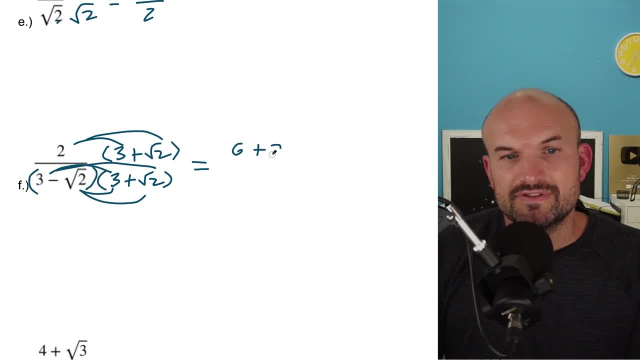 is going to be six. Two times a square root of two is going to be a positive two square root of two, And that's going to be all over here. Now, here I'm going to have a three times three, which is going to be a nine. Now it's really important to watch out. Notice my inner and my outer terms. 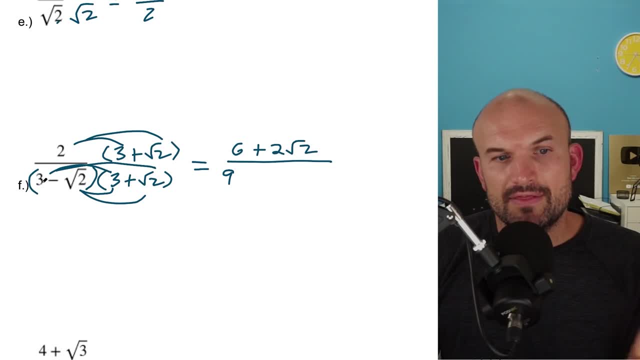 Three times a negative square root of two is a three negative square root of two, And then three times a positive square root of two is going to be a positive three square root of two. So basically, three square root of two plus a positive three square root of two. Well, what's going to happen? 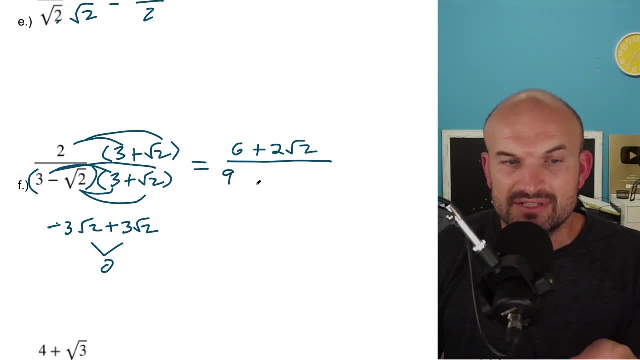 to those. That's just going to go to zero, right, So I'm not even going to waste my time spending that in there. What I will multiply, though, is a negative square root of two times a positive square root of two, which is going to be a negative square root of four, which is now going to be a. 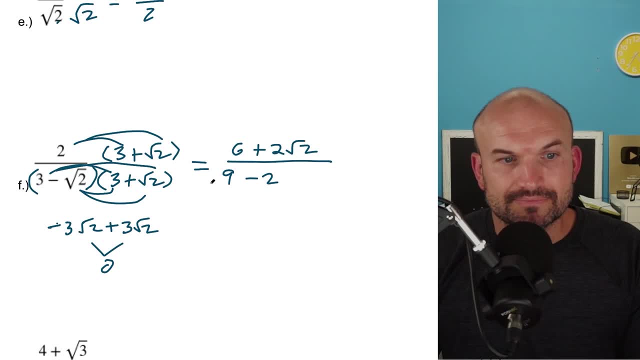 negative two. So that is something I can definitely go ahead and simplify in that case. And then I can't really do anything with the six plus the two square root of two, but so I can say six plus two square root of two, And then nine minus two is going to be a seven. 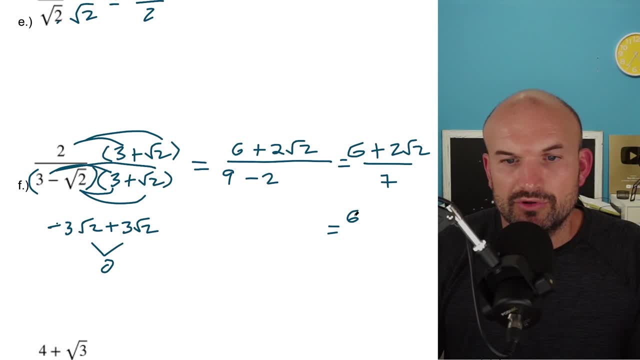 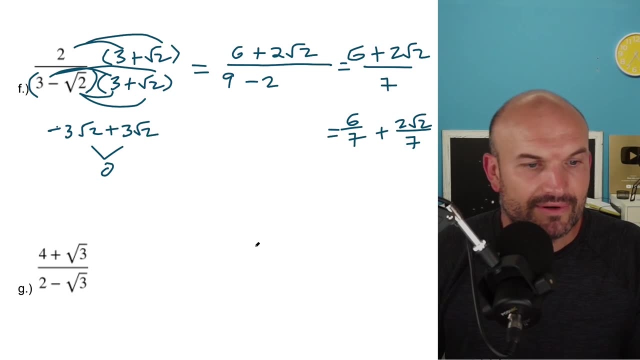 So I could leave it like that. or you could definitely distribute the seven into both of those, So you could say that's a six sevenths plus a two square root of two sevenths, And there you go. That could be like a simplified answer for you on that one. All right, In this example. 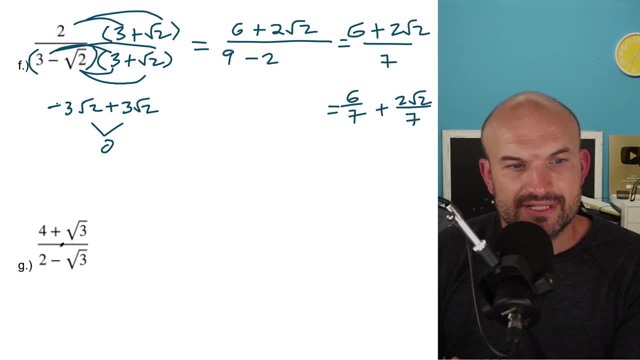 you can see, we basically have kind of the exact same thing going on. We just have. we just need to multiply by our conjugate. Now, the one difference here I would make is I'm going to put parentheses around this in the numerator as well as in- the- I'm sorry- denominator, as well as in. 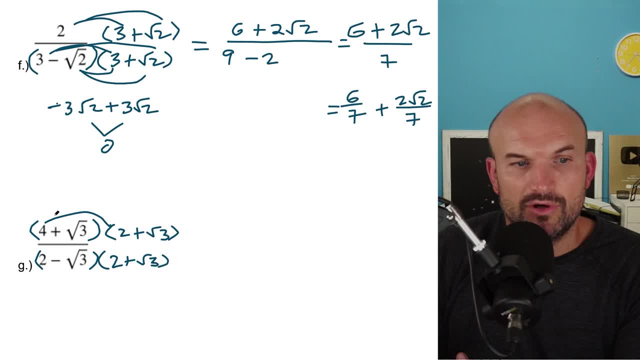 the numerator And just because you can see, it's just like kind of good practice here of multiplying or applying our distributive property here. Now again this is going to give us a difference of two squares, So hopefully we can kind of do. 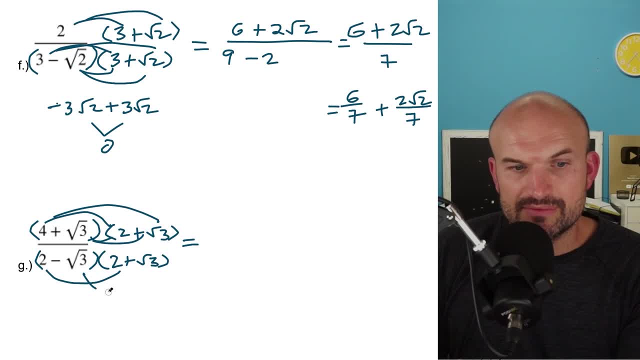 this rather quickly. We basically just need to multiply the first two terms and the last two terms, Cause again, the middle terms are going to add to zero right Whenever you have the same expression but one explain expression with the same terms, but one's positive and one's negative. 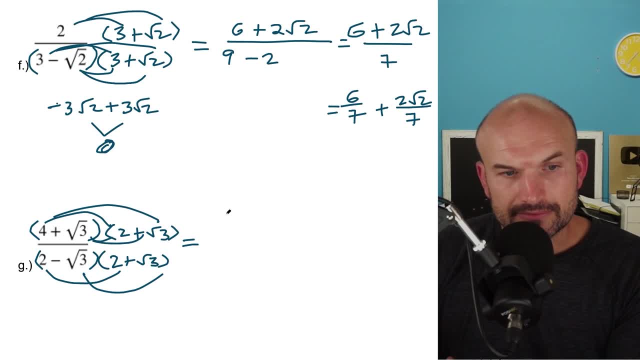 then you're going to have that difference of squares relationship up top here. I'm just going to have to multiply everything by everything. So four times two is going to be an eight. four times square root of three is going to be a four. square root of three two times square root of three is: 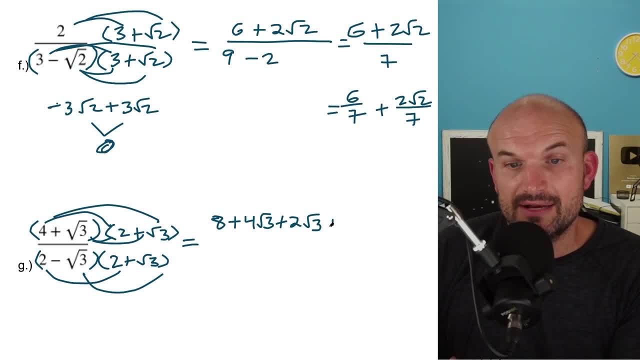 going to be a two, square root of three and square root of three times square root of three is a square root of nine, which is going to be a three in the denominator. here I'm going to have two times two, which is a four, and a negative. 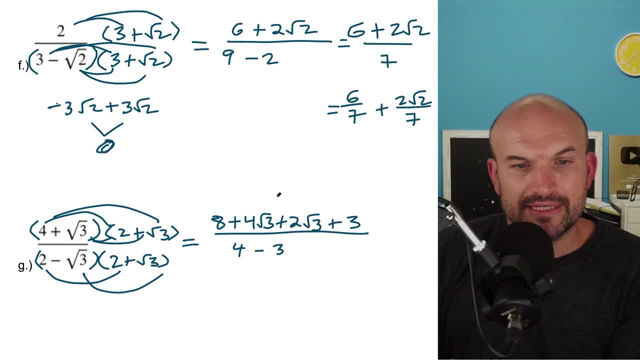 square root of three times a positive square root of three is going to be a negative three. All right, So now I can combine my like terms whenever you're adding radicals. right, We're going to keep the radical, but we're going to add the coefficients, So therefore, that's going to be. 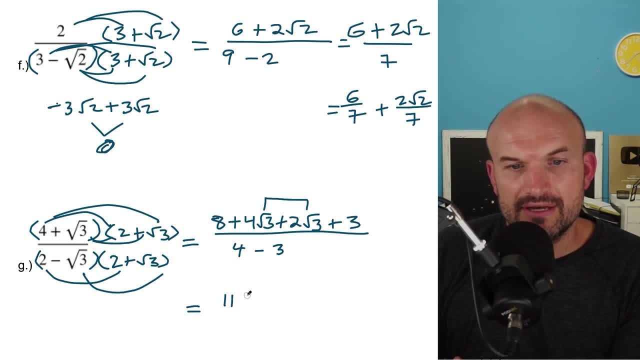 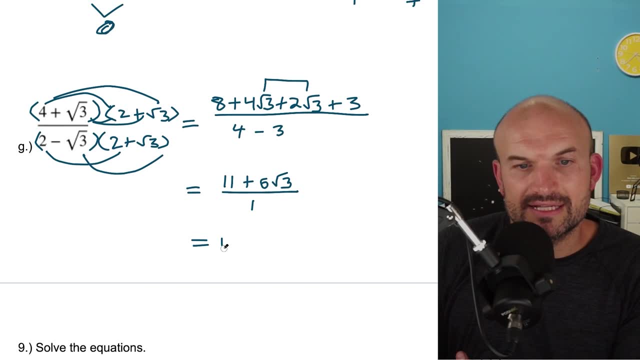 a six radical three, and eight plus three is going to be 11.. So it's 11 plus a six square root of three and all over one. So therefore I don't really need to read it all over one. You can simply just rewrite this as 11.. 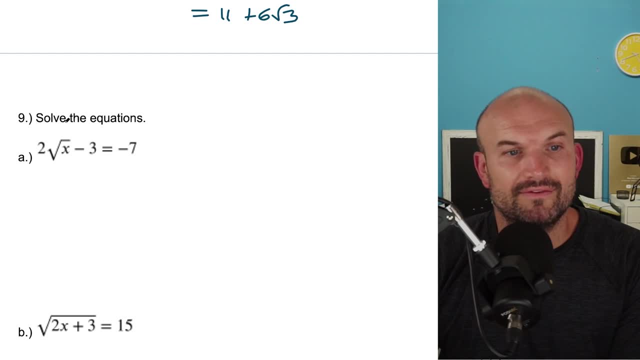 11 plus a six square root of three. Our next example we have. we're going to be solving some equations. So we have two radical square root of x minus three equals seven. So the main thing here we want to make sure we understand is the inverse operations. right, And if I said like x plus two, 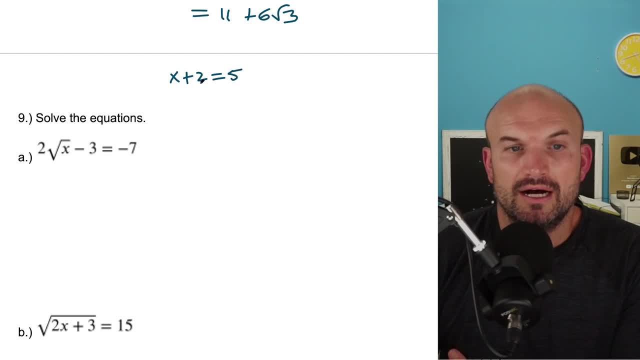 is equal to five, right, We need to apply the inverse operation here of what's happening to x, right? So x is being added by two. So the inverse operation of adding two is going to be subtracting two, right. So the inverse operation of a square root of x is going to be squaring the x. But 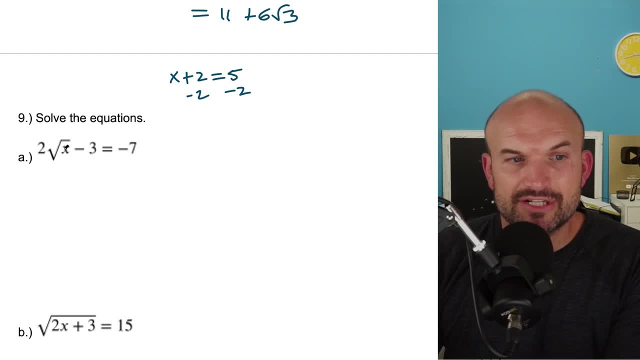 before we go and apply our inverse operations here, what we need to make sure we do before we square both sides, we need to make sure we can isolate this x here, So what I'm going to do here. and then also we want to make sure we check our. 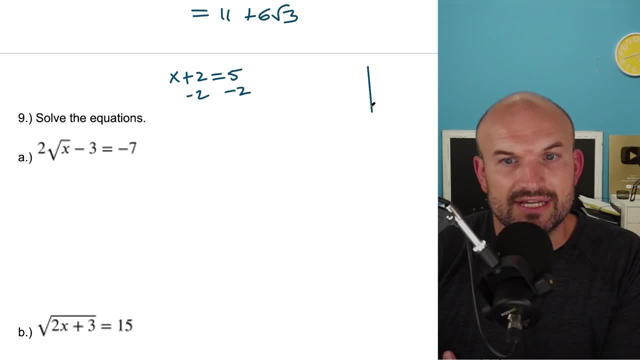 answer because the square root function. if you remember what that graph looks like, that doesn't always, that isn't always going to be checking our crossing right. You could have a graph like this that's actually not going to have the x intercept or any solution, So let's go ahead and 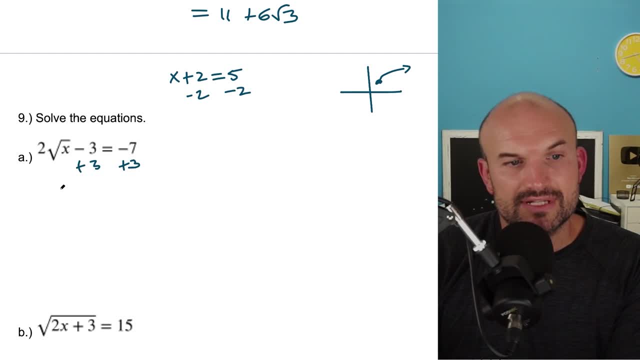 go ahead and apply our inverse operation. So the first thing I'll do is I'll add a three on both sides. So I have a two square root of x equals a negative three. So I'm going to do that. So I'm going to do a negative four, and then I will divide by two. right, And now we have something. 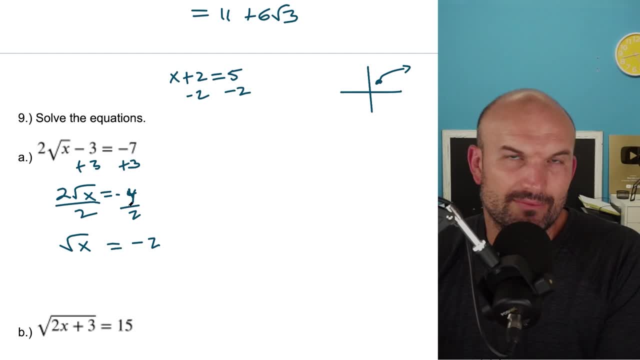 that's kind of interesting. The square root of x equals a negative two. Well, what can you like? what numbers? can you think about the real number system that you can take the square root of something and it's going to be a negative, right? That doesn't make any sense, right? Especially. 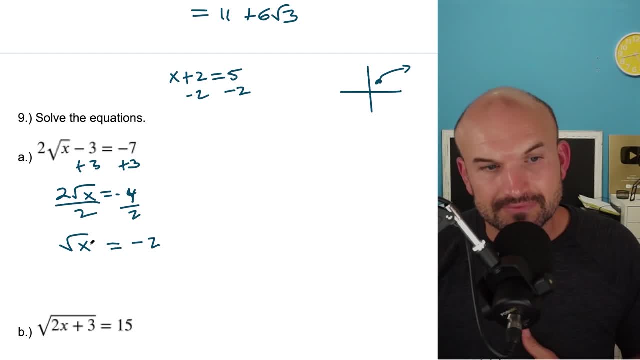 the even root. You can't take the even root of something and it's going to be a negative. So therefore, from this case we could say it's going to be no solution. Now again, you could also check this by saying: oh, I'm not sure if that is exactly the case, So let's just 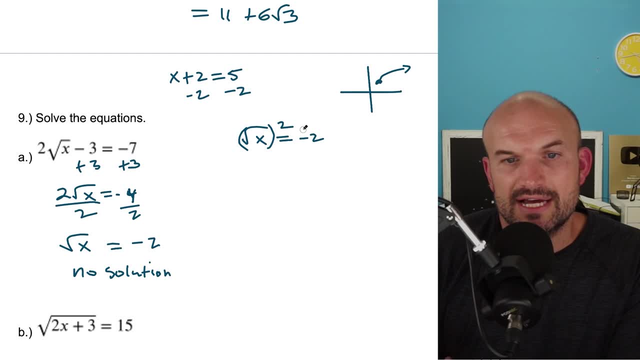 let's just go and check it out. What do you say? Well, what could I do? What if you squared both sides? Okay, then you'd have a x is going to equal a positive four. Well, go and take your answer and 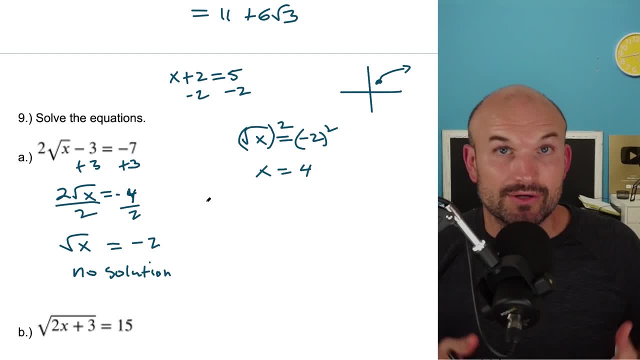 plug it back into the equation, right. So that's something we learn. Remember, like in algebra one, you should always make sure you go back and check your answer to make sure you don't have any like extraneous or no solutions. So when I do that, I get a two square root of four minus three equals. 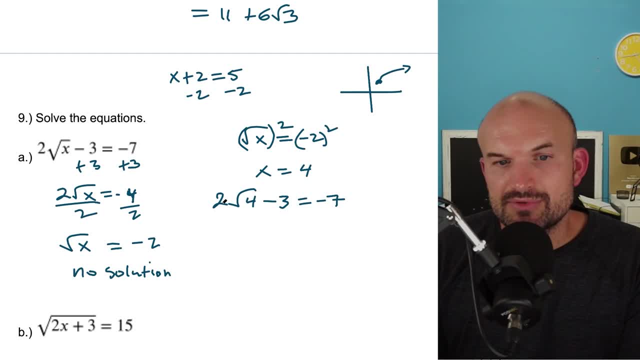 a negative seven. And again, when you calculate this, square root of four is two. two times two is four. four minus three is one. Well, one does not equal a negative seven. So make sure you, when you are applying your operations or you're simplifying, that you're also go ahead and checking. 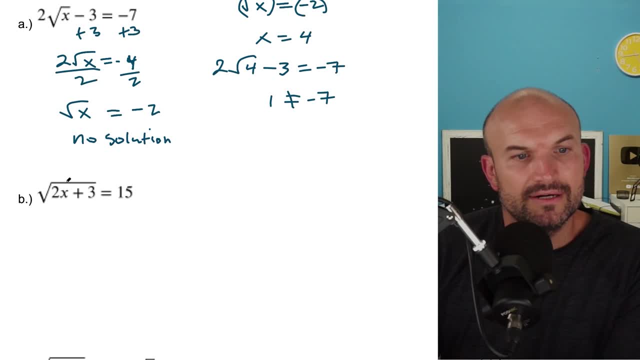 your work. Okay, in this example here, the first thing I'm gonna do is, again, you can see my radicals already been isolated, So I'm just going to go ahead and square both sides here. So I have a two x plus three is equal to a 225.. Now what I'm going to do is I'm going to subtract a three on. 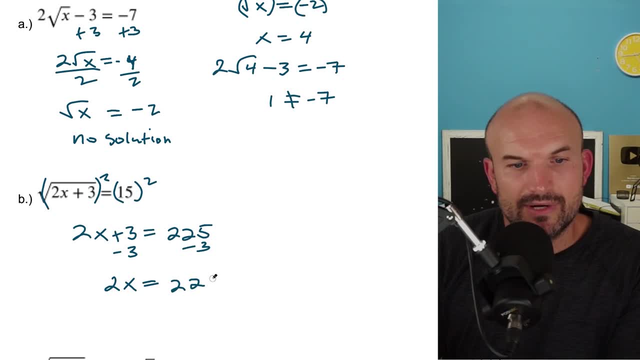 both sides. So I have a two: x is equal to a 222.. Now I can go ahead and divide by two and I get x equal to 111. And again we can just go ahead and check our answer here. But again this one kind of 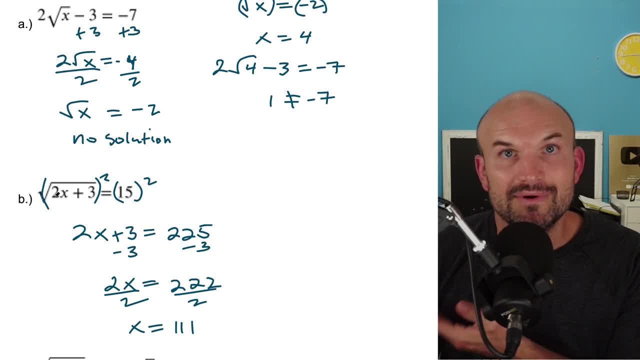 makes sense, Like when you plug in 111 multiplied by two, that's 222 plus three is 225.. The square root of 225 is going to be a you know positive 15.. So this one is going to go ahead and check. 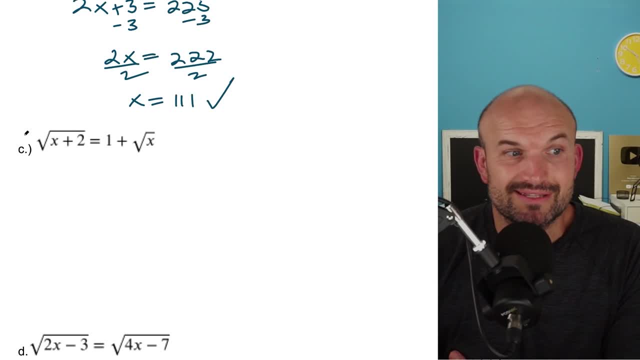 out. Okay. in this example, what we have is the square root on both sides. So what we need to do is obviously get rid of the square root. So to do that, what we're simply going to do is just square both sides. Now, remember, these are binomial squared right. So therefore, 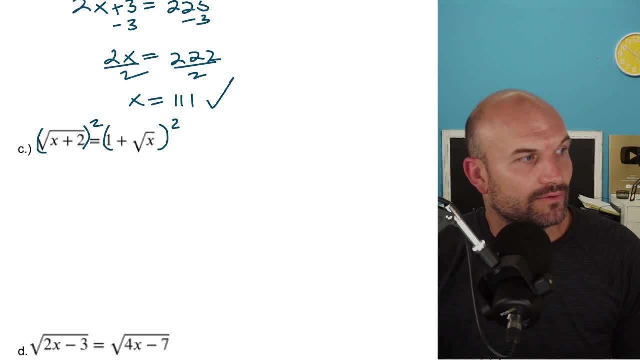 basically this binomial being multiplied by itself. So the main thing we're going to want to do in this case is, you know, multiply like square root of x plus two times square root of x plus two is just going to give us a x plus a two And one plus square root of x times a one plus square root. 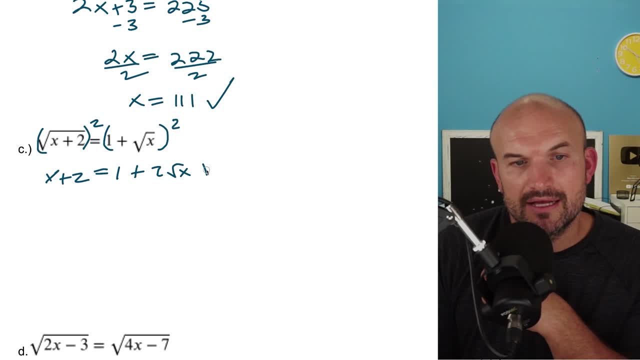 of x, that's going to give us a one plus a two square root of x plus x, right? Because basically that is a perfect square trinomial And you could definitely go ahead and expand it on the right hand side. Now what I'm going to do is just kind of get my x's here to the same side. So if I'm 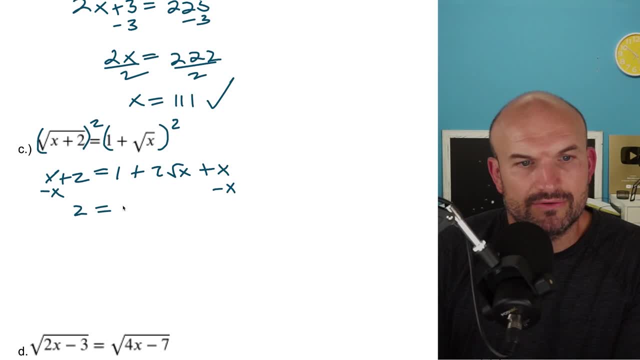 going to subtract an x on both sides here and therefore I get a: two equals a one plus a two square root of x. I can subtract a one, So I get a one equals a two square root of x. divide by two. divide by two and I get a one. half is equal to the square root of x And again. 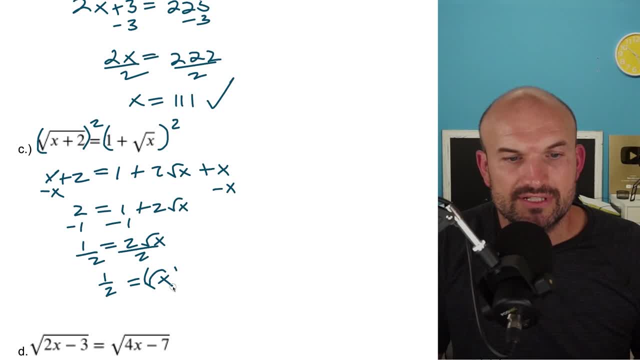 can you take the square root of what number is going to equal a one half? Well, let's go ahead and figure that out. So I'll go ahead and square it on both sides and I get: x is going to equal a one fourth, And therefore then what we can do is just go ahead and plug a one fourth. 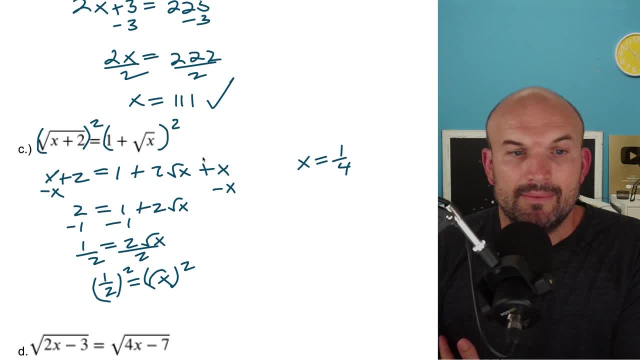 equation to go ahead and make sure to see if that would indeed go ahead and work. And again, you know, if you want to go ahead and check it out, let's just go ahead and check our work here. So I have a one fourth plus two is equal to a one plus the square root of a one fourth. Okay, So in 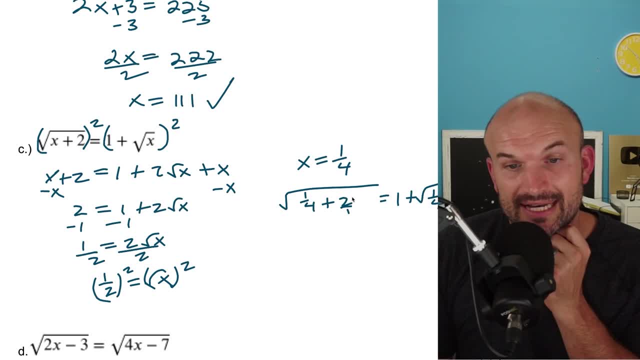 this case a one fourth plus two. I can basically rewrite that to an eight right, An eight over four. So therefore this is going to give me a nine over four, And then this is going to be the square root of one fourth is basically one half right, So that's going to be one. 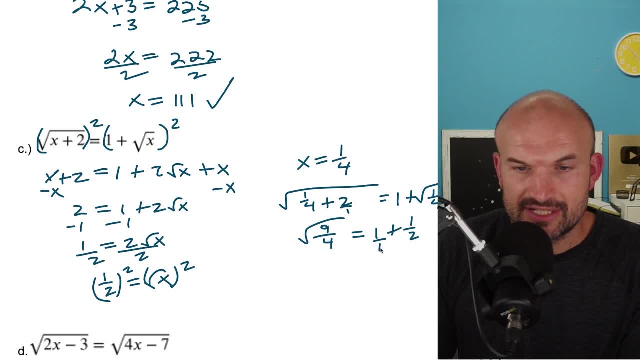 plus a one half. Now again, technically, you could write this as a two over two. So nine fourths is a three halves. And then if you did read this, if you rewrote this as a two over two, then this would be equal to a half. So you can see how that kind of works. 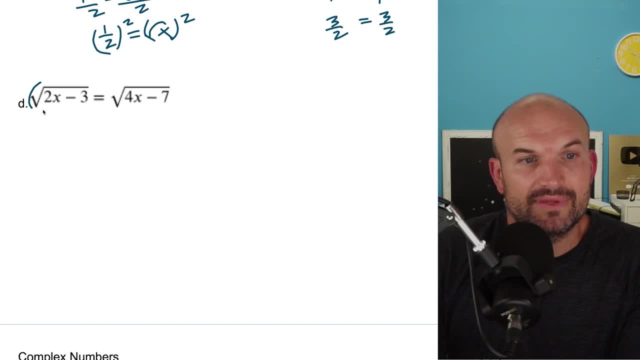 This is again another example. you're going to do the exact same thing here. So we're going to quantity square on both sides And when we do that, I get a much easier equation to work with. A two x minus three is equal to a four x minus seven. Now it's just basically solving my equation. 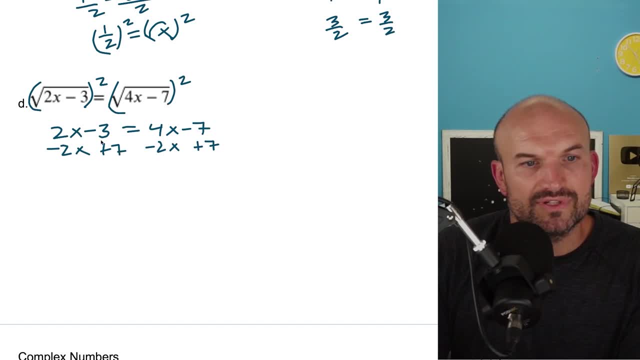 get my variables to the same side, I'll add a seven to both sides, And in this case I'm going to get four equals a two x, and then I can go ahead and divide by two And therefore x equals two. And again- now this one's a little bit easier to like mentally check. 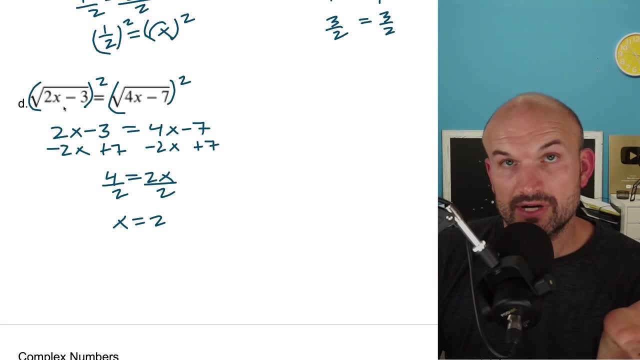 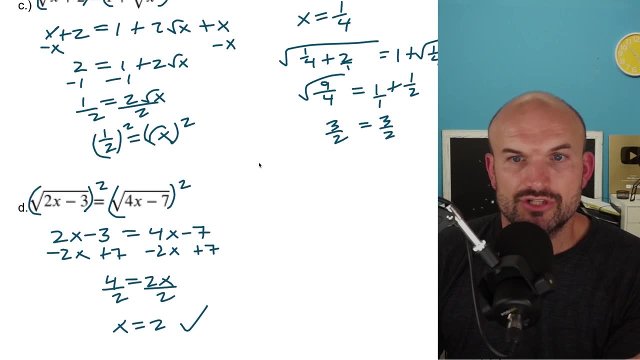 let's just plug it in: Two times two is four minus three is one, So square root of one is one. Two times four is eight. eight minus seven is one. square root of one is obviously one. So therefore this answer checks out just like that answer did. All right, now let's go and look into some. 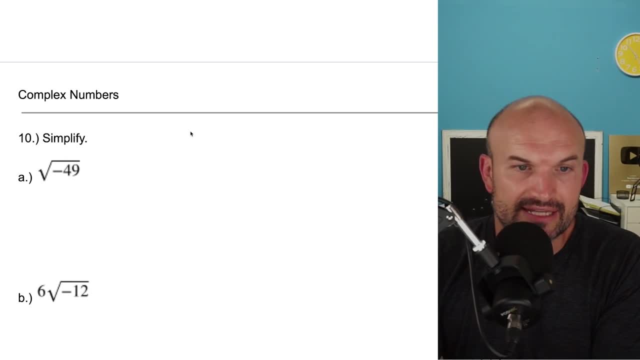 complex numbers. So complex numbers do come up in, definitely in pre-calculus because we're going to deal with them, where we're going to get into a little bit with our polynomials And then also once we learn, kind of our vectors and kind of stuff like that. So it's going to get to some fun things. 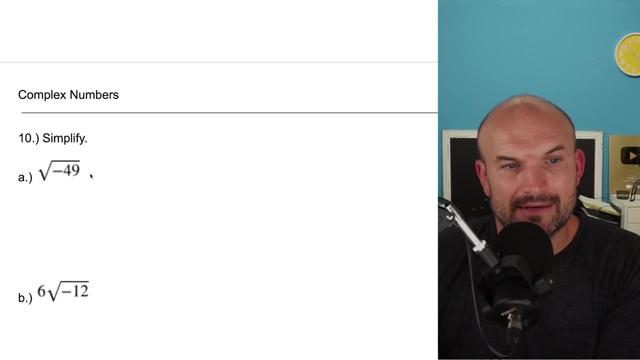 especially like the polar coordinates and everything like that. So all right. so the main thing we want to understand is the imaginary units. right, The square root of a- sorry, the square root of negative one- is going to equal a i. So what I always like to do in a problem like 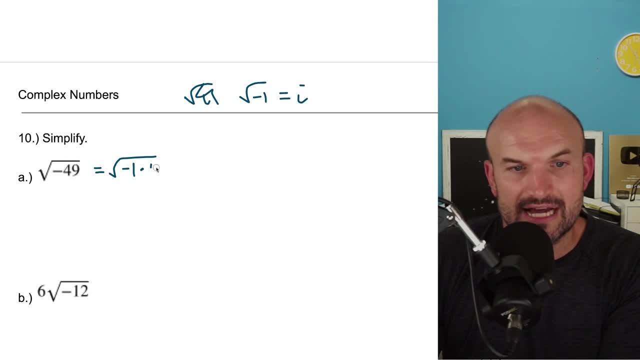 this is just remember. you can always rewrite the square root of a i, So what I always like to do in a problem is write this as a negative one times a 49, right, So now we could break that up and do the square root of negative one times the square root of a 49.. Well, the square root of negative one. 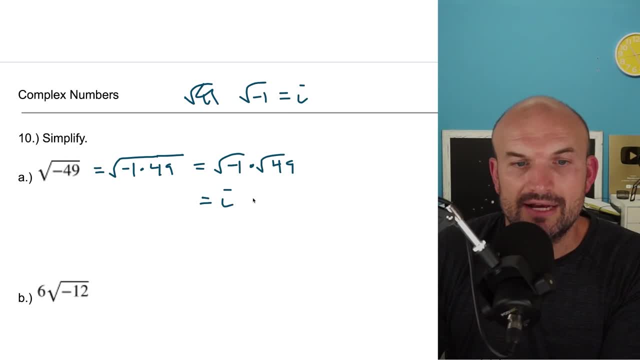 which, that is our imaginary unit, which is i and the square root of a 49, which is going to be a seven. Now, typically we write the i kind of like, even though it represents the square root of negative one, we still write it as like a variable. So we'd write this as a seven i. Now in this: 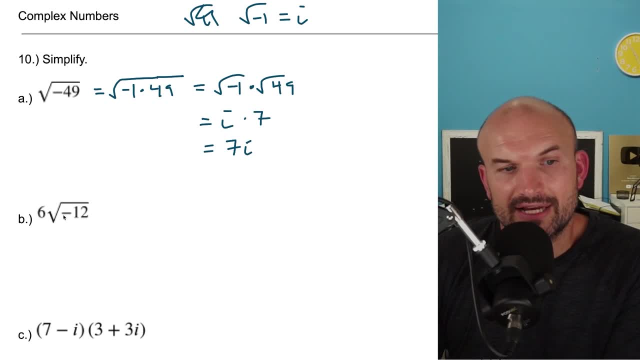 example. we're just going to simplify this just kind of like a radical right. So the first thing I can do is kind of like take out the negative right, Just taking the square root of a negative, and just kind of rewrite this as a six. i times the. 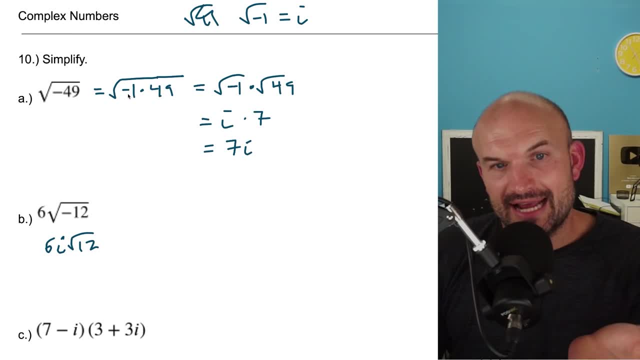 square root of 12, right To kind of see what I did. rather than just, you know, writing a negative and then saying that's i. you can just kind of like take that out, Now I can go ahead and rewrite. 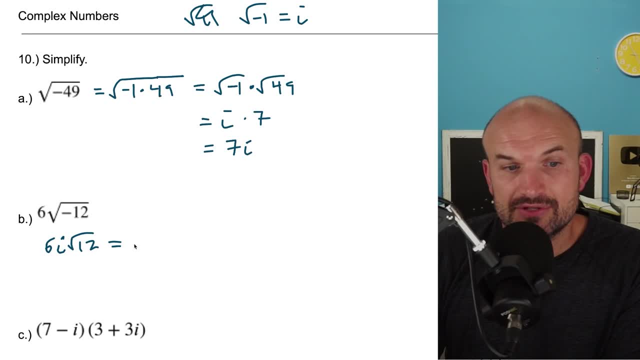 the square root of 12 as a four times three. So six i times the square root of four times three. Now I can take the square root of four, which is going to be two. I can't take the square root of three, so that's going to remain in there. And then two times six is going to be a 12 i times. 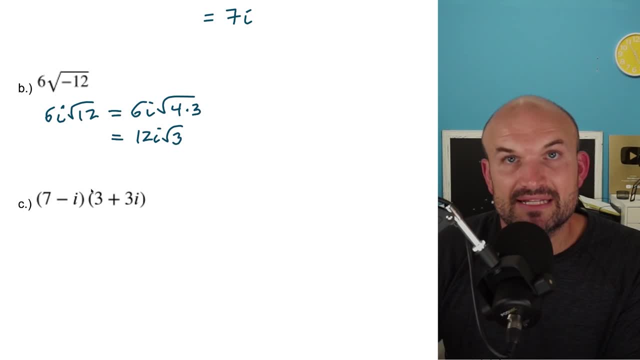 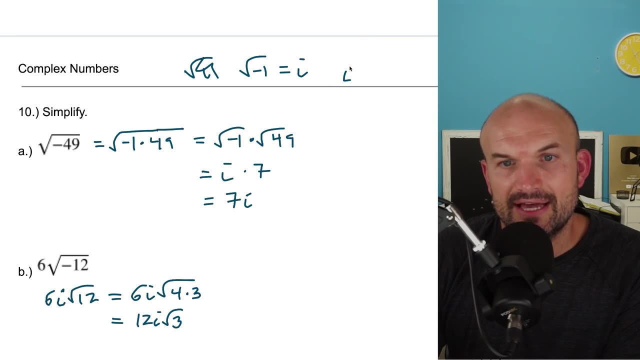 the square root of three. Now, in this example, we basically have two binomials multiplied by each other. So the only important thing to recognize here is, if we have the square root of negative one is i, then if we were to square both, 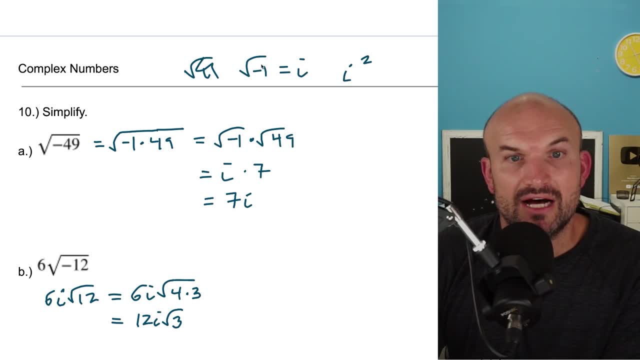 sides, we'd have an i squared. Well, i squared. then. what's the square root of a? what's the square root of square? sorry, what is? yeah, what is the square root of negative one? squared is what? Just equal to negative one? So it's important to recognize this relationship. 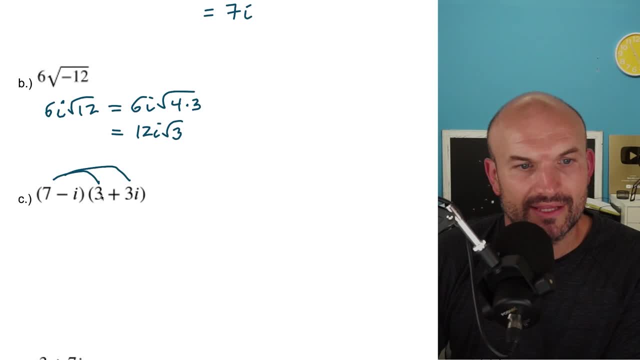 i squared is equal to negative one, Because when I go ahead and multiply this, when I go and apply my distributive property, what I'm going to get is a seven times three, which is a 21,. a seven times three i, which is a 21. i a three times negative one. 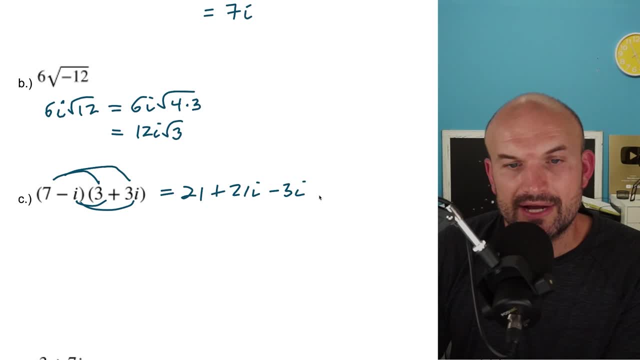 which is a negative three i and a negative i. times a positive three i is going to be a negative three i squared right. So now we have here is i squared is a negative one. So let's go and combine our like terms. So 21,. you can think of the i as kind of like a variable as well. like you know, x. 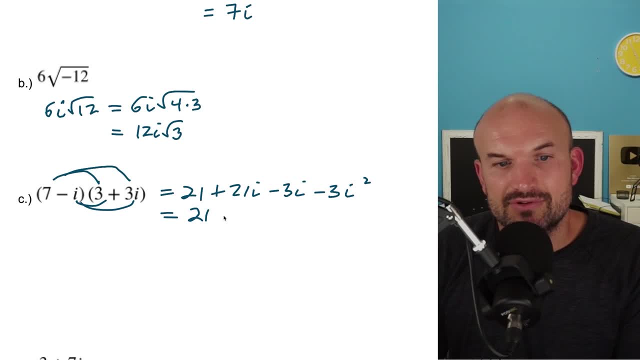 x plus x is two x, So 21 i minus a three. i is going to be a positive 18 i, i squared is negative one, So negative three. i is going to be a negative three, i squared. So let's go ahead and combine our. 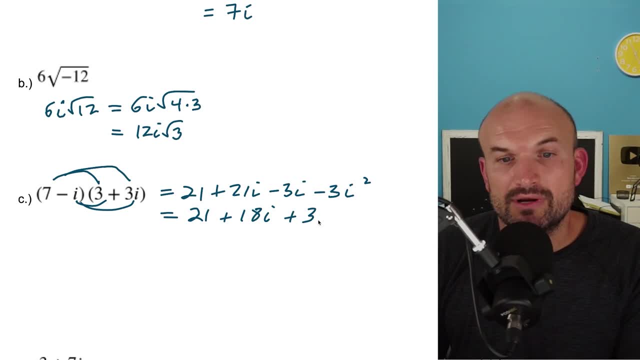 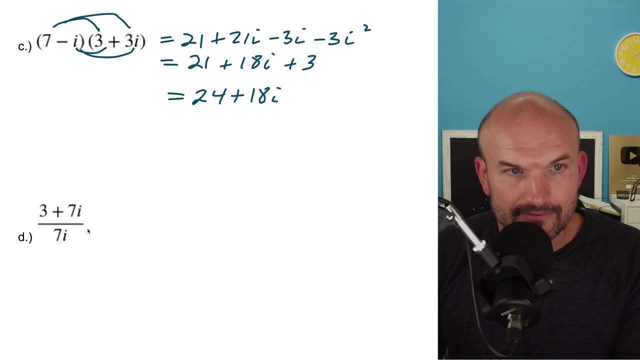 three times negative, one is going to be a positive three, And now I can combine the 21 plus a three, So that's going to equal a 24 plus an 18 i, And therefore we're all set. And then, just like we, 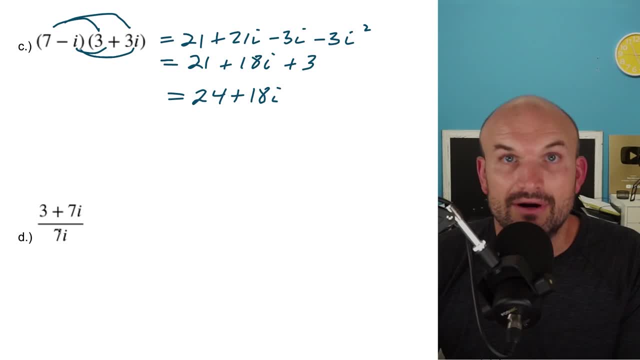 rationalize the denominator with our radicals. we can rationalize the denominator with our i. Basically, we don't want to divide by a irrational number. We don't want to divide. Also, we don't want to divide by an imaginary number. So what I can do here is just multiply by i on the top and 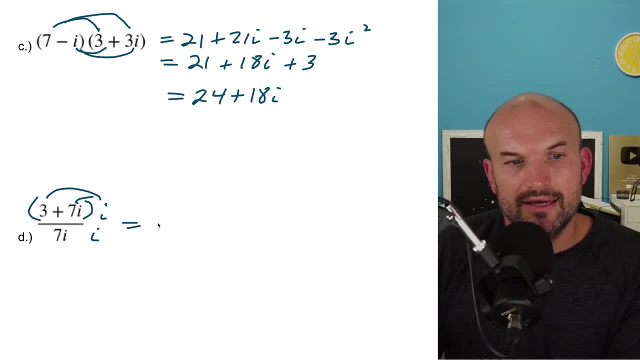 bottom. Make sure, though, you put this around parentheses, because we're going to have to distribute that, And when I do this, I'm going to get a three. i plus a seven. i squared is all over a seven, i squared. Okay. Now remember, i squared is negative one, So negative one times seven is going. 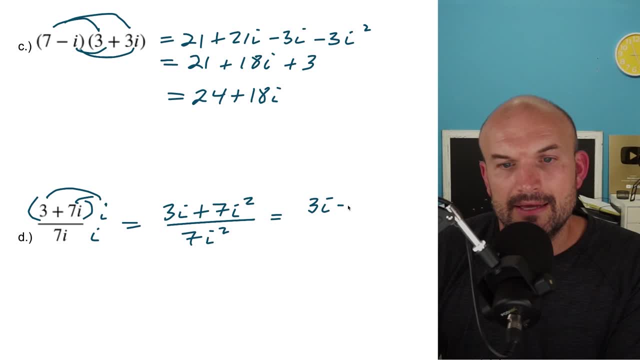 to be a negative seven. So therefore this is going to turn into a three i minus seven divided by a minus seven. Now again, do not distribute or do not cancel out those negative sevens. You have to divide this negative seven into both of these terms. So when you do that you get a negative. 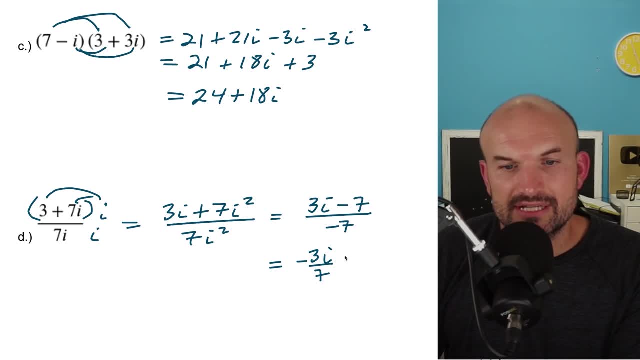 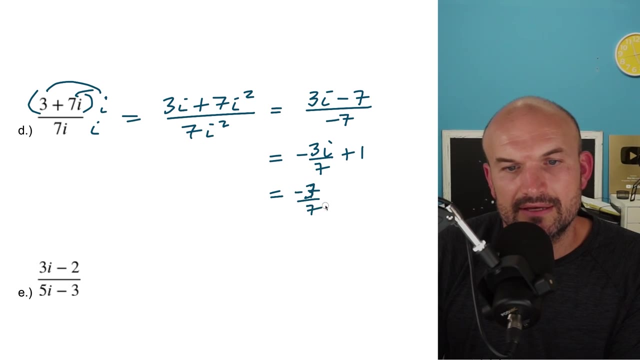 three, i, sevens, And then therefore, this is going to be a plus one. Now, typically we can go ahead and we can just go and write it like this. you know many different ways. We can definitely write this like a negative, sorry, negative, three sevens, i. That just kind of. 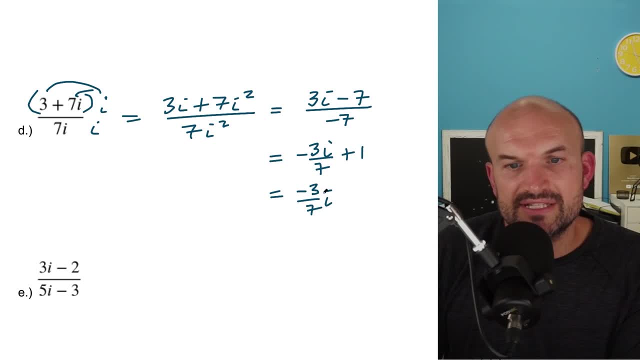 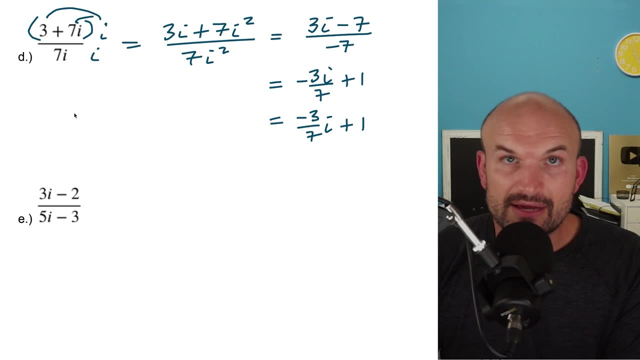 looks bad, So let's go and fix that. So it'd be a negative three sevens, i plus one and same same thing like that. In this case we have kind of the exact same thing that we did before Again. you notice, here we have a binomial, So therefore we need to now. 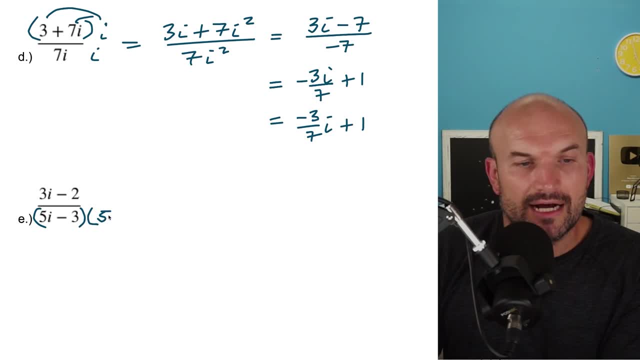 multiply by the i. So we're going to do that. So we're going to do that, So we're going to do that. So what I'm going to do here is I'm going to do now. big mistake that students will make is they'll. 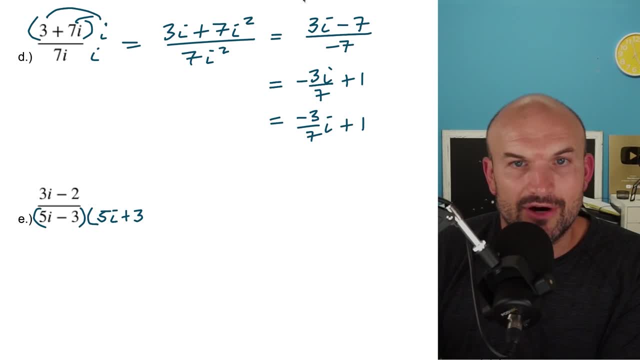 say: this is the conjugate. That's not the conjugate actually. So this is actually kind of confusing. You want the i or whatever you're trying to do, to be your conjugate, So what we're actually going to need to do in this case. you can leave it like this, but I always like to just like. 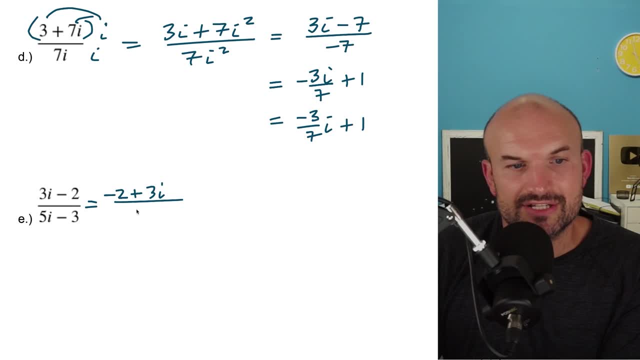 rewrite this. So negative two plus a three i. So I'm just going to rearrange this, So my i is going to be after right. So therefore I can say this is negative three. Oh, a plus bi. There we go, Sorry. 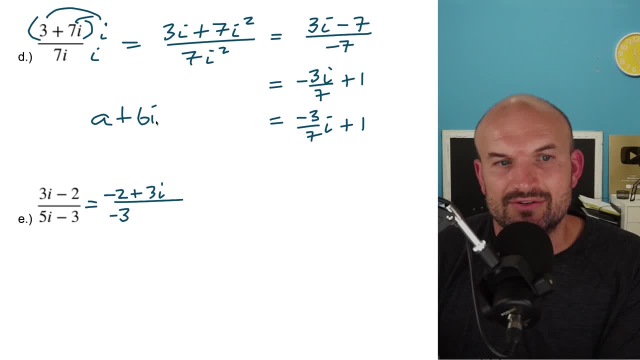 about that. I was kind of remembering um, a plus, bi. So typically we always like to write the the constant in front of our variable with that. So therefore I actually have to rewrite this as a one minus a three sevens. i. Okay, And that's exactly what you're going to want to do here as 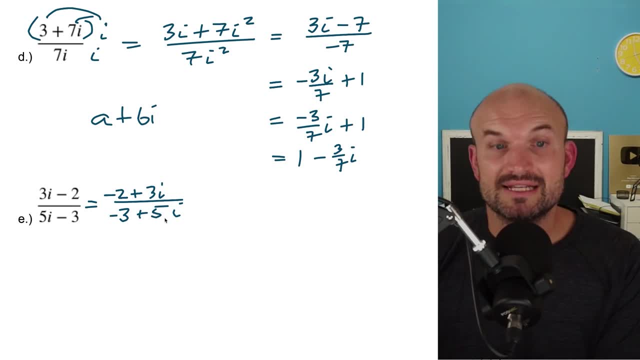 well, Um, you can do a negative three plus a five i. Okay, Now we can multiply by the conjugate here, And so what happens here is, when I multiply by the conjugate, what I'm going to get is a negative three, Um, and therefore that's going to be a minus a five i, And we're going to do that on. 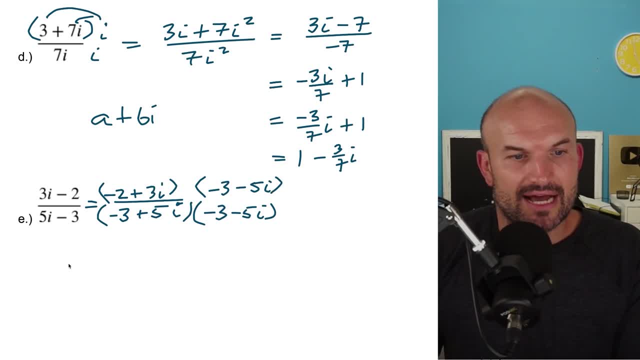 the top as well as on the bottom. Okay, Um, so now let's go and see what's going to happen up top. here. We're going to have a six. um, let's see, plus a 10. i- negative three times three. i is going to be a negative nine i and three. i times negative 15. i is going to be a. 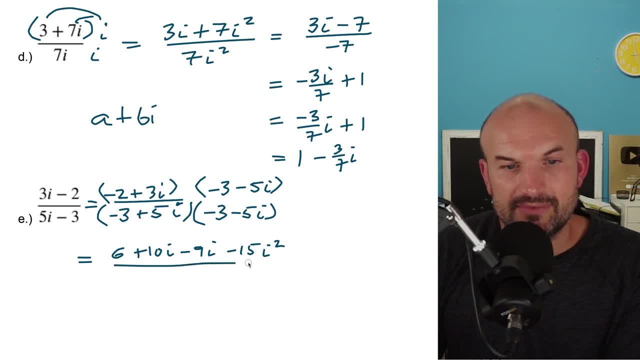 negative 15 and that's going to be an i squared Okay. Now. this is going to be all over Now. remember this is a difference of two squares right Negative- three times negative three is a positive nine five. i times negative five. It's going to be a negative 25. i squared Okay. So. 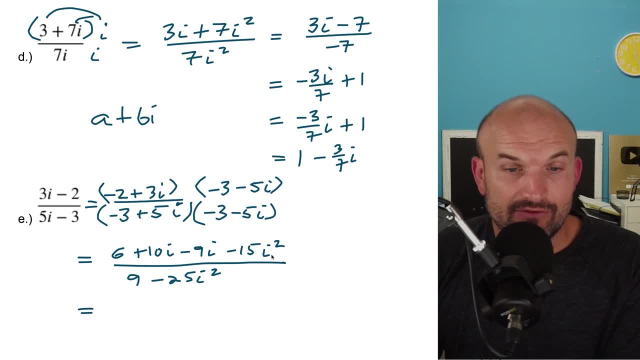 that's cool. Um, now again i squared is negative one, negative one times. fifth. negative 15 is going to be a positive 15.. So I can add those up together: Six plus 15 is going to be a 21,. 10 i minus a nine. i is going to be a positive i. So I can say plus i And then over. 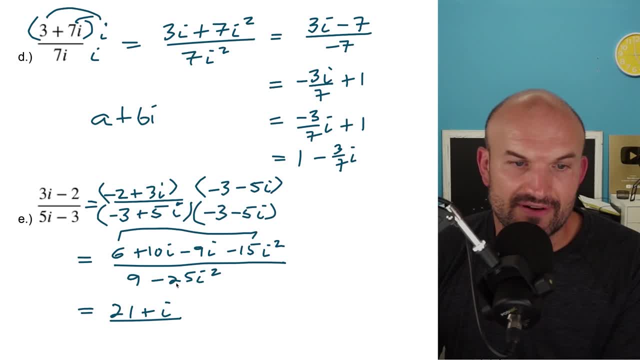 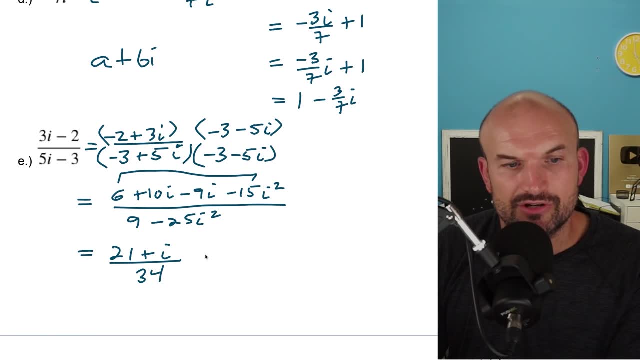 here we have an i squared which is negative one. So negative one times negative. 25 is now a positive 25, nine plus a positive 25 is going to be a 34.. Okay, So again now we can just kind of distribute. 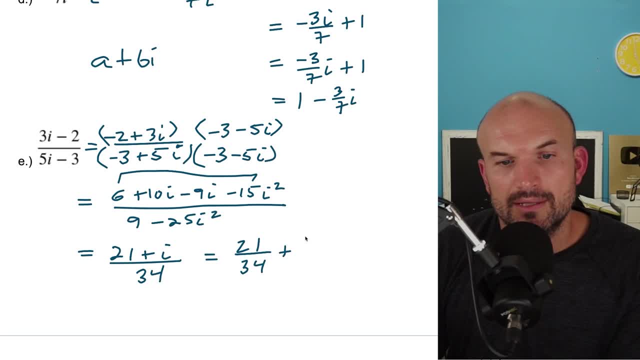 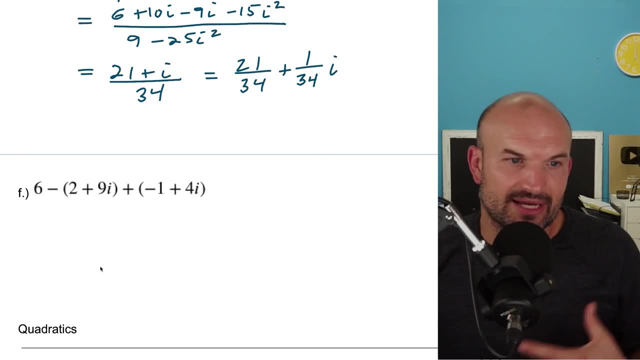 this So I can do a 21 over 34 plus a one over 34 i Um. and then, last but not least, you know also, just like we kind of worked on, you can also like add and subtract, um your terms, right? So just trying to a lot of times when you're thinking, 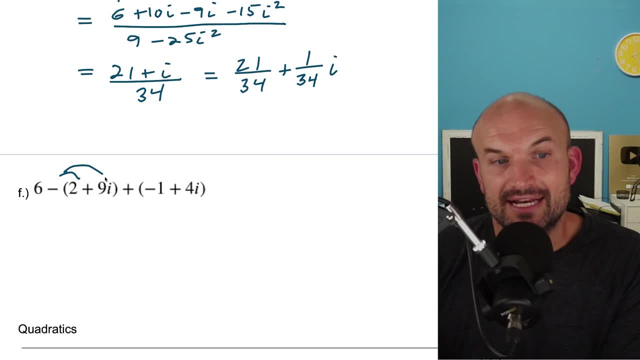 about this, you know, make sure you're just combining, like if they have an i, you can add and subtract them, right. So we let's go ahead and apply subtraction here. So it's six minus two, minus a nine i, Um, and then plus a negative is really just same thing as minus a one. 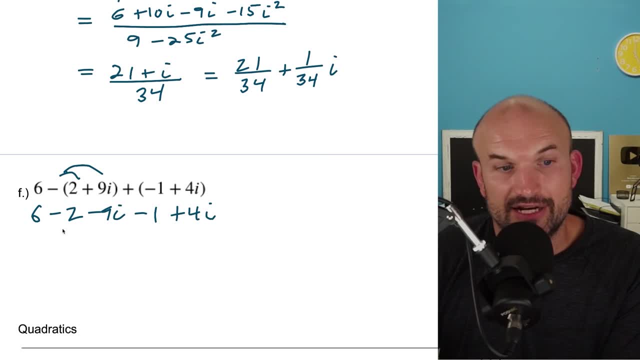 and you know, plus a four i. And now I can just kind of group things together: So six minus two minus one minus a nine i plus a four i, So that's going to be a negative one minus a nine i. So basically what I'm doing is just right into the go. So six minus two is going to be a four. 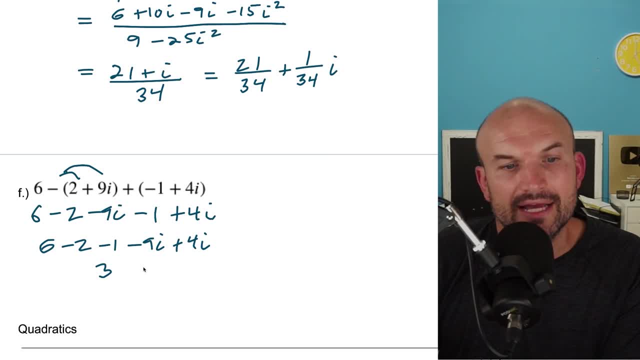 four minus one is going to be a three negative nine i plus a four i, It's going to be a negative five i, And therefore that would be your simplified term Again, you always want to write it in that a plus b i format. All right, So now let's go and move on to quadratics. 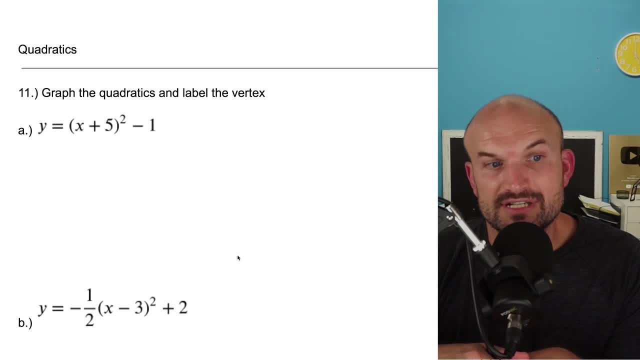 So we want to graph the quadratics and label the, the vertex. So in this case we have: y equals a x plus five, quantity squared Um minus one. So just remember when we're dealing like with the parent graph here. Okay, Um, a couple of things I just want to kind of quickly review. So here's your quadratic. 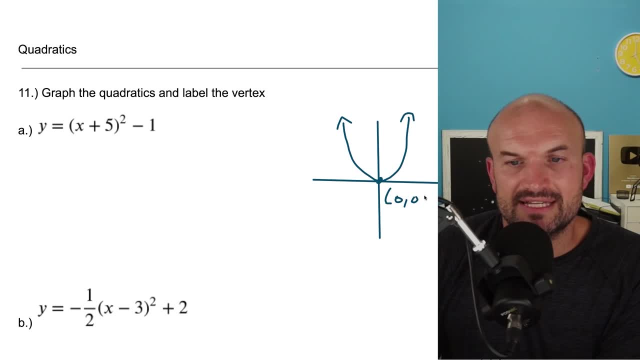 Okay, And when we're talking about the vertex, uh, the parent graph, it's at zero, comma, zero, and we have F of X. Let's just call this F of X. Um, this is going to be at a, a times X minus H, quantity squared plus K. The vertex is the bottom or the top of your graph. 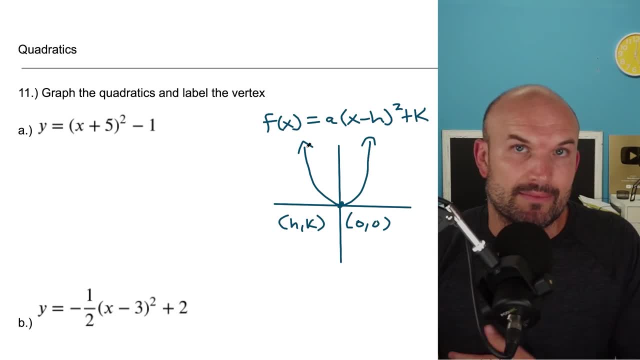 And a lot of times we also will just represent that as your H comma K: Okay. Now, another way we could actually write this is X minus parentheses, H squared, Okay, So that's kind of like a really important thing. Um, that I want you to kind of focus in on here, because 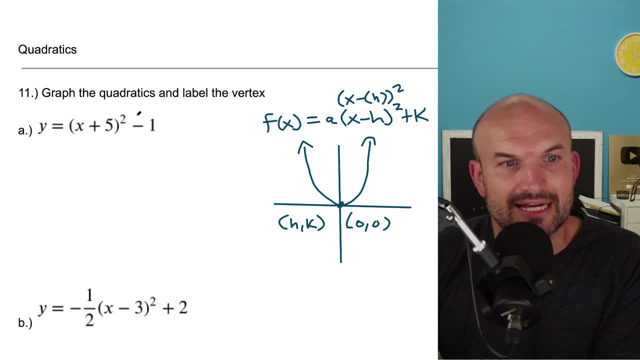 it's X minus H. So when you see a problem like this, a lot of students will say like, Oh, five negative one is the vertex. And no, that's not the vertex. What you're simply going to do is write it in this exact same form. So if I do that, what I could write this as? as an X minus. 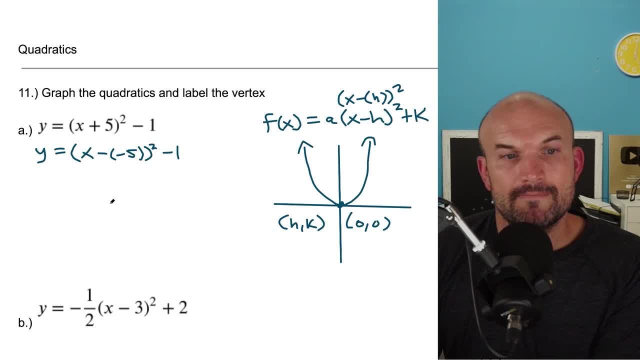 a negative five quantity squared minus one right, Because isn't minus a negative five, positive five- Yes, it is. So that's going to be very helpful Now. now, what we can do here is we can say: all right, H equals a negative five and K equals a negative one. So now I can write my vertex. 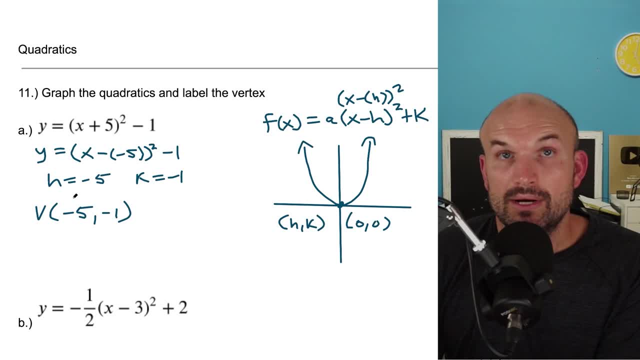 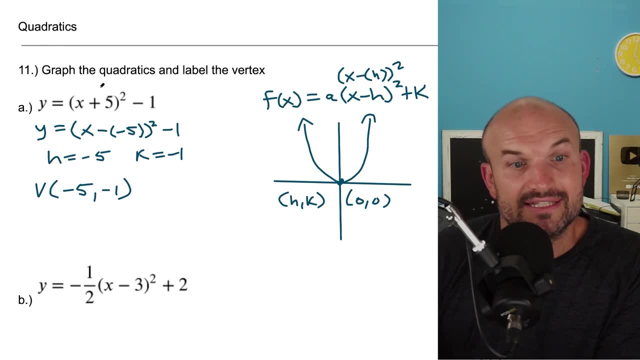 So I'll just write, say: vertex is going to be a negative five comma, negative one. Um, this example: uh, we're basically going to do the exact same thing, the exact same. Oh, do I supposed to graph it? Yeah, I said graph the function, Okay, Um, now in this example, 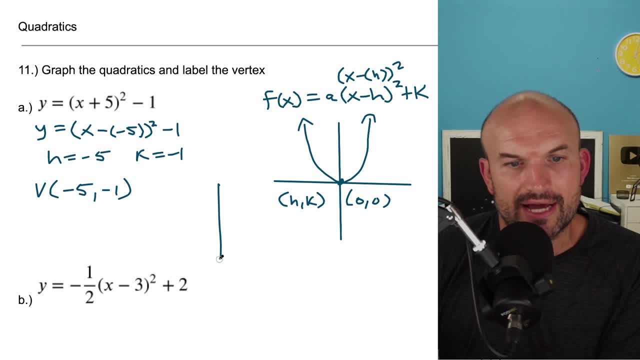 so let's go ahead and do a quick little graph. Um, so what I'm simply going to do now is just take this parent graph that I made, which I made it kind of too big, but what we're going to do is take this paragraph, and now we're. 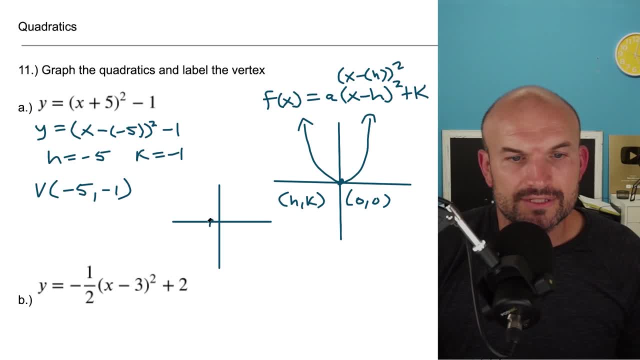 going to shift it five units to the left and then one unit down. one, two, three, four, five and then one unit down. Okay, Now it's important that the understand from about quadratics If your teacher is wanting you to kind of get um, kind of like dialed in or like really good on. 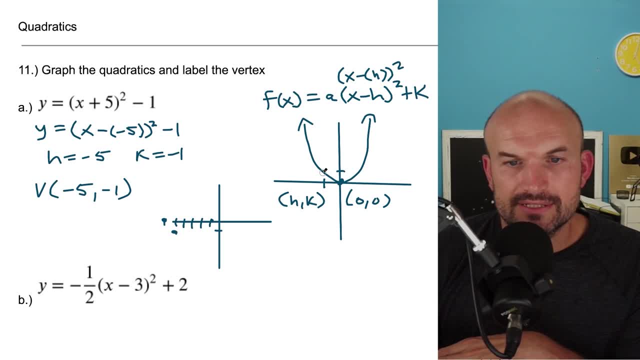 your graphing, that the graphs go up one over one, right? So you have this point up one over one And then you go up to up four. So one, two, three, four. So up two up four, up two up four. Okay. 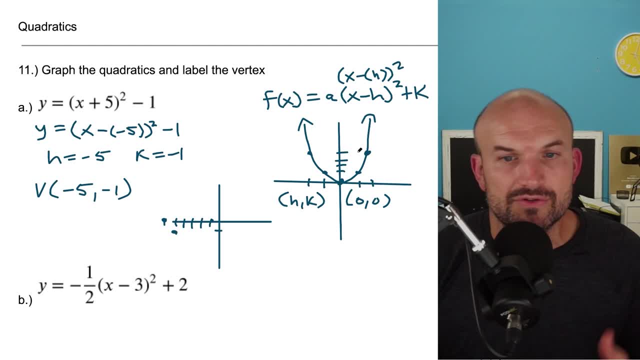 Because, right, If you said like two, two squared would be four, right Negative, two negative, two squared would be four. So that's kind of the relationship that that graph is going to be um kind of taking. So I'm just going to follow that exact same pattern. So I went left five. 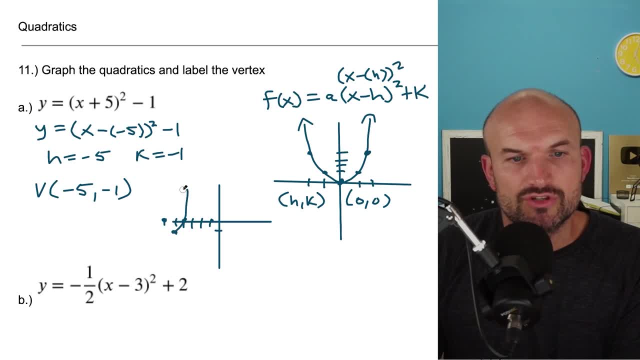 down one, So I can go left one over one, because there is no stretch or compression of this graph. So that's what that graph would look like And that is going to be my vertex here of negative five common negative one. All right, Um, and also it's going to be opening up, because my a, which is a 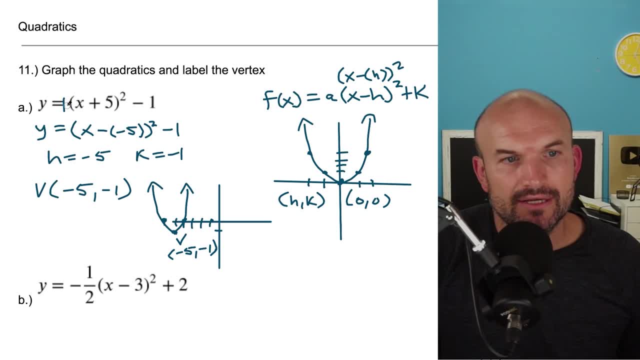 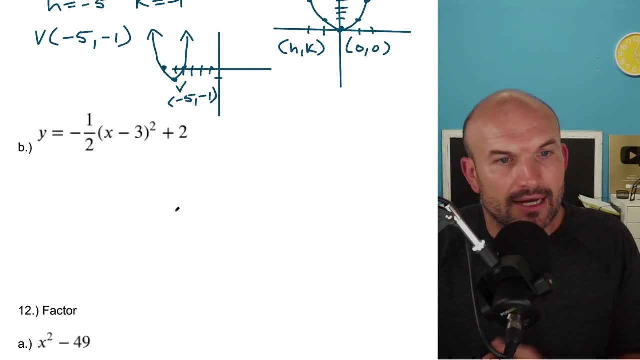 one. right, You can. technically, my a is a positive one, So therefore there's no stretch or compression, but the graph is going to be opening up because it's positive. Now, in this example, um, what I want you to see is that the a is now negative and it's actually being vertically compressed. 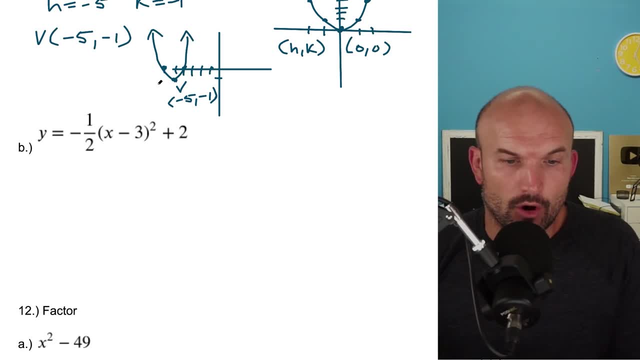 So what's happening is: um, when I go over one instead of going up one, is only going up one, half right. So when I go over two instead of going up four, it's only going up two, but actually. 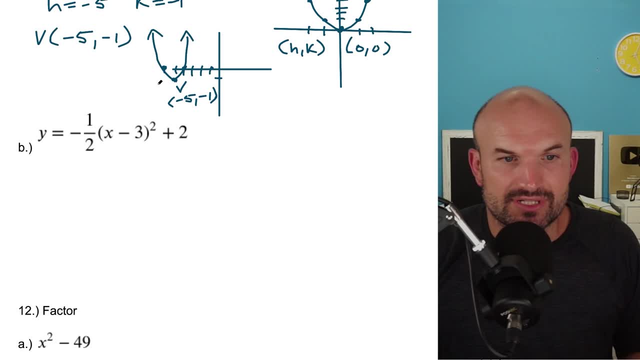 we're not going up, We're going down because it's negative. right, When you have a negative, that's going to be forcing it down. So hopefully you recognize the vertex here is going to be a negative three, positive, two. Um, the graph is going to be very similar to the one we just did, So we're just 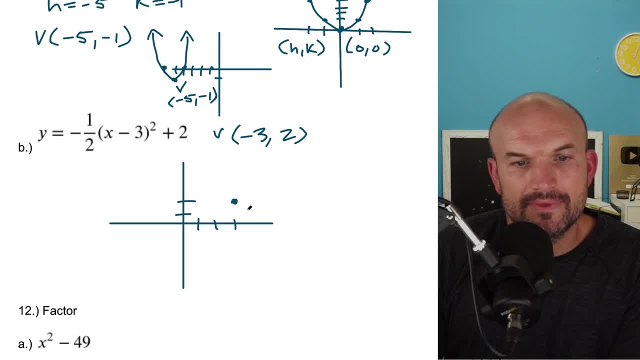 going to go one, two, three up two. Okay, But now if you, just if you have to be a stickler, you know again, as I mentioned, remember the other one was over two, it'd be down four. Well, this one. 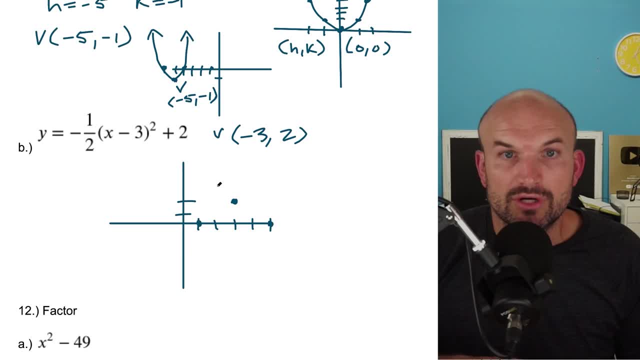 so it'd kind of be. it's going to be a little bit more. this is what we call a vertical compression And, again, since my a is negative, that's going to be forcing this graph to go down, So you can see how this one's a little bit wider, It looks like, or vertically compressed, All right, Um. 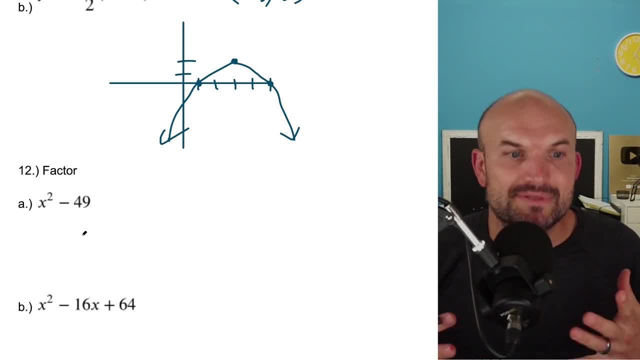 another thing that I would probably say is like one of the hugest things that you absolutely need to know, um for this guys, is two factor like factoring comes up time and time and time again in pre-calculus. So you're just going to have to get really, really good at factoring. 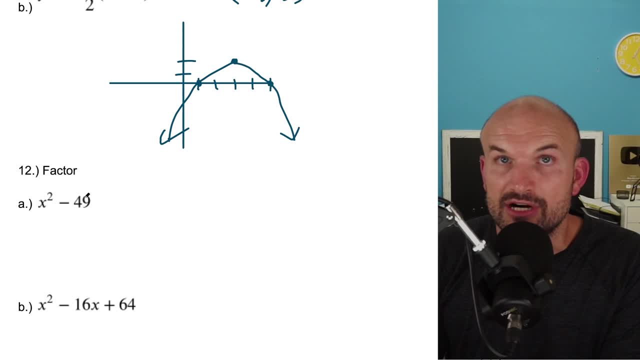 Um, so, one thing to recognize: whenever you have a difference of two, whenever you see two terms quadratic, just you know, think about difference of two squares, difference of two squares right And again, that relationship is whenever you have the form of a squared minus B squared. 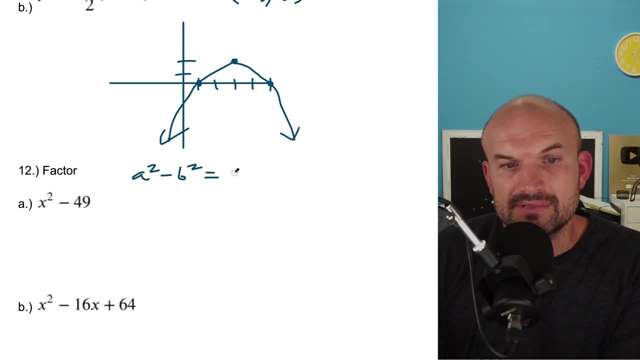 So the first term is squared and the last term is squared, And that's a difference of those two terms. Remember, that's a minus B times a plus B. Okay, So what's the square root of X squared? Well, that's just going to be an X, right? So you could say a is equal to X. Well, what's the square? 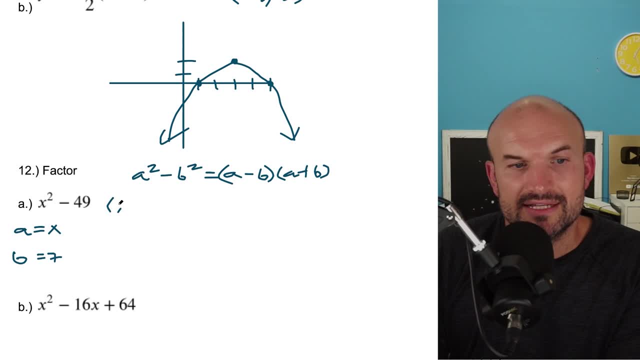 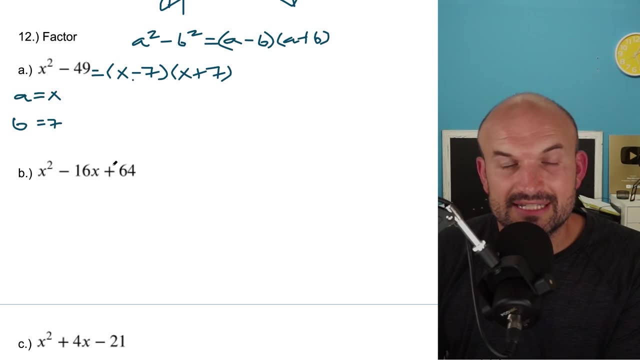 root of 49?? Well, that's going to be a seven, right? So now I can write this as a X minus seven times a X plus seven, And voila Um. now, in this case, again, something else is important We recognize. here Again, we have a first two terms. 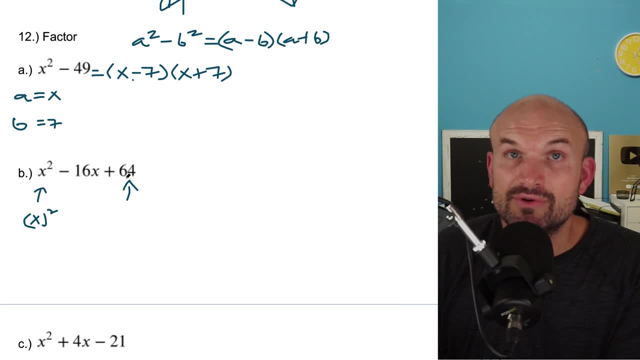 which is a square number right, So that you can rewrite that as an X squared. and you can rewrite 64 as a square number right, That's a eight squared. So when the first term and last term are squared, think difference of two squares, of as two terms, or think of a perfect square. 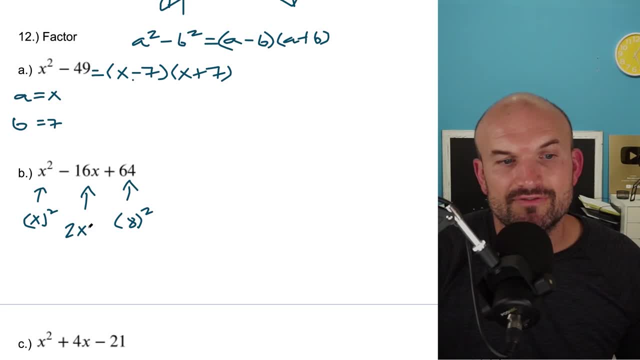 trinomial If the middle term is two times your first term, or in times your last term, right, So that two times X and again, does that work? Yes, it is a 16.. Now, again the negative. all that's going to tell you. 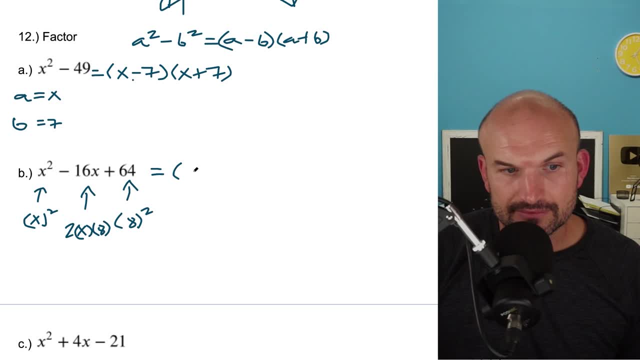 is that the binomial needs to be a, also negative. So therefore this form is going to be an X minus eight times an X minus eight. Okay, And that's how that works, Cause negative eight times negative eight is positive 64. negative eight X plus a negative eight X is going to be a negative 16.. 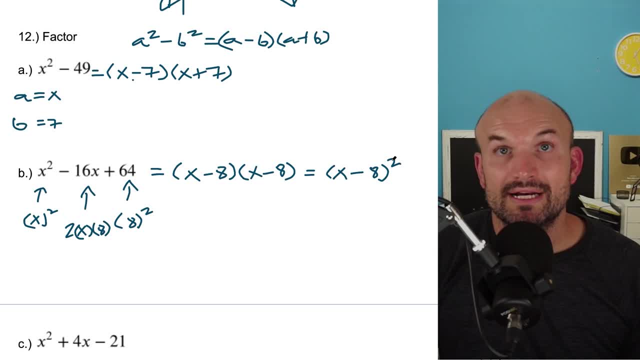 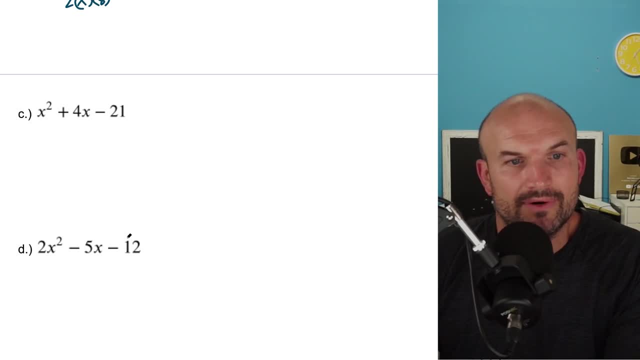 And we can rewrite this as a X minus eight quantity squared. Now the next one, um, now we're going to be looking at is: now, you notice, my last term is now square number, right? So now what I'm going to do is basically just say: 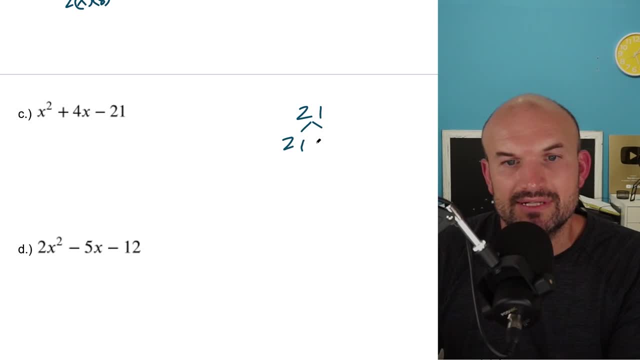 all right, what two numbers multiply to give me 21.. Okay, And you have 21 times one- And a lot of times, guys, you remember you need to do this in your head- and a seven times three. Now, whenever the last number is negative, what you're going to do is look at the difference. 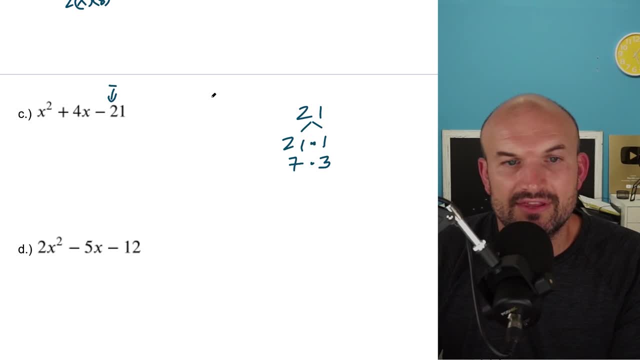 Okay, So when the last number is negative, what you, what I want you to think is negative, is difference, right? So look at your factors and say which of these factors have a difference of your middle term, which is four. Well, obviously, you can see, that's seven and three. 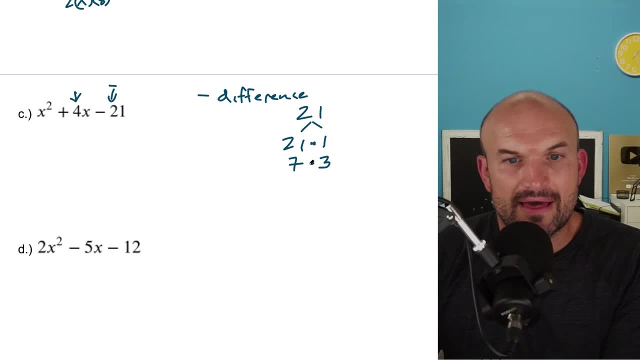 right, Those have a difference. Now, since they have a positive difference, that means my seven has to be positive And my three has to be negative. One of them has to be negative though, because when you multiply seven times three, to make that a negative 21,. one of them has to be negative, But since the difference is 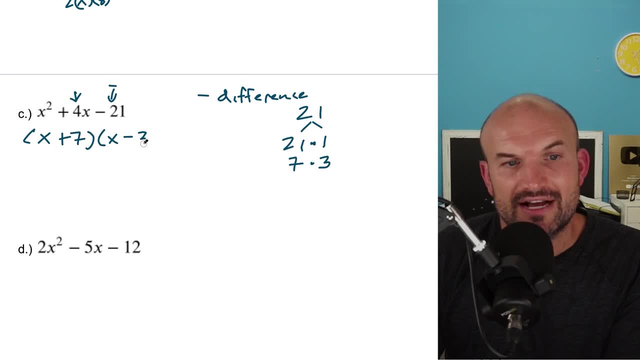 positive, the larger of the two factors is going to be your positive factor. So therefore, the factor form of this is to be X plus seven and an X minus three. Now, in this example- um, this one gets a little bit more difficult. So the main thing I want you to recognize about this is: you know, 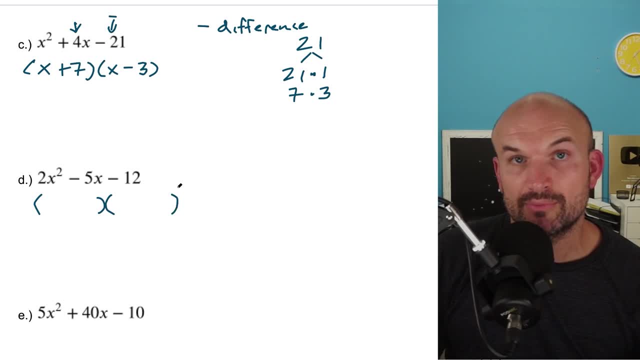 all quadratics. all quadratics can be broken down into a product of two binomials. So you always want to see if you can factor something out, which in this case, unfortunately, we cannot. but we do know, like if I was to multiply this out right, If I was going to use foil, I can have a two X times an X. 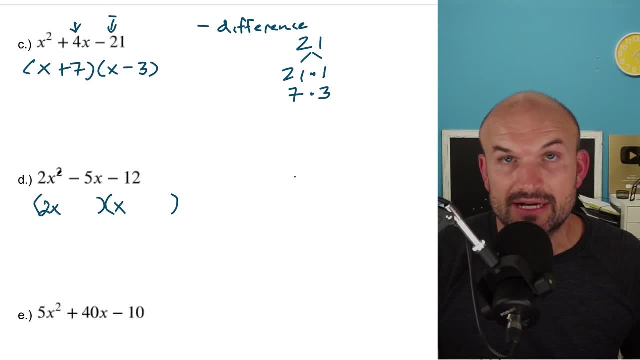 right, And you know that would work- to give me that two X squared. Now for the 12, though. we have options. So we have a 12 times one, Um, we have a six times two and we have a four times. 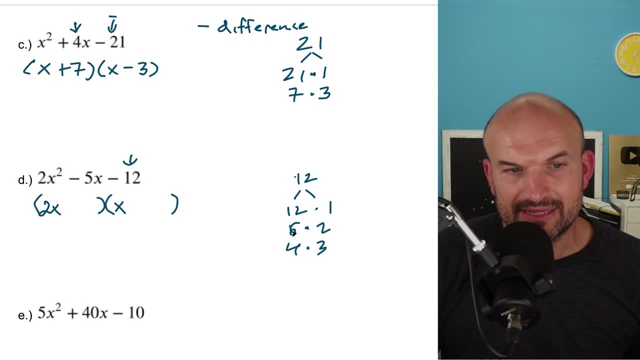 three. Now, again, we're looking at a negative right. So we're thinking about the difference, but none of these have a difference of five. Well, and that's for good reason, because what we're actually looking for is we're looking for the products of my inner and my outer to have. 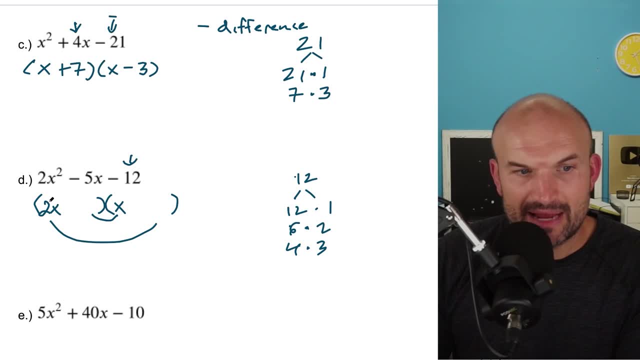 a difference of five. So now what we're doing is kind of doing a little mental math, Like if I did a two X, if I put a 12 here, two X times 12 would be a 24.. Oh, I need to. what am I going to multiply? 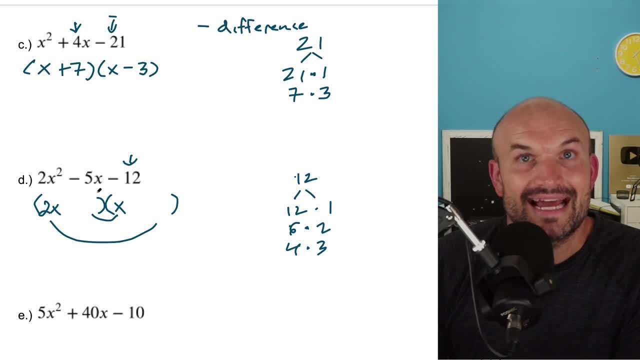 X by to get it to be a difference of five. right, That'd be like I need to get to 19.. That's going to be kind of difficult. So I kind of made me think about: well, if I did a, what about if I did a two X. 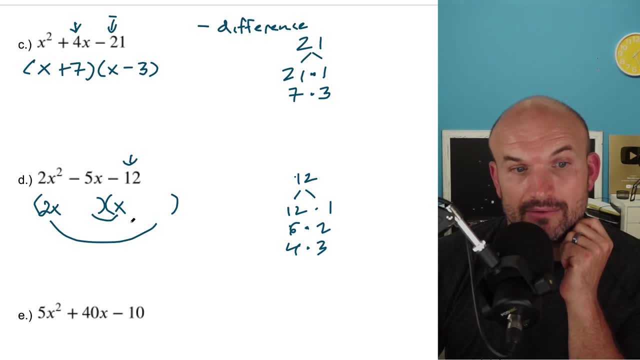 times four, that'd be an eight, and eight and three, right Cause, then a three times X. well, that would give me a difference And like, yeah, that'd work. Now, since my middle term is negative, my larger of my two products, either my inner or my outer, needs to be negative. 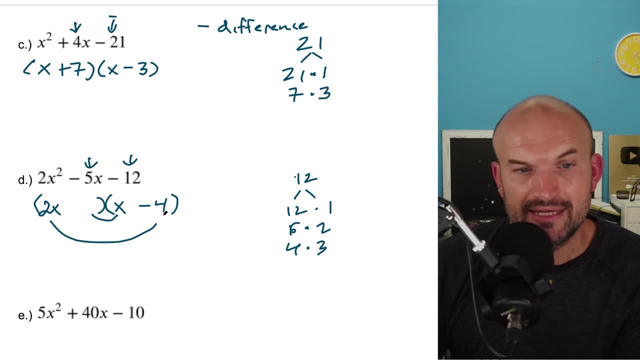 So two X times a negative four is going to give me a negative eight right, And then a three positive three times X gives me a positive three right. So I have a three X, Um, and then I'm going to add that to a negative eight X. That should give me a negative five X. Do you see how that? 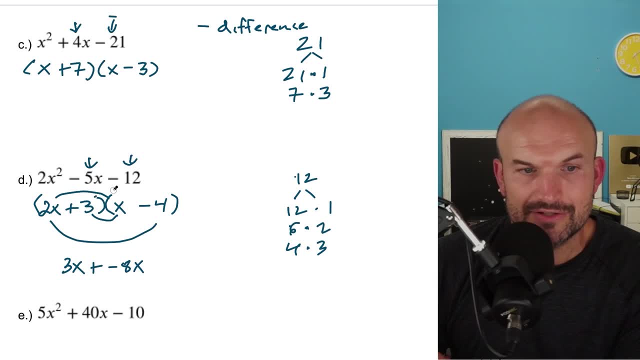 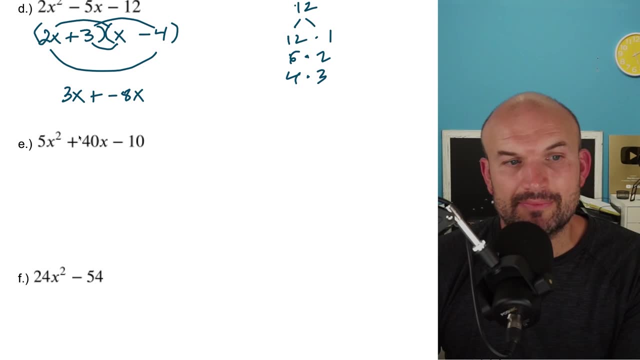 works here. And then, obviously, my first two terms needs to give me two X squared And my last two terms needs to give me a negative 12.. So again, guys, it just takes some practice, but that's why we are working through all these examples. So in this example you can see we have some larger. 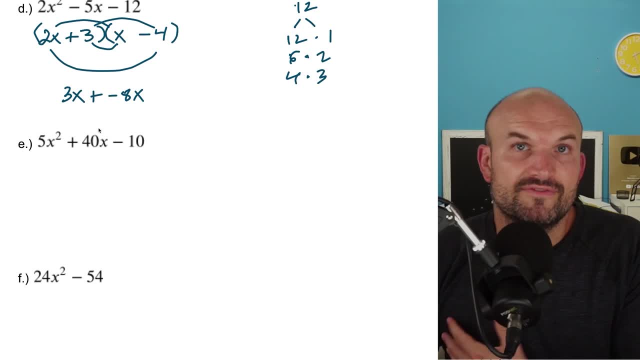 numbers right, But we always want to look to see if there's something you can kind of, you know, easily factor out first And you hopefully recognize here that these all are, all these terms, the five X squared, the 40 X and the negative 10 are all divisible by five. So therefore, 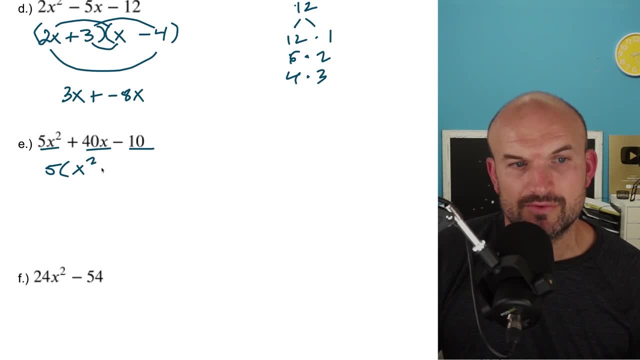 I can take out a five. Um, when I divide out a five, I'm going to be left with a X squared plus minus a two. Now, unfortunately, though, this is not going to be factorable any further, because you know, if I had like a two, like what two numbers multiply to give me two like two, and 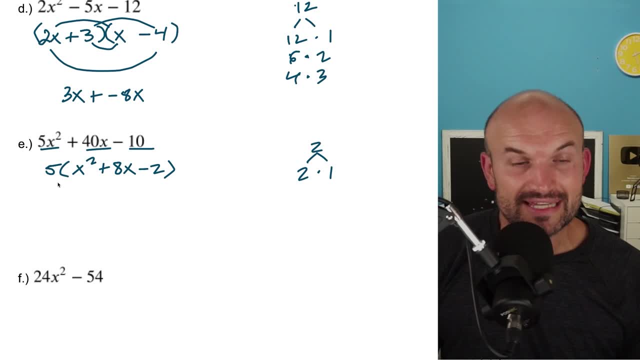 one like. that's my only option. I'm never going to be able to get an eight right. So then this is just going to be our factored four. Now, obviously, when we get into solving, we could actually use, like completing, the square or quadratic formula. But again for right now, 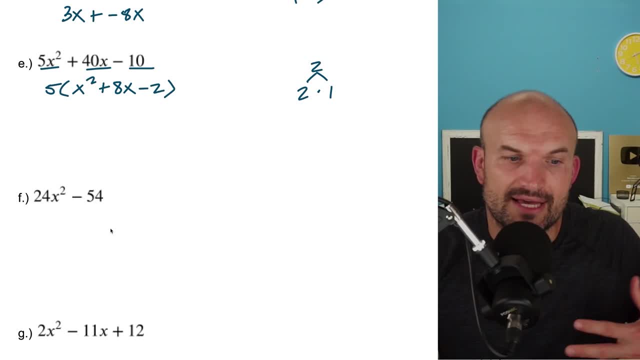 we're just trying to factor out our terms And again, we always want to look for terms that they have in common. So here's another example of saying, like all right, what does a 24 and a you know 54,, like what do these you know have in common? And to me it looks like we can divide. 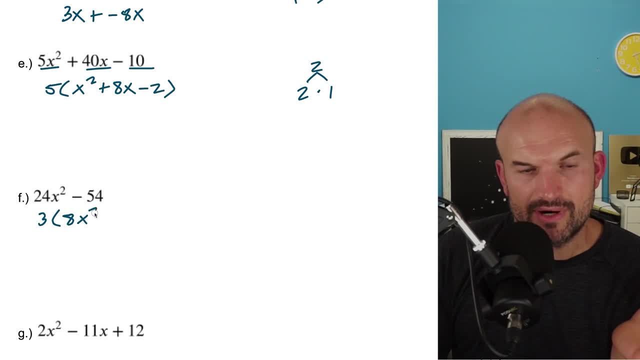 out a three. So if I divide out a three, that's going to give me an eight X squared, and divide out a three here, That's going to give me a minus an 18. So actually I could probably do a six, right? Yeah, I should have done a six So you could do a three, but then you're going to divide. 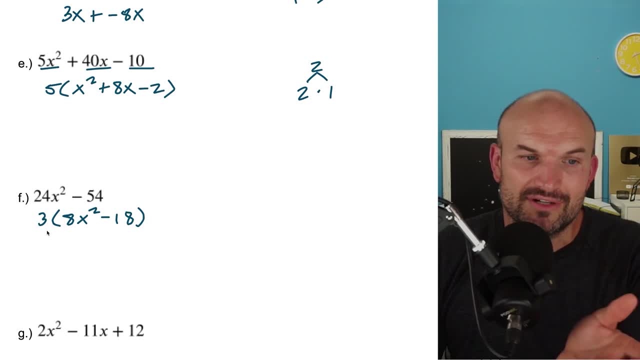 out another two, right? So why don't we just go from the six in general, Cause we want to get this to the most factored form. So if I go ahead and factor out a six right now, it's going to give me a 54 X squared. And then a six six times nine is going to give me a 54.. Okay, Now you can. 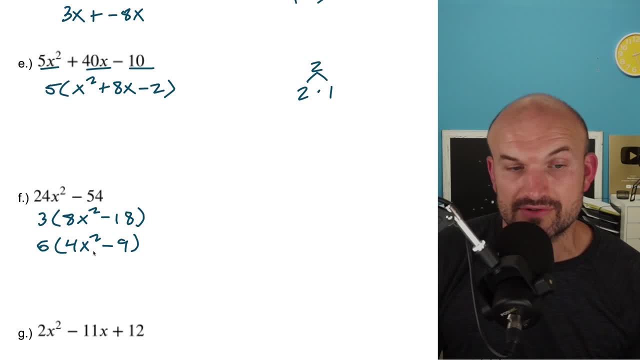 see I can further different um factor this down. This is the difference of two squares, right, I have a squared term minus another square term, So the way that I can factor this would be a two X minus three times a two X plus three. Okay, So, even if something like: if you didn't recognize, 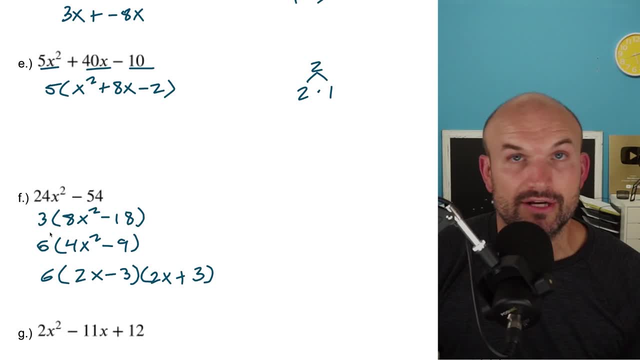 a six at first, like pick something right, Usually three or two or a five, you know those are kind of easy. And then, if you can further factor it down, you'll kind of notice what are the terms. you can kind of do, Um, and then you, then you can kind of. 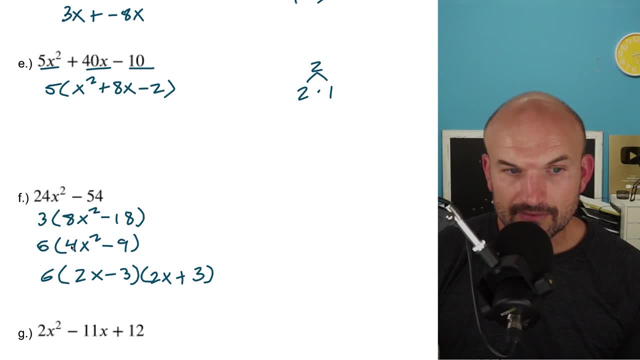 go back and redo it again, Right, But also, again, look for that special factoring technique. This is an example where we're actually able to factor out multiple terms. um, you know, factor out not just the common number, but then do a difference of two squares, And then, in this example, um. 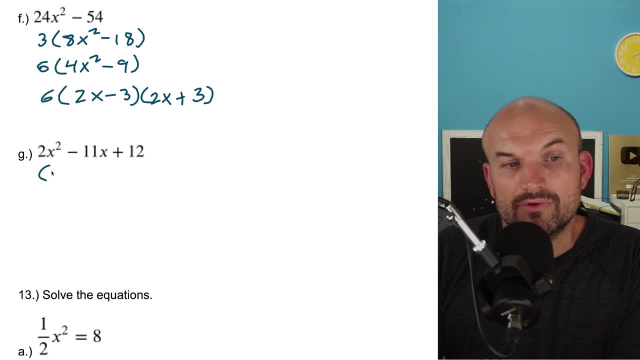 again, we know that binomials- I'm sorry, trinomials- can be brought written down as a product of two factors. So therefore I can rewrite this as a two X times X. Okay, Now I'm trying to look for the sum of these to be able to add to give me a negative 11.. But again, it's not the sum. 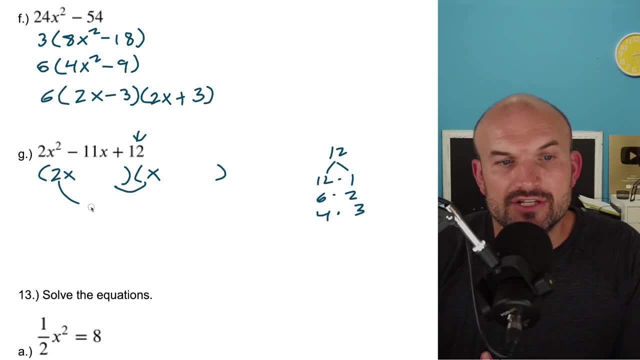 of the factors, because I have a coefficient here of my X squared, So it's going to be the sum of these two products, right? So two X times what plus a X times what is going to give me negative 11.. And again, those what's are going to be over here. So again, since this is a 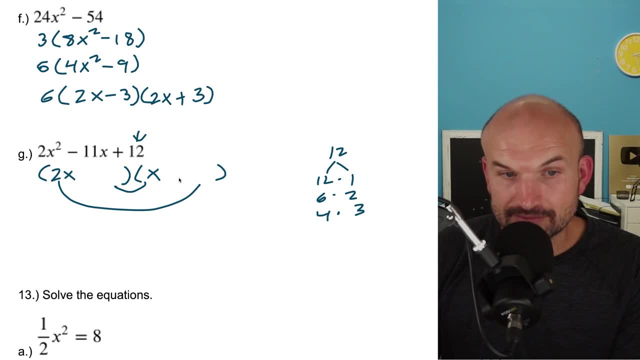 a positive. that means my two factors have to be the same, have to be the same signs. So what I notice here is- and they also have to be negative, since my middle term's negative- If I do a two X minus four, right, that's going to give me a negative eight. And if I did an X minus three, 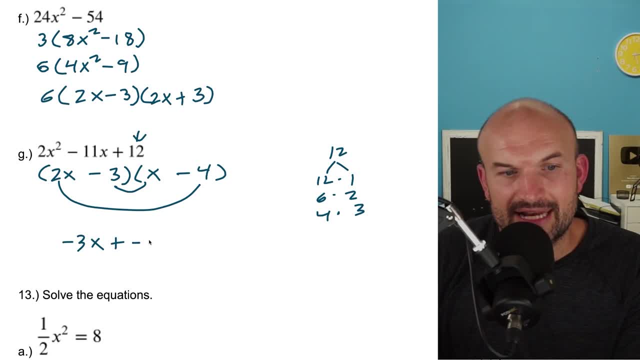 right, So that's a negative three X, and then that's going to be plus a negative, not negative, eight. That's going to be negative four X, right, So a negative four X, And you can see that that is going to add to give us a seven, which is not. I'm sorry. 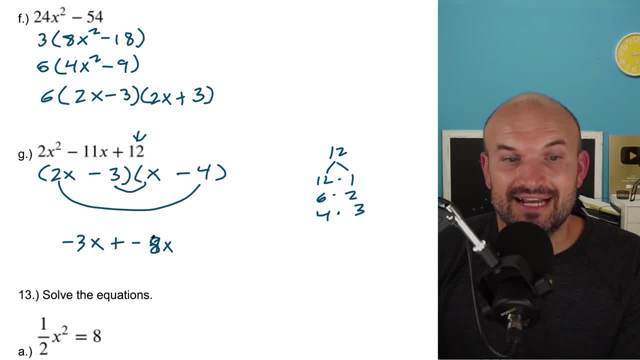 two times four, that's an eight. I'm making some mistakes here. So negative three X plus a negative eight X is going to give me a negative 11 X. Okay, So you can see how that's going to work in that regard. So, and then, yeah, that's going to be your factor form, And again, 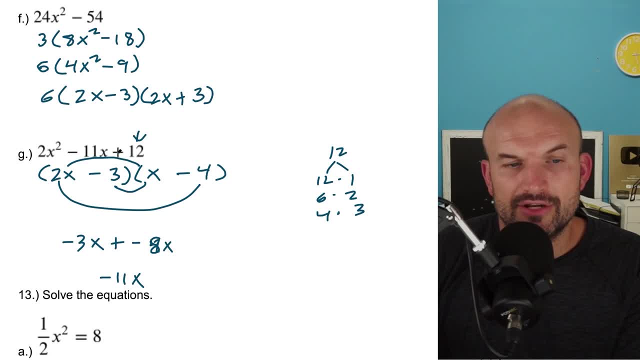 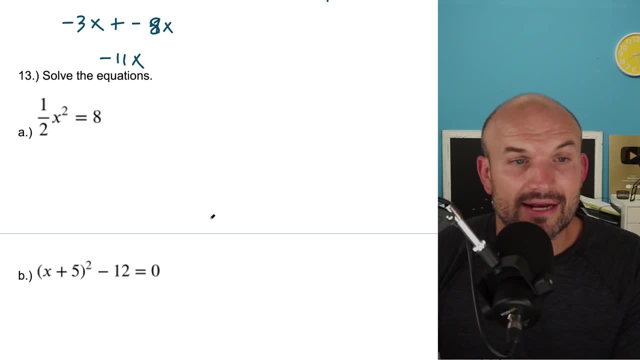 you can always check the first two terms right: Two X times X is two X squared. And you can also multiply negative three times 12 is going to give you a positive 12.. So you can see how that works out. All right now. So factoring is very important because we're going. 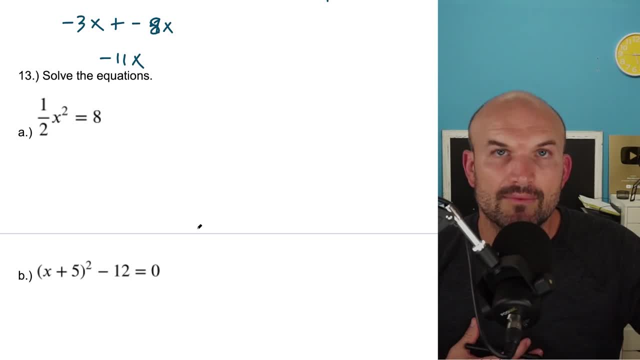 to not just do factoring in quadratics. It's going to expand to polynomials, Rational functions, trigonometric functions, But also we would need to make sure that we can factor or, I'm sorry, solve quadratic equations. So, like what we did with our radicals using the 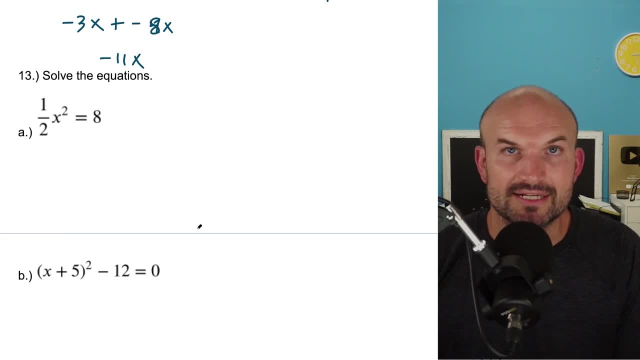 inverse operations. that's exactly the same thing we're going to do for the quadratics, Like: if you only have one term, if you only have one term squared, you can use your inverse operations. So basically, what that means is just undo what's happening to the variable. So in this case, 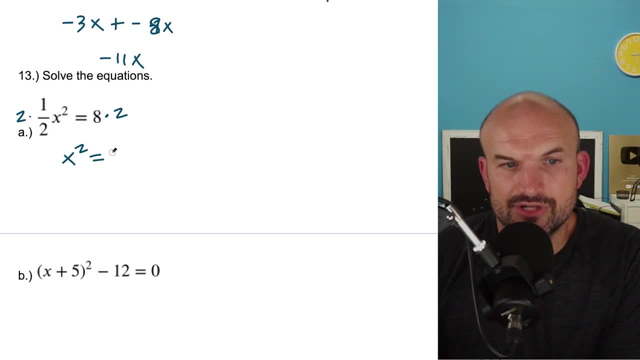 we're going to multiply by two on both sides, and I get a X. squared is equal to a 16.. Now it's very important, though, to recognize that you can only use your inverse operations when you have that square isolated right And when you take the inverse operation of the squaring that's going. 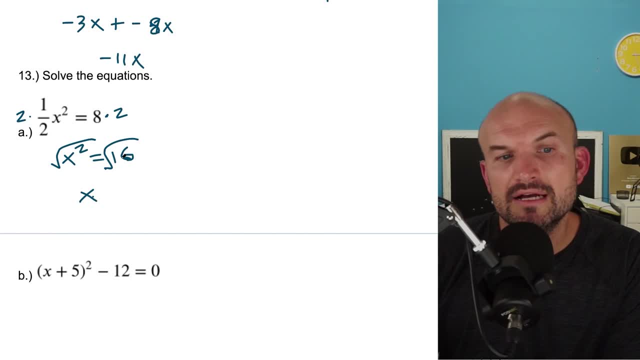 to be the square root, You have to make sure you include the plus or minus. So the square root of 16 is going to be a plus or minus a four, Okay, So you have to make sure you include both of those solutions. And again this kind of goes back to our options for quadratics. right, A quadrat can? 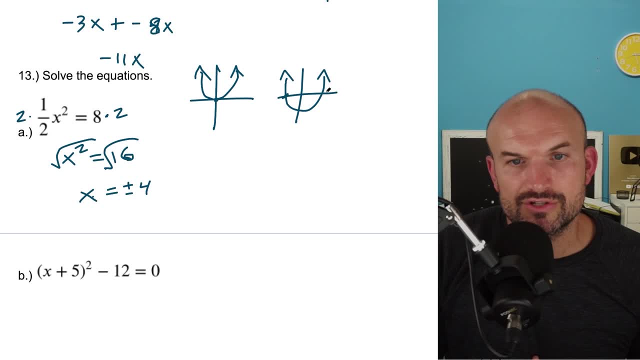 have one X intercept or one solution. It could have two solutions, right, Or it could also have no solutions. So that's a little bit more complicated, but it's a little bit more complicated. It's a little bit different than the square root function, right, When we were dealing with the 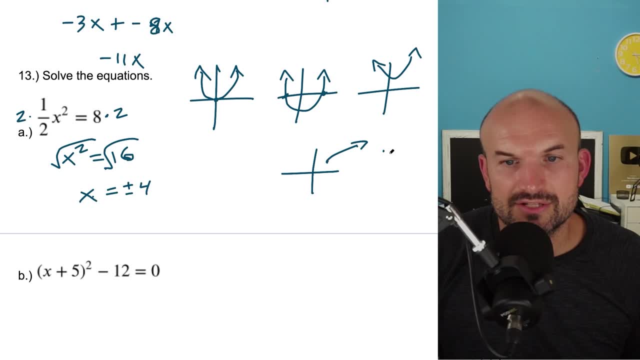 square root function, you could have no solution, but you also could have one solution, right, But there was no way that we were going to have, like, more than one solution going on. Now let's go and take a look at this example. Now again this example. notice: I only have one, X, right, So what? 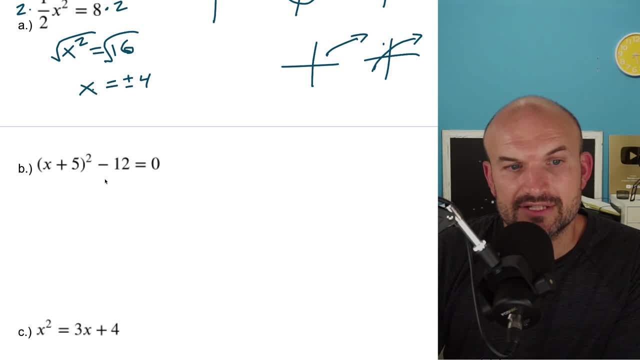 I'm going to do here. before I take the square root, I need to isolate this. So, to isolate this, I'm going to add a 12 to both sides. When I do that, I get an X plus five. Quadrat squared is: 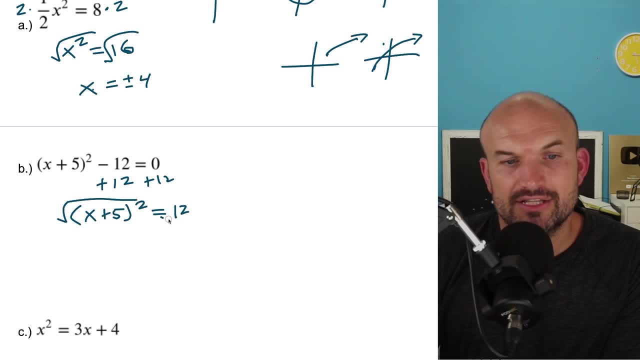 12.. Now I can go ahead and take the square root. So I'm going to take the square root on both sides. That's going to leave me with a X plus five equals the square root of 12.. Now we've simplified the. 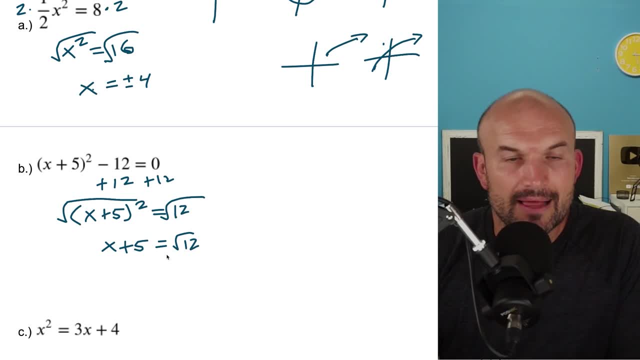 square root of 12. here already That's just going to be a two radical three. But again, remember, we introduce the square roots. That's a plus or minus, So be careful, Make sure you're always including that. So X is going to equal a negative five plus or minus a two square root of three, And that's. 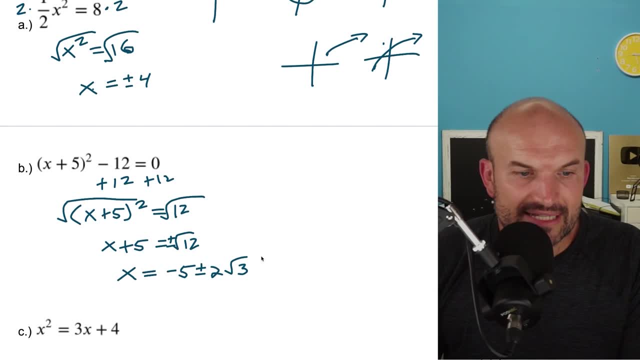 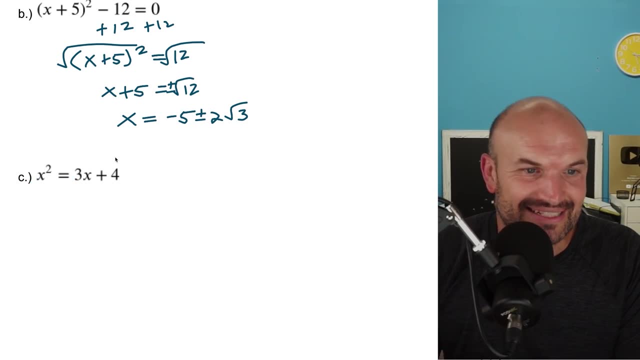 going to be your final answer. Again, we have our two answers here. Now, one of the big mistakes that students will make here is they get a problem like this and they say, oh, let's go ahead and take the square root to both sides. Don't do that, Please do not do that. Okay, What I want you to. 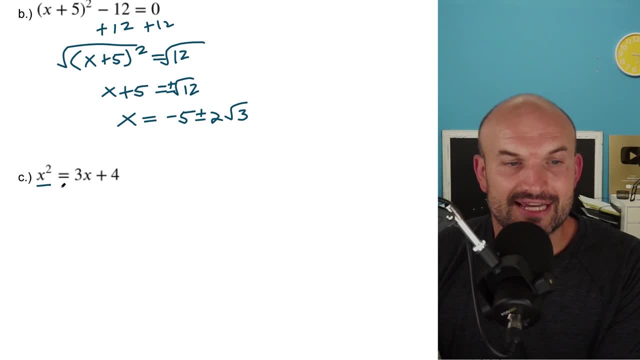 do in this case is whenever you have a quadratic and you have more than one X. in this case, you have an X squared and you have a linear X. What I want you to do is get them all over to the same side. You have to have your quadratic equation equal to zero, So we want it in our standard form. 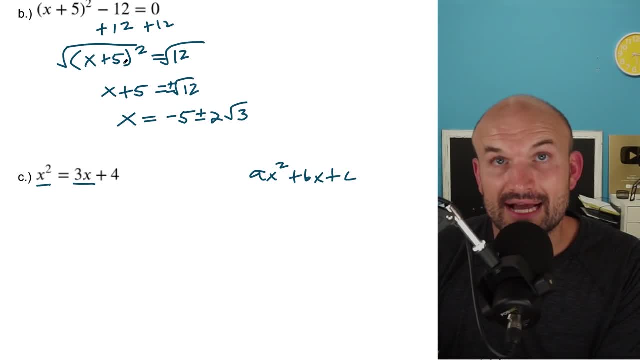 AX squared plus BX plus C. Again, if you have only one X, use inverse operations, But when you have an X squared plus BX plus C, you have to set it equal to zero. So what I'm going to do is I'm going. 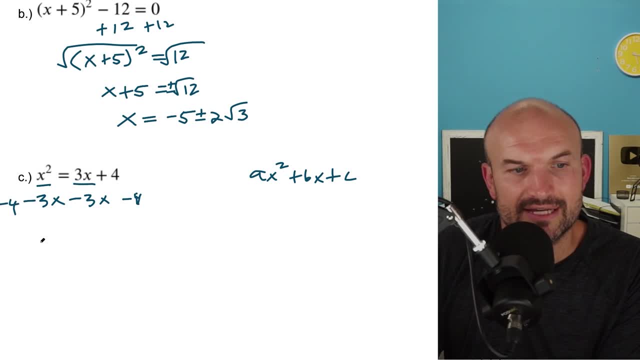 to get everything over on the right-hand side, just over to the left-hand side, And I'm going to put it in standard form here. So I'll have an X squared minus a three. X minus four is equal to zero. Okay, Now the first thing I want to do is check to see if this is factorable, right What? 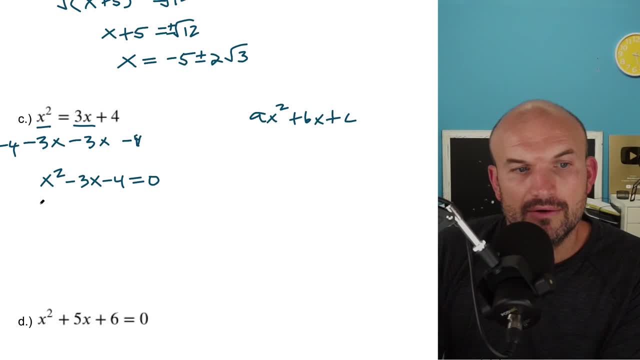 two numbers multiplied to give me negative four, add to give me a negative three. Well, that's not too bad. That's going to be an X minus four times an X plus a one, And that equals zero. Now we have property right. So I can say: X minus four equals zero and an X plus one equals zero. So now I can. 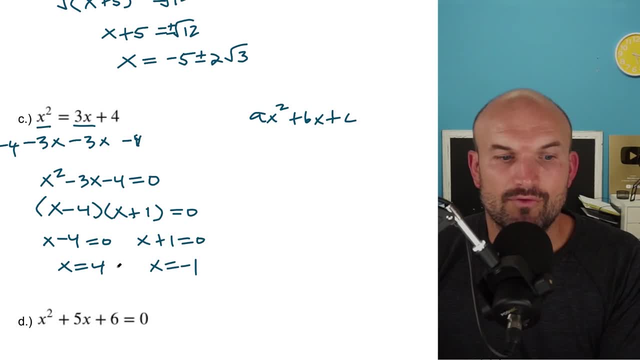 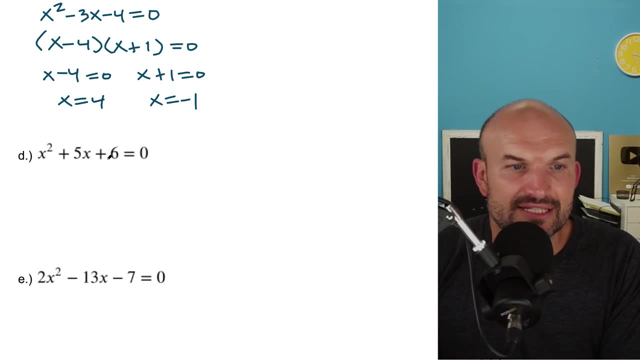 say, X equals four and X is now going to equal a negative one. In this example it's already set equal to zero. So we're basically going to apply the same approach. You know what two numbers multiply to give me six, are going to add to give me a five, And we recognize here that, hmm, that. 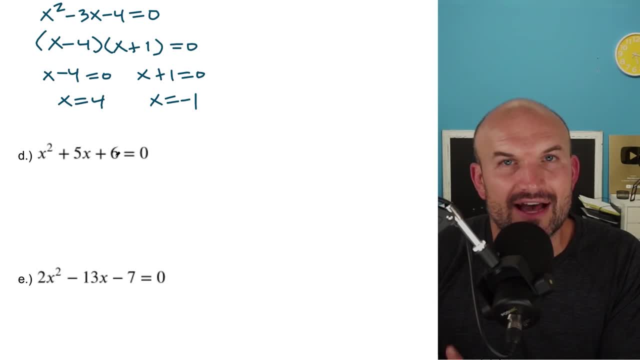 doesn't work right, Like there's no two numbers that multiply to give you six, add to give you five, but that's if you're thinking about six and one. So a lot of students will think, oh, six and one, that doesn't work. 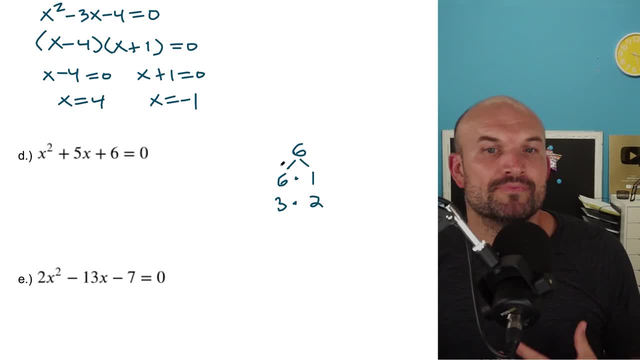 But what about three and two? right, Remember, there's multiple factors. So that's why I think it's always helpful to kind of write down all of your factors. Um, because when you're looking at this last term as positive, you're looking for the sum of your two factors to equal your middle. 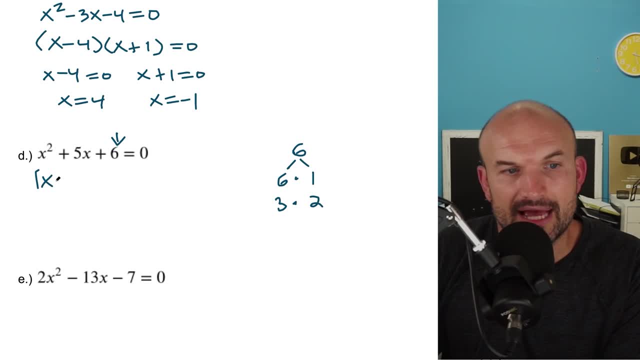 term, And that's why three and two are going to work. So this one could be a X plus three times an X plus two, quantity squared, And that equals zero. Therefore now I can say X plus three equals zero, X plus two equals zero And therefore X equals negative two. No, X equals a negative. 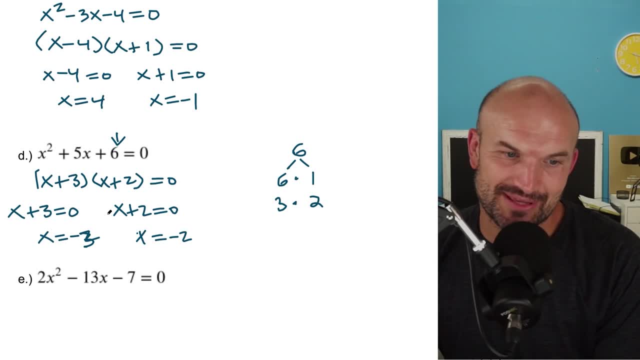 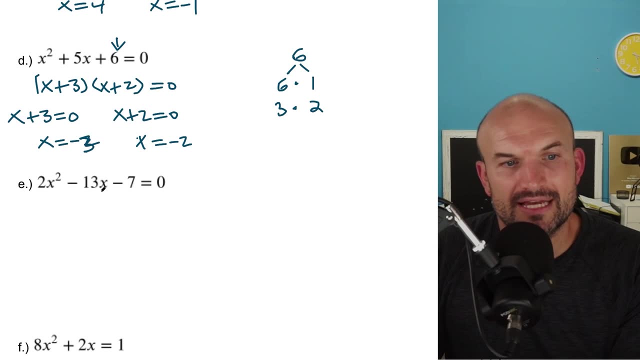 three. Then here an X equals a negative two. I think I was just kind of switching them up. Uh, on this next example, again we're going to be looking at the same thing here. Um, as far as trying to see if it's factorable, Now again I want to be able to see. can I rewrite this? 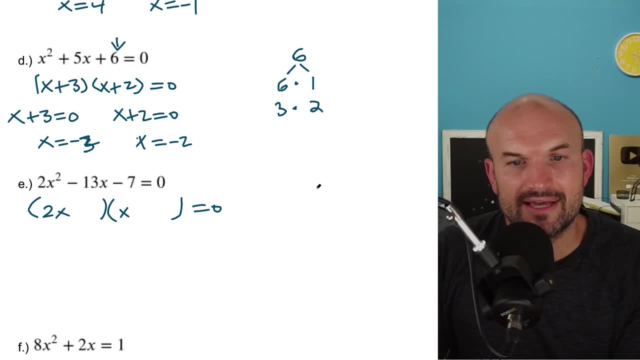 in factored form, right? So I have a two X and an X. Now again here. forget about the negative, just for a second. Let's do seven. That can be a seven times one. Well, again, if I want a, 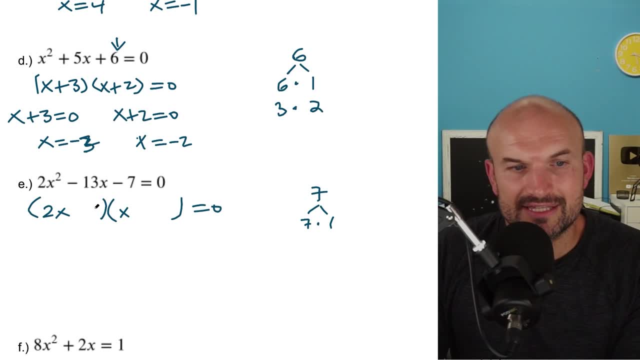 difference of 13,. like if I did it, like, just think about it, If I put a negative, I'm going to put a seven here and a one here. right? Two times, two times one is two, seven times, you know, one is. 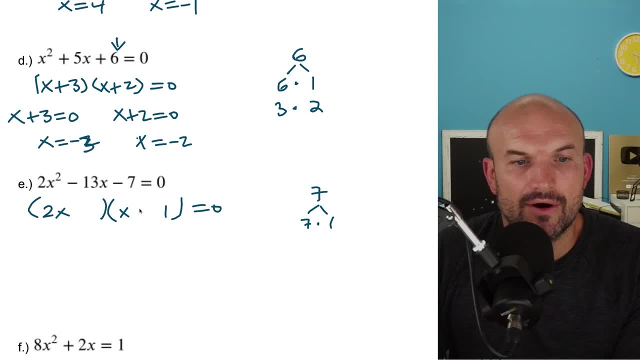 going to be seven. That's have a difference of five. That's not going to work Right. So I do recognize. though, when I do two X times a seven, that gives me a 14 X. that's really close to a 13. 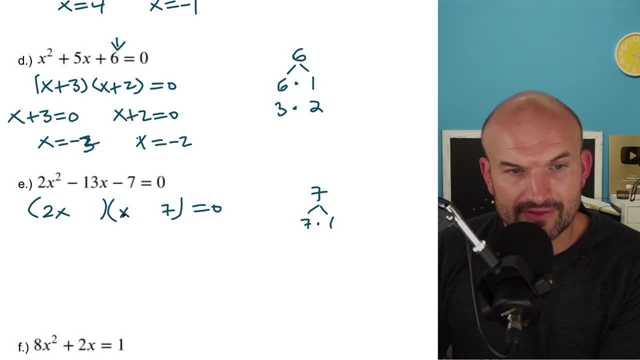 X. And then also, you know this there, um, one times X is going to give me that one X that's going to give me that difference. Now, since my middle term is negative, I want my larger of my two products, my inner or my outer right, To be negative, So I'm going to put a seven here and a 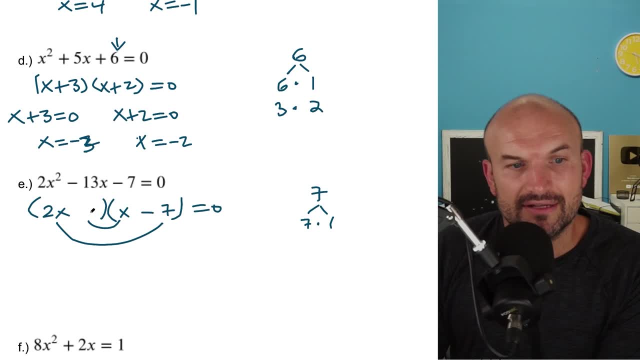 negative. Well, the larger of the two products is going to be the two X times seven. So that's a negative seven and that's going to be a positive one. Okay, But again, now we're trying to solve. So now I can set these both equal to zero using the zero product property And therefore, 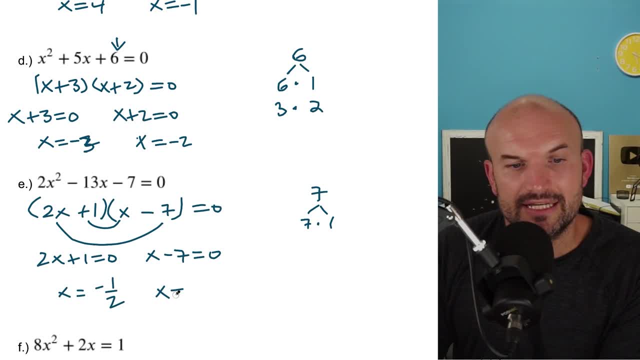 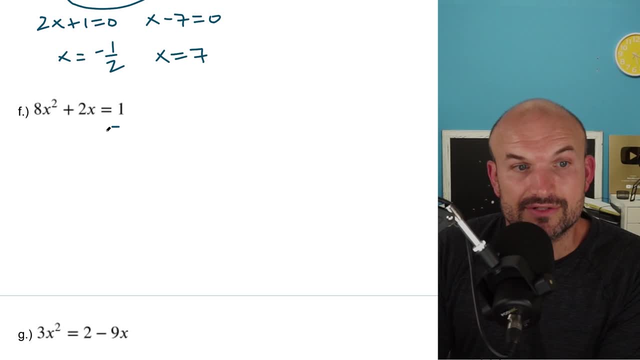 I get: X equals a negative one half, And here X is going to equal a positive seven. Um, now, in this example- uh, again, make sure you are setting it equal to zero. So you subtract the one on both sides and I get an eight X squared plus a two X minus one equals zero. 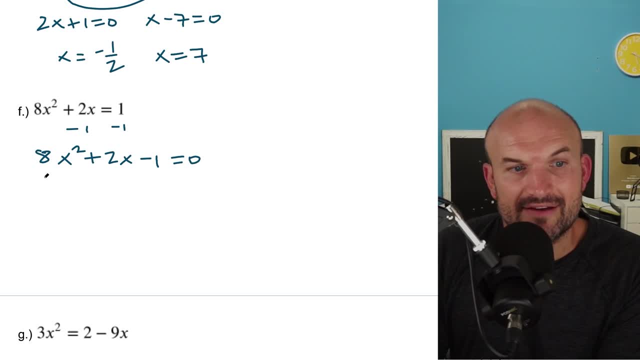 And again, in this case, what I want to simply do is now: now, here we kind of have some options right, So you could say, um, I could do an eight X times X, or I could do a four X. 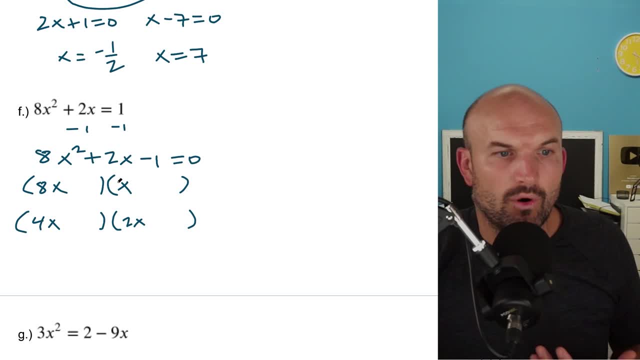 right Times a two X And again my options for a negative one. um, you know what two numbers multiply to give me negative one. Well, you know, I only have a negative one times positive one right Um, now it looks like here I can get a difference of two If I went ahead and said: 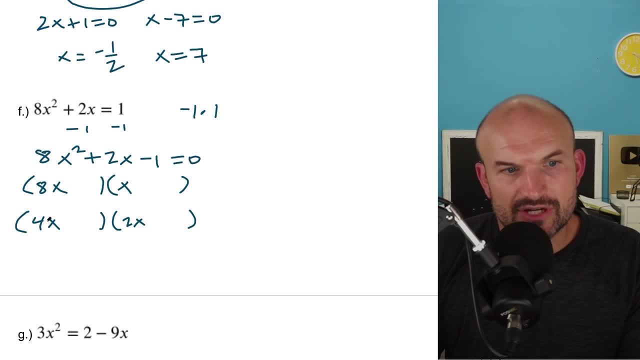 and again, I want that difference to be a positive right. So if I did a four X plus one and then put a negative one right here, I think this would work. And again, let's just check your work: Four X times two X is an eight X squared right. Negative one times negative one is going. 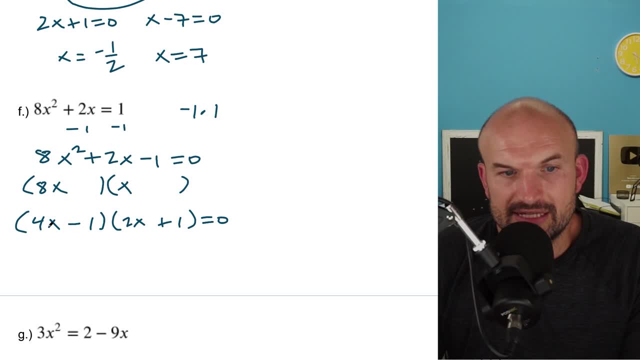 to be a negative one. This is going to be giving me a negative two X, right. This is giving me a positive four X, And you can see that. Hey, yes, it does work. So now I can set them both, Actually. 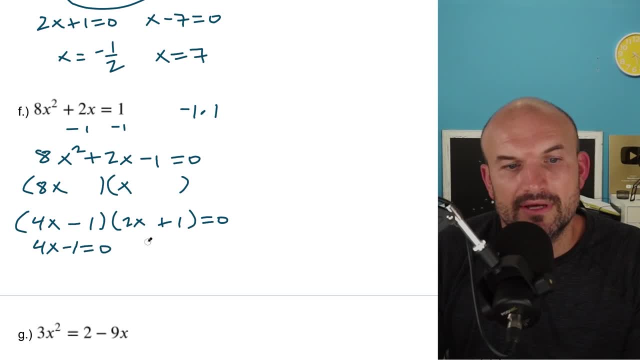 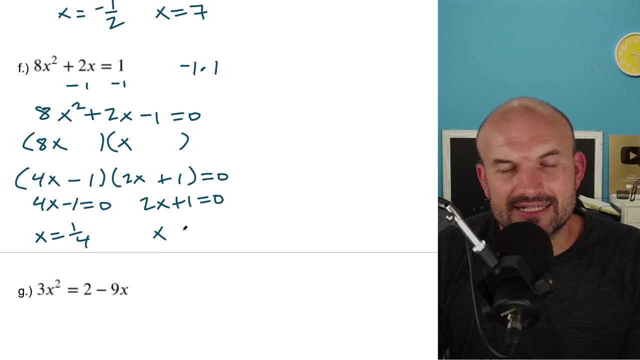 let's do it over here. And we got two of them. So four X minus one equals zero, and a two X plus one is equal to zero. And now I can see X, it's going to equal a one fourth. And here X is going to equal a negative one, half. And again. 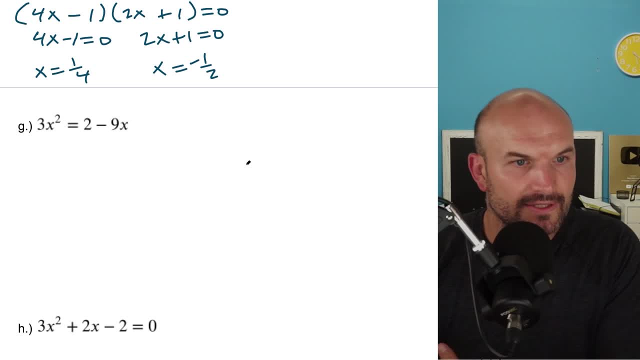 all I'm doing is just using my inverse operations to solve for them. Okay, Um, now it's going to work on these two examples. So again kind of same idea. Again, don't use inverse operations. Notice how we have two Xs. Let's get everything over to the same side. So let's add a nine X. 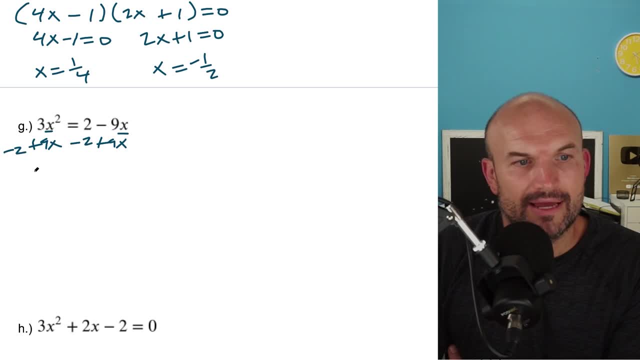 and let's subtract a two. Okay, So therefore I'm left with a three X squared Um, let's see, plus a nine. X minus, Say two, equals zero. Okay, Now again I'm looking into factoring this out Like: 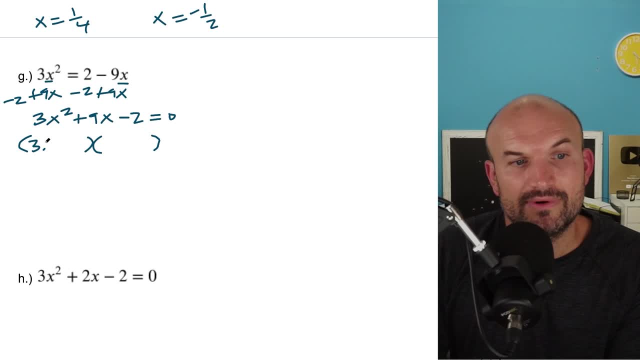 is this factorable, right? What can I multiply here? A three X times an X to equal a zero. So in this case, um, we need to get a negative two. and I'm starting to come into, you know, some problems here, Like, if I do a negative two, negative two times three is a six, Like. 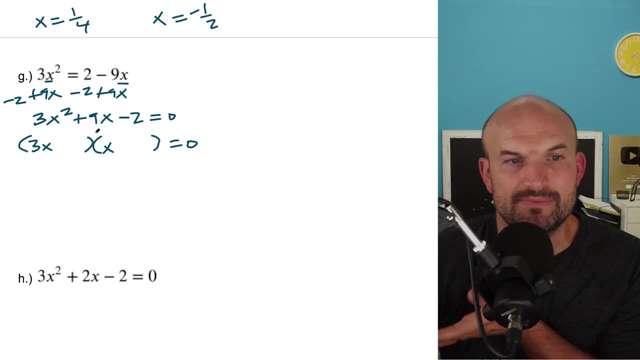 I would have to add that to a three to give me nine. Like I don't see that that is going to be factorable. I don't see there's anything I can multiply here by my factor. I don't see that I can. 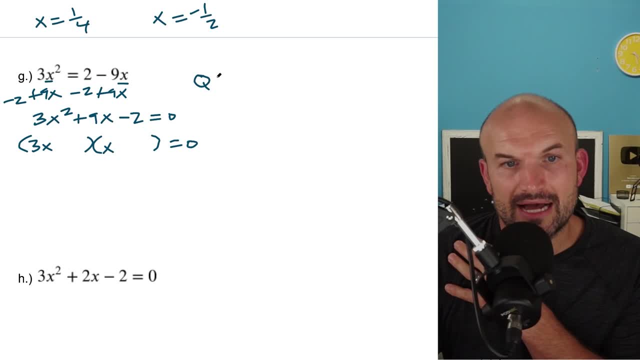 multiply by my factor. I don't see that I can multiply by my factor, So I'm going to add a negative two to get me to a nine X. So therefore, in this problem I'm going to need to apply the quadratic formula. If you remember, the quadratic formula, X equals a opposite of B plus or minus. 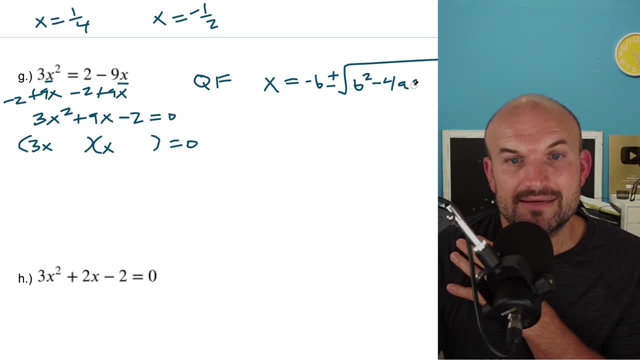 the square root of B squared minus a, four times a times C, all over a two times a. So again, remember that comes from our standard form of a X squared plus B. X plus C is equal to zero. So in this case we could say a equals three, B equals nine and C equals a negative two. So a nice thing. 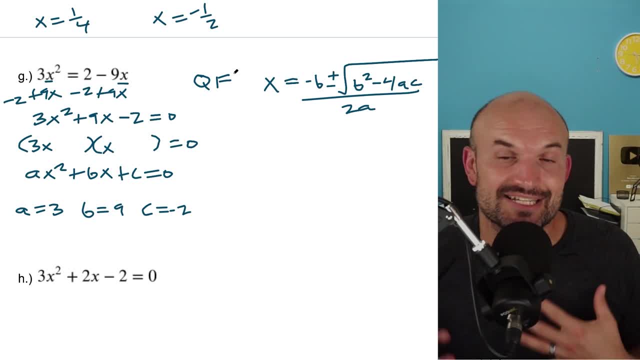 about the quadratic formula. I mean, I still think factoring is going to be their fastest, easiest way for you to be solving quadratics, but you should be able to adjust if something is non-factual which is going to happen. 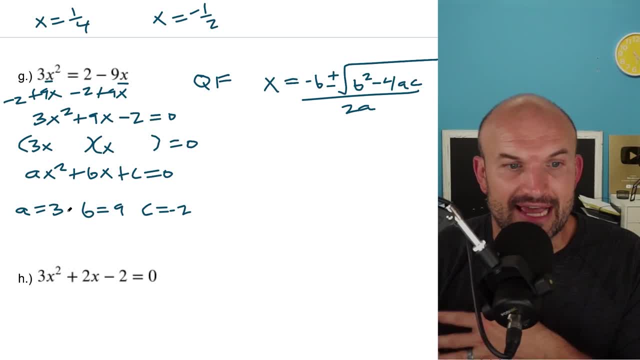 You need to be able to, however, you need to be able to identify these values, A, B and C- and then plug them into this equation. So when you go ahead and do that, that's going to be a negative nine plus or minus a square root of nine squared minus a four times, three times C. 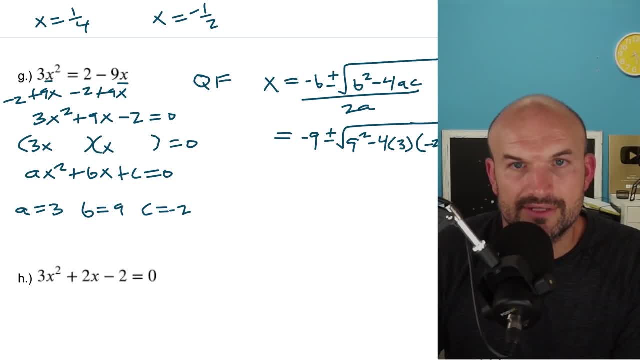 which is a negative. two: Am I running out of room? So yeah, let's go ahead and move that over. Sorry about that, Apologies, No, not the two. We can bring you back over, Okay, And then again, remember, that's going. 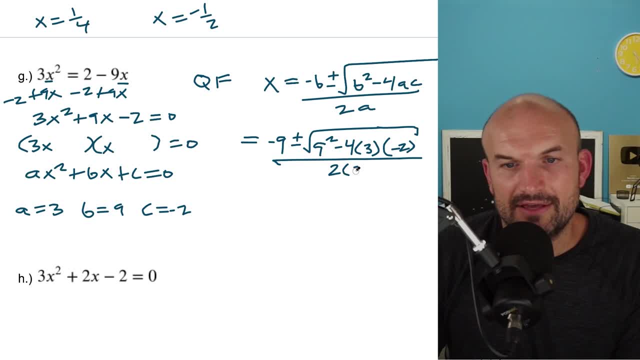 to be all over my two times a, which in this case, is going to be a three. Okay, So now we just need to go ahead and simplify, clean things up, basically. So a nine squared is going to be a 81.. Okay, And then, in this case, I have a three times um, three times negative two, which is a. 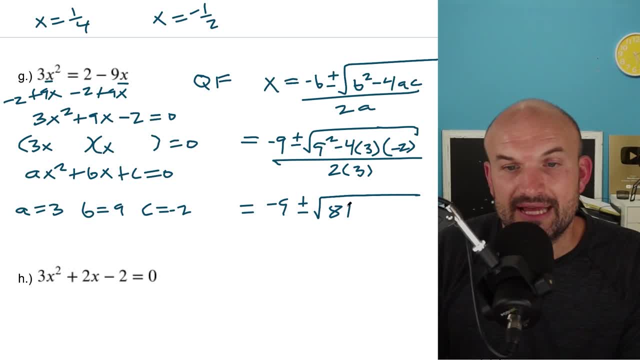 negative six negative six times a negative. four is going to be a positive 24.. And this is going to be all over my two times a, which is a negative six times a negative. four is going to be a six Right. So therefore I can rewrite this as a negative nine plus or minus, now um 81 plus 24 is. 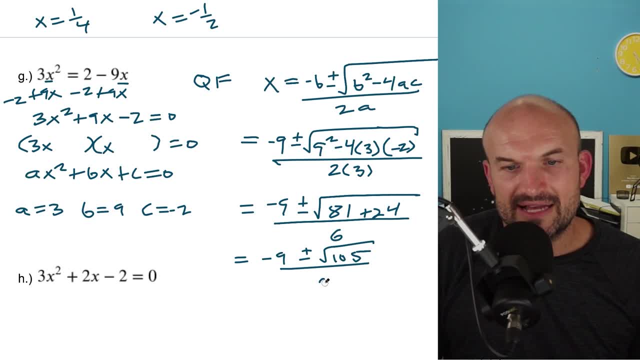 going to be a hundred and five And then that's going to be all over six And I'm not sure if there's anything else I can simplify that square root. I'm just trying to think of Tom numbers in my head, square numbers in my head that would evenly divide in a hundred five, And I'm kind 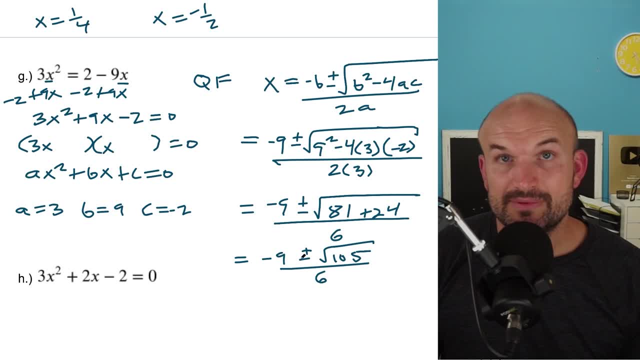 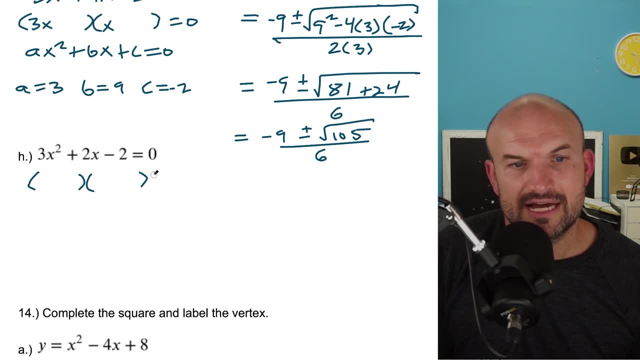 of coming up with a blank at the moment, So I believe that is going to be your simplified version. Now, in this example, we can do exam again the exact same thing. So I'm going to do a like: what two numbers, right? Can we factor this out? Right, Always look to factoring first, So we 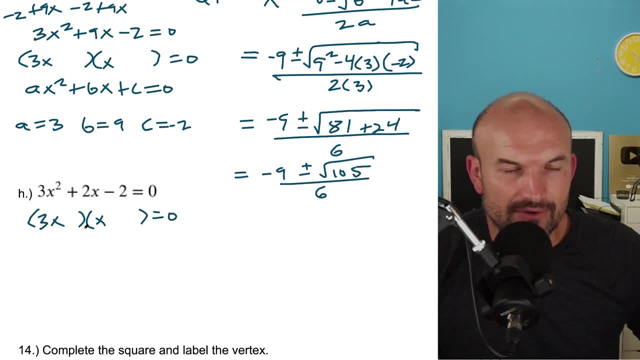 have a three X and an X. We again have that last term to be a negative two, And again we want a difference of two. Um, and you know, no matter what I do, I'm not going to get a difference of. 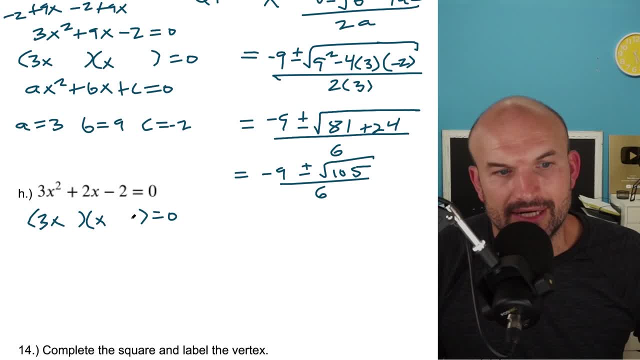 two. multiply this. It doesn't matter if I put a two here, a one here, a one here, a two here. I'm never going to get that difference of two. So therefore, again, I need to use the quadratic formula. So in this case, my a equals three, my B equals two and my C equals negative two. So let's. 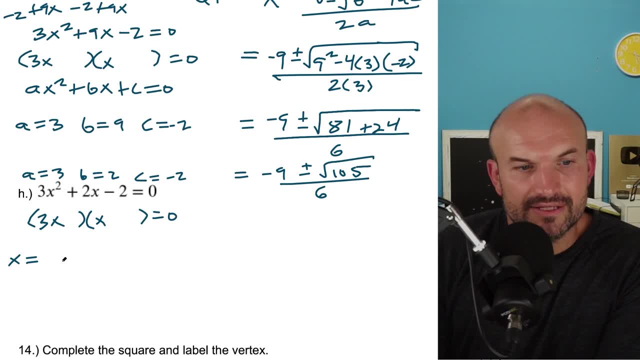 go ahead and try this out. So I have X equals opposite of B, So that's going to be negative two plus or minus a square root of a B squared, So that's going to be two quadrant squared minus a four times B times C, which is negative two all divided by a two times. 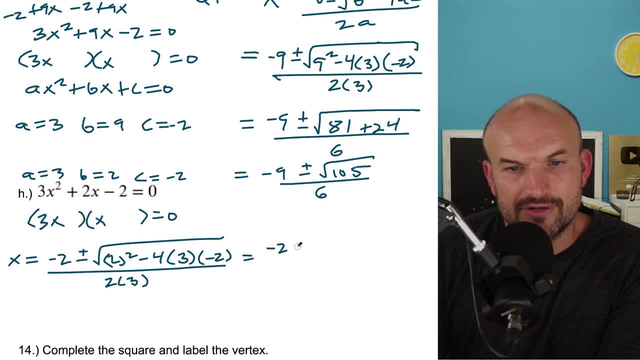 A, which is three. Okay, So what we have here is a negative two plus or minus. Now let's go and clean this up: Two squared is going to be a four. Okay, And again we have the same thing here. 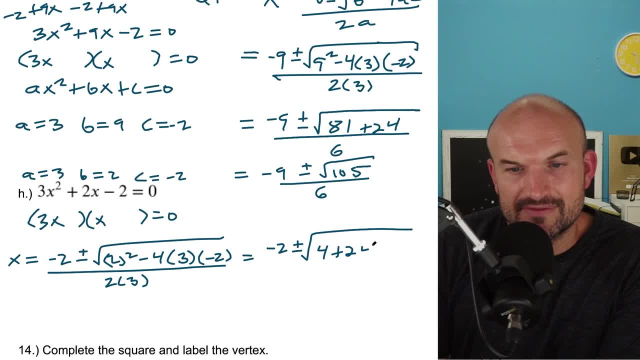 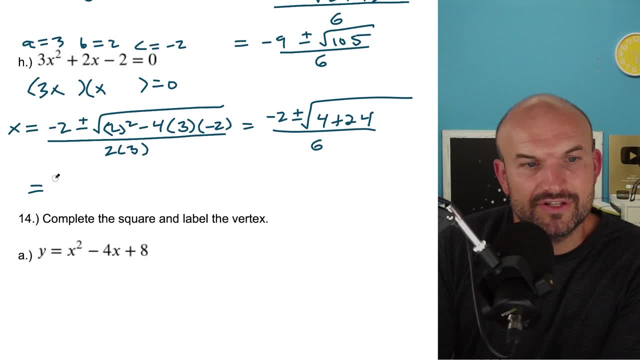 Three times negative. two is going to be a positive 24.. So that's going to be a positive 24.. And that's going to be all over six, All right. So I'm going to kind of bring this back down over here. So let's see, here I have a negative two plus or minus. Now this is going to be a square. 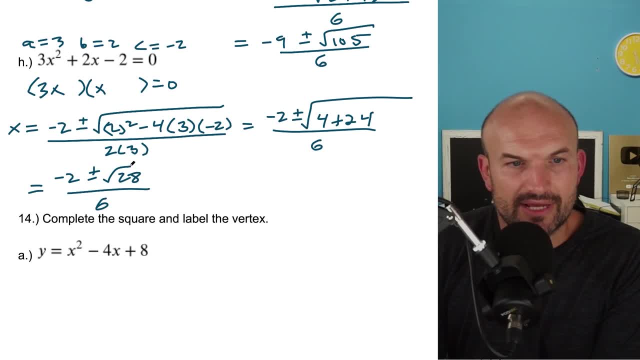 root of 28 all over six. Now square root of 28.. I want to see what square numbers evenly divide into 28.. You can say four, right, Four goes into there. So we have a negative two plus or minus. Let's see. square root of four is going to be two, two or sorry. four times seven is 28,, right So? 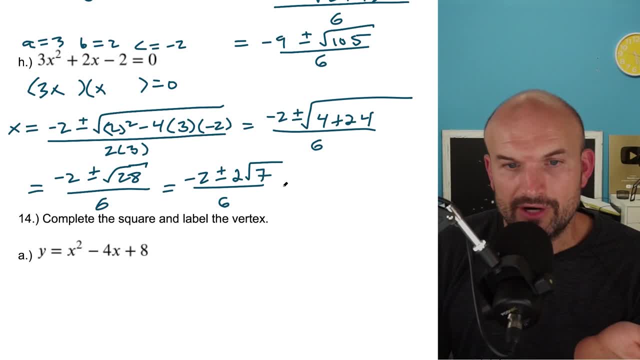 that's going to be over a six. Now, the reason why I had to simplify that? because I'm kind of running out of room, but I can divide a two in the top and all the bottom. So therefore that's going to give me a negative one plus or minus a square root of seven over three. So basically what? 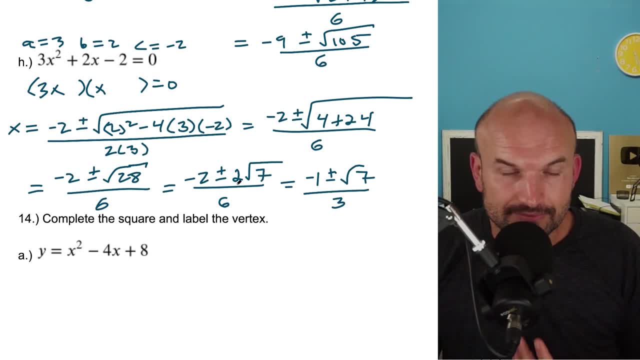 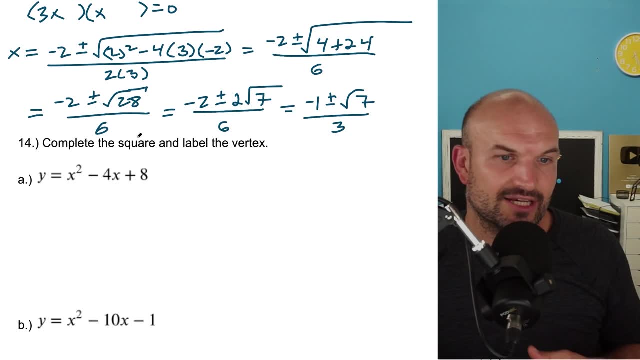 I did. out of all three of these terms, I divided out a two. All right, now let's go and take a look at the completing the square. So the main thing when we complete the square is: this is actually another technique we can use to write an equation from standard form into vertex form. It is a: 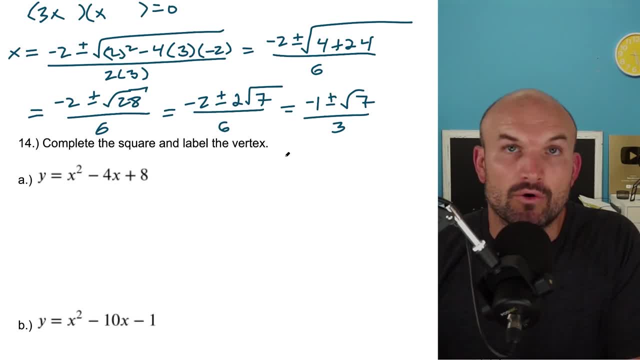 solving technique. I prefer either to look at factoring or go into quadratic formula, but you can also use completing the square for solving. I think it's just. I think it's a good, very helpful for rewriting my equation. I don't really like to use it for solving as much, but the main idea that we're trying to do. 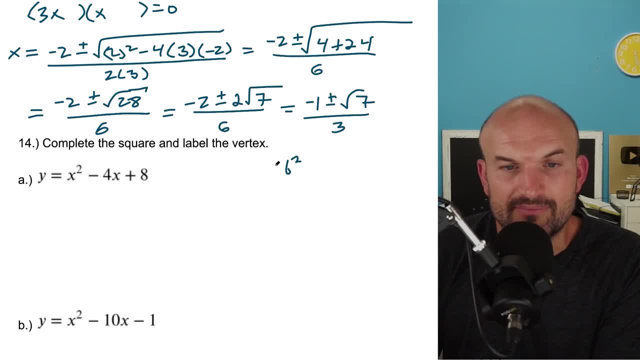 is find the value C. that completes the square. So to find the value C, basically all we're going to do is: C is equal to a, B divided by two quantity square, All right, And our goal here is to create what we call a perfect square trinomial, which can be factored down into a binomial square. 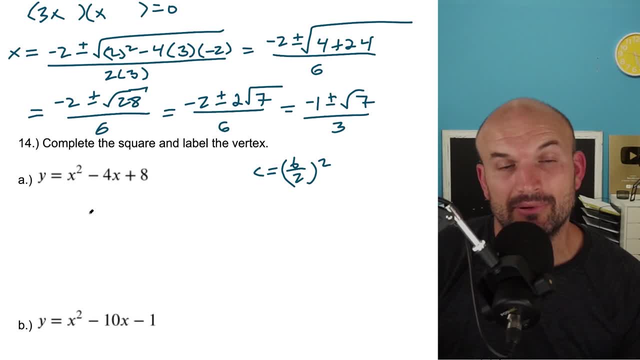 What we want to do is we want to see, if you remember when we were factoring, I think the second example I did in the factoring was I found a perfect square trinomial And what that means is that could be factored down into a binomial squared. Now, this is not a perfect square trinomial. 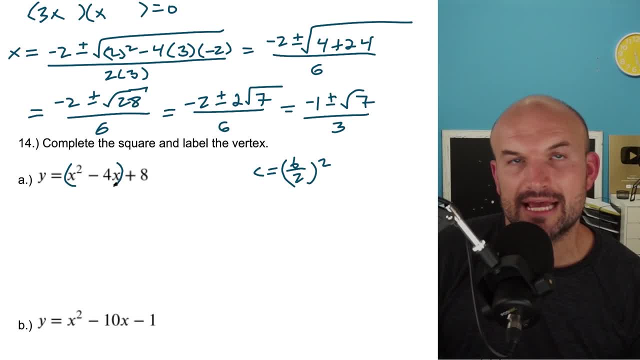 because eight is not a square number. So what I'm going to do is I'm going to create a perfect square trinomial and we need to label the vertex. Okay, So I remember labeling the vertex: Y equals A times X minus H, quantity squared plus K. right, So I remember the vertex is your H comma K. 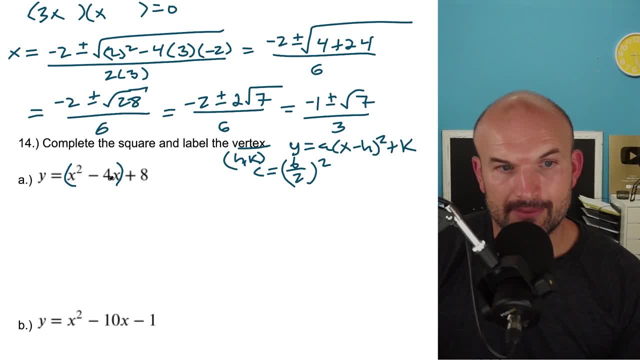 Okay, Important to remember that. All right. So what I'm gonna do is, inside, I'm going to create a perfect square, trinomial. So what I'm going to do is I'm going to find the value C that completes the square. So what I'm going to do is I'm going to take my B. 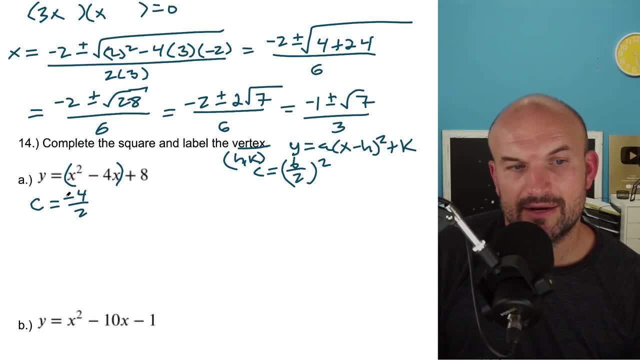 which in this case is negative four. So take a negative four divided by two squared. So negative four divided by two is a negative two. Negative two squared is going to equal positive four. I'm going to take this number and add it inside my parentheses. Now remember whatever you. 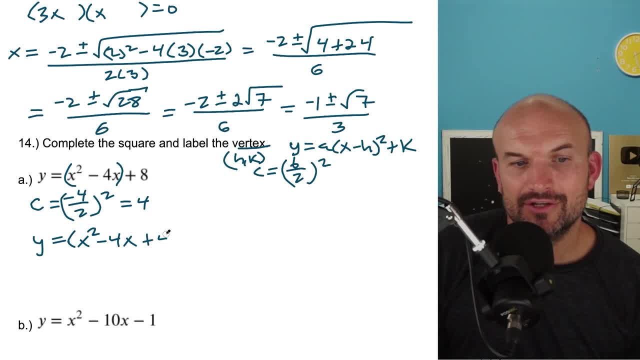 add inside your parentheses, on one side of the equation. you have to either add it to the other side of the equation or subtract it on the same side. So if I add four, I'm just going to subtract it for outside the parentheses and that's plus eight. So now what I'm going to have. 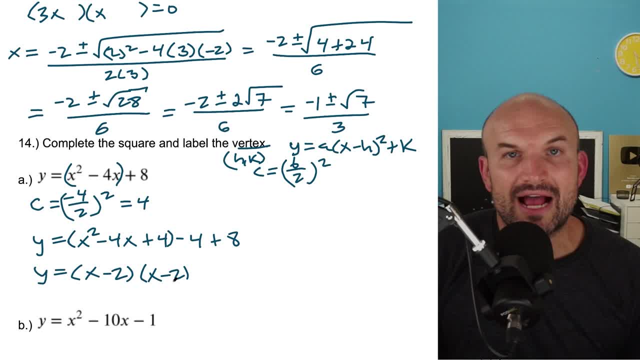 here is a X minus two times an X minus two, right, If you practice your factoring right, This is what you do whenever, every single time you create, do the perfect square trinomial. you always create a perfect square trinomial. So when I have an X minus two times an X minus two, that's going to 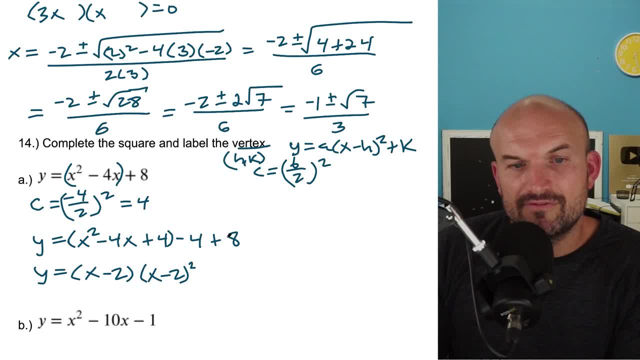 give me an X minus two, quantity squared Okay. And then negative four plus eight is just going to give me a positive four. I don't know why I wrote an equals, but that's supposed to be a plus four, So I'm just going to go ahead and do that. So I'm going to do that. So I'm going to do that, So I'm. 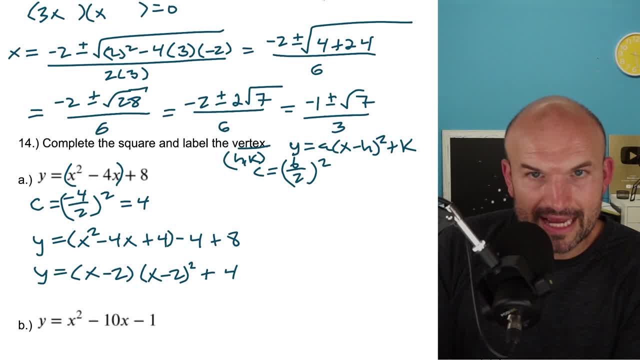 going to go ahead and write a plus four in this case, and that's not supposed to be there. But again, you what you can see here is: this is going to be an X minus two times X minus two, which is going to leave me now with an X minus two, quantity squared plus four. And if you remember the vertex, 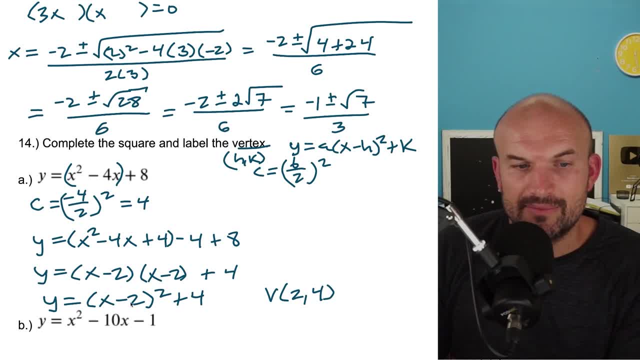 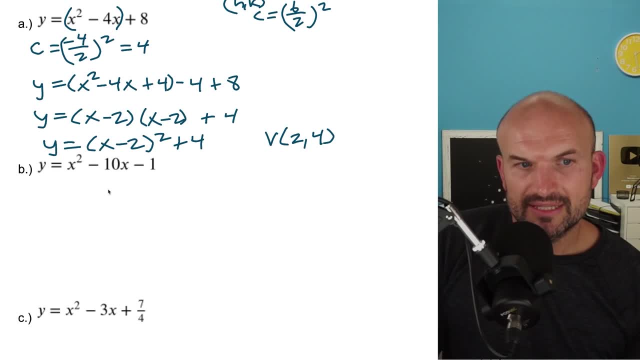 here in this case is going to be now a two comma, four, right, Because it's X minus H, right. So therefore the minus two. they actually shifted it to the right two In this example we're just going to. you know, it's just basically again practicing the completing the square, Completing. 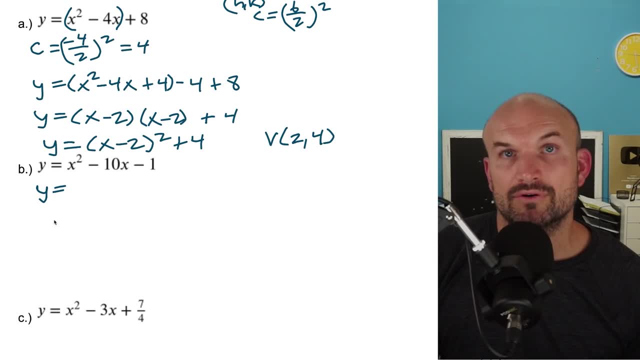 the square does come up. So it is very, very easy to do that. So I'm going to go ahead and do that. It's very important that you can, you know, practice this and feel comfortable with this process. In this case, I'm just going to go ahead and, you know, group these first two terms And 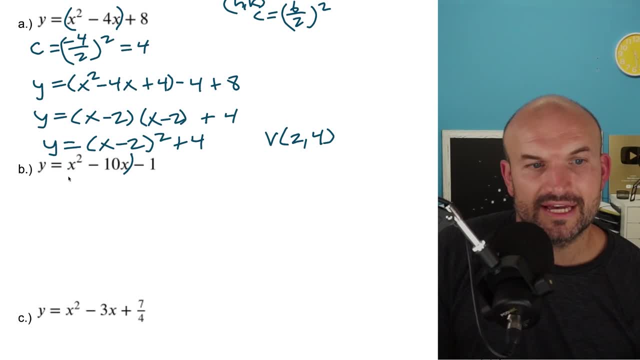 actually, let's just figure out what my B is in this case. So my B in this case is going to be a negative 10.. So I could say: C equals a negative 10 divided by two. quantity squared. Negative 10 divided by two is a negative five. Negative five squared is going to equal a 25.. Okay, So I'm going. 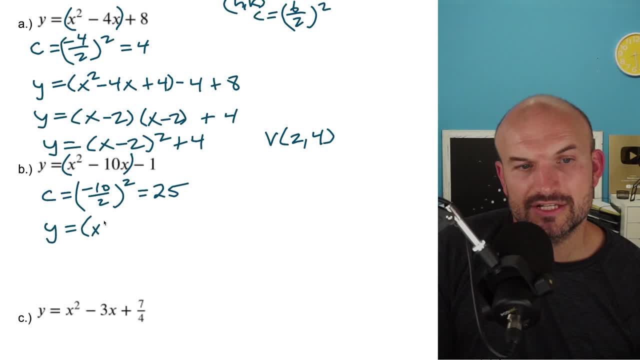 to add that and subtract it. So I have a Y equals a X squared minus a 10, X plus a 25, minus a 25, and then minus one. Okay, Now, here again, this is a perfect square trinomial. What two numbers multiply to give me five, add to give me negative five, And again. 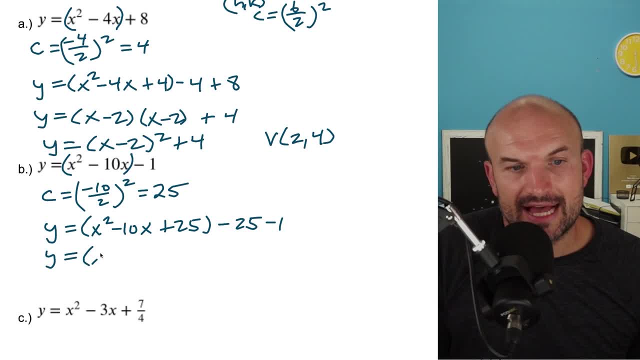 they're going to be exactly the same. In this case that's going to be: Y equals a X minus a five quantity squared minus a 26.. And now we can say: my vertex here is going to be a positive five comma a 26.. Now it's like simple. A lot of students will get confused here because they'll 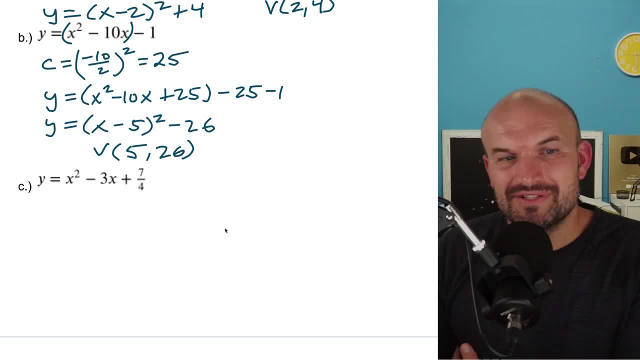 be like: Oh, fraction. I don't want to do fractions Like that, looks confusing, Right. But again, just follow the steps. right? We want to group our first two terms. Okay, Group the first two terms and then find the value C that completes the square. So C, in this case is a negative three. 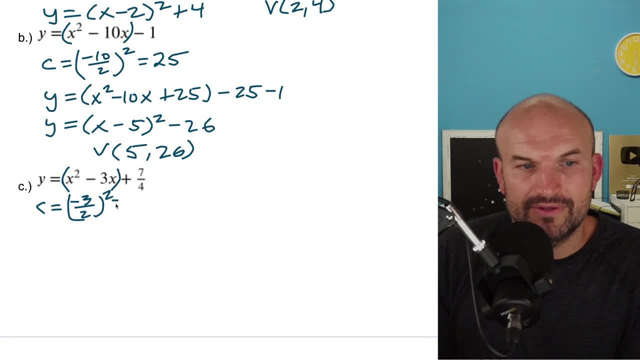 divided by two, quantity squared right. Well, negative three divided by two- or can't divide that out, but you can square it, which is going to be a nine force. Okay, So I have Y equals a X. now that looks kind of confusing: minus a nine force and then plus a seven force. Well the good. 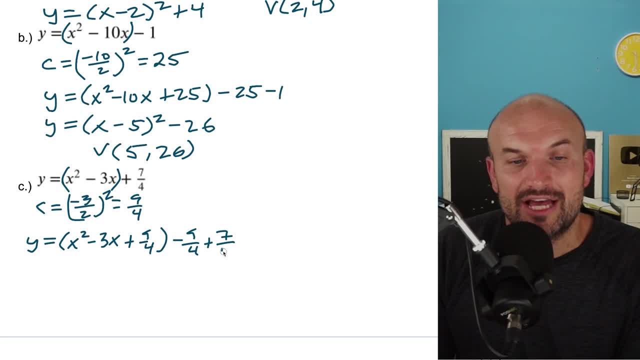 thing here is- at least I added it with another fraction. That fraction is actually helping us out, because now I can combine those rather easily. However, how do you factor this out? So the one thing I want you to kind of understand here is when, when you have a perfect square. 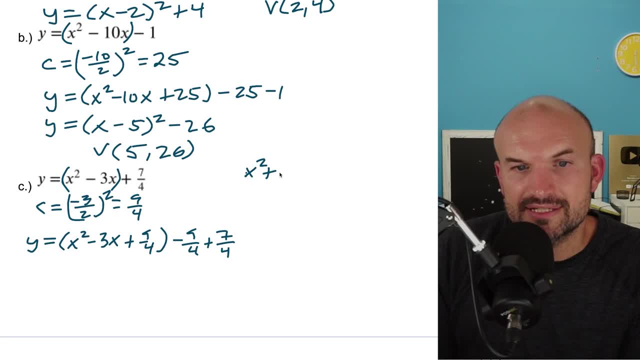 trinomial, um, when you have it at like a- X squared plus um a, two B, X plus X squared, Okay, When I want to try and find my X, uh, actually, I don't, really, I want to go far that way. Um, the best thing I hear I can explain to you this way, The best. 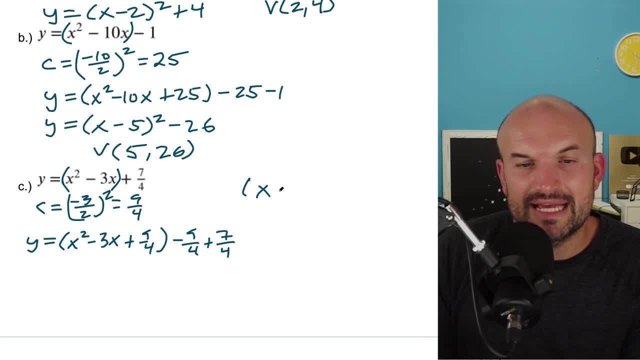 way, if you want to know what this binomial squared is going to be, it's going to be X plus or minus, a B divided by two squared. Okay, Now again, the plus or minus just means: is your middle term going to be negative or is your middle term positive? Actually, I chose all negative. 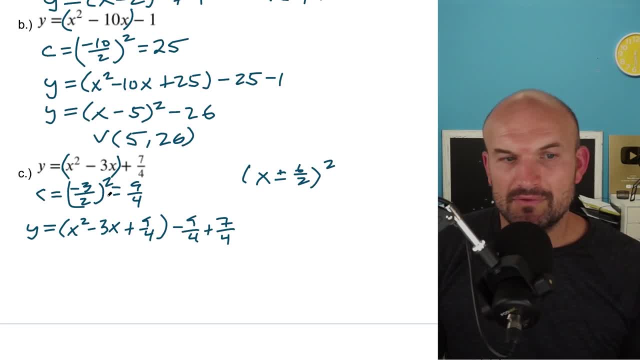 examples. So our middle term has always given me negative. So what was my B divided by two? My B divided by two is a negative three halves. So therefore, since my middle term is negative, I want to use this Negative solution So I can rewrite this as a X minus a three halves times an X minus a three. 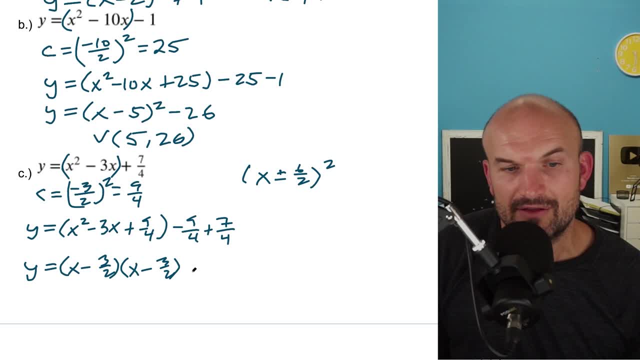 halves. Now again, you could write it back in the square term, right, But I want to show it to you how this works. And then this is going to be a negative two fourths. Oops, I'm sorry, We already have that as a negative, right, So it's gonna be minus a two fourths, Okay. So here's what I want. 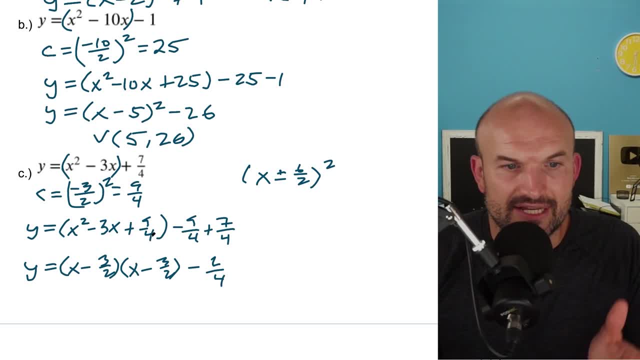 you to be able to do and see how this works. Negative three halves times negative three halves is a positive nine fourths right. Negative three halves plus negative three halves is a negative six halves, which is a negative Three. So you can see how this works. So, therefore, this is gonna be X minus three halves quantity. 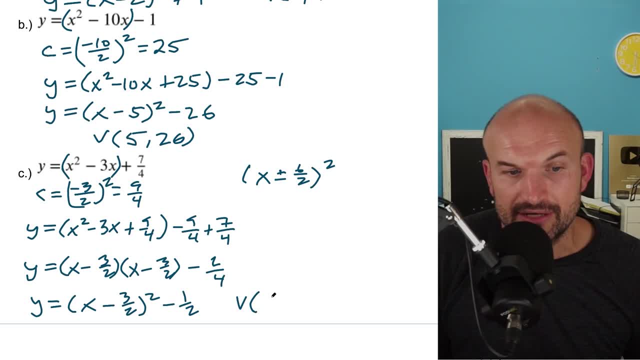 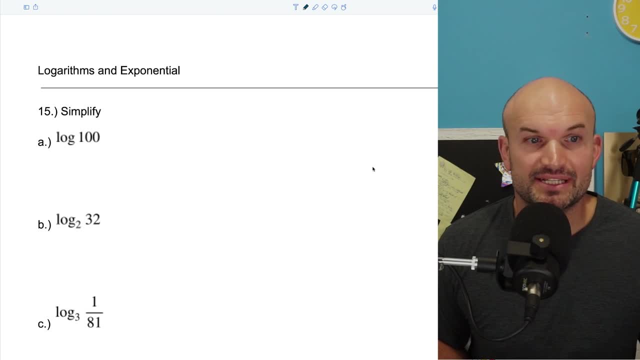 squared minus a one half. So the vertex in this case is a fraction, right, But it's gonna be a positive three halves and then minus a one half. Okay, So moving on to the next section, we're going to be dealing with logarithms and exponential functions, So just a couple of things to remember. 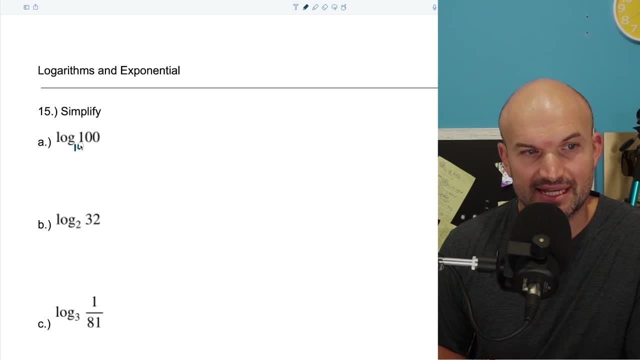 Remember, whenever we have a logarithm, you know, and there's no base here, that's going to be base 10.. And the main thing we need to understand when we have a logarithm like that, we're trying to evaluate this right, We want to find the value of this logarithm. 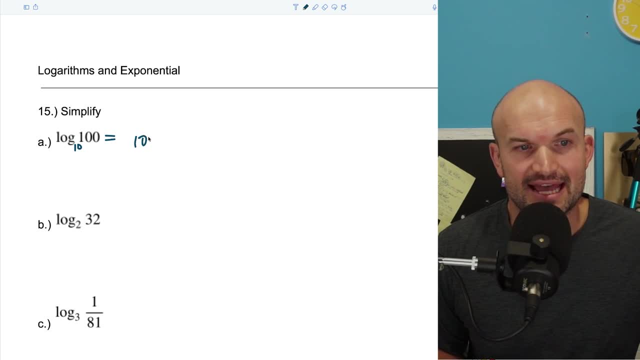 So what this is basically asking is you want to say: take the base. It's saying 10 raised to what number is going to equal this argument, which in this case is going to be a hundred. So hopefully you understand here that with just a little bit of simple math we can represent that that is going. 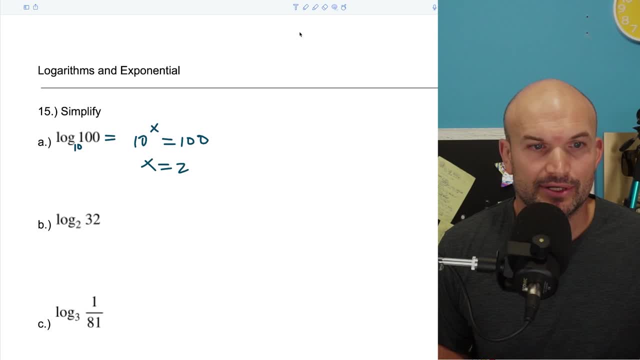 to equal. So therefore we can say X is going to equal a two. So what I'm going to do is actually move this over here, but that is basically what we're asking. When we're looking at the logarithm, you can kind of sometimes think of a logarithm as in its exponential form. So when I say log, 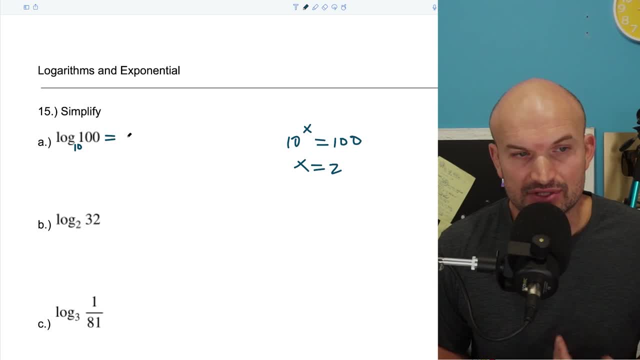 base 10 of a hundred. like what am I asking? Well, I'm saying: 10 raised to what number equals a hundred. So you can see that it is two. In this case. we're saying: two raised to what number equals a 32.. Well, hopefully you recognize. 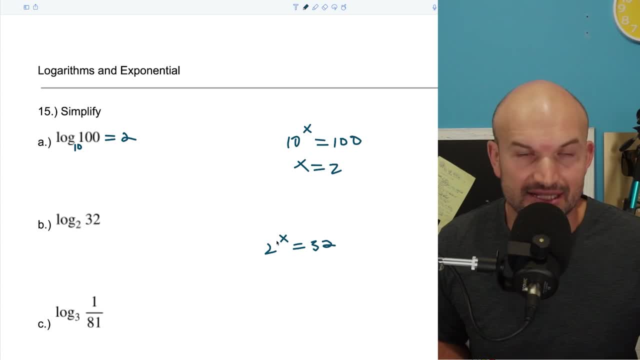 that two raised to the second, power is four, two. third power is eight. fourth power is 16.. So the fifth power is actually going to be a 32.. Okay, Now, some of these you should hopefully you know, as you kind of remember going back through there in your head once we get into problems like with 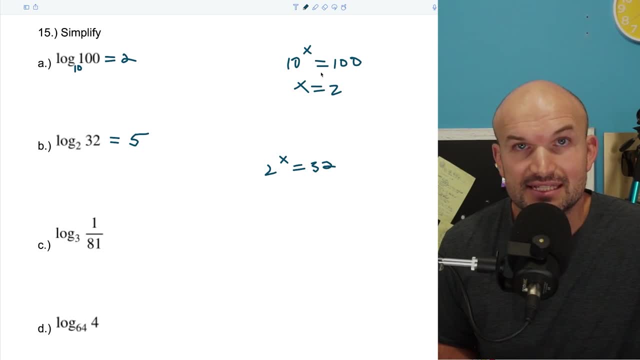 fractions. that's a lot of times where things can kind of get confusing. That's why I like setting it up in the exponential form. So here I can say: three to the X right Is equal to one over an 81. But in this case we're saying two raised to what number equals a 32.. So what number equals a 32?? 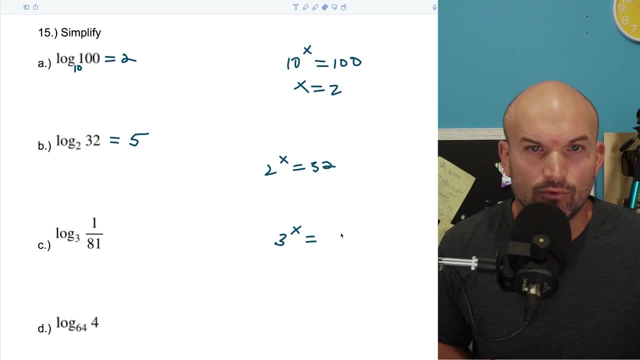 In this case. we don't want to write it as a fraction. What we're going to want to do here is rewrite 81 as a with a negative exponent. right, I can rewrite this as 81 raised to the negative first power. Now what I want to be able to do is also be able to say: well, three raised to what? 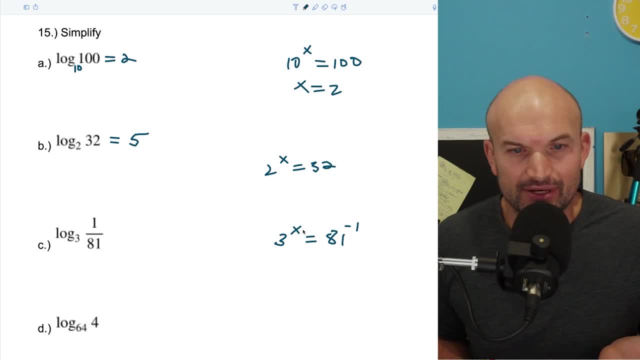 number equals 81, right? Because you know if I'm trying to say three raised to what number, like I got to be able to see what, what that's going to be- to 81. And that might not be apparent to you. 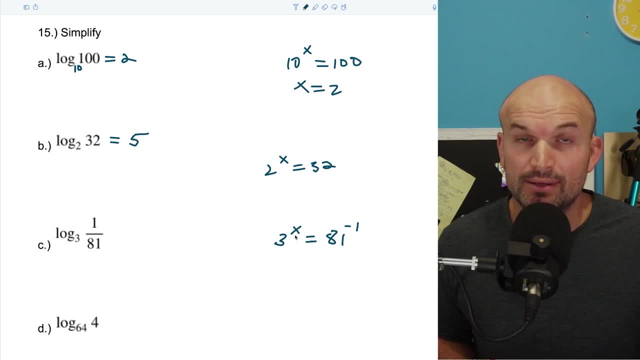 So one thing we can kind of recognize here is using what we call the one-to-one property, right? So the one-to-one property basically states: is: if I have, like you know, um, a to the X is equal to a to the Y, then X is going to equal Y. 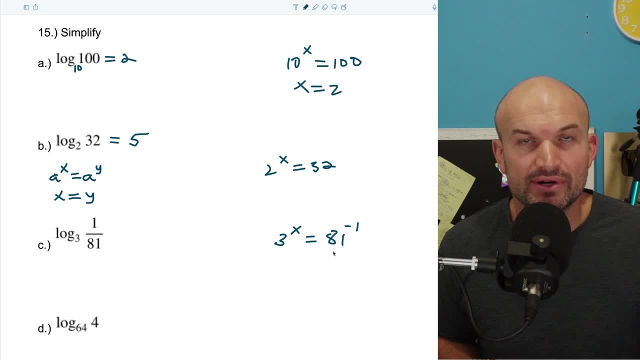 All right. So we want to get these to be the same base. So three raised to what number equals an 81. Well, guess what? That is going to be a four. So I can say three to the fourth. power is the same. 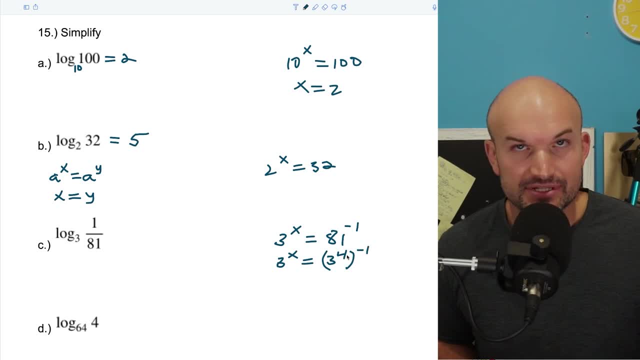 thing as 81. And that's raised to the negative first power. Now, using my, now using the product rule of exponents, negative one times four is going to be a negative four. So therefore, X is equal to a negative four. So when I want to say three, raised to what number equals an 81,. 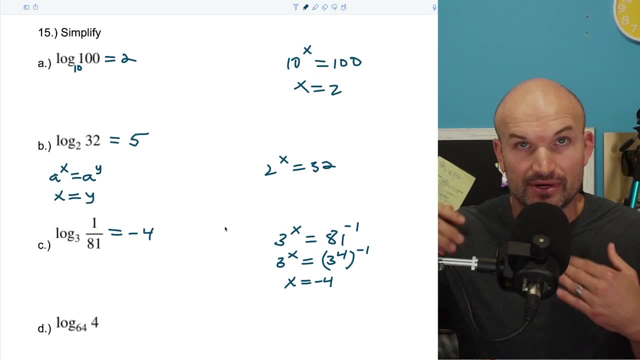 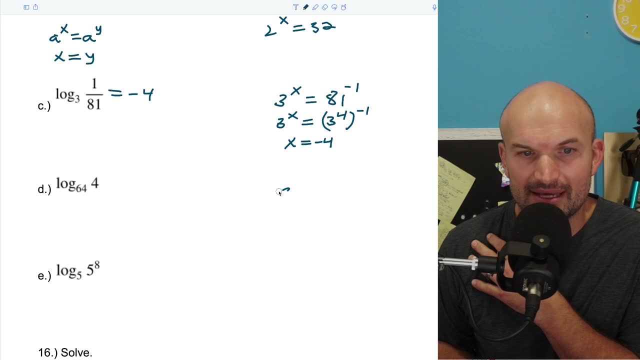 that's just going to equal a negative four. Okay, Cause, again, that makes sense Like three raised to the negative first power. You're going to put that in as a reciprocal and it kind of works. on the second example: same kind of thing, same kind of idea. What we're going to want to do is 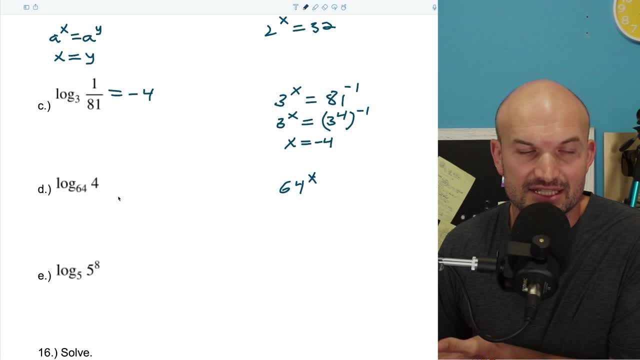 make sure we write these with the same base. So cause- again this one makes sense- why we're using a fraction or at least a negative number, because when I hit 64, raised to what number equals four. well, how do you have something that's being raised to a power and it's going to go smaller? 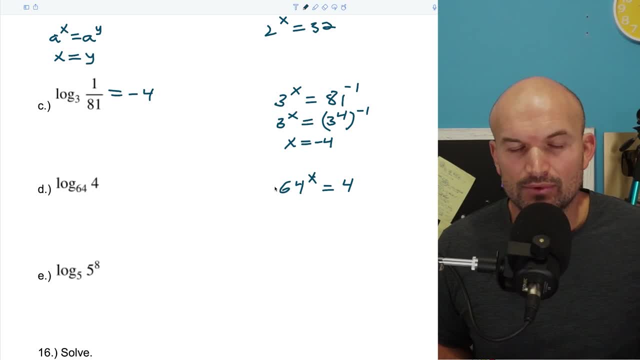 in value. That's where negative powers come into play. So, again, what we're simply want to do here is we want to go ahead and say: all right, well, six or four, I'm sorry, raised to what number equals a? you know X. well, four squared is going to be 16.. And if we multiply that four, one more. 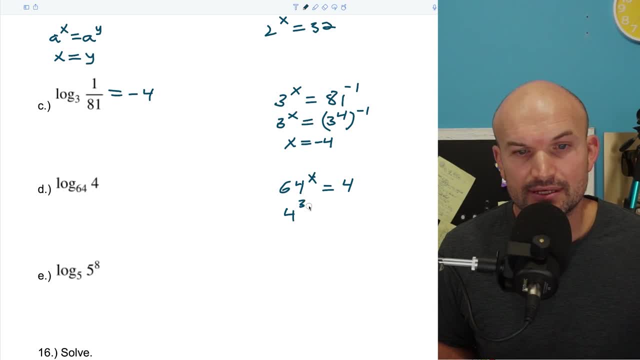 time that's going to be 64.. So there I can say: four cubed right Is equal to a four. Now I can basically say: well, that's really a power to the one. first power, actually not fraction, It's not a 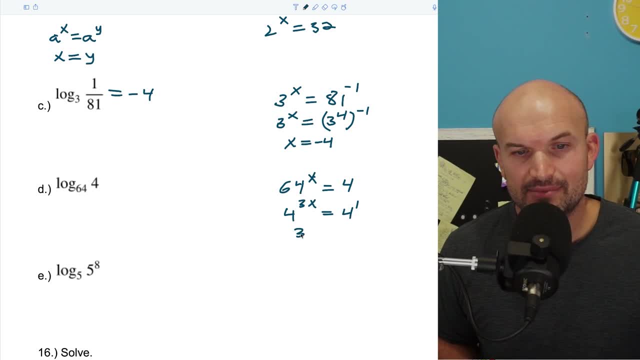 sorry, not a negative number, It's going to be fractions, right? Because now I can say that's going to be a three: X is equal to one and divide by three on both sides, And X is equal to a one. therefore, in this case, I can say that this answer is going to equal a one third, which, again, 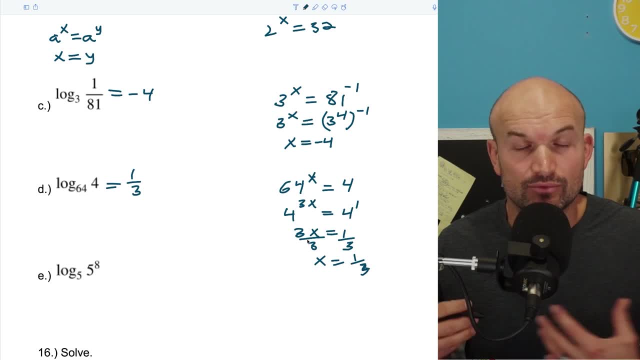 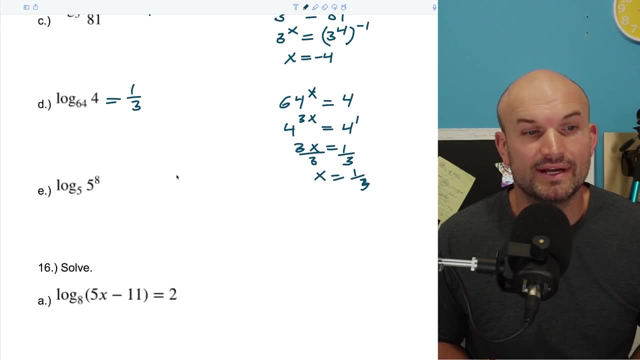 is kind of like taking the cube root right And because, remember, we can write it, rewrite a rational power as a radical, And so therefore, the cube root of 64 is indeed a four. Okay, Now, in this example, we're just basically just going to use the rules of logarithm. So, whenever you have 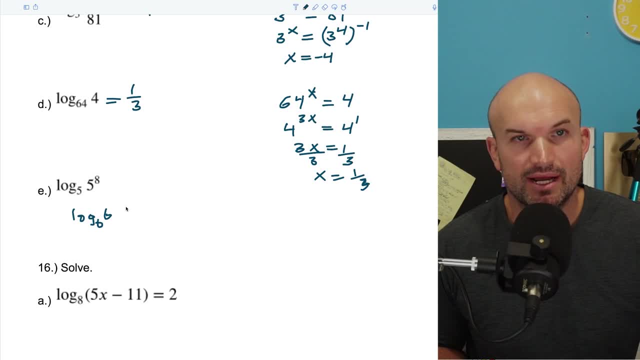 a logarithm with the same base as its argument, right then that's just going to equal one. But if you have a logarithm with the same base and its argument raised to a power, then that's just going to equal the power, And there's a couple of different. 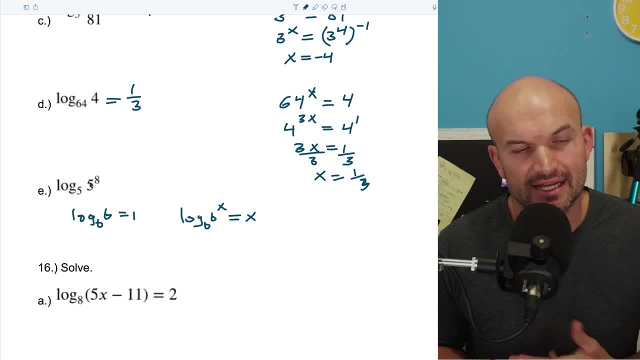 ways we can verify that. We'll, you know, kind of explore again inside, you know, through working through in the chapter of chapter on logarithms. But in this case, basically, you're going to see that, using these rules, my answer is going to be the power, which, in this case, is going to be an 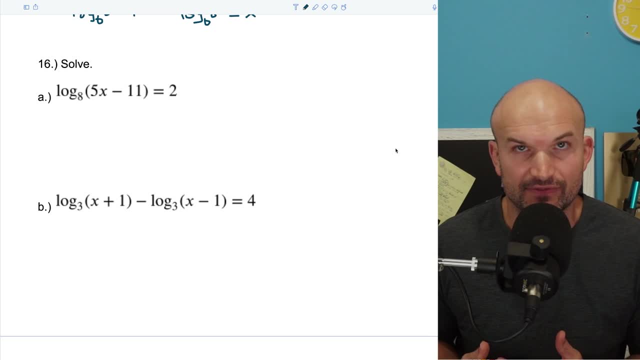 eight. Now for solving logarithmic equations. there's a couple of different things we want to do. The first thing we want to do is always make sure we that we have a logarithm kind of isolated. In this case, you can see, I have a logarithm equal to a value. Now to undo a logarithm. 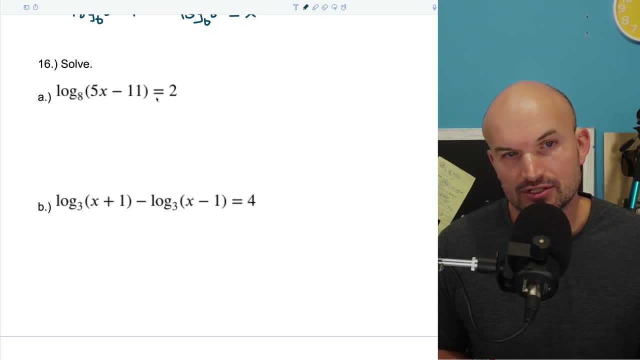 I need to use my inverse operations, right? So how do we undo a logarithm? So one way we could do it is rewrite this in exponential form, but the undo, the logarithm, is what would be to be able to exponentiate on both sides. So what I'm going to do is I'm 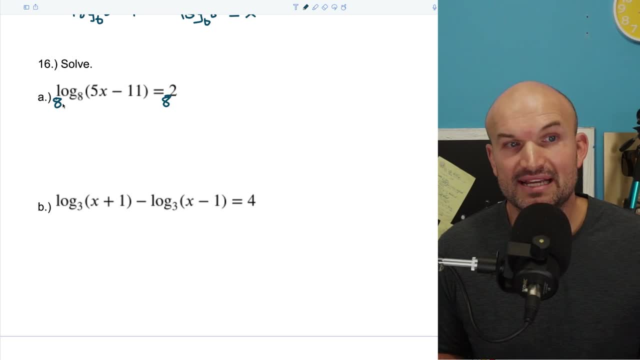 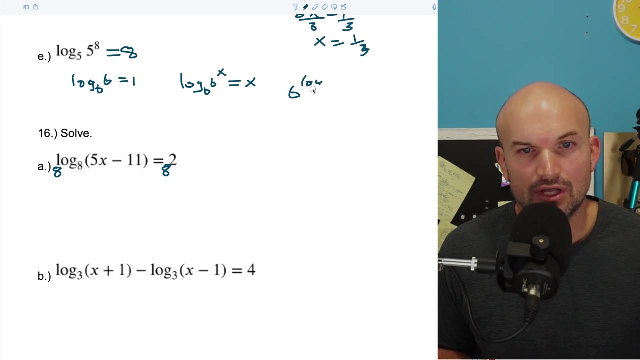 basically going to base, have these be the powers with a base eight. So just like I did here, log base B of B raised to the X. the same thing works over here. If I have B raised to a log base B of X, that is also just going to equal an X right. So when I have an exponent with the base, 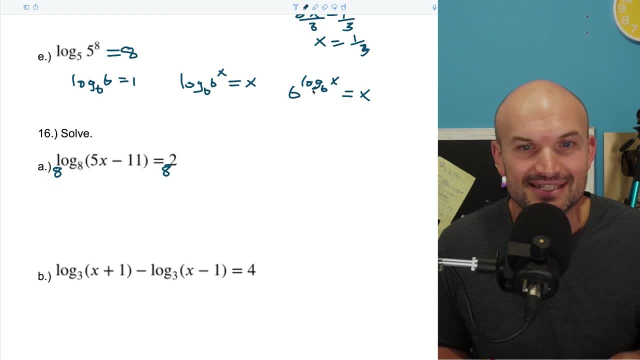 raised to the logarithm of that same base, of what the base of the exponent is. then it's just going of the logarithm, So by exponent exponentiating on both sides. now what I'm going to go ahead and get is a five X minus 11 is equal to an eight squared, which is going to be a 64.. Now I can. 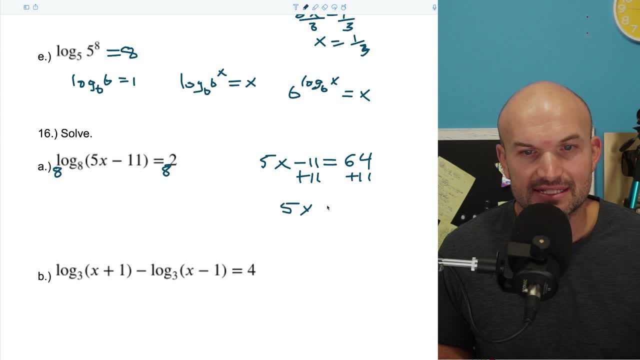 just go ahead and add an 11 on both sides and I get a five. X is going to equal to a 75, right? And so now I can just say: how many times does five go into 75.? So I can divide by five on both sides. 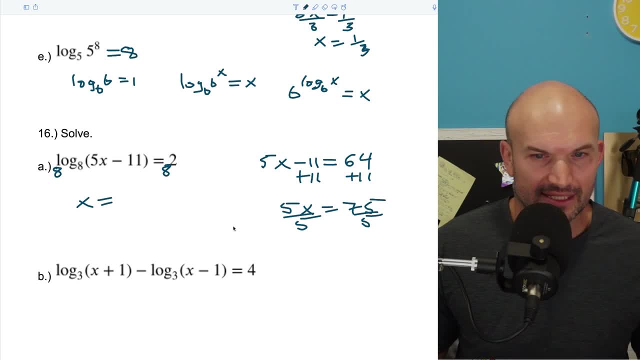 And in this case I'm going to get an. X is going to equal a. let's see that's going to be into a 50.. That's going to be 10 times, So that'd be a 15.. Okay, Now the other thing. that's really. 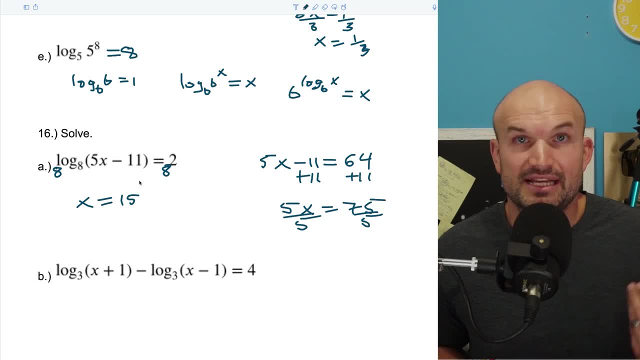 important when we're dissolving logarithm equations is just to plug it in, like to make sure that it is going to make sense. So you know, if I plug this in, we want to make sure that it's still going to give us a value that would not be negative, because sometimes we will get extraneous. 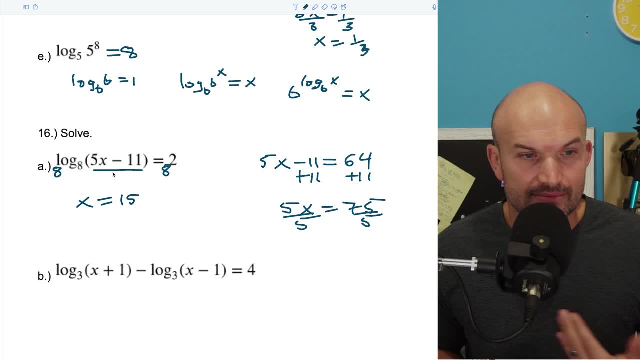 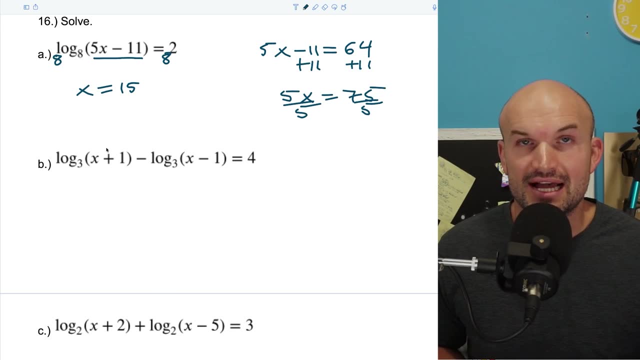 solutions on logarithms. So you know you can just go ahead and plug it in to make sure it's going to be verified. Now, in this example, I can't simplify my log or I can't like exponentiate on both sides until I have exactly one single logarithm. So I'm going to go ahead and plug it. 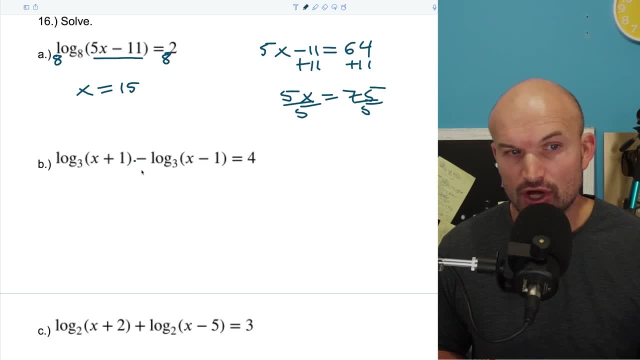 in. So what I'm going to need to do in this case is actually use my rules of logarithms to condense this. So you remember, when you have the difference of two logarithms, as long as they have the same base, you can go ahead and rewrite that as the quotient. So I can rewrite this as a log base. 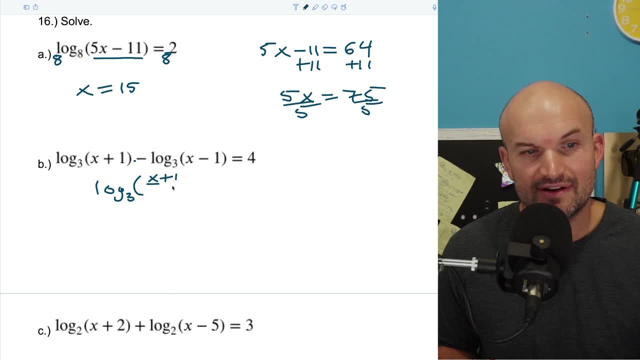 three of a X plus one divided by an X minus one. Okay, And that's going to now equal four. Now you can see I can go ahead and exponentiate on both sides to kind of get rid of my logarithm. So therefore I'll raise it to the base three, And again the reason why I want to choose the base. 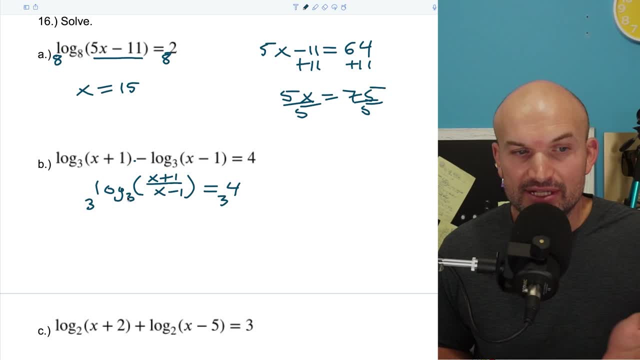 three is because that's going to get rid of that logarithm. Right, Because the logarithm is raised to, it has a base of three, Hence why I did the logarithm over here with a base eight, And so therefore now I'll just have a X plus one divided by an X minus. 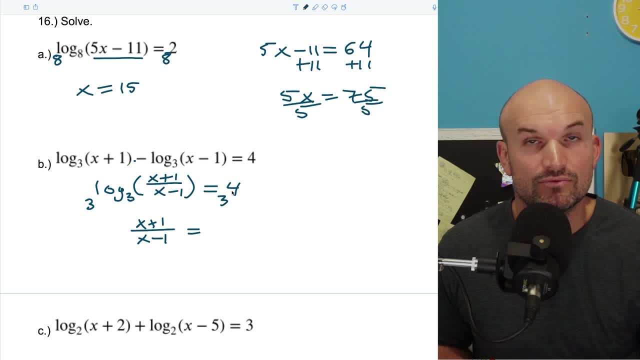 one, And therefore this is going to be a three raised to the fourth power. If you remember, that was going to be a 81, right? So that's going to be equal to 81.. Now I need to solve for X. I have. 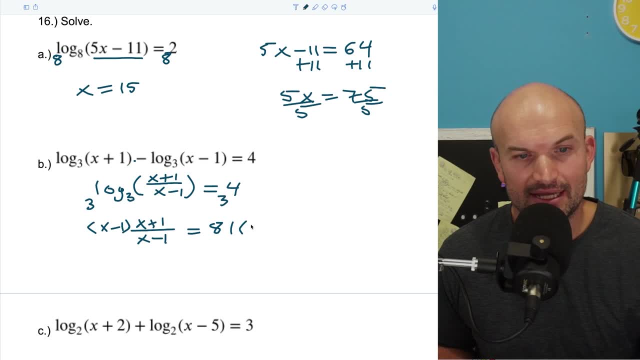 two X's right. So I need to get the X off the denominator. So I'm going to multiply by X minus one here on both sides And let's see what's that going to leave me with. That's going to leave me with an X plus one. 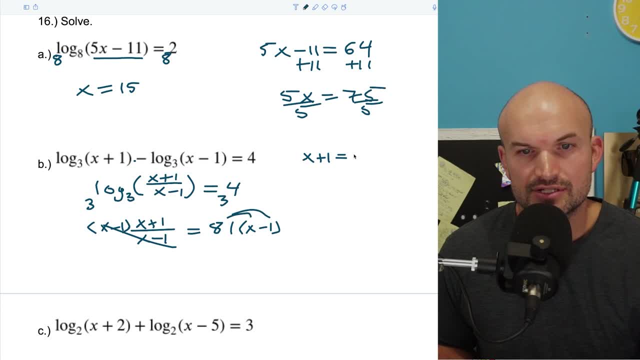 Is it going to equal to? let's go ahead and apply here some distributive property. So this is going to be an 81- X and then minus 81.. Okay, Now, what I'm simply going to do is to go ahead and go ahead and solve. So therefore, I can add an 81 to both sides. I will subtract an X. 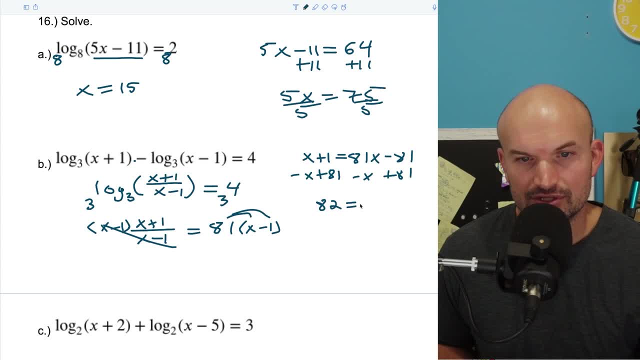 over here And therefore I'm going to get an 82 is equal to an 80 X. Now I can just go ahead and divide by 80 on both sides, And now what I'm going to get is an 81 X. So I'm going to get an 81 X. 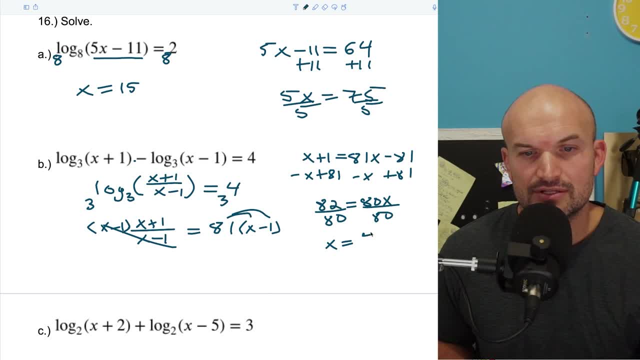 X is going to equal to looks like I can reduce this by two, So that's going to be a 41 over a 40. And again, the main thing is like I want to make sure I can plug that in. It's not going to make. 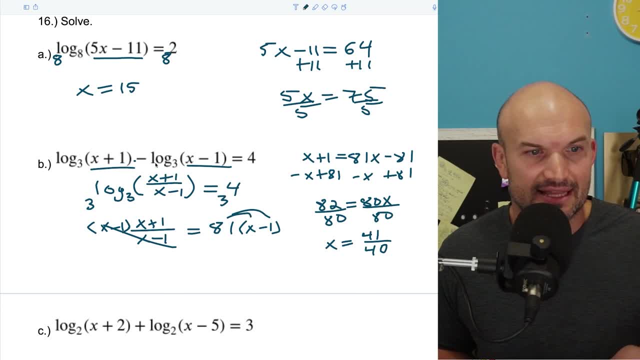 either of my arguments negative And you can see in this case that that is going to work. You could obviously go ahead and check it out to make sure you know, check it out to plug it in using a calculator. But the main thing is I just want to make sure both of my arguments are going to be. 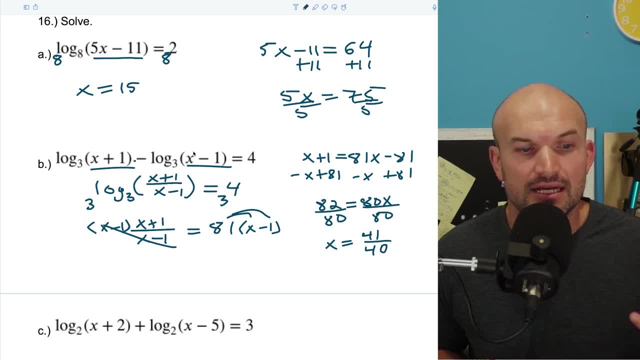 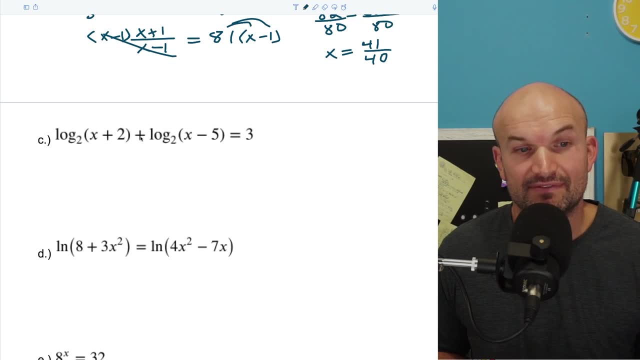 positive. Therefore, I'm not going to have to worry about any extraneous solutions in that case. Um. this example is going to be basically the exact same thing when we have a logarithm, um, when we have the addition of two logarithms. 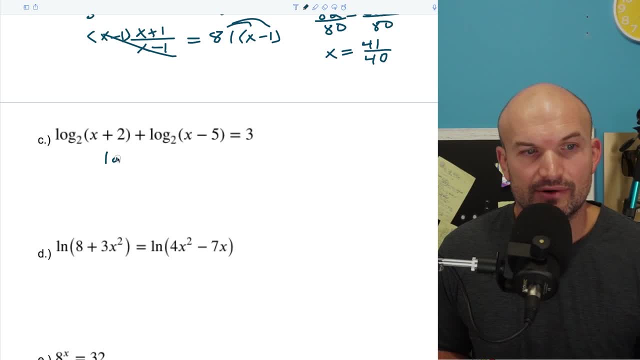 then now what we can do is just go ahead and use that as a product, So I can rewrite this as a log base two of an X plus two times a X minus five equals three, right, So now I can go ahead and exponentiate on both sides. So I'll read these to base two and then I can multiply the binomials. 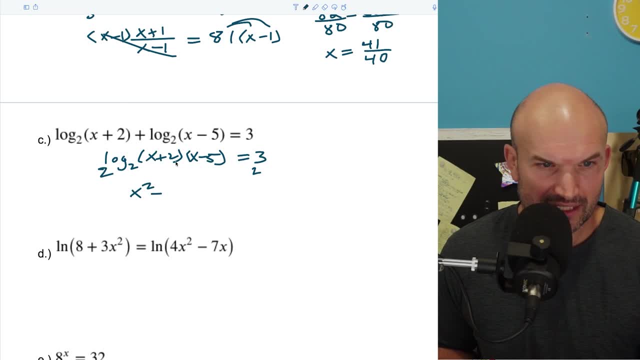 X plus two times X minus five. So that's going to be an X squared, And let's see that's going to be a two. So that'd be minus a three. X minus 10 is going to equal a eight. Um, that is not an eight. Yeah, it's an eight. Um, then let's go ahead and subtract that over. 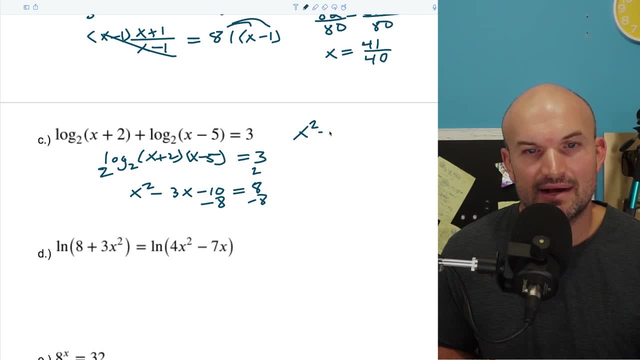 here. So now I have a. let's see a X squared minus a three. X minus 18 is equal to zero. Okay, So now I want to be able to. I need to go ahead and factor this: uh, what two numbers multiplied to. 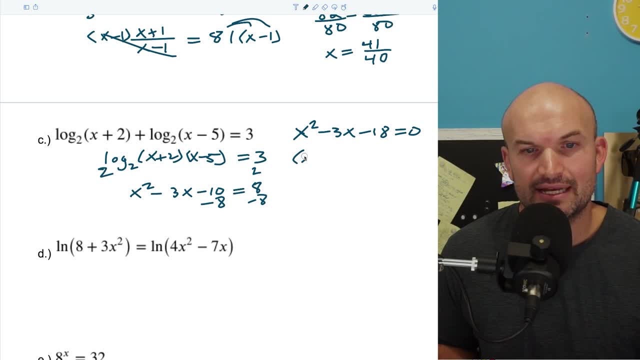 give me negative 18 and give me a negative three, And that's going to be an X minus six times a X plus three is going to equal zero. Okay, And now I can use a zero product property. So by setting them both equal to zero, right? So X plus three is going to equal zero. Okay, And now I can use a. 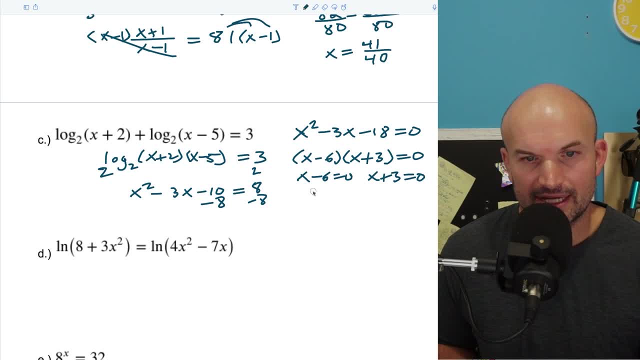 plus three is equal to zero. Just want to make sure, And therefore I get: X equals six and X is equal to a negative three. Okay, Um, now, one thing I one thing that's really important here is: we want to make sure that none of these are going to make us have extraneous solutions, right, So I can? 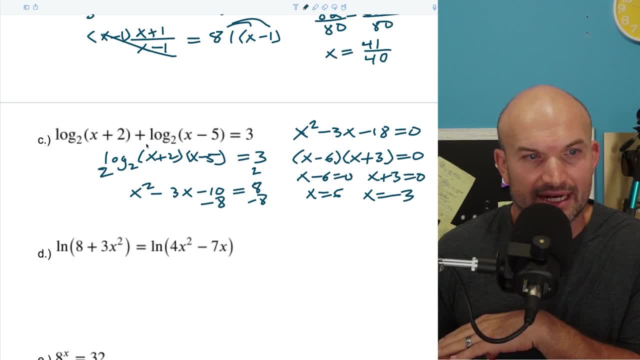 plug in the six to both of those. Um, that's going to work. And if I plug in a negative three, though, notice, when I plug in negative three- negative three minus five is a negative eight. two raised to what number equals a negative eight. That's, that doesn't exist. So this is going to be. 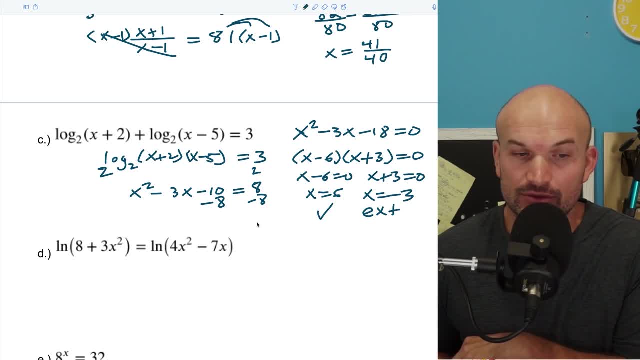 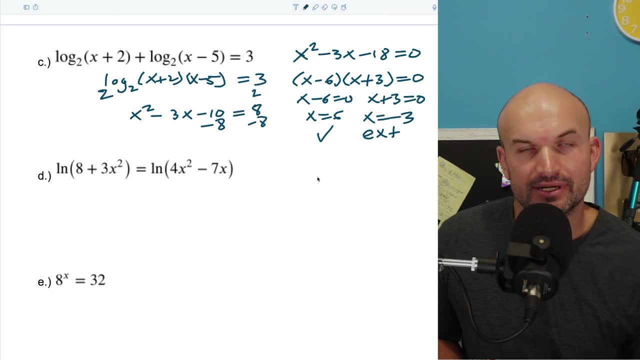 an extraneous solution. So my only answer is going to be: X equals negative. three is an extraneous solution. Um, so do you remember that one? do you remember that one-to-one property that we talked about for exponential equations, Like if I? 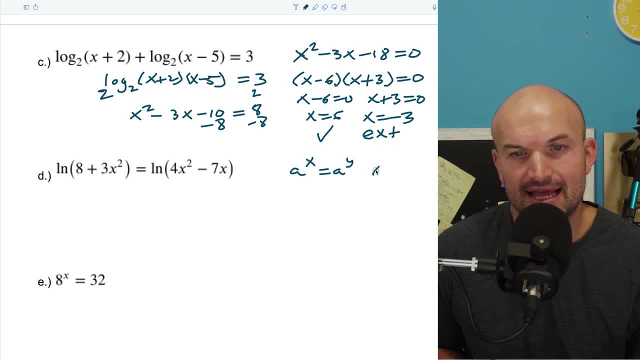 have a to the X is equal to a to the Y, then X is equal to Y, right? That's the one-to-one property. that works for exponential equations. That also works for logarithm equations. So if I have a logarithm equal to a logarithm with the same base, in this case they have the same base, which is: 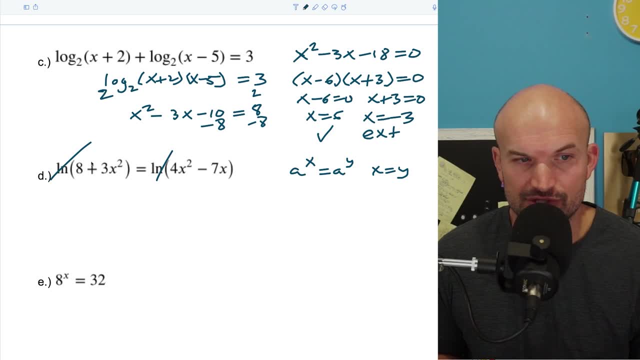 both E. then you can simply just set the arguments equal to each other. So now I basically just have an eight plus three. So I can plug in the six to both of those, And if I plug in a negative three plus a three X squared is equal to a four X squared minus a seven X. So now I have a lovely 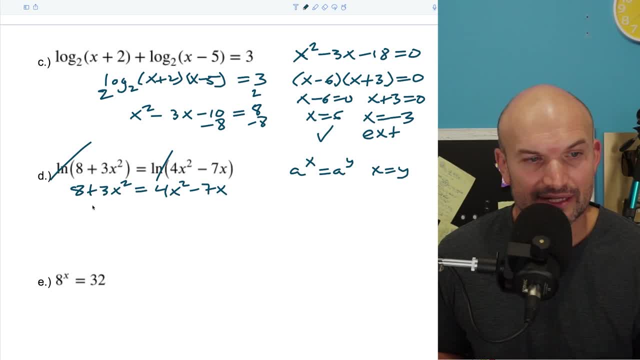 quadratic equation that I just need to go ahead and set equal to zero to go ahead and solve. So do that. I will subtract a three X squared on both sides, and I'll subtract an eight on both sides. All right, So I get: zero equals a X squared. Let's see: minus a seven, X, minus eight Um. 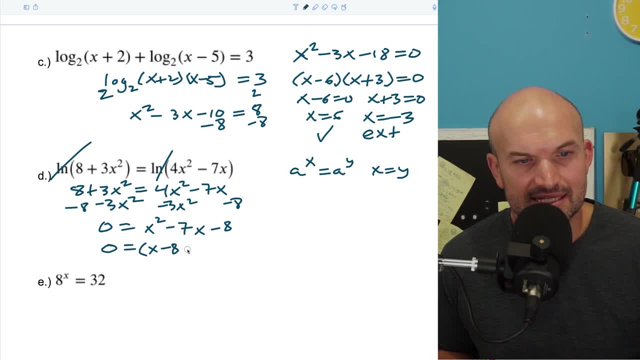 and therefore now I can go ahead and factor this into an X minus an eight and an X minus one. Now I could go ahead and use the zero product property like I did up here, or hopefully you recognize here that I can determine that um X is going to equal an eight. 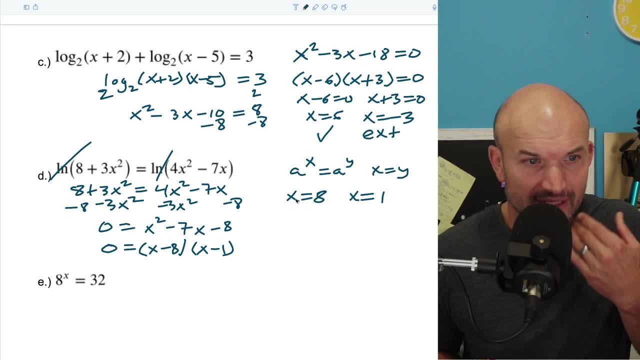 and X is going to equal a positive one. Now what I simply want to do is go ahead and make sure that both of those are going to work right. So when I plug them in, I want to make sure that my arguments for each logarithm are going to be positive. Well, obviously, squaring both of them. 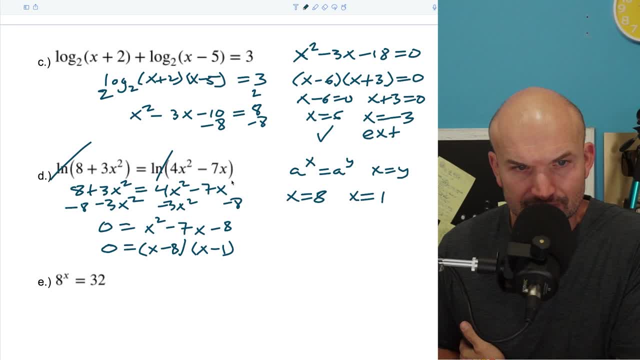 is going to be positive plus eight, that works Um in this case. you know, when I do a um, if I plug in a eight, seven negative, seven times eight is going to be a 56, right. But when I square, 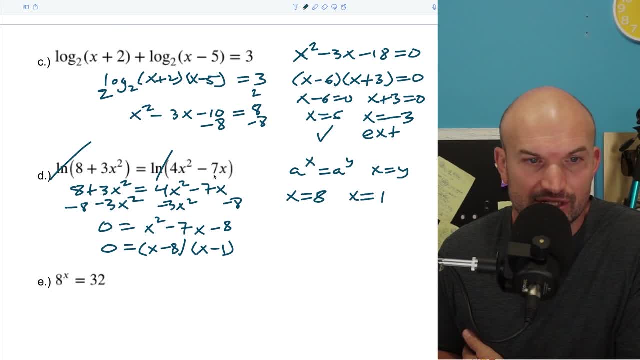 eight at 64,. so 64,, you know, minus a negative number, that's going to work. However, when I plug in one, that gives me a negative seven, that gives me four. So four minus seven is negative three. One is not going to work. So therefore that answer is extraneous. Okay, So now let's. 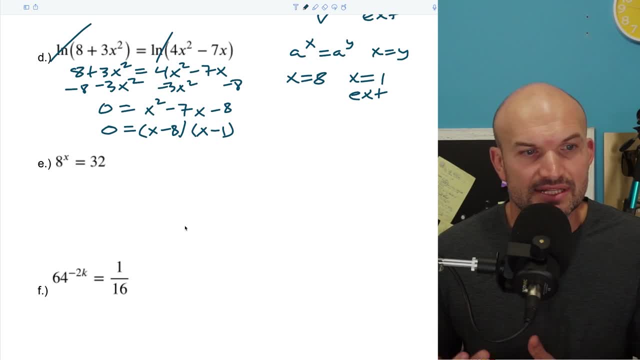 move into exponential equations, And when we're focusing on exponentially, we're focused on exponential equations. The main thing that we're going to want to do in this case is just kind of make sure that we have the basis We want to look for using our one-to-one properties. 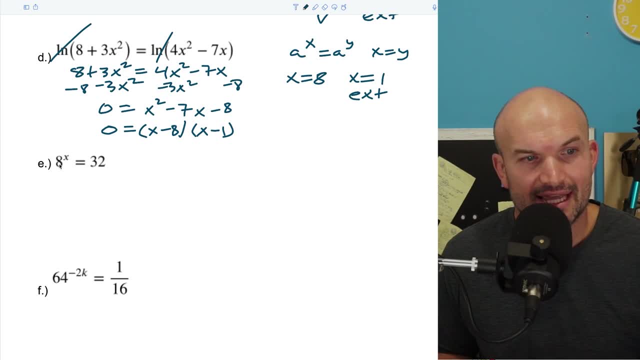 So in this case, what I'm simply going to do is just rewrite a um. I want to be able to see what. how can I rewrite eight and 32 with the same base? So to rewrite eight? um, what I can do is rewrite: 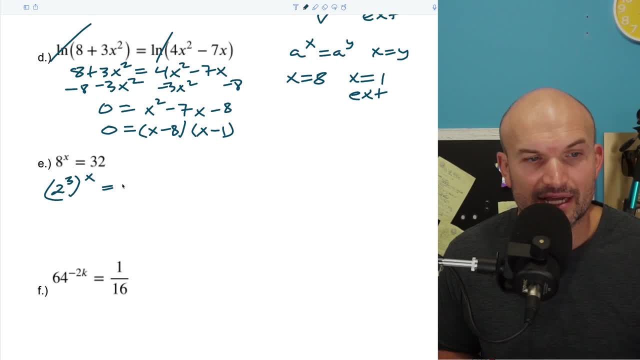 that as a two cubed raised to the X and a 32.. I can rewrite that as a two to the fifth power. Okay, Now you can see that they have the same base. So now I can write the equation of three: X is going to equal five divided by three. divided by three, X is going to equal a five thirds. 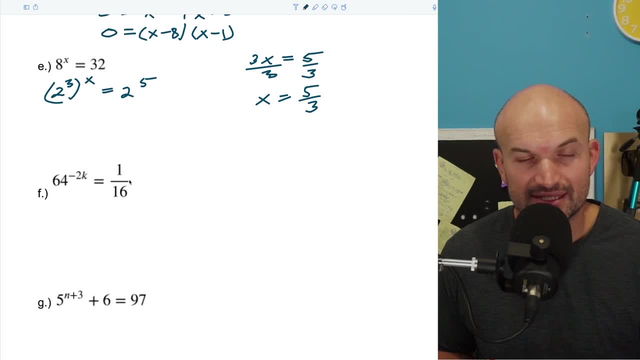 In this example. same thing I'm going to want to do. Um, I'm going to want to rewrite the 16 as a negative number, uh, or with a negative exponent, I'm sorry. So that's a 64 negative two. 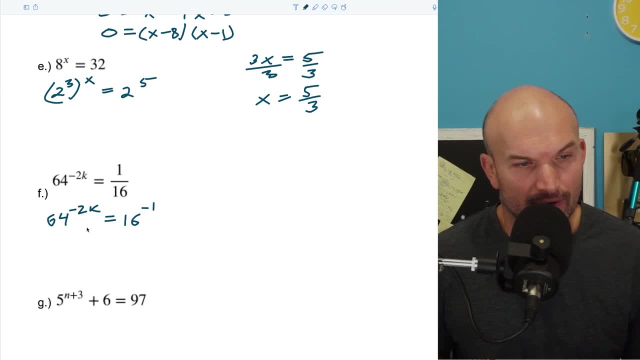 K is equal to a 16 to the negative first power. Okay, Um, so now I want to see what numbers will they raise? Now a lot of people will say eight, right, But yeah, eight goes into 64,, eight times. 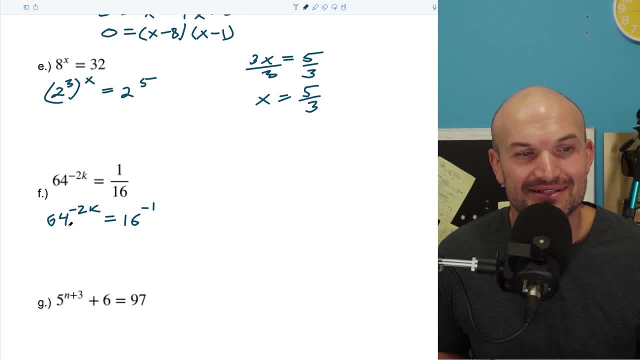 and eight goes to 16,, two times. but that's not the same base, right? So we got to use them as a base. Uh, we got to use them with powers. So um 64 can actually be written as two to the sixth. 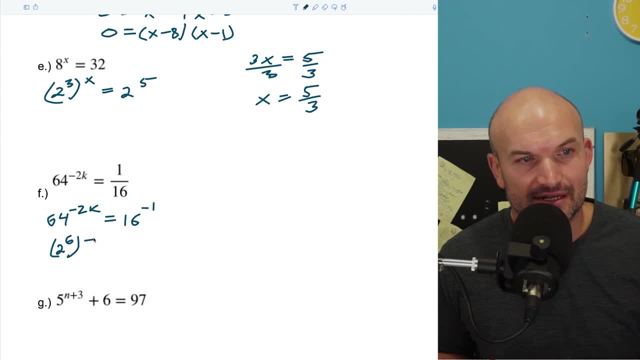 power and that's going to be times a negative two. Okay, And then 16 can be written as two to the fourth power, So that'd be two to the power raised to the negative first power. And again, notice how I'm using my parentheses. Notice how I'm using my parentheses in this case. So, 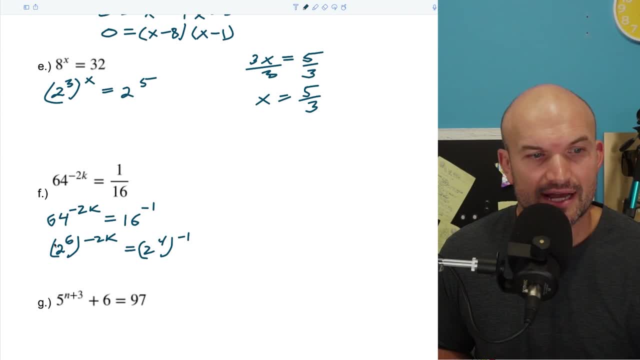 therefore, we can make sure that, um, we multiply those. So now I can just apply the one-to-one property And what I'm going to get here is a negative 12. K is equal to a negative four. Okay, So divide by negative 12,, divide by negative 12.. And then, in this case I'm going to: K is going to. 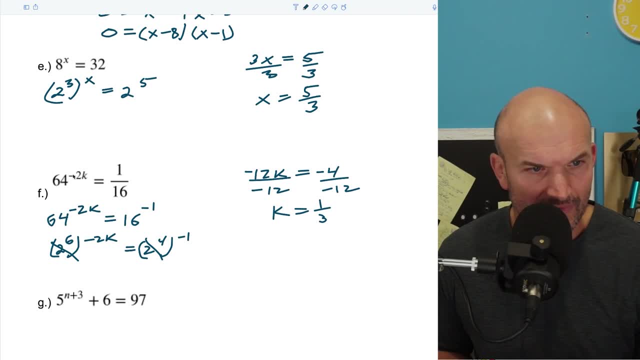 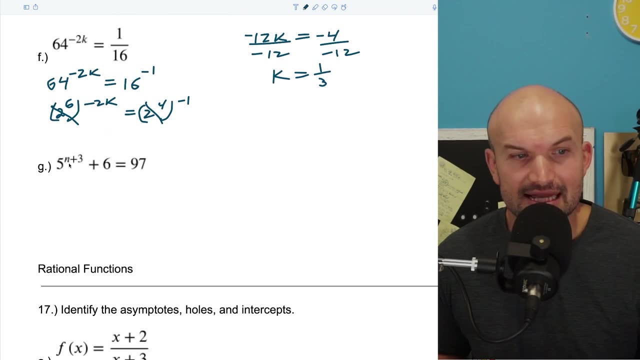 equal to a positive one third And and yeah, that would, uh, definitely that's going to make sense here. as far as plugging that in Um now in this, in this last example here, we have five raised to the N plus three plus six equals 97.. So when I go ahead and subtract a, 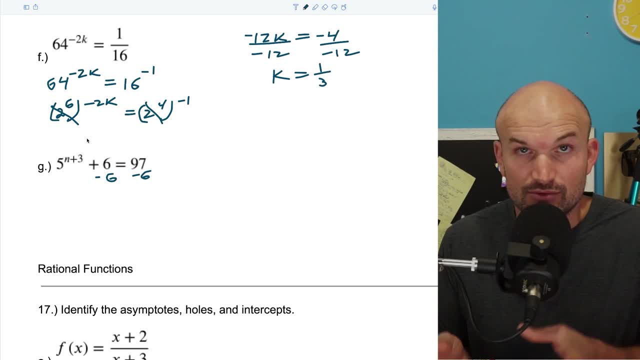 six. right, because just like the logarithms, how we want to isolate the logarithms or get it to one logarithm, the same thing we want to do for exponential equation- We want to isolate this. five to the N plus three is going to equal a 91. We want to isolate the exponent. So now we need: 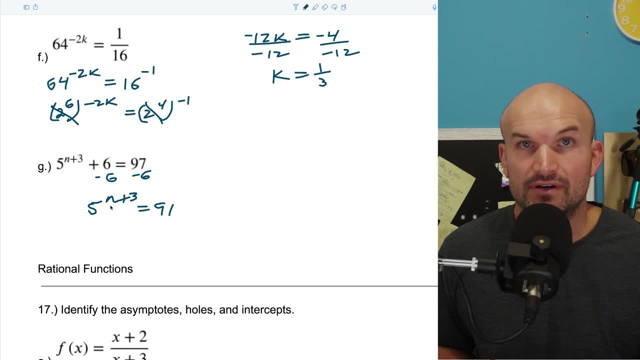 to be able to do. well, how can I solve this, Like how do I get the N plus three off of the numerator? Well, if you're remember that, going back to that rule, if I have log base B of B raised to the X, like if I want to, 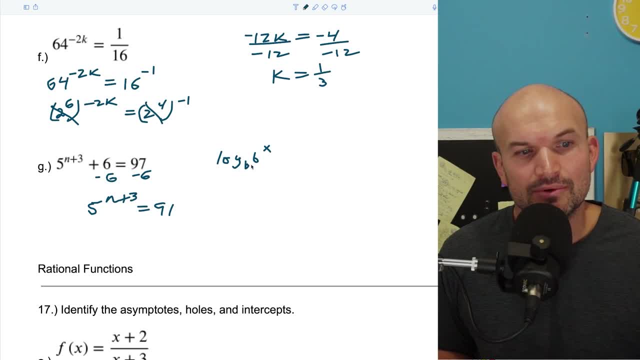 get. if I want to find out what's in that exponent, I need to, um, I need to. let me see. Yeah, If I have a B raised to the X, if I take the logarithm of that, that's just going to equal an X. So 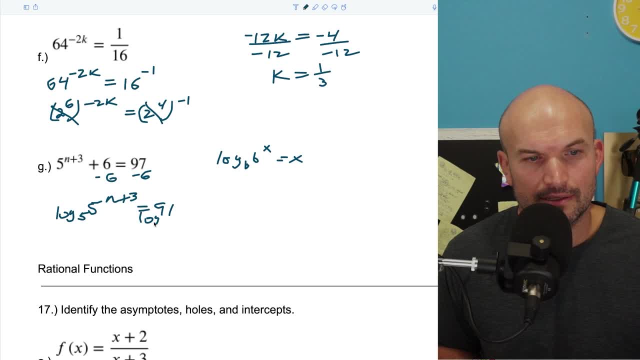 basically, what I want to do is take the logarithm of base five of both sides. So what that's going to now give me is a N plus three is equal to a log base five of 91. Now I can just subtract three on both sides. 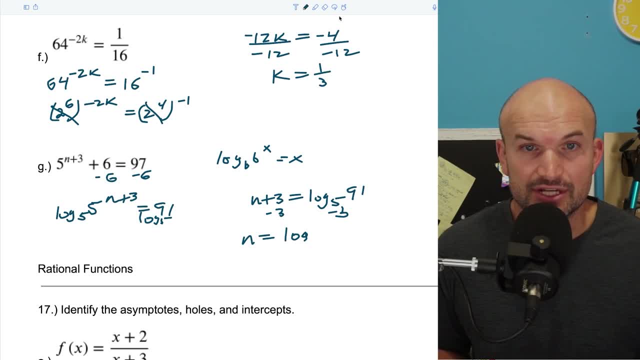 And N is going to equal to a log. Now, in this case, a lot of calculators- you're not going to be able to type that in exactly how it is right. So what I'd recommend you do here is go ahead and 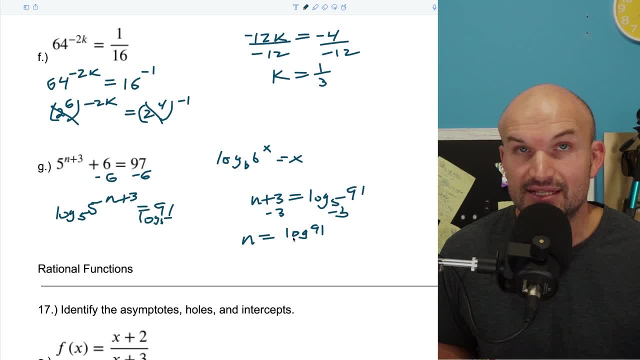 use the um, go ahead and use the change of base formula. So I rewrite this as a log of 91, all over a log of five, and then you're going to minus a three. So in this case, now the, now this is. 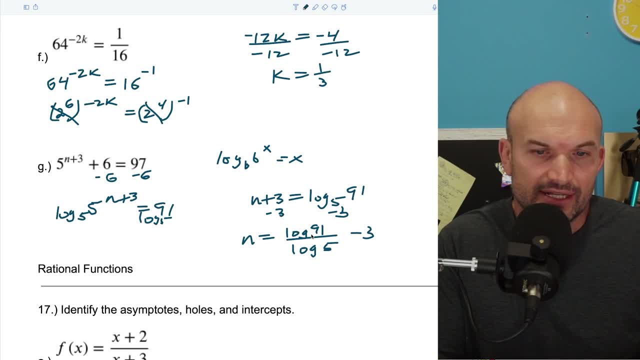 going to be a log base 10, um on your calculator, rather than using the you know log of 90, log of base five and 91. And I'm just going to go ahead and approximate this. Just make sure you're. 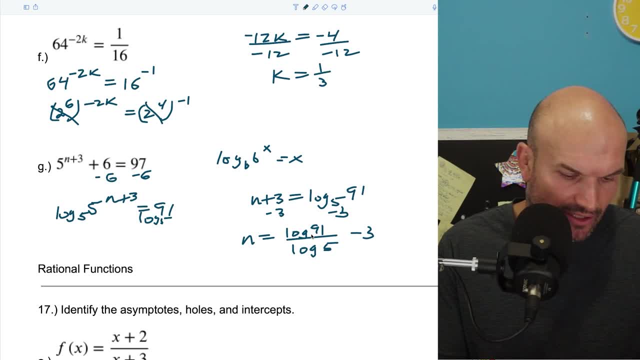 closing your parentheses when you're doing this, I'm going to plug this into my calculator and kind of see what I'm going to get: um minus three, And that's going to give me a negative value, which again 95 to the negative. Yeah, Okay, That's going to make sense, Or at least that. 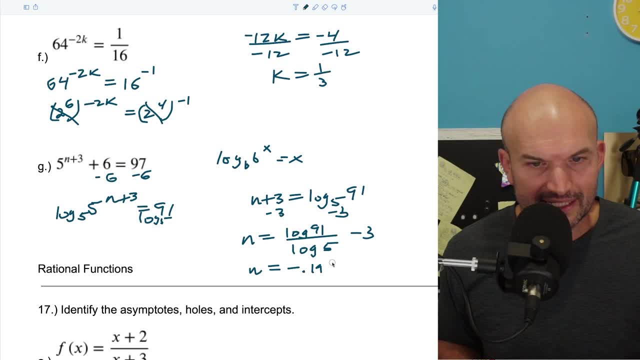 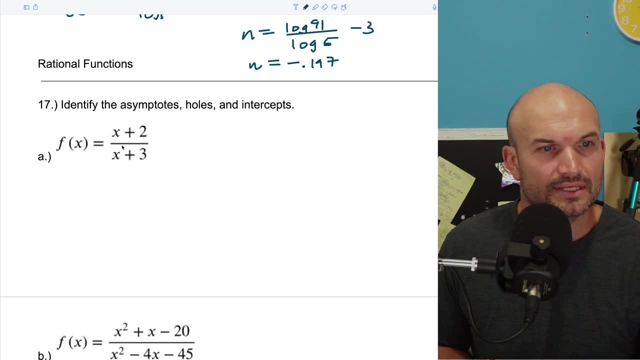 would work, And that I'm getting approximately negative 0.197, and I'll just round to the nearest thousands in this case. All right, Um. so now let's get into rational functions. So in this first example, we're just going to identify the asymptotes, holes and intercepts. So we can't 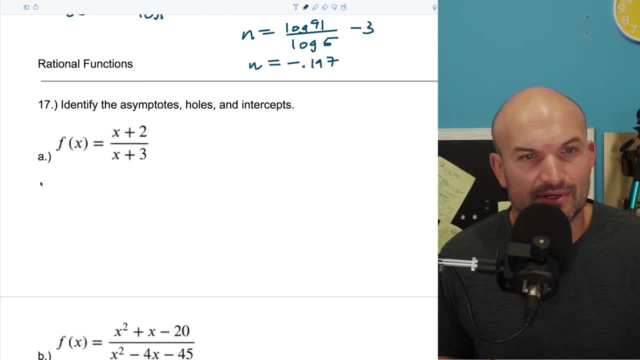 look to simplify first. Um, so just remember the. let's go and talk about the vertical asymptotes here. Vertical asymptotes are they going to be the values that make your denominator equal to zero. So what I always like to do is set my denominator equal to zero and go ahead and solve, And you can. 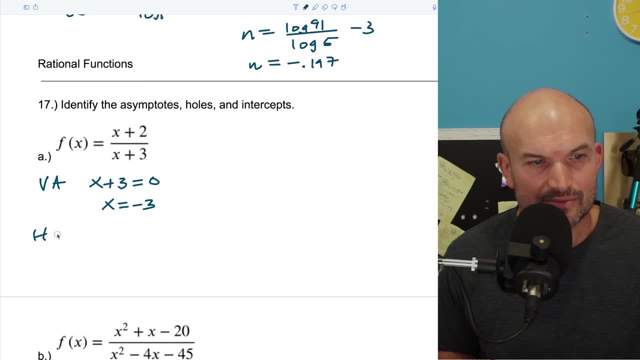 see, X is going to equal a negative three for the horizontal asymptotes. We need to use the horizontal asymptote test And when we're comparing our degrees in our numerator and denominator, then we know that the horizontal asymptote is going to be the leading coefficient. 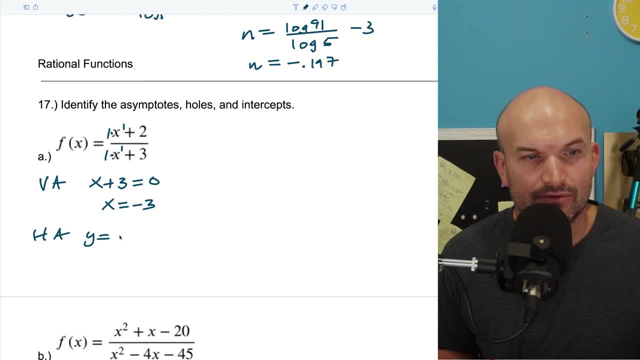 over the leading coefficient. So therefore, this case is going to be: Y equals a one over one, which is just going to be a one Um. so holes would be when we have something that's removable, something that can be divided out, Um. but in this case there are no holes because 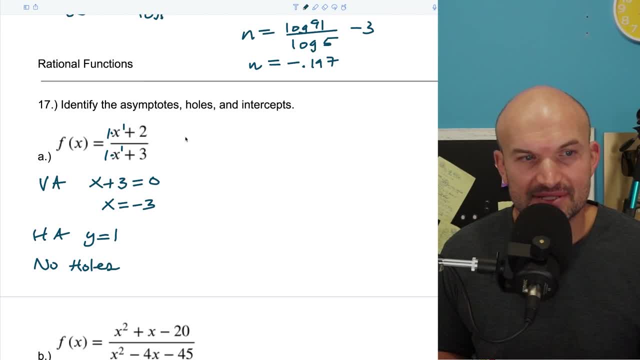 nothing can be divided out or simplified. Now to find the X intercepts. um the best you know, the X intercept is Y is equal to zero, right. Well, if you plug a zero in for F of X right. 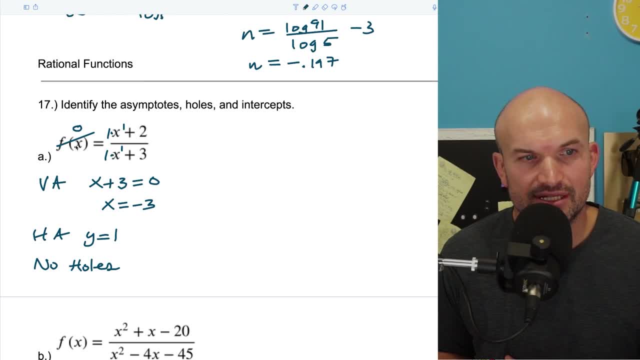 The first thing you're going to want to do is multiply by an X plus one on both sides. So let's see the um X intercept. Okay Is basically all you simply need to do is set your numerator or equal to zero, because when I go ahead and multiply an X plus three on both sides, 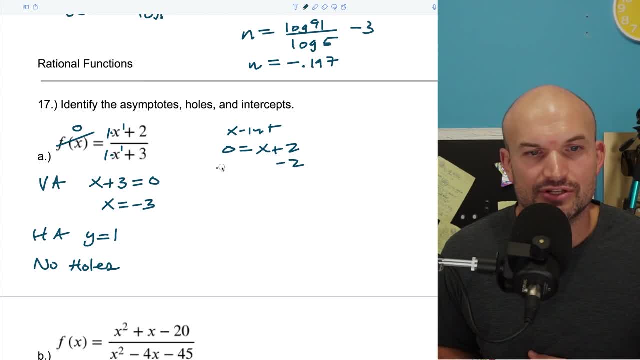 I'm, that's just going to go to zero. So therefore I can subtract it to on both sides and I get a X equals a negative two. And then to find the Y intercept. the Y intercept is when X equals zero. So if I plug a zero in for X and zero and for X here, I'm just going to get a? um, that's. 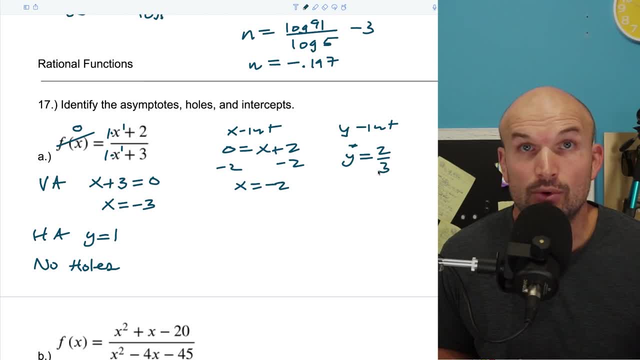 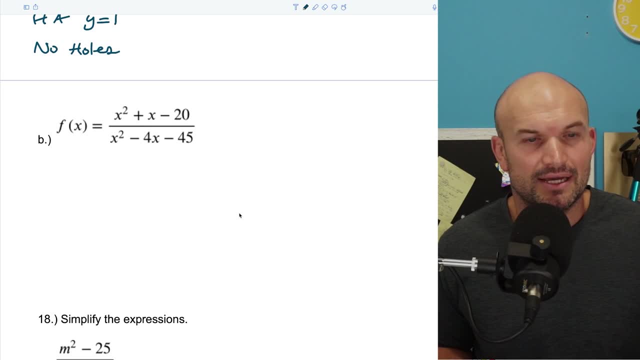 it's just going to make everything just a two or three. So Y is going to equal a two thirds. Um, Oh, we do kind of do another one, So let's go ahead and work on In this example. So this is again. first thing we're going to do is actually simplify this, Okay. 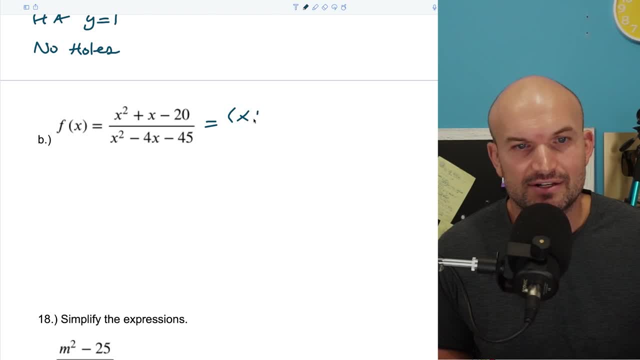 So what we're going to do here is: I want to factor this, So this can be factored into an X plus five times an X minus four, Um, and this one can be factored into a X minus nine times an X plus five. 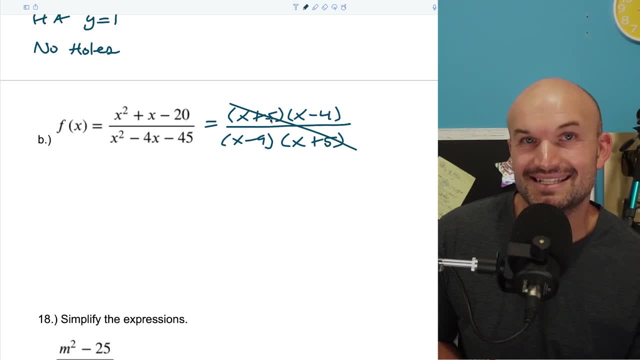 Okay, Now we want to see what can be divided out. and voila, you can see that those can be divided out. So the important thing here is when we're dealing with our vertical asymptotes. um, our vertical asymptotes- if I remember, I said that's when the denominator equals zero. however, 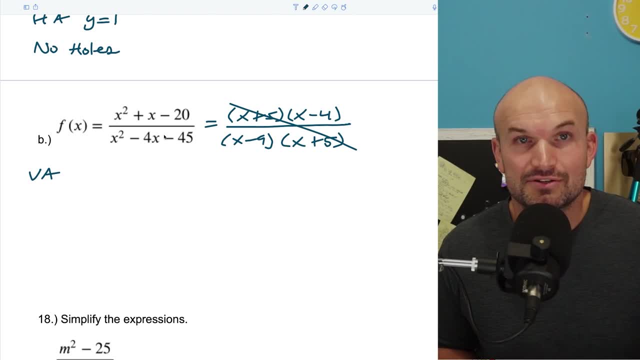 that got divided out. So that is not a vertical asymptote, that is going to be in whole. So the only thing, the only place where we're going to have a vertical asymptote, is when X minus nine is equal to zero, which is at X equals nine- right, Because that's the value that makes your. 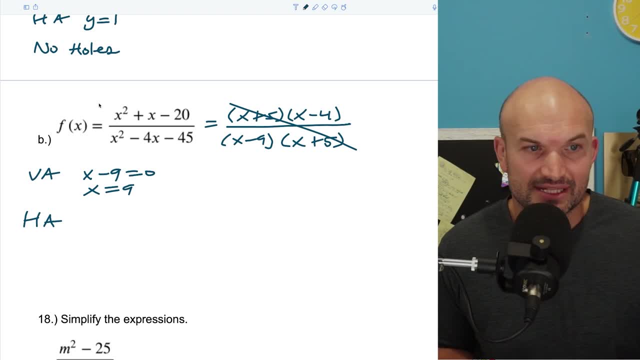 denominator equal to zero. Um, my horizontal asymptote is going to be exactly the same. Notice this: quadratic equals quadratic. So again, you take the linear coefficient over the linear coefficient, which is: Y equals one over one, which in this case is one. So it's only, it's only the. 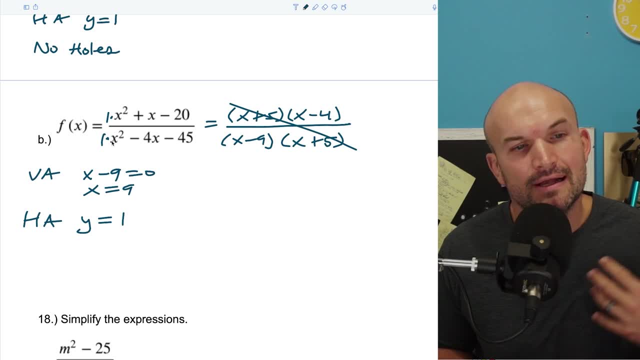 linear coefficient over linear coefficient when the powers are the same. Okay, Um, but remember you could also have a slant asymptote or no asymptote. So that's all within the horizontal asymptote rules. Um, as far as my holes go, um again. this is going to be divided out, right? 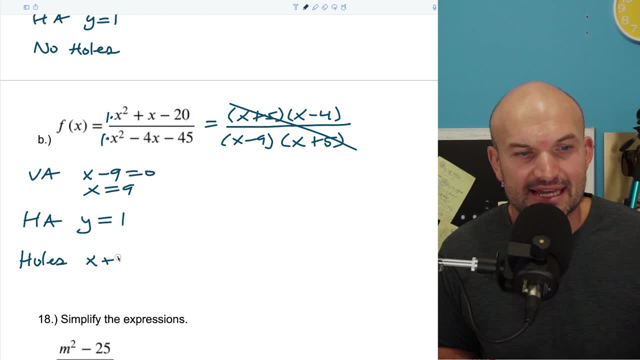 See how the X plus five simplified out, So my X. so what I'm going to do is I'm going to take the value that gets divided out and that's going to be your whole. So therefore, um, I don't know why. 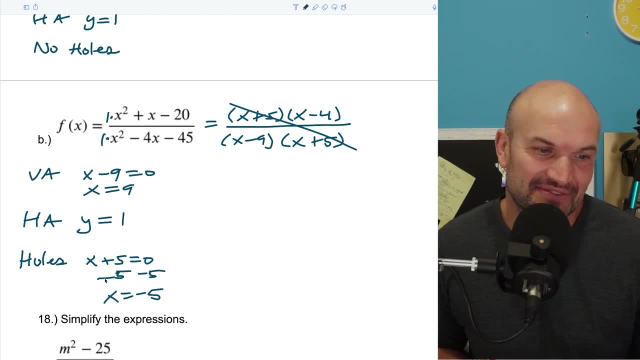 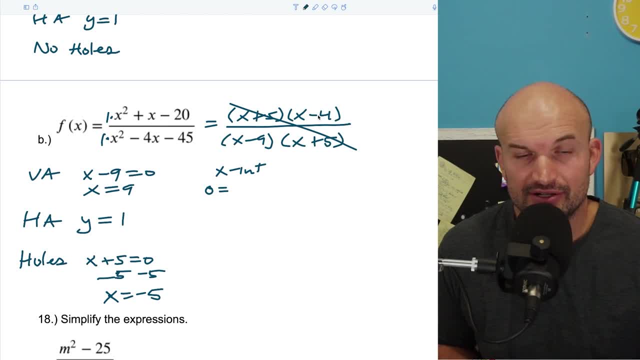 right? So let's go ahead and rewrite this in factored form, right? We already factored it, So let's just write that out. So X plus five times an X minus four, um to do X plus five times an X minus four, and the X plus five got divided out. That's a whole. so that's not an. 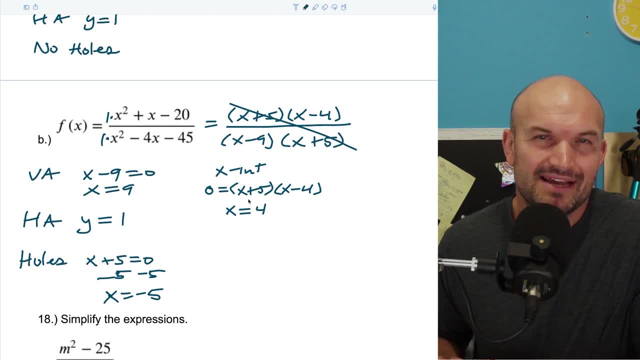 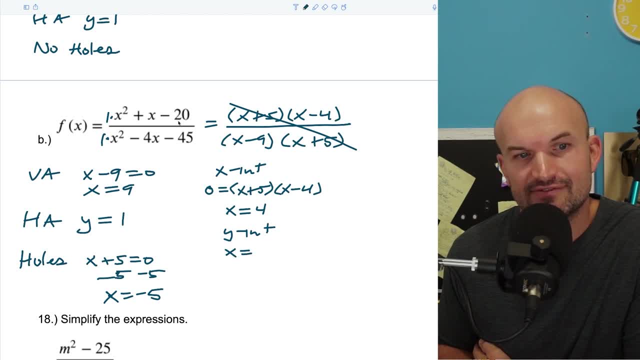 goes zero. So therefore I'm just going to have an X is equal to a negative 20 over a 45.. Um, let's see I can probably simplify that. Let's go and see what it'd be. So five goes in 45, nine times. 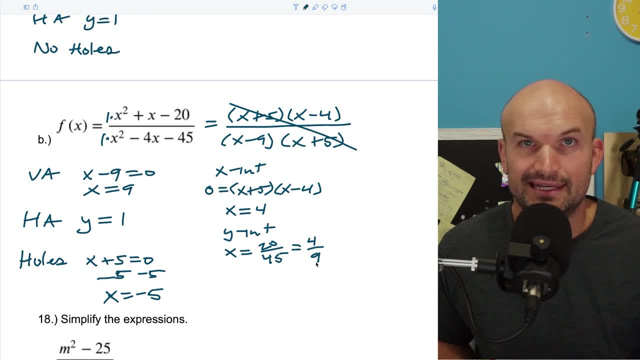 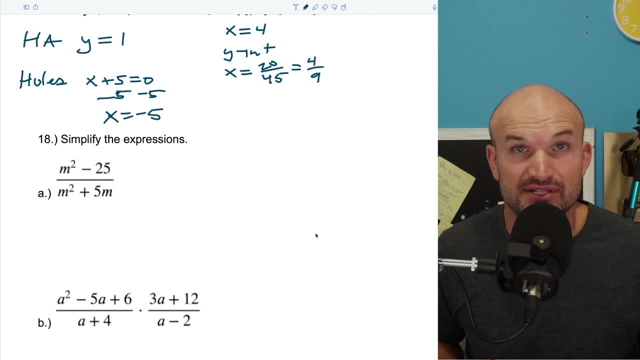 So that's a four nights can be simplified. Hopefully I did that right. Um, all right. so let's just practice simplifying some expressions. And basically what we're new is we're just going to be factoring, factoring, factoring, factoring, factoring. So, um, I'm 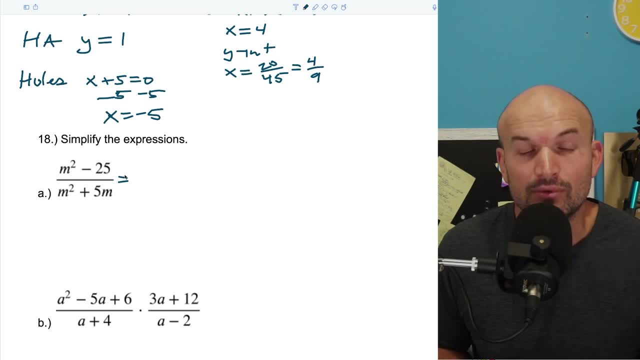 not going to spend a lot of time explaining the factoring process. I'm just going to kind of go through. I will explain what I'm doing. Um, but again, the only way you're going to get better at factoring is practicing. Okay, Not watching, watching YouTube videos or watching. 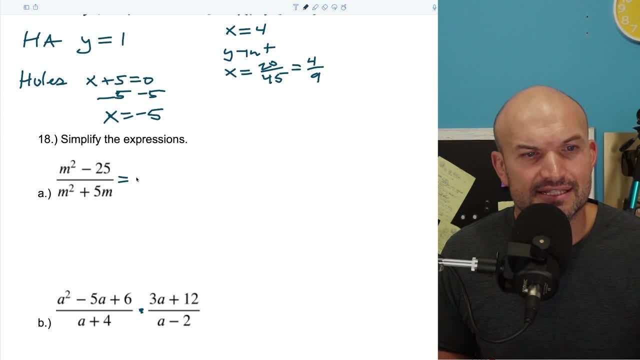 myself do it Okay. So in this case, um, this is a difference of two squares, So that's an M minus five times a M plus five, Um, and then down below here I can factor out the M first and that's: 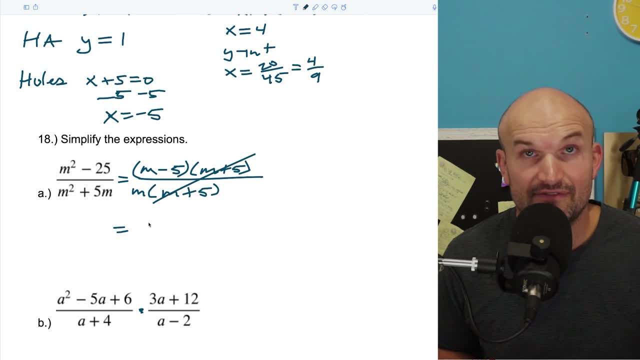 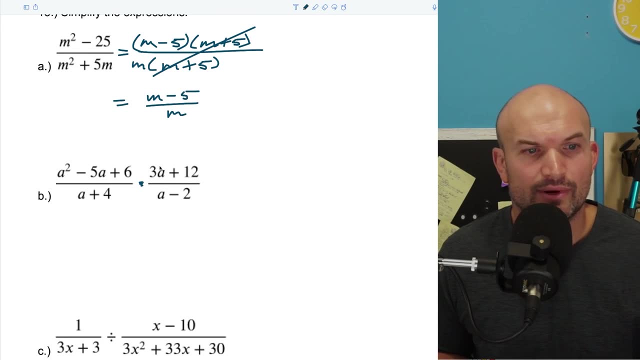 going to leave me with an M plus five Those divide out. So my final simplified expression is a M minus five all over an M Um in this example. here again, we want to simplify before we multiply. I remember when we're 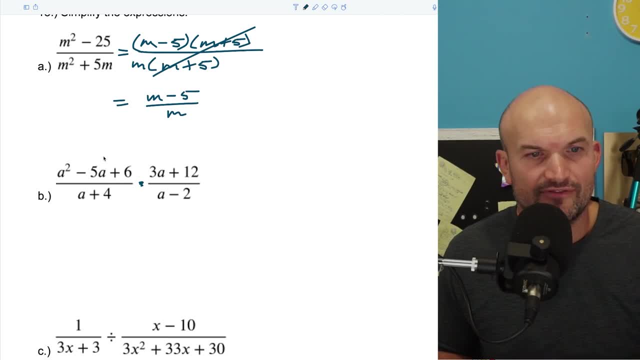 multiplying rational expressions, you're multiplying straight across. So let's just go ahead and factor everything we can, And um in this case. so this one would be a a minus three times an a um minus two. And then here I can factor out a three and that's. 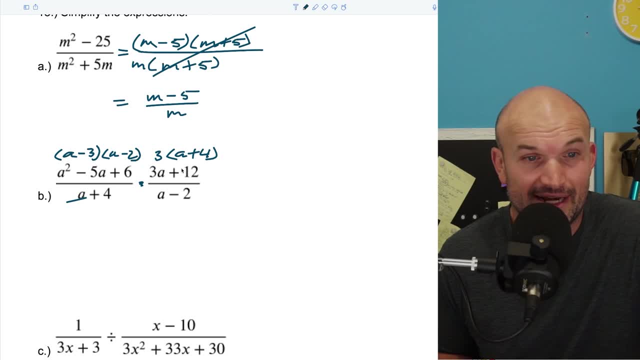 going to be an, a plus four. Okay, So let's divide out things that actually can be divided out before we actually multiply. So those are going to divide out. So now both denominators divided out. So I'm going to do a three times an, a minus three. So that was kind of simple. Um, in this case, 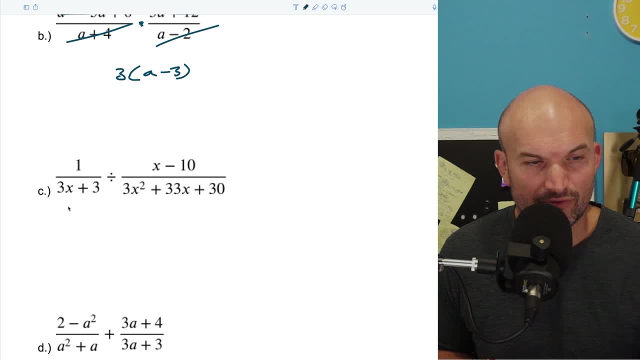 remember, dividing is the same thing as multiplying by the reciprocal. But before we do that, let's go ahead and simplify. So here I can factor this out to a three times an X plus one Um. here I can factor out the three. that's going to be an X squared plus what? 11 X um plus 10.. And then 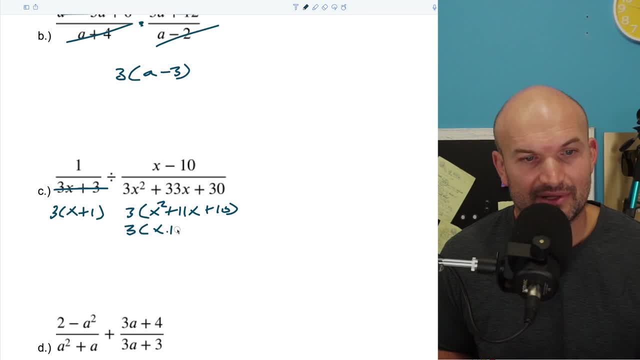 that can again be factored out to a three times a X plus 10 times an X plus one. Okay, Guys, don't be like, don't be scared of like showing your work, Okay, So when I'm dividing this, that's the same thing as a three times three times X plus one. 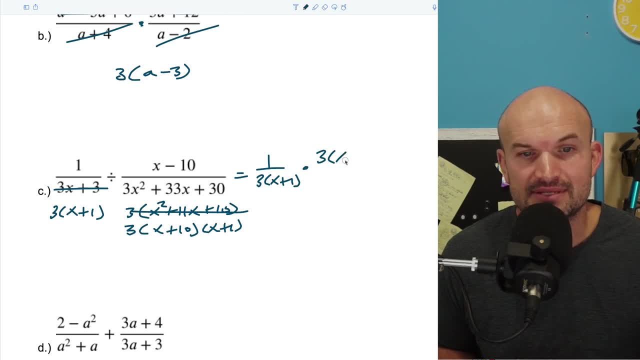 And then remember, we're going to multiply by the reciprocal, So a three times X plus 10 times an X plus one, Okay, And that's going to be all over a X minus 10, right? So basically I just reciprocated the divisor and now you can see: the threes will divide out, the X plus ones will divide. 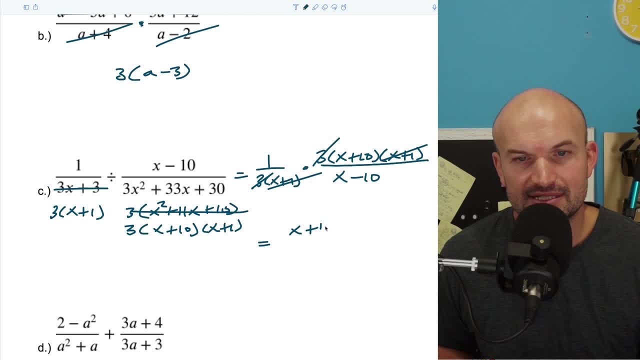 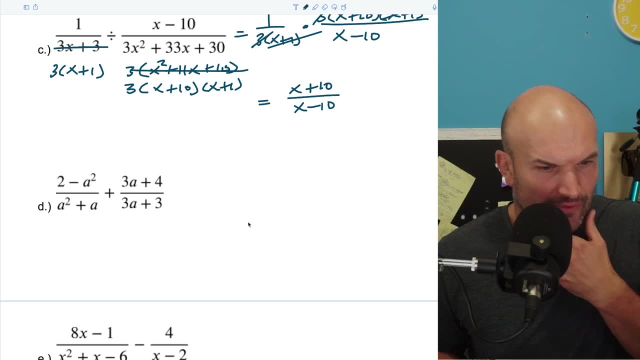 out, And now it's going to leave me with a X plus 10 all over a X minus 10.. Now, when adding? and so the next example we're going to be- I think we're, yeah, I do- an adding and subtracting. So for adding and subtracting, remember we got to get common. 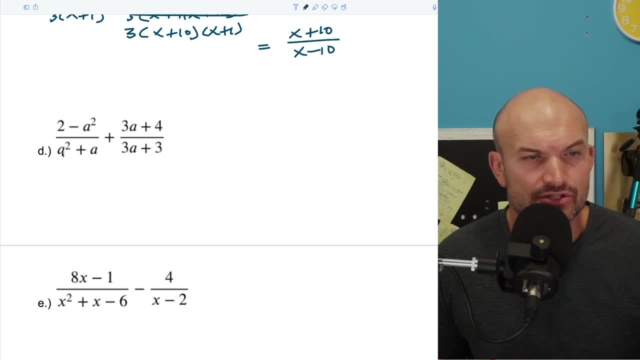 denominators And um, so to go ahead and do that. what we need to. first thing we always need to do, though, is simplify, simplify, simplify, simplify is always going to be your best bet. I do not like the way that's this written- this two minus an A squared, So what I'm gonna do is I'm going to. 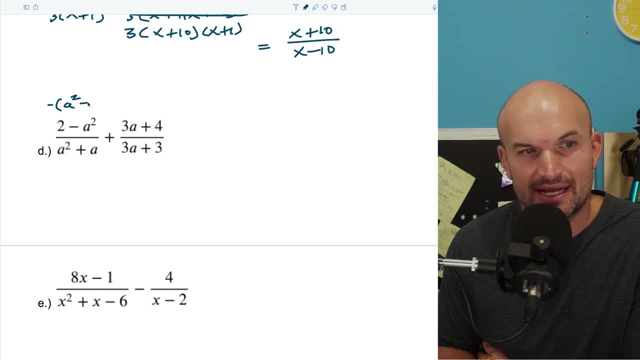 factor out a negative and I'm going to rewrite this as an A squared minus a two. That doesn't really seem to help me out anymore. um from in there. So actually I think we'll be okay, Let's go ahead and factor out our denominators. 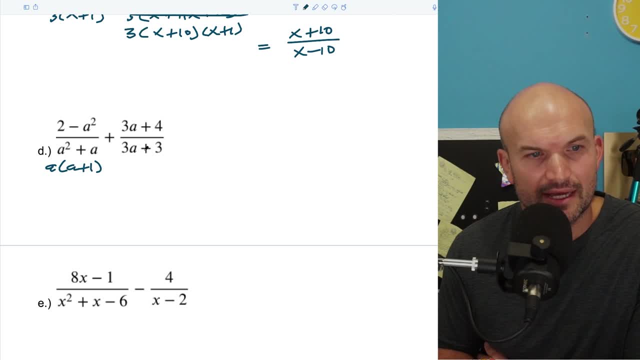 So here I can factor out an A, that'd be an A plus one, And here I can factor out a three, which would be also give me an A plus one. Okay, So there's my two denominators. What do they have in common? An A plus one, right? What do they not have in common? An A and a three. So what I'm? 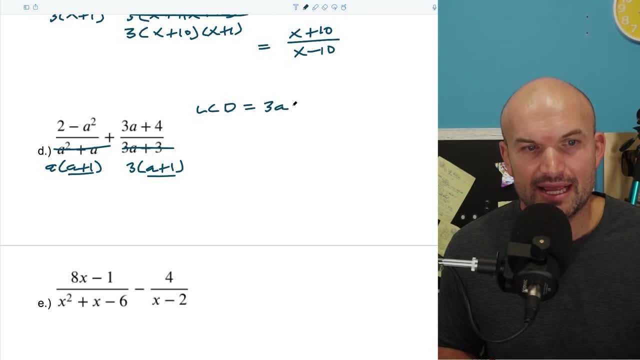 going to do is I'm going to list out my LCD. My LCD in this case is going to be a three A times an A plus one. Okay, So to. to get my common denominator here, I need to multiply by three over three. to get my common denominator here, I need to multiply by an A over A. Now again: 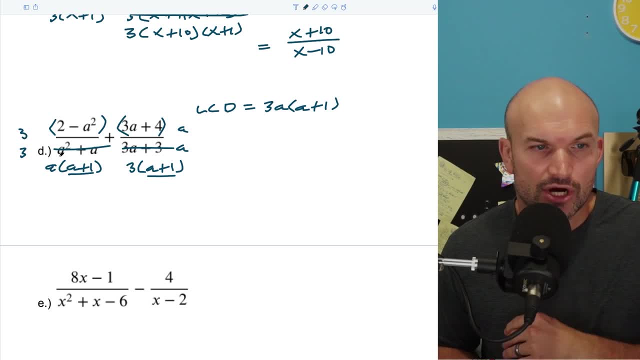 make sure you put parentheses around here when you're using an LCD. So therefore you can simplify correctly. So when I multiply three times an? A times A plus one, I'll get the LCD. When I multiply an? A times a three times A plus one, I'll get the LCD. 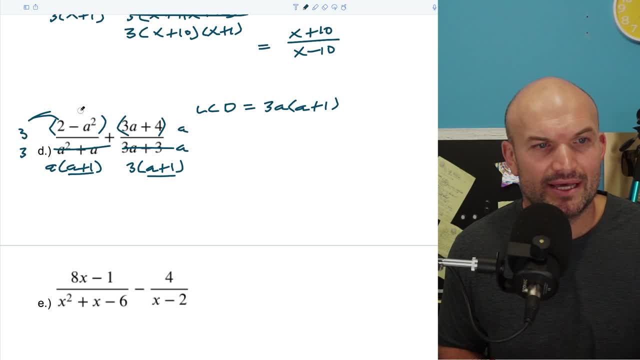 That's exactly what I'm looking for, So I'm going to go ahead and multiply this and then just going to rewrite everything all over the LCD, Cause I'm going to have to simplify that. Okay, So we're going to have a six minus a three um a squared, And then over here. 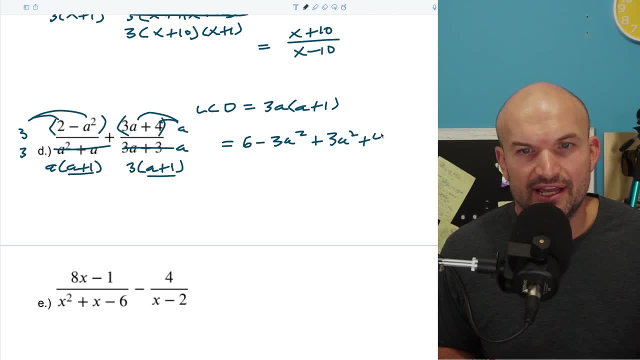 I'm going to have a plus a three a squared, plus a four a, and that's going to be all over my LCD, which is going to be a three a times an A plus one. All right, So now you can notice that these are going to add to zero. 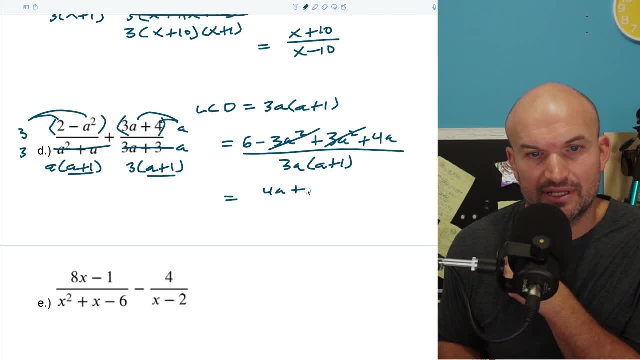 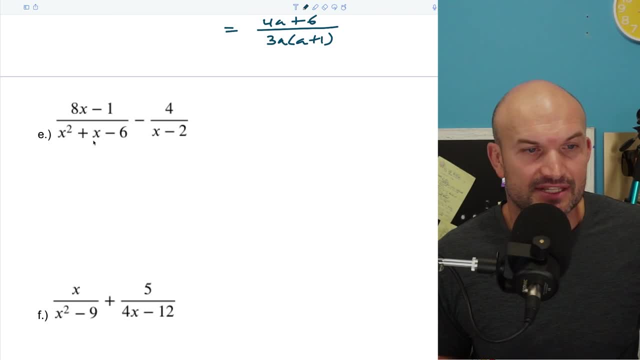 and then, therefore, I'll left with a final answer of a four a plus six all over a three a times an A plus one. Okay, Um, all right, let's go and take a look at this. one Same thing We need to. 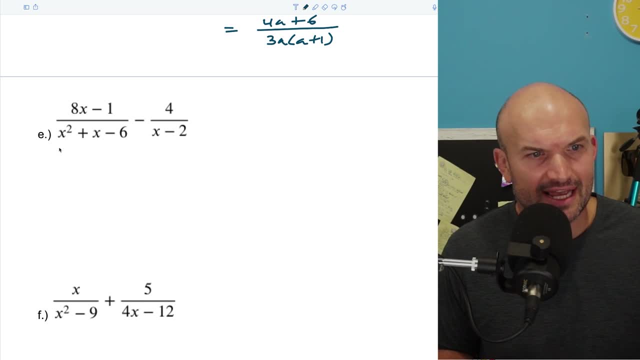 find the LCD Um. so I want to factor that And when I factor this one. so now we're just going to apply the operation differently. Now we're just going to subtract the numerators. So in this case I'm going to have a X um minus two times an X plus three. 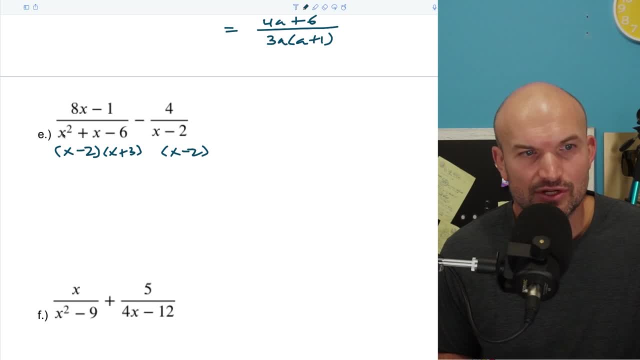 So notice how they both share the X minus two. So the only thing now to get this LCD on the right hand side is I just need to multiply by an X plus three. Okay, So I'll just do that And I'll just label that, and LCD equals um. let's see X minus two times an X plus three. All right, So make. 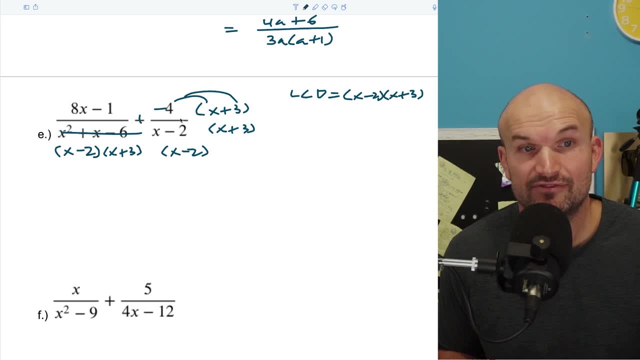 sure you apply distributed property and also make sure that that is a negative four, Okay, So sometimes I like to write it as a, as an addition problem and just with a negative. So therefore, this is now going to give me a eight X minus one, uh, minus. 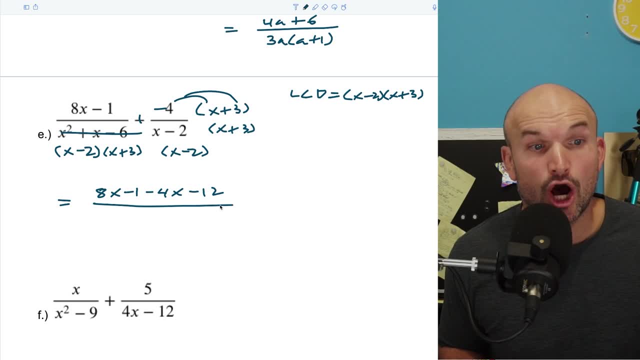 a four X And therefore that's gonna be minus a 12. And that's gonna be all over my LCD, which is a X minus two times an X plus three, And a lot of times we just leave it exactly as it is. Um, we. 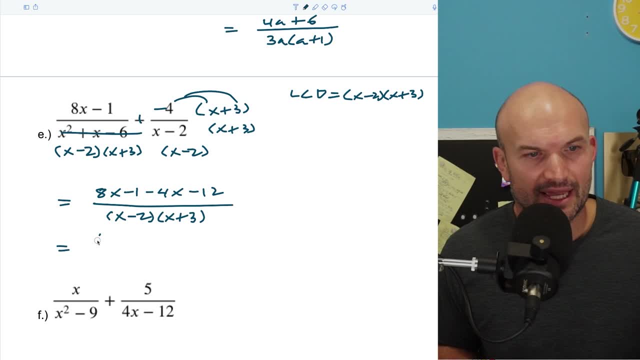 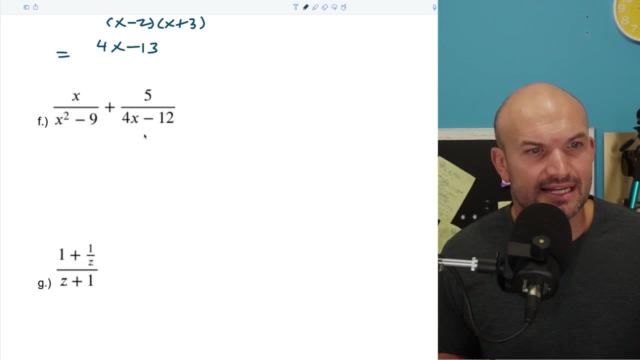 don't go any further from there. Um. so therefore, now, this is going to give me a four X, um, minus a 13.. Okay, Um, now, in this next example, I guess I'll just do another, another one from here. So. 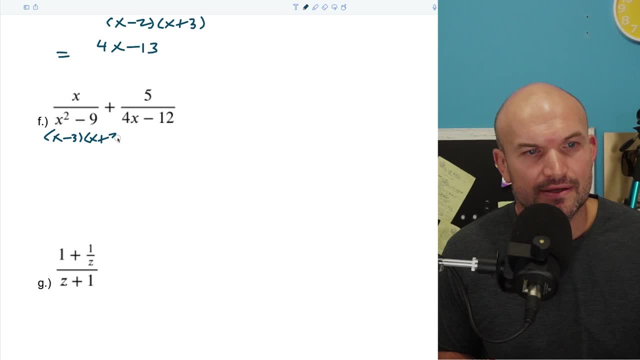 factor this into an X minus three times an X plus three. here I can factor out the four Into an X. uh, let's say, factor out four, That's gonna be an X minus three. So again, from here I need to multiply by a four over four, And over here I need to multiply by an X plus three. 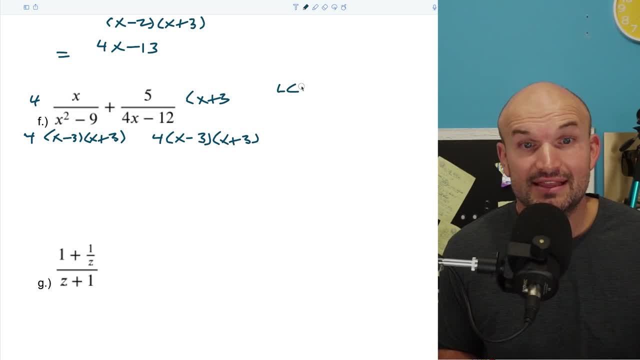 over an X plus three. Okay, So my LCD in this case is going to be a four times X minus three times an X plus three. All right, So now I'm going to get a. let's see, just apply distributed property here. So I'm going to get a. no, I don't like to write my fours like that. 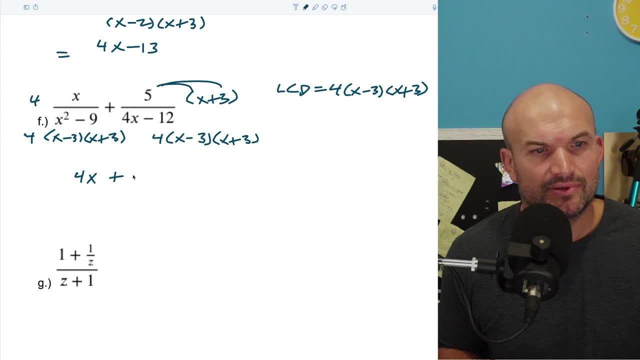 So now, in this case, I'm going to get a four X and that's going to be plus a five X plus a 15. And that's going to be all over here: A four times a X minus three times an X plus three. 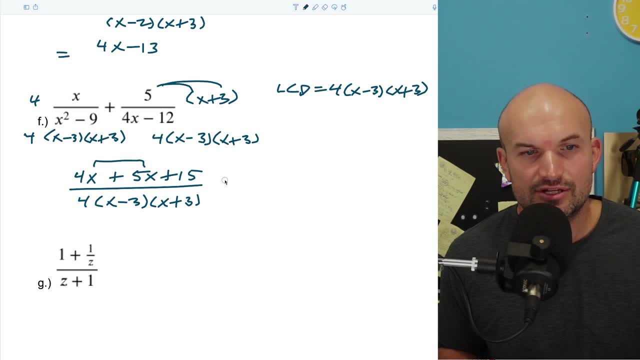 And then again you need to simplify that right To give you a nine X. So my final answer is going to be a nine X plus 15, all over a four times X minus three, times an X plus three. Perfect Okay. 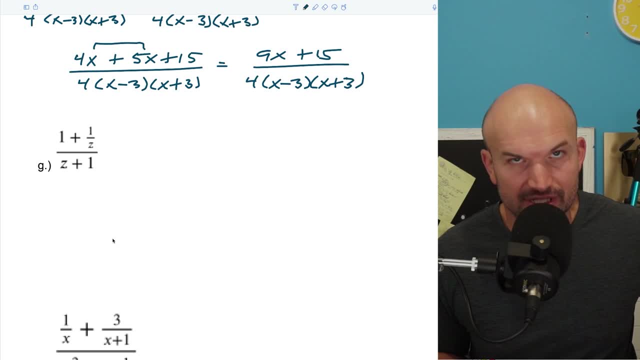 So now let's go and take a look at some complex fractions, because, like, complex fractions usually gets to a lot of students, but it's basically, you know, the same idea. We we have so many. when we have multiple fractions, we have a complex fraction. So what I'd recommend for a problem like this is just to go ahead and 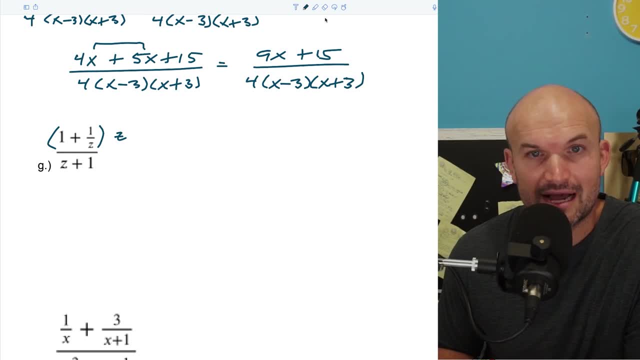 multiply by a Z or sorry. you need to find your common denominator. So you might say: well, what is my common denominator? Right, There are so many denominators going on. So, basically, what you want to do is just go and look at the denominator of each of your terms. Okay So, 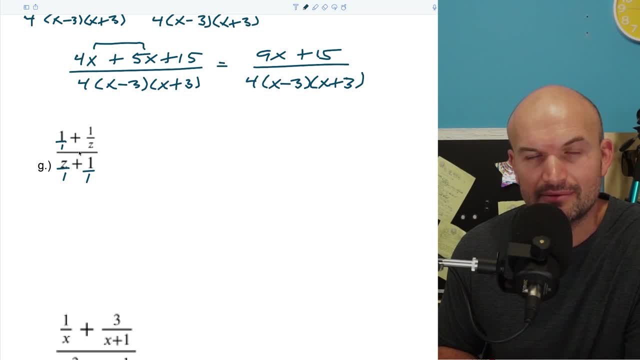 in this case, we have all these, we have a numerator, a big numerator and big denominator, right, But you can see, here there's only really one denominator, Z, and one. So my LCD, in this case, is just going to be Z. So what I'm going to do is I'm going to multiply everything times Z. 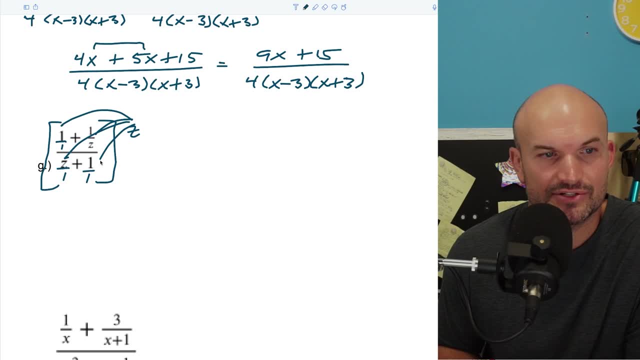 Okay, Now when I do this, you need to make sure you're multiplying. everything times your Z. So when I do that, I get a Z plus Z times one over Z. It's just going to be over one times a Z times Z is a Z squared, And then Z times one is going to be plus a Z. Now I can go ahead. 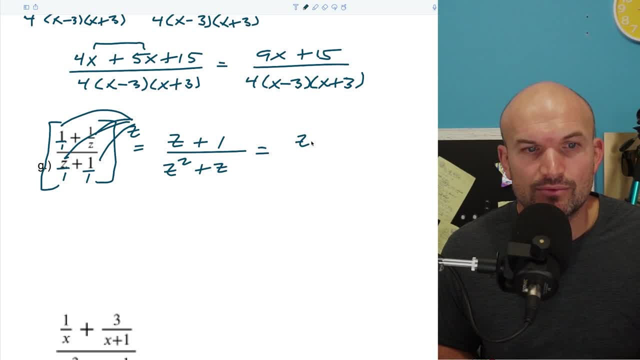 and simplify or factor out a Z right. So always make sure, once you like, get rid of your fractions in the numerator and the denominator by multiplying by the LCD. Now you want to see if you can simplify, So here I can factor out a Z. So that's going to be a Z plus one right. 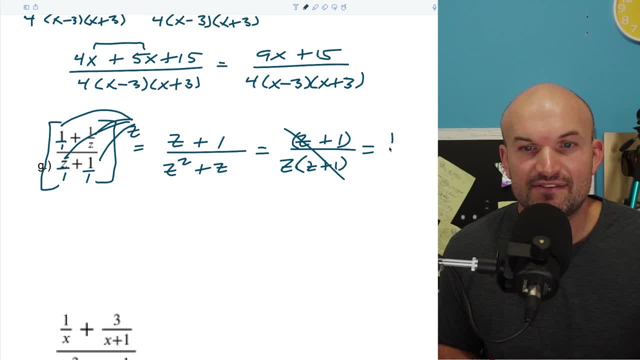 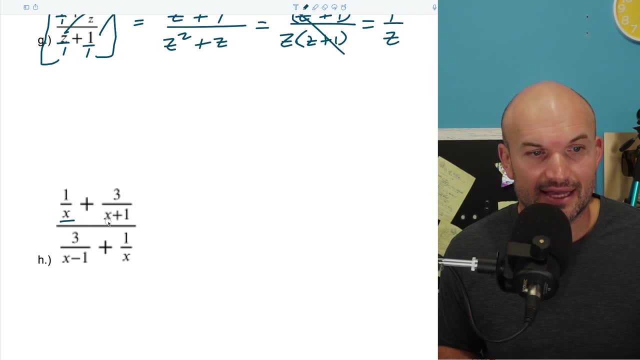 And guess what Those are now going to divide out, And that's just going to leave me with a final answer of one over Z. So let's go and take a look at here. Now we have some again, some more denominators. right, I have an X, X plus one, X minus one and X, So my LCD in this case. 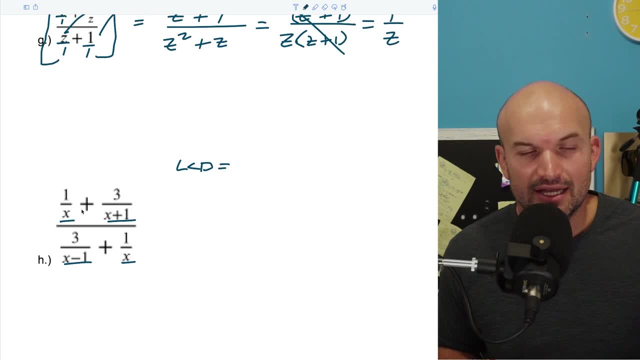 is going to be just the, basically the product of those You don't. you don't need to write X twice, right? All you need is really one of them to be able to divide out, But then I'm going to have an X plus one and a X minus one. Now, this problem could take me a really, really long time. 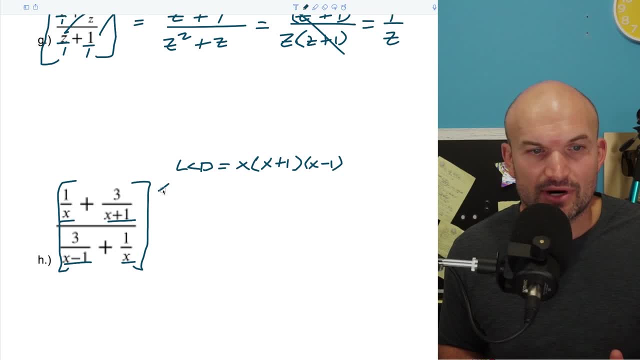 If I was to rewrite the LCD times each and every one of these products. So I'm just going to try to make sure I talk a little bit slower and go through this a little bit smaller As I multiply this times each and every one of these. Okay, I don't want to draw the lines, though, because it's 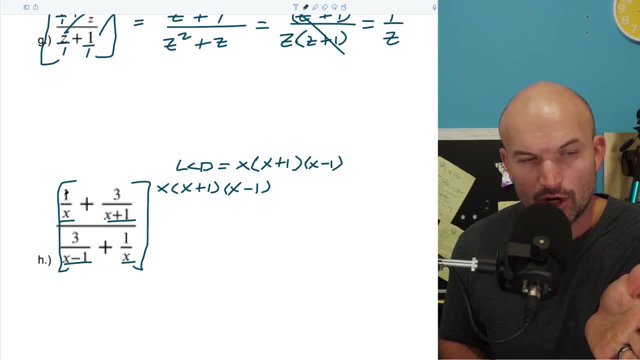 just going to be like such a mess. So let's do this first one, one over X, plus one. When I multiply this times that, right, When I multiply this times, my LCD, the X's are going to divide out. So that's just going to leave me now with a um X times a. 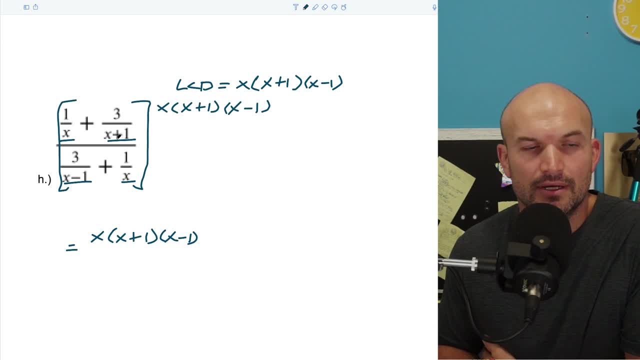 X plus one times a X minus one. Okay, All right, Now let's go and take a look at this example. When I multiply this fraction times this fraction- Oh, I'm sorry, And um, that's going to be multiplied by one, right, There's still that one there. Make sure you have your. 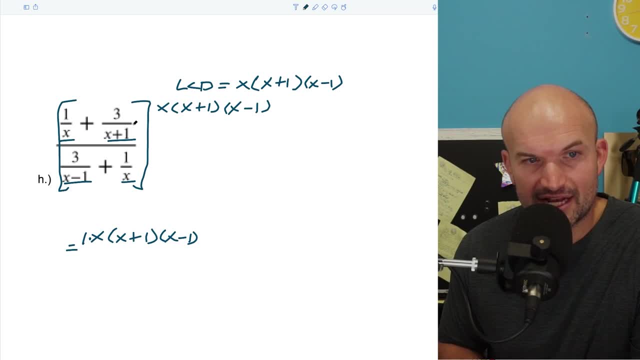 accounting. When I multiply this fraction times this, the X plus ones are going to divide out. So what that's going to leave me with is a three times a X times a X minus one. I don't know why I'm writing the X- X in parentheses. Let's just write it like this: So it's a three. 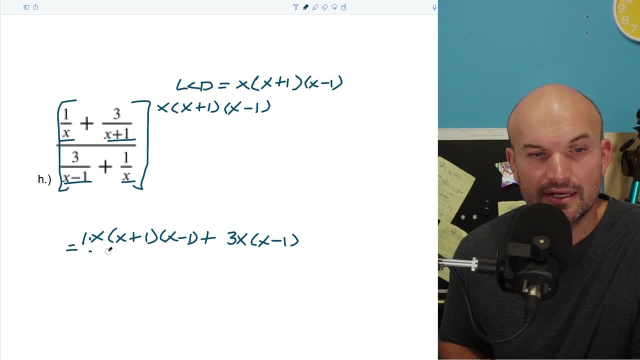 X times a X minus one. All right, So that's it for the numerator. Now let's go over to the denominator. here the X minus ones are going to divide out And that's just going to be with a three times X times X plus one. So three times an X times an X plus one. Okay, And then over here. 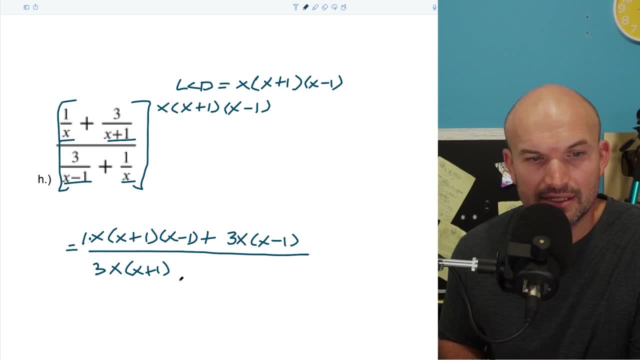 again, the X's are going to divide out and that's going to leave me with a one. So that'd be plus a one times a X plus one. X minus one, So X plus one. Um, I don't know, That looks really bad, So let's go and fix that. So that's going to be. 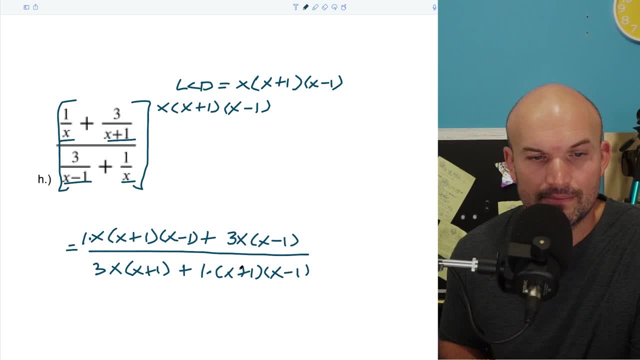 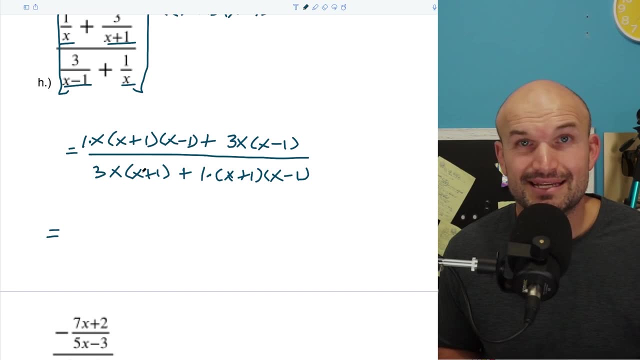 X plus one, And that's gonna be times a X minus one. Okay, So now let's go and see what are some things we need to know. Um, so X plus one times X minus one is X minus one squared right, So that'd. 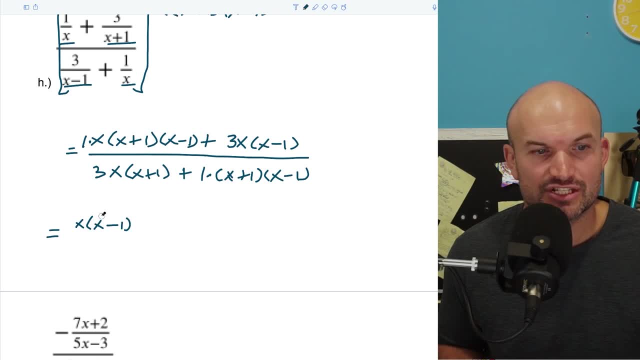 be X times a X minus one, I'm sorry, X squared minus one, And then this is going to be a three X minus one, or sorry, that's a three X squared minus a three X, right? Make sure you apply distributive property, Um, and then I can apply distributive property over here. but we'll do that. 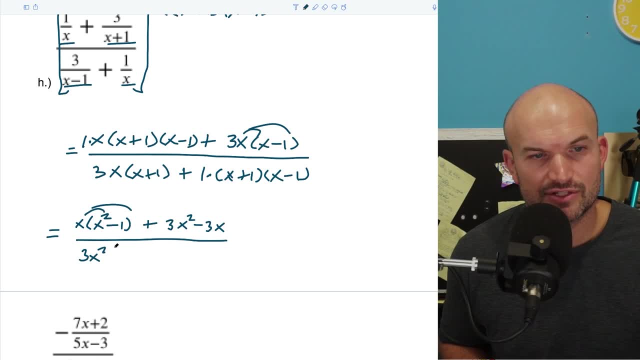 in the second round. So over here I apply distributive property. That's a three X squared plus three X. over here That's going to be plus a X squared minus one. Okay, So the only thing I didn't be able to do distributive property was this one. So that's going to give me what a X. 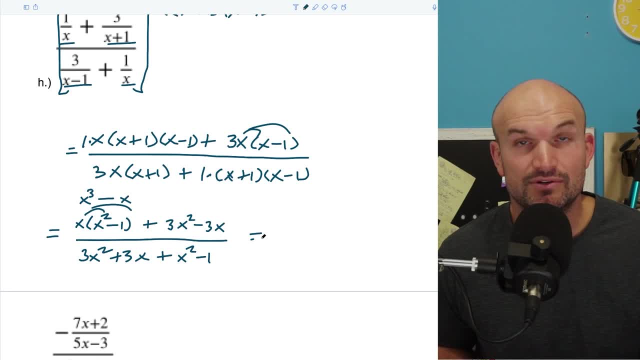 cubed minus an X, right Okay? So let's go and simplify. now write the final answer. So I have an X cubed um and then negative X minus three X is going to be a negative four X, but let's do the X squared next. Sorry, 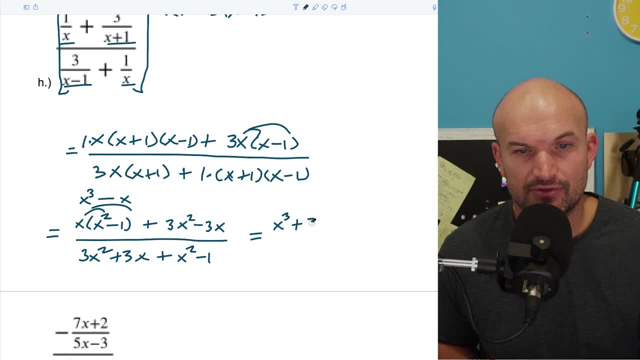 So I just have an X square, I only have one X squared, So that's gonna be plus a three X squared, And then negative X minus three X is going to be a negative four X And that's, and then denominator: here I can only combine these two, So that's gonna be a four. 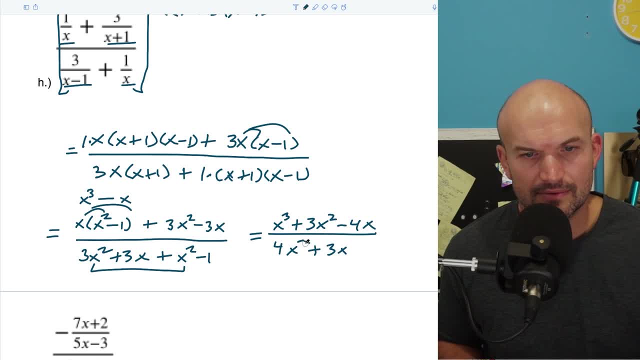 X squared. um plus a three X minus one. All right, And then you could- I guess we could- go ahead and factor these and see if there's anything that simplifies out. So if I factor out an X, that leaves me with an X squared. 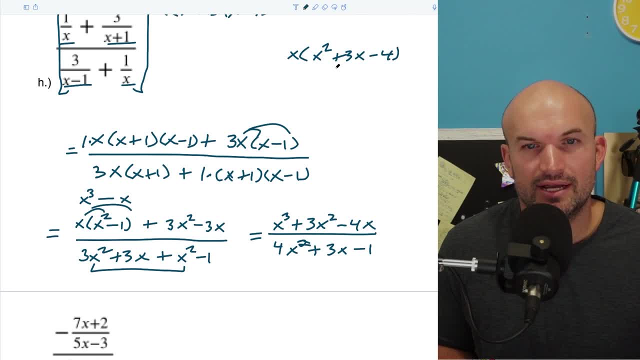 Plus three, X minus four, right, And that can be factored down. So that can be factored down into a X plus four times an X minus one. Okay, And then let's go and do this one. Um, so that is my numerator and then my denominator. Let's see, how could I factor out a. 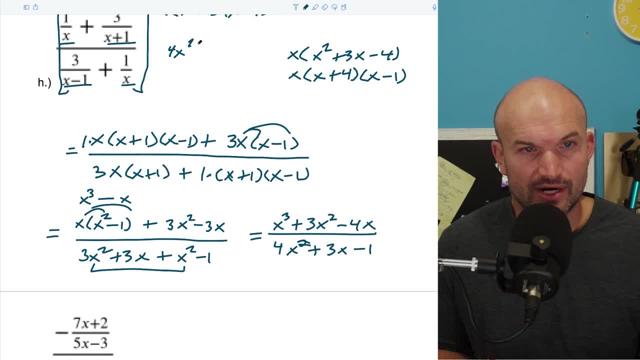 so could I rewrite this as a four X squared plus three X minus one? Okay, How could I factor that? Let's see, I could do a four X Times an X, And then if I did this at plus one, and then this would be a what a minus one. 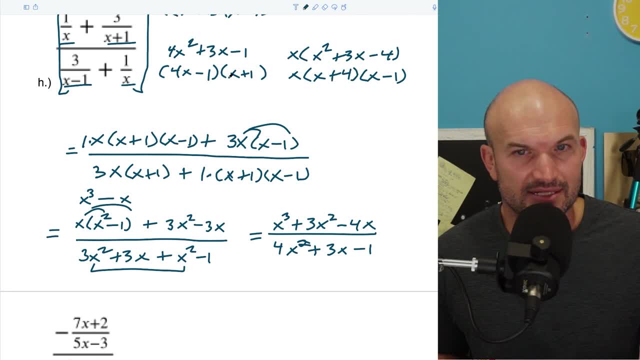 I think that would work. Yeah, There'd be four X and that'd be three X, but it's not going to divide anything out, Right? So that is going to be my final answer. You always want to see if something can divide out or simplify, Um, but in this case, thankfully, nothing is going to. that's not going. 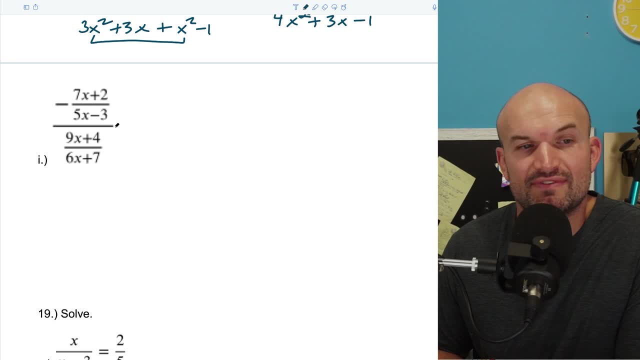 to happen. All right, And just remember. remember when we were dividing rational fractions, we multiply by the reciprocal. Yeah, That's exactly what we were doing here. You have a fraction divided by another fraction, right, This? like you could rewrite this as a division problem if you wanted to. right, You could just rewrite this. 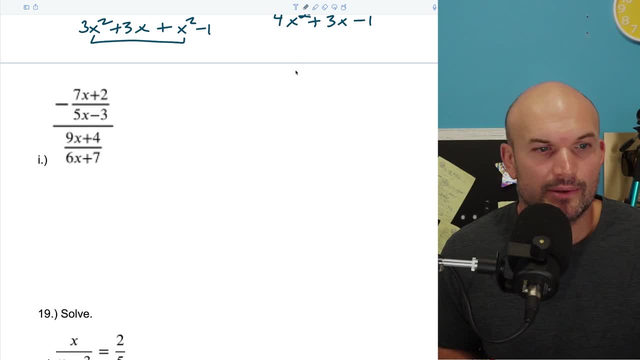 as a seven X. Oh, not, right, there, Let's start. Oh well, you could rewrite this as a seven X plus two, divided by five X minus three, divided by a nine X plus four, divided by a six X plus seven, Right, So just rewrite as a multiplication problem. So you just flip, multiply by the. 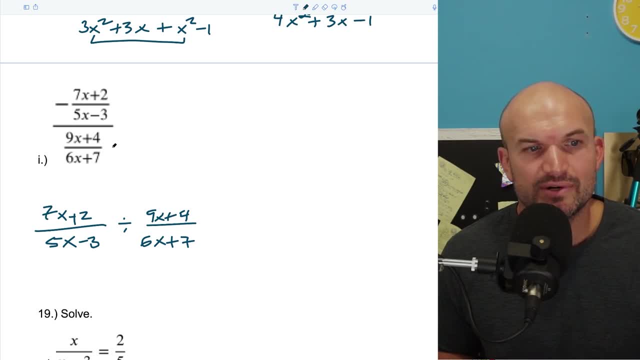 reciprocal right, And that's basically all we are simply doing here. And the reason why that works is when you multiply by the reciprocal. what does that do to the my denominator over here? that makes my denominator? that makes my denominator go to one right? That? 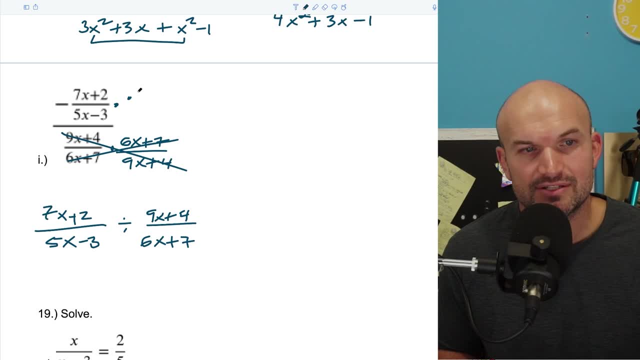 goes to one. So. but whatever you do in the new denominator, you also have to do in the numerator nine, X plus four. Now, nothing actually simplifies in this case. So what I'm going to actually do is actually have to multiply both of these out to using lovely foil. So let's go ahead and put: 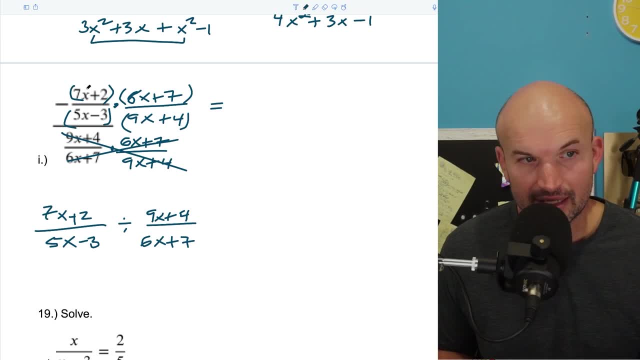 parentheses around everything and let's go and multiply it out Now. do remember that we have a negative Now. it doesn't matter if you put the negative up top or if you put the negative on the bottom. you could distribute the negative, but I'm just going to put the negative on the bottom. 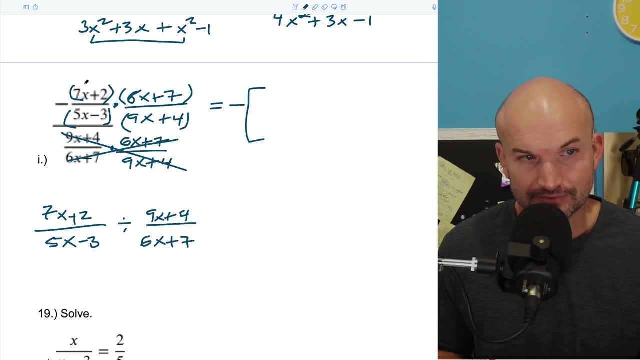 Leave everything that negative on the outside and do some math here. So seven X times six X is a 42 X, seven X times seven. I'm sorry, Let's do the inner, Let's do the X's first, for that's 42 X squared Seven X times seven is going to be a 49 X um six X plus six X times. 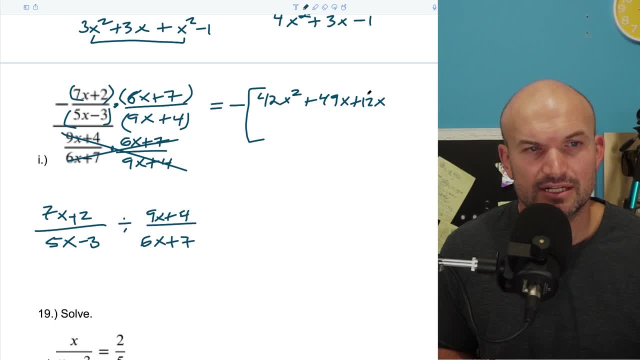 two is going to be a plus a 12 X, and two plus two times seven, I'm sorry, It's going to be a positive 14.. And then in my denominator here I have a five X times nine. X is a 45.. 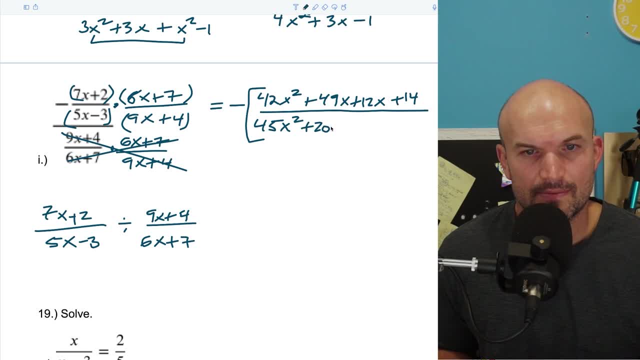 X squared. Um, I have a five times four is going to be a 20 X. Um, I have a nine. nine X times three is going to be a negative. 27 X right And negative. three times four is going to be a negative 12.. Cool, All right, So let's go ahead and combine our like terms here. 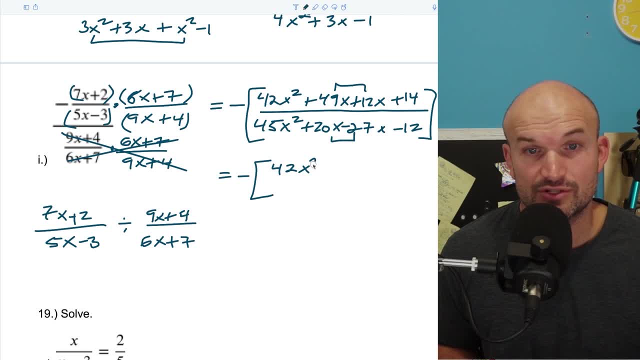 So, therefore, now I'm going to get a final answer of 42 X squared Um. let's see that's going to be plus a 61 X plus 14.. And then, over here, this is going to be a 45 X squared Um. and then, over here, this is going to be a 45 X squared Um. and then over here. 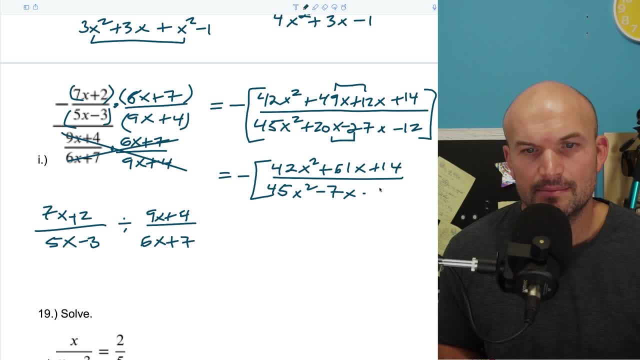 this is going to be a negative seven X minus 12.. Okay, Now we should also go and check to see if these are factorable. but these look like pretty difficult problems to go ahead and factor. I'd probably be sitting here for a little bit. I'm trying to see if they are factorable, So I am. 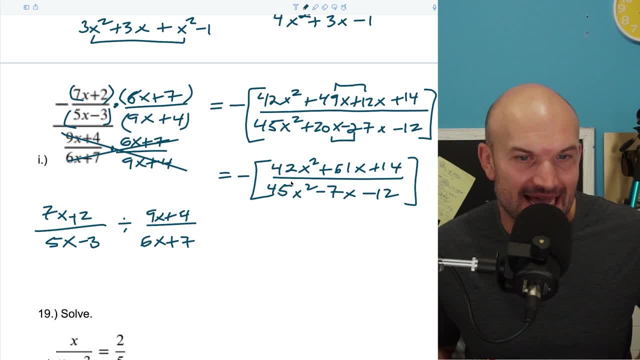 just going to leave the answer out like this. I personally, I would not even attempt to actually try to see if this is factorable um by myself. What I would simply do is go ahead and use graphing technology or, you know, some kind of computer system to be able to check if those are. 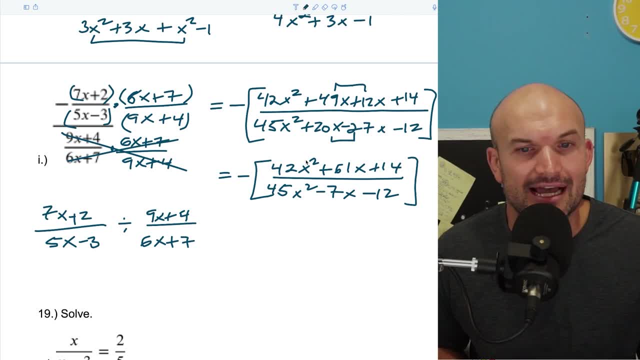 factorable and if it could be further simplified. I don't know, I don't know, I don't know. I don't think that's a great use of your time to be manually checking this, because this could be pretty crazy. Okay, But um, I'll just leave my answer as this, but just give a note: It could. 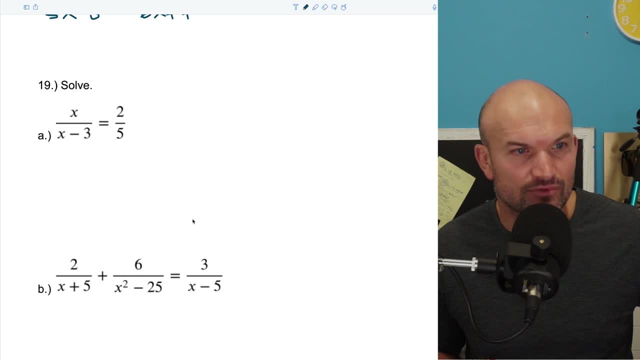 be simplified. All right, Now we're just going to solve on solving rational expressions. So when solving rational um equations, I'm sorry, we want to get rid of these denominators. right, I don't like denominators, Just like we didn't like the complex fractions. we got rid of the 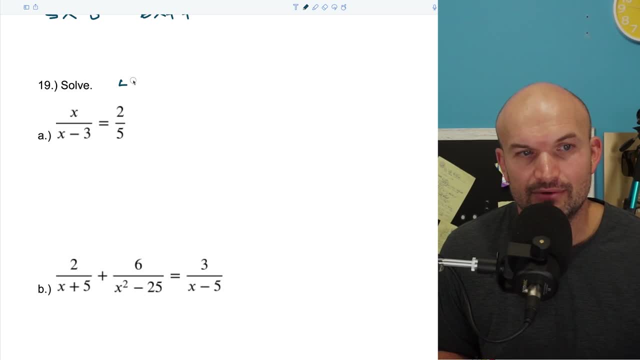 denominators. So in this case, what I usually like to tell students is: get rid of the denominators by multiplying everything by the LCD. So the quickest, fastest, easiest way to find the LCD is to just multiply everything by the LCD. So the quickest, fastest, easiest way to find the LCD is to 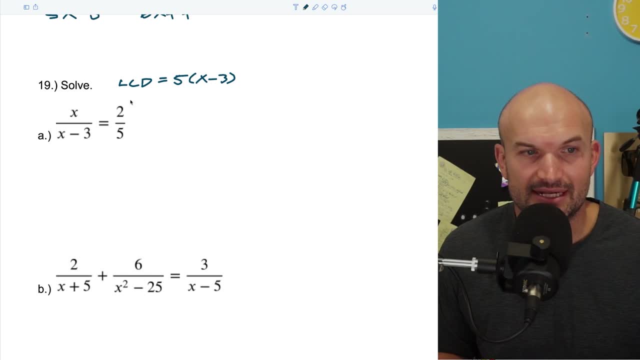 just multiply everything by the LCD. So the quickest, fastest, easiest way to find the LCD is to just multiply by your denominators. Now, that doesn't always work, which will happen in the next example, But in this example it does work, because five and X minus three do not share anything. 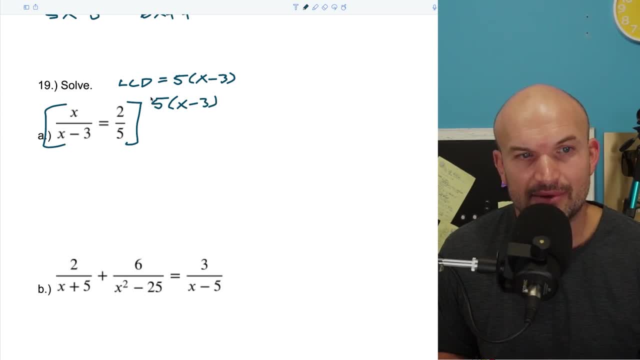 So, therefore, if I multiply by my LCD, which is a product of my denominators- and again we're going to multiply by everything You got to make sure you multiply everything to produce that equivalent equation. Um, that's now going to get rid of my denominator. So again, 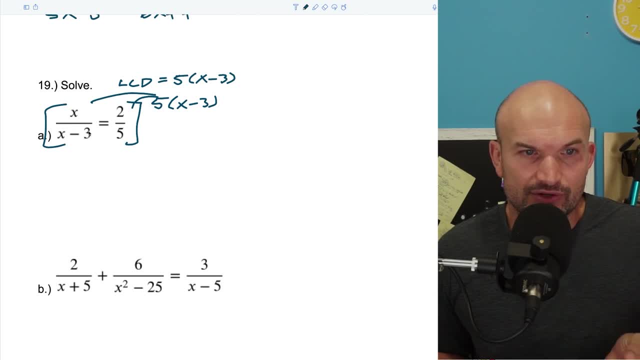 what I want you to do is like: well, as I multiply this through, X minus three is going to evenly divide into that, right? So that's going to leave me with a five times X. here The fives are going to divide out. That's going to leave me with a two X minus three. Well, now it's just a two-step. 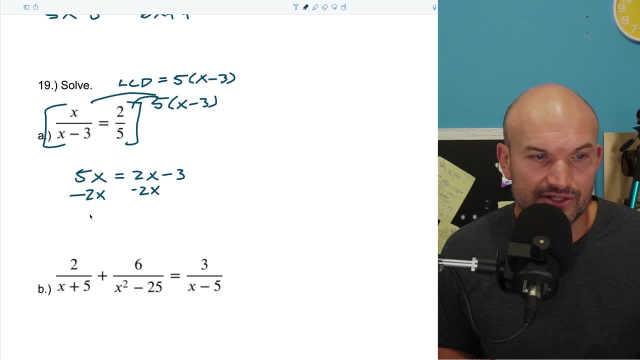 equation. So or not a two-step equation, but a? yeah, I guess it is two-step equation, So now I can just go ahead and solve. So, divide by three, divide by three and X is going to equal a negative one. However, we got to make sure that whatever our values are are not going to make 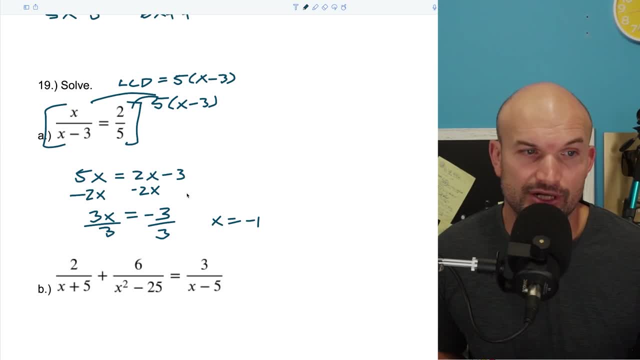 my denominator equal to zero, That would then be an extraneous solution. So the only value that would be extraneous in this case would be a three, And if I X equals negative one does not, it's not three. So therefore the solution works, but you will want to make sure, just like 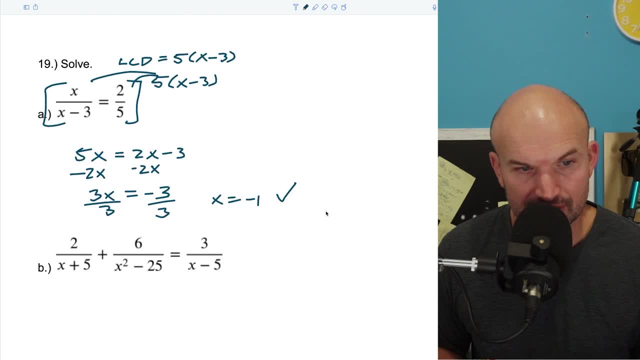 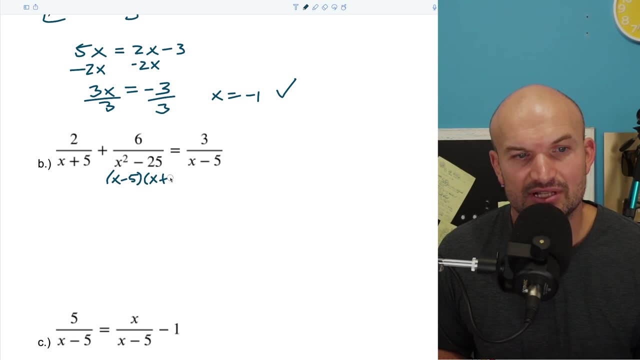 with logarithms, you will want to make sure you can check for extraneous solutions. Now, in this example again, I'm going to, I'm going to do is here: factor this: So this is X minus five times an X plus five. Okay, So now my LCD is not going to be X plus five times X minus. 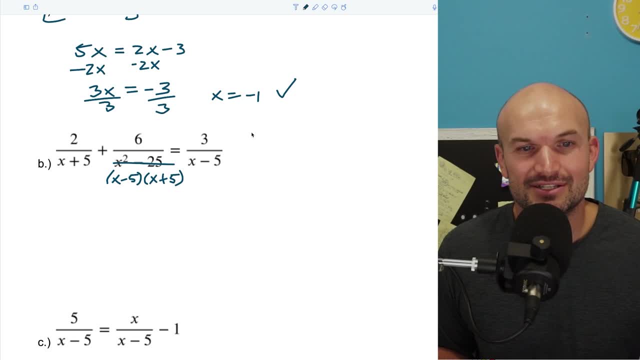 five times X plus five times X minus five. You don't want to do that. What you want to do is you only need to write them down once, So you just want to take into account what they share. So I have an X plus five is shared, right? So I just need one of them. 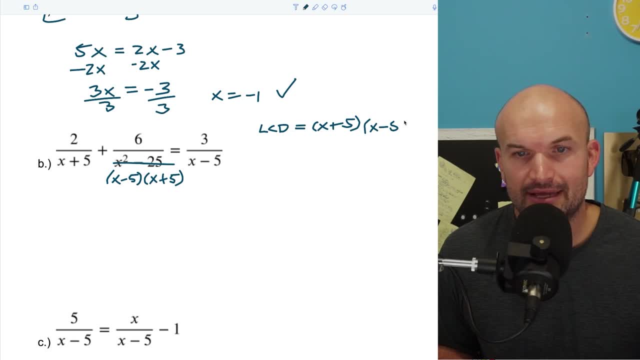 And then also an X minus five is shared. So again I just need one of them. Okay, So that's my LCD and I'm going to multiply everything times that LCD. Okay, Now again, I'm not going to show my work going through it, I'm just going to kind of mentally do it. So when I multiply an X minus, 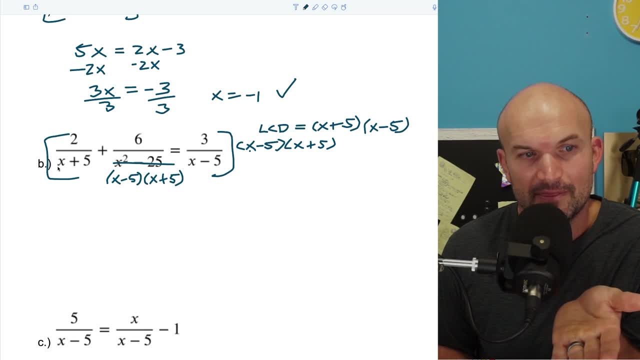 five times X plus five times a two over X plus five. the X plus fives divide out. That's just going to leave me with a two times an X minus five. over here, both my X minus fives and my X plus fives will divide it out. That's just going to leave me with a six, And then over here. 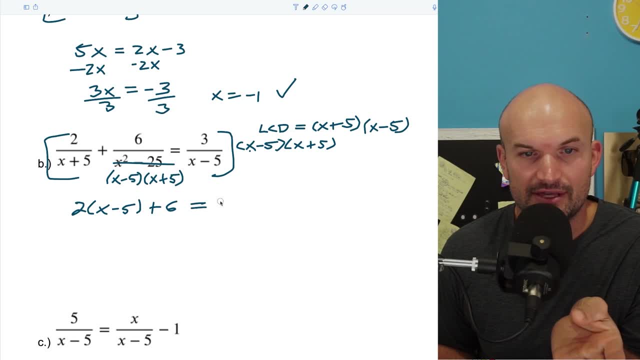 my X plus fives, X minus fives divide out, So that's just going to leave me with a three times an X plus five. Okay, So now I can just apply some good old distributive property. That's going to be: a two X minus 10 plus six equals a three X plus 15.. And then let's go. 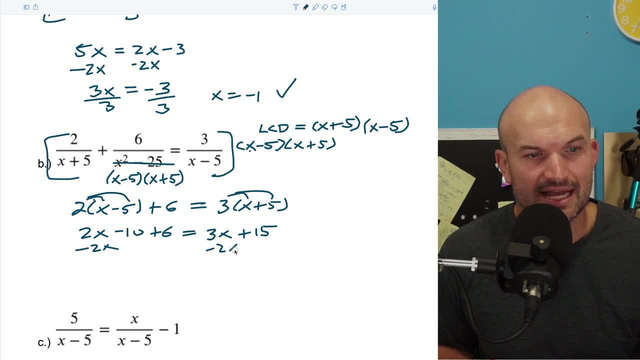 ahead and combine like terms. get my variable to the same side. This is going to be a negative four equals an X plus 15 minus a 15.. And therefore we can say negative 19 equals an X. Okay, And again we want to make sure that's not going to make any of my solutions extraneous, which in this case, 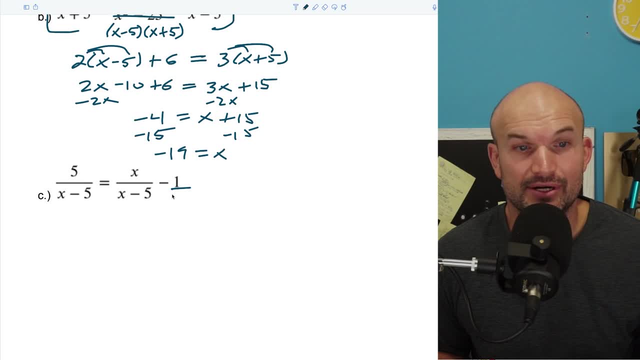 it does not In this case. we don't have a denominator here so you can rewrite that as over one. So hopefully you recognize here with my LCD is just going to be an X minus five. Okay, So LCD is equal to an X minus a five, And that's what I'm just going to. multiply everything by So X. 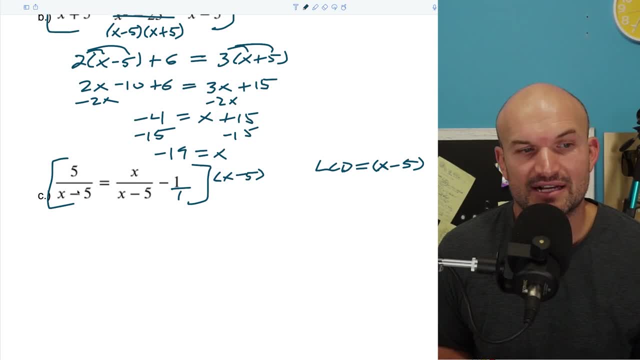 minus five. So when I multiply it times five over X minus five, I'm just going to have a five, right, The X minus fives will divide out. over here, X minus fives dot out, That's going to leave with an X, And then over here that's going to be minus a X minus five. 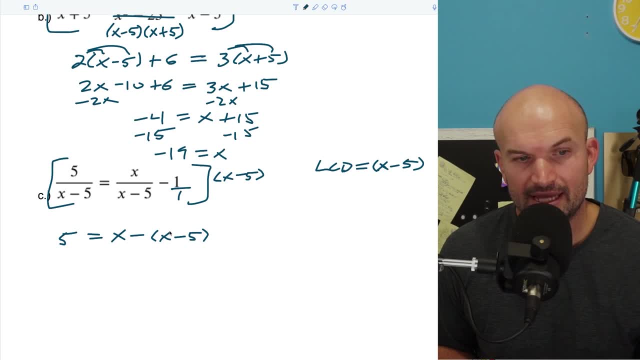 Again, notice how I use parentheses here. Students will make mistakes here, and they will. they will forget to use parentheses and they won't distribute. So we got to actually distribute in this case. So I get a five equals. a X minus X is going to be a zero minus five. Does five equal? 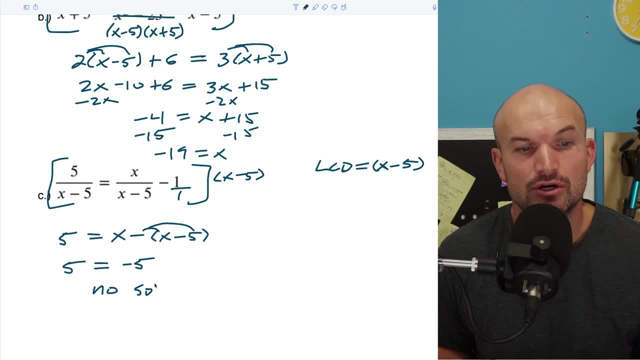 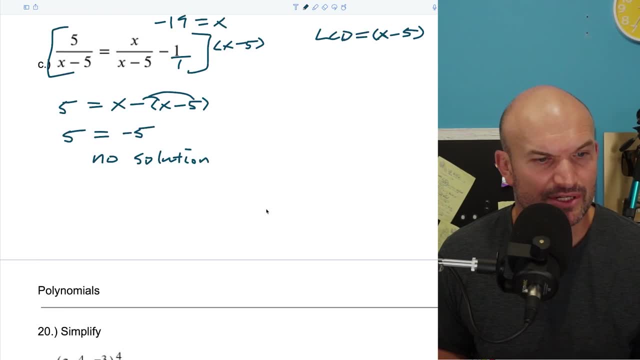 negative five No, So in this case we have no solution. Okay, So it is possible to have no solution for your rational function, as well as having like extraneous solutions which I guess I didn't provide any examples on. So, either way, 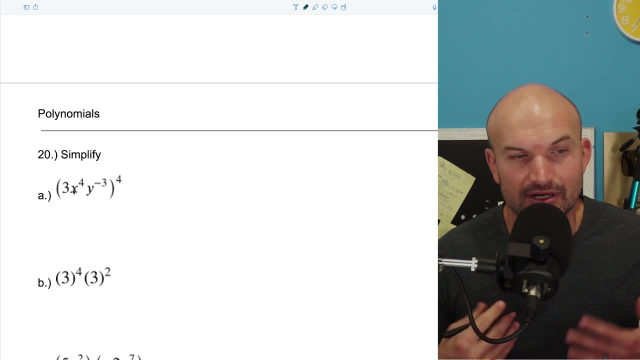 Um, all right, let's go and take a look at our polynomial. So one thing we're also going to want to work on is just using our rules of exponents. Okay, Um, so we're going to cover like a lot of. 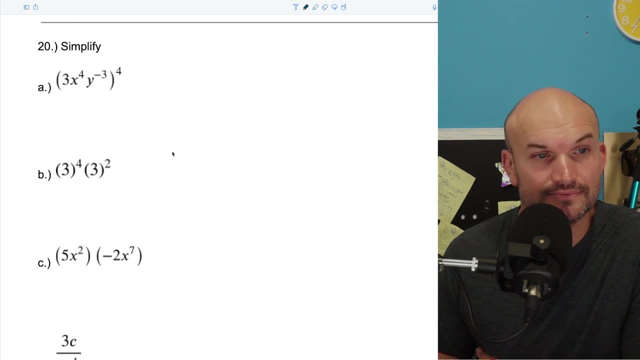 rules of exponents here and just kind of do a quick little good review for you. So the first thing um this one is going to be the power to product rule. So basically, whenever you have, as long as you have terms separated by multiplication, you can go ahead and distribute. 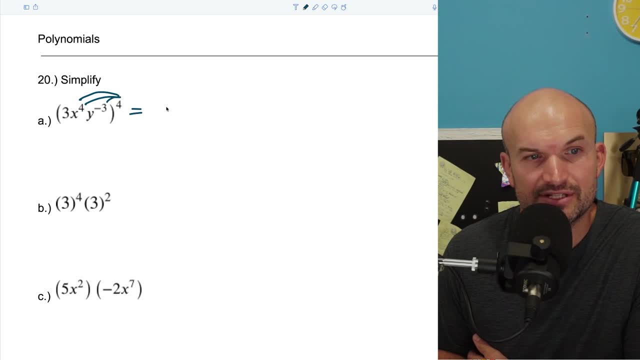 that power to each and every one of those terms. So in this case I have a three to the fourth power. So this basically can write it like this: three to the fourth power. I don't know why I wrote my X like that. Let's just go ahead. 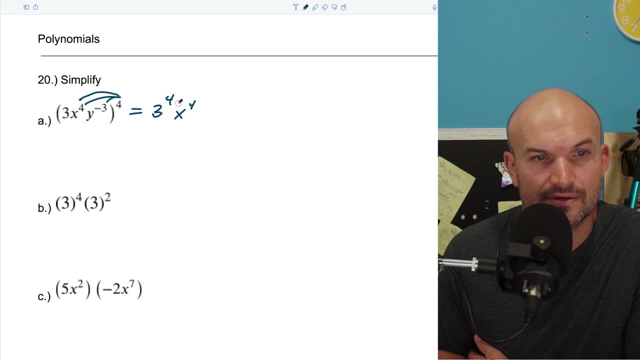 And delete that. So this would be a X to the fourth. Keep on forgetting things. So that'd be an X to the fourth. Let's try this again. There we go: X. three to the fourth times, X to the fourth. race to the fourth. 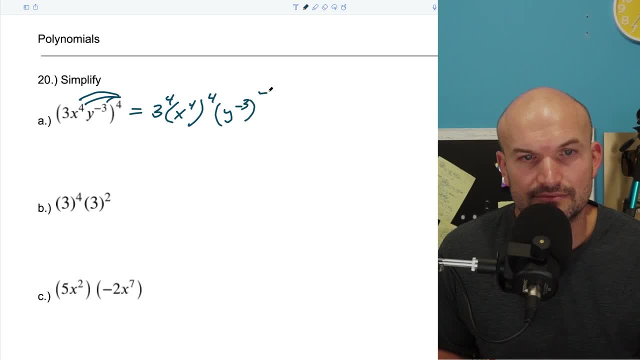 And then this would be a Y to the negative third. race to the fourth. Okay, So now, in this case, what we can basically do is not simplify. So, three to the fourth, power is going to be an 81, X to the fourth, race to the fourth is going to be an X to the 16th. Um, and then this would: 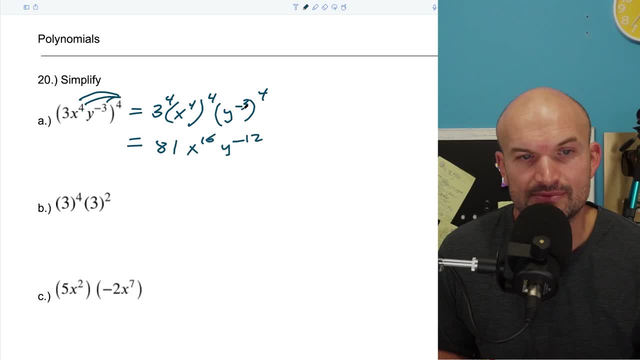 be a three to the fourth, times X to the fourth. raise to the fourth. be a y to the negative. 12th power. right, You multiply those powers And then just remember that whenever you have a negative power, you can rewrite that as a positive power by writing it as: 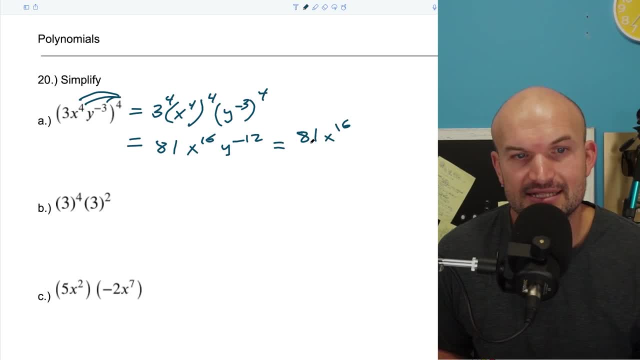 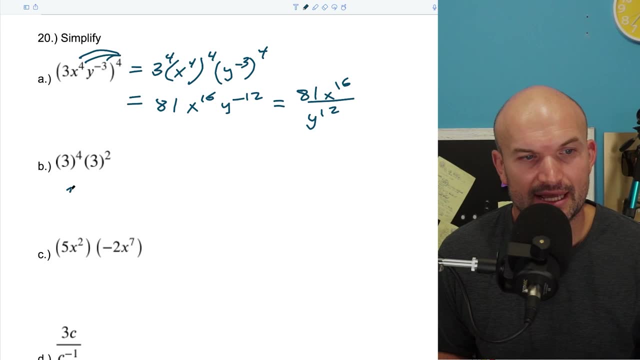 the reciprocal. So my final answer is an 81x to the 16th over a y to the positive 12th Over here. I'm just basically multiplying these, So this is going to be a 81 times a 9. And 81. 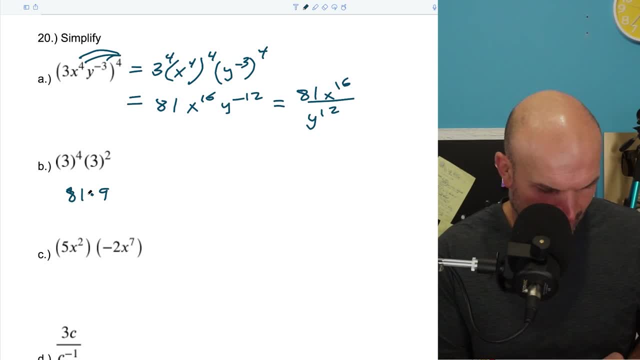 times 9 is- I should probably know this on top of my head or be able to do it, but I'm not really sure- So that'd be 720 times 9.. So yeah, that makes sense. So therefore, the answer is 729.. 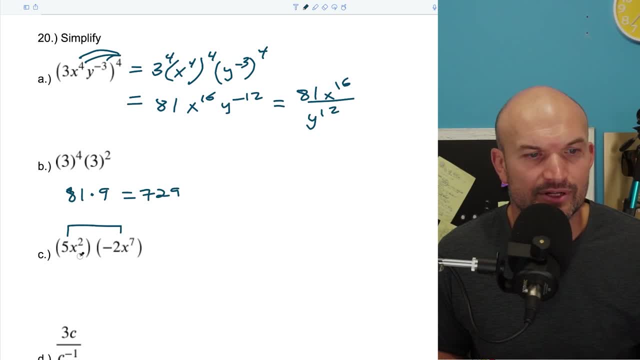 Now remember: when you're multiplying exponents, you multiply your numbers And you can multiply exponents as long as they have the same base. But remember you're going to add the powers. So therefore, this answer is going to be a negative 10.. And then 2 plus 7 is going to be a 9.. 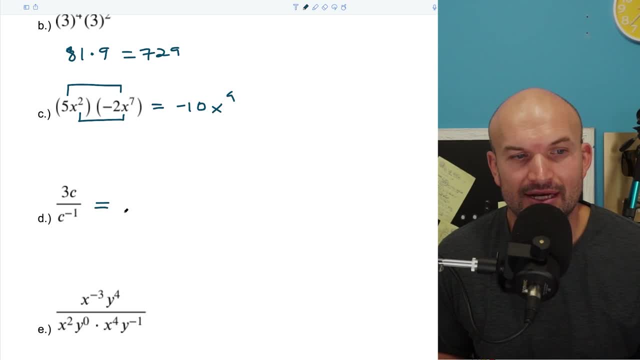 Over here. remember, I can rewrite this with a positive power by rewriting it as the reciprocal. So therefore I can say this is a 3c. Instead of dividing by a c to the negative first, I can multiply it by c to the first power. Well, 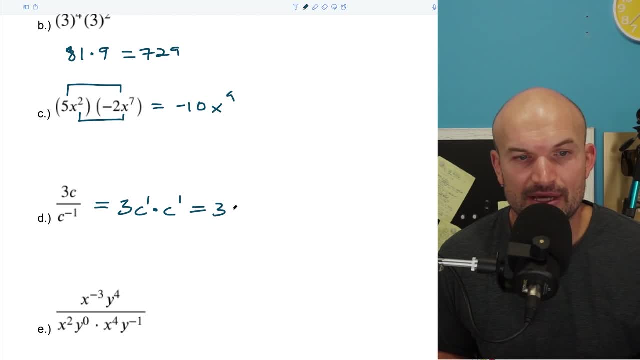 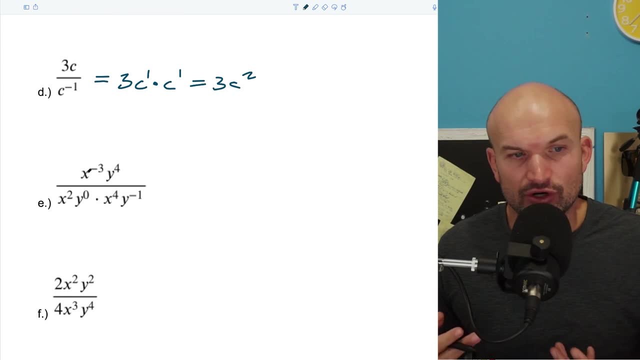 this is also being raised to the first power. So my final answer here is going to be a 3c squared. Now, on a problem like this, what I always like to do is kind of clean up the negatives and the zeros and then go ahead and simplify. So remember, whenever it's a negative, I can rewrite it as: 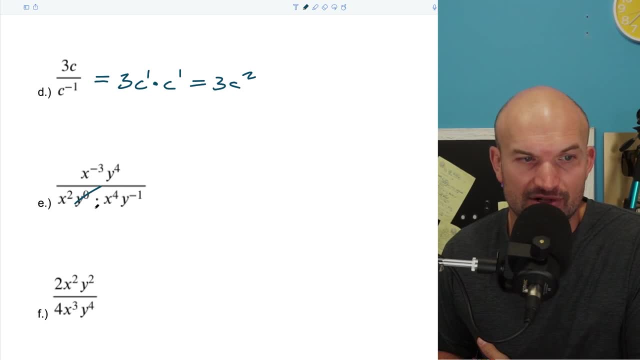 it's reciprocal with the positive power, And just remember: anything raised to zero power is just going to be 1, right, And so I don't really need to write it there. Okay, So now let's go ahead and write what I have here. That's just going to be the 1c, So I'm going to write the negative. 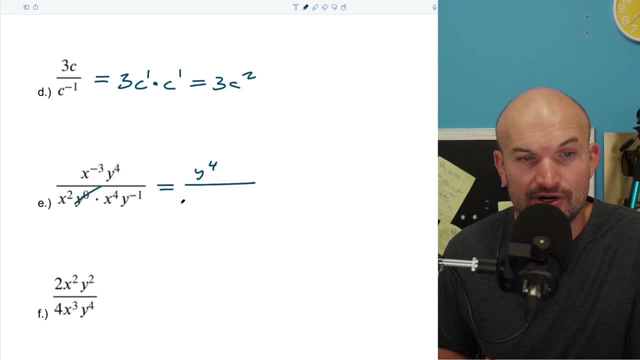 y to the fourth. I'm going to bring down these x to the third. Okay, Then I'm going to have this x squared. I'm going to have this x to the fourth, but then this y to the first. I can bring that up. 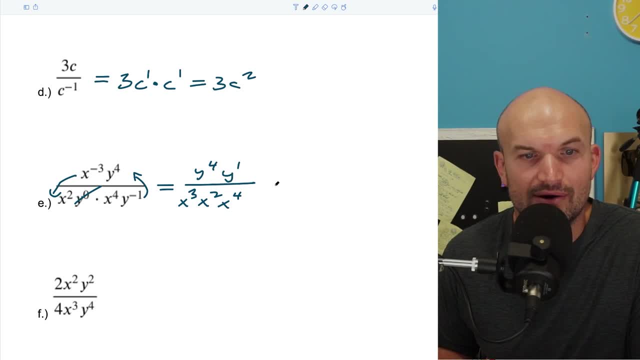 So basically, I just have two values that I can switch, and that'd be y to the first power. Now I can multiply them and add their powers, So this would be y to the fourth times y to the first, which would be a y to the fifth, And then this is going to be x cubed times x squared. 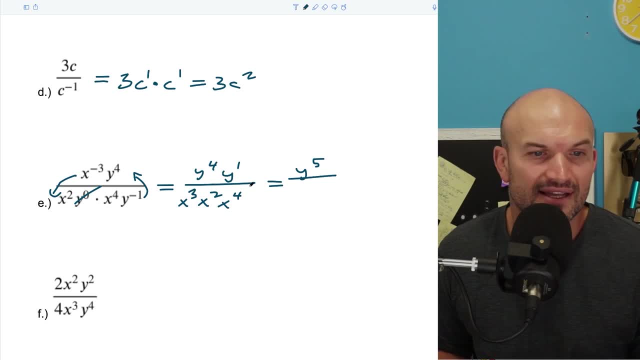 Sorry, Sorry, You're just adding the power. So three plus two plus four is going to be a x to the ninth power. All right, And then let's go over this one. Basically now, it's just going to be the quotient property. So the quotient property. remember when multiplication for the 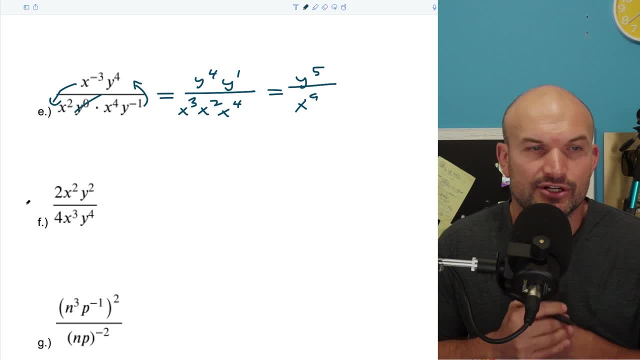 product property, you add the powers, right. So for the quotient property, basically you're just going to be subtracting the powers. So I have two over four, That's just going to equal a one fourth. And then I have a x squared divided by x cubed. I'm sorry, Let's subtract those, So that's. 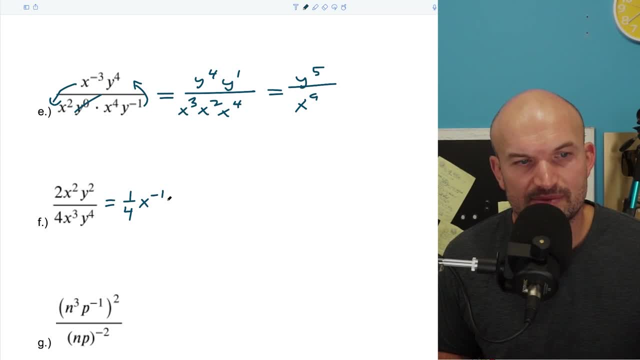 going to be an x to the negative first power And then two minus four is going to be a y to the negative second Right. So since these are negative right, these are technically in the numerator right Cause I just provided that power. So to write this correctly, I need to write these in. 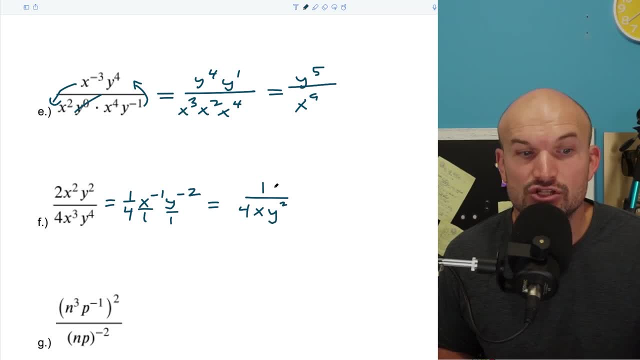 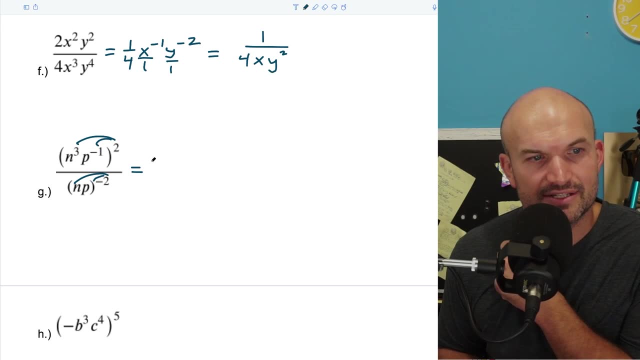 the denominator. So it'd be a four times x, y squared. Uh, and this problem. we need to use the power to product, rule first, rule first, and then we'll just go and simplify. So let's see, remember the power product you're going to multiply your powers, right And when you have. 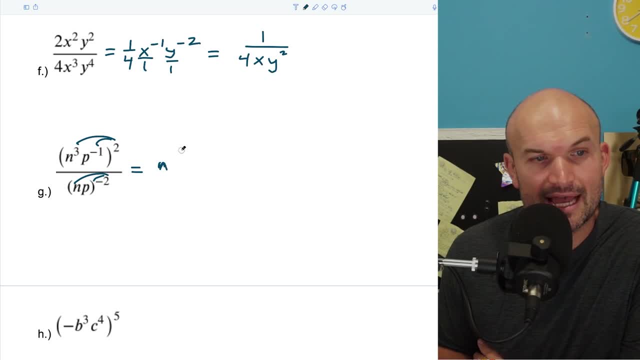 an exponent raised to a power you multiply. So this is going to be a n cubed times p to the negative second power. Um, this is going to be a n to the negative second power. So this is going to be a n to the negative second power and a p to the negative second power. Well, what do we know? 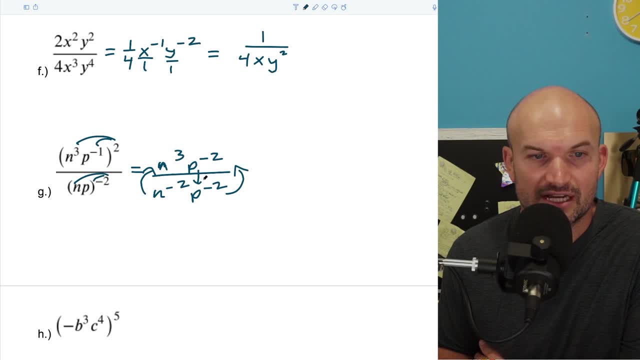 about the negative second power. We can bring those up and then this p to the negative second power, we're going to bring down Um. but notice before we have a niche to do that whenever you have an exponent raised to a power, that's exactly the same in the numerator and denominator. What's? 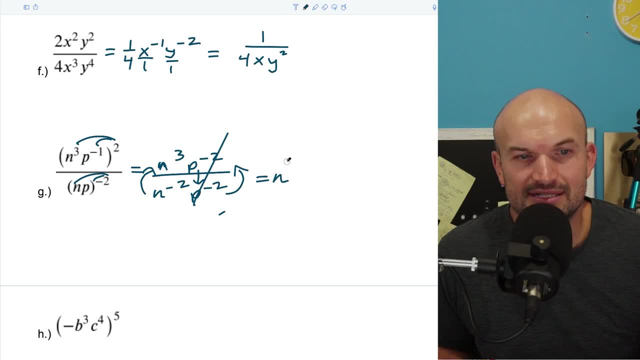 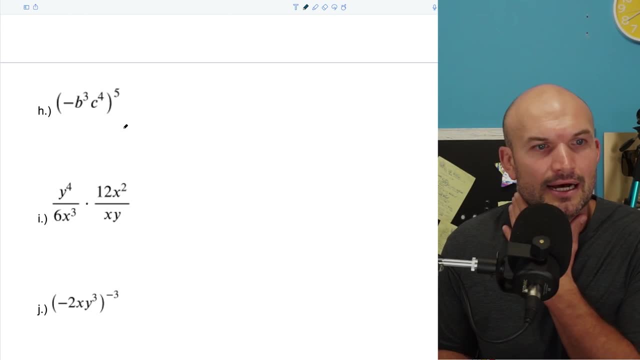 going to happen. Those are just going to divide out, right? So really, what I have here is an n cubed times an n squared, which is just going to equal a n to the fifth power. Um, over here, I'm just going to go ahead and distribute, So, um, now here's an important thing. 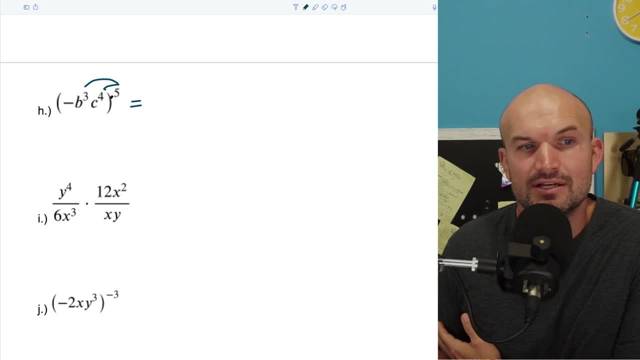 Is I have a negative b to the fifth power, right. So what's really important here is you can actually rewrite this as a negative one times a, b to the third power and c to the fourth power. Okay, And that's all being raised to the fifth power. So, technically, what we're doing here is we're raising. 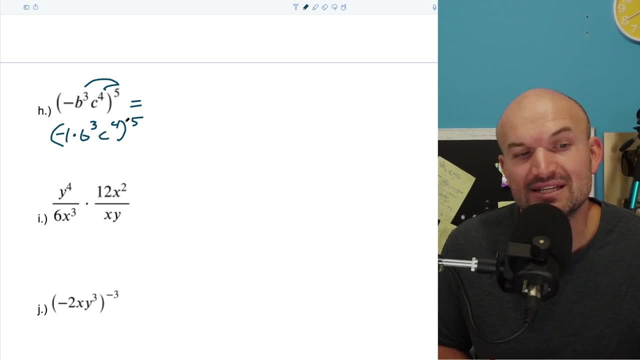 the negative one to the fifth power. So everything's still going to be negative, but if it wasn't, even power. you just want to be aware of that, Okay, Um, all right, So now what we're going to do is: what else are we going to do? Yeah, Just raising the power. So, therefore, 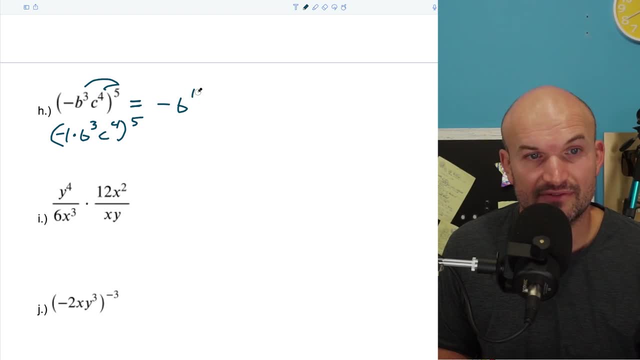 it's going to be a negative. Now, remember, we're going to multiply these, So that's going to be to the 15th. This would be a c to the 20th power And I think, yeah, everything's good. Um, over here. 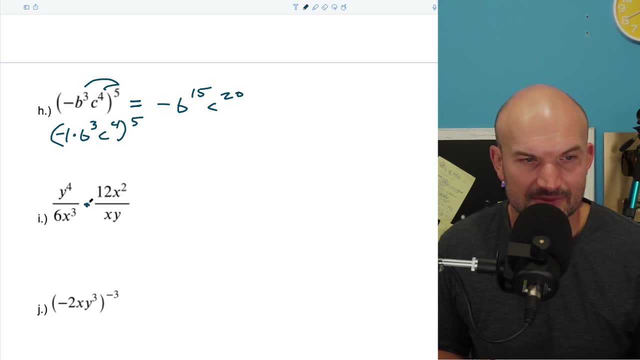 we're going to multiply. Now, the cool thing about this is, when you're multiplying these exponents, since everything's separated by multiplication, you can actually just do the work Like you can just write it as one, as one, like X expression, right. So 12 X squared Y to 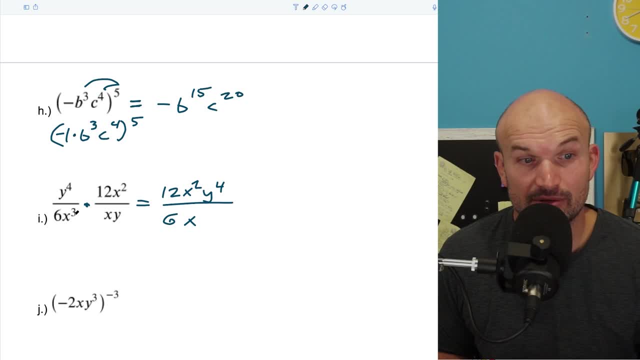 the fourth all over a six X, So you can multiply these. That'd be X to the fourth Y. Okay, Now let's just go ahead and simplify. Now another way to do it, rather than like subtracting and getting negative exponents. 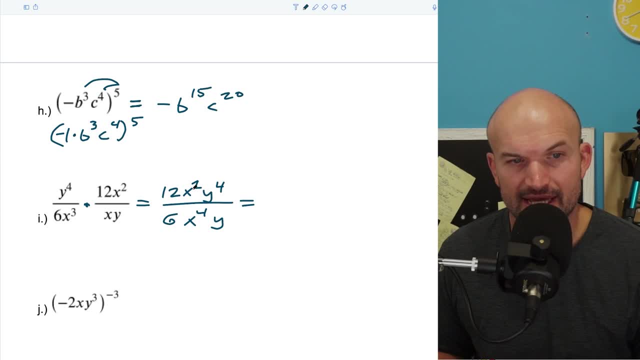 and dividing um. what you can do is just like re reduce everything. How it is Like, if I have X squared over X to the fourth, like I can divide it to on both sides, That's going to give me a um. sorry, if you divide it. let me think about it another way. Yeah, If you divide out a. 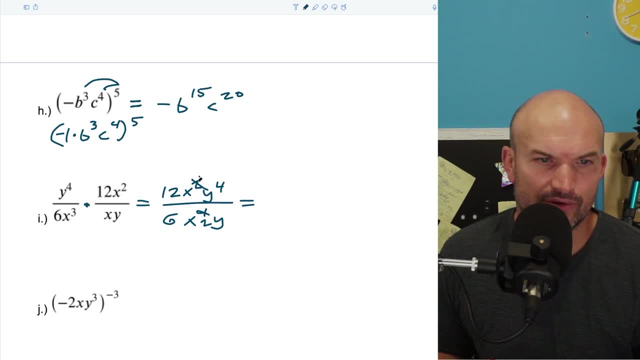 if you do it at a two, that'd be a two and or you got. it's not really dividing out the cancel. You're basically like canceling out those terms. So the way I explain that was kind of confusing. So it'd be X to the fourth, Okay, So basically I have an X times X. 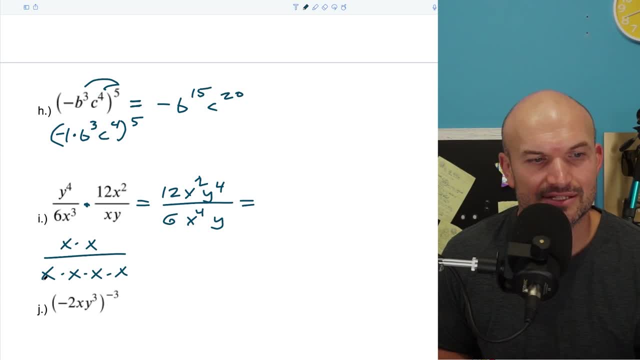 right over an X times X times X times X right. So those two are going to be divided out. Leave me with just an X squared in the denominator Um, 12 or six that can be divided to a two over one Right Um, and then a Y fourth over Y to the first power. I can divide out one Y on the top. 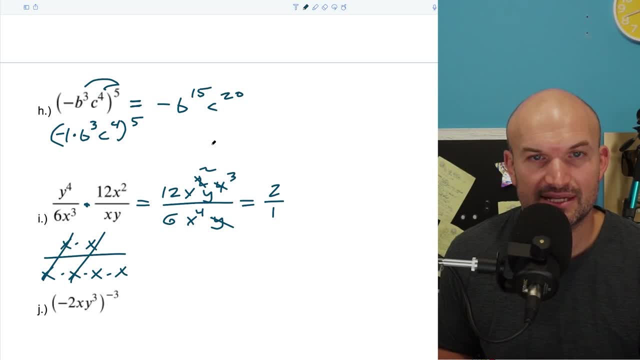 and bottom. That's going to give me a three, So I can divide out two of those. Um, that's going to give me a zero actually. So when I divide out a squared, that's going to go like that. That's going to go like that. 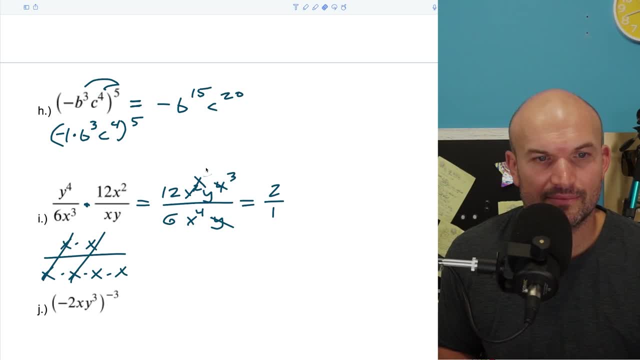 That's going to leave me at the two. Uh, that's going to give me a zero. Man, I'm having trouble here. That's going to be zero and that's going to be two. Okay, So now what I'm going to have is X to. 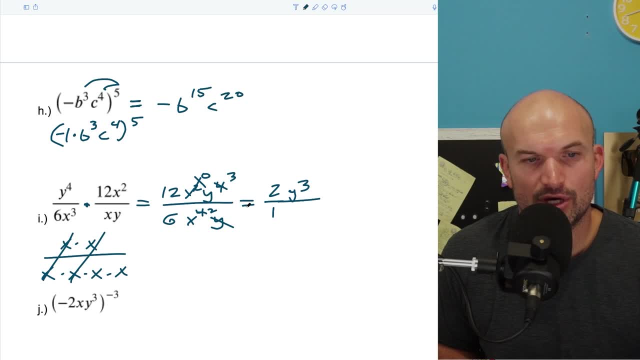 zero, which is just one. So that'd be Y cubed, And then that's going to be all over. that reduces to a two over one, Um, and then this is going to be a X squared. So my final answer: I'll just write a. 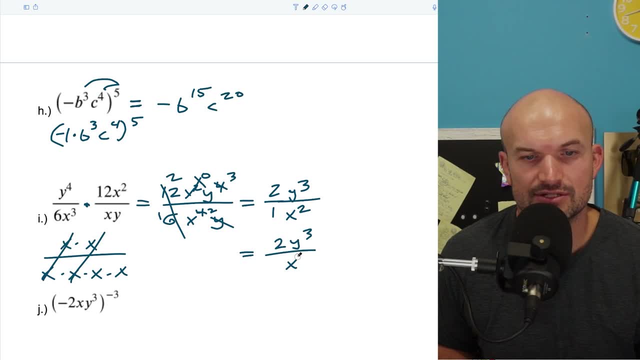 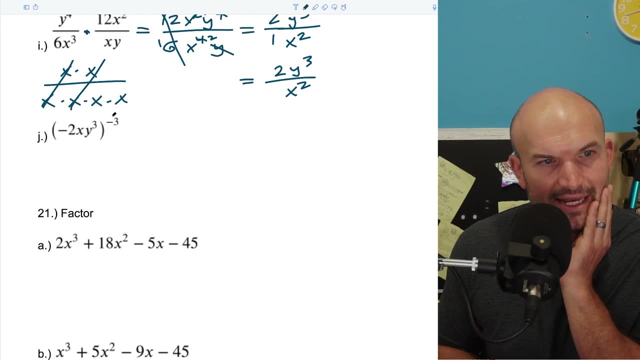 little bit better is going to be a two Y cubed over X squared, Okay, Um, another. another one over here is: go ahead and again distribute. Okay, Now, um, again. that's going to be a. this is really important, though, because what I want you to understand is like this negative here: 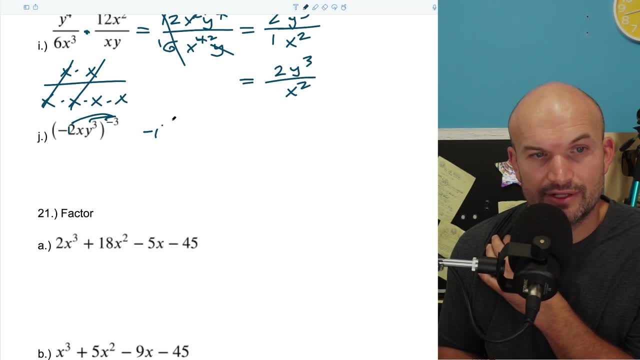 this is a negative one, right? So that's a negative one to the negative third power times a two to the negative third power times an X to negative third power times a Y to negative third power. I'm sorry, I said that wrong. That's a. let me do this. It's a um, so I have the two. 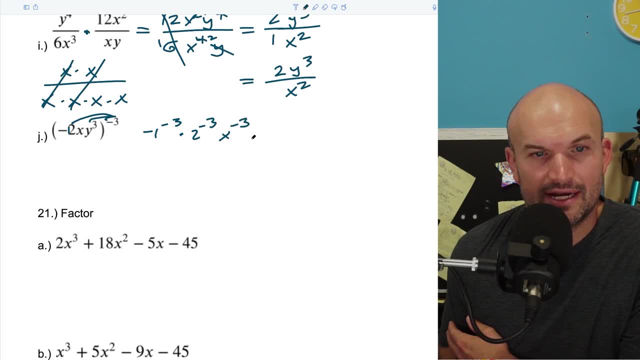 raised to the negative third power. That's an X to the negative third power, right, And that's a Y cubed to negative third power. Okay, So Y negative one to the negative third power is going to be a one over negative one, which is still just a negative. So it doesn't matter where you put it. 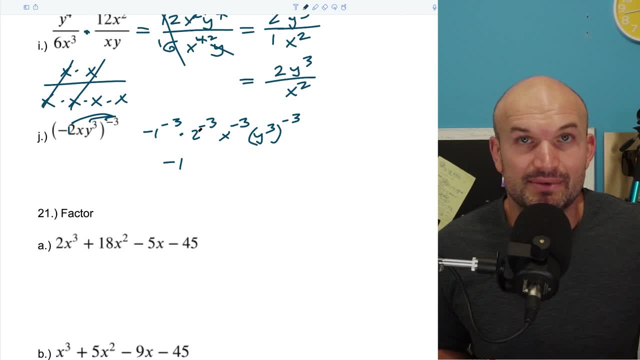 We can just put that in the numerator right, Um, but over here this is going to be two to negative. third power is going to be a one over eight, here is going to be a one over X And here is going to be a one over sorry times, a one over nine. So therefore, my final answer is nine times. 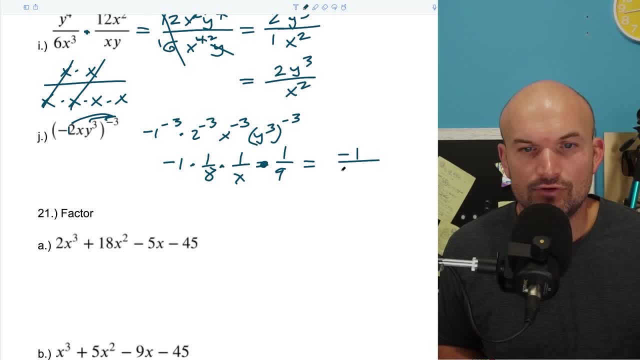 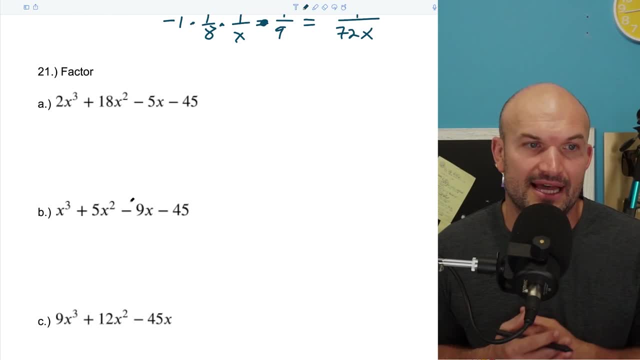 eight, It's going to be a 72. So, therefore, this is going to be a negative one over a 72 X. Okay, So now let's get into factoring some polynomials, And this is definitely something that you are going to want to make sure you are familiar with with um factoring polynomial, uh, factoring polynomials. 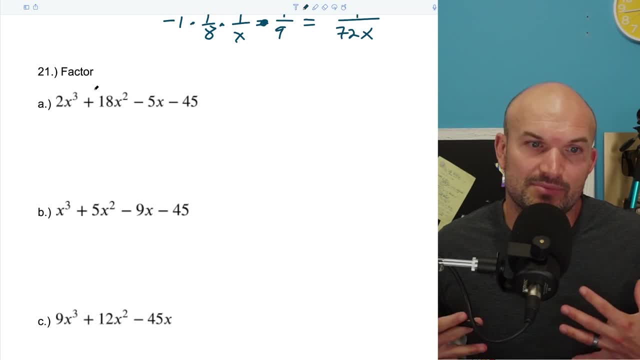 So, whenever you have four terms- right, we talked about factoring quadratics- That should be like a staple of of your your ability, like your math up to this point. But when you have four terms, what we're going to want to do is look for grouping. So when you're doing grouping, 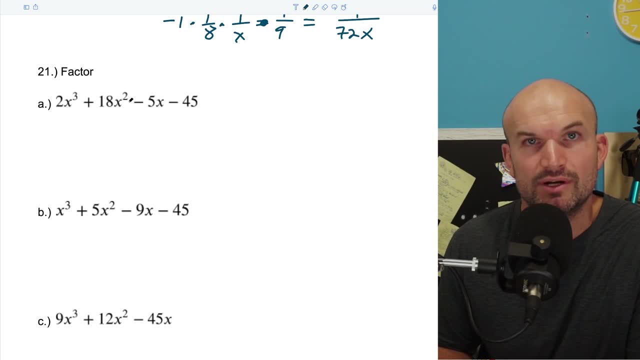 the main thing you want to do here is just kind of rewrite this Like you understand. like subtraction can be the same thing written as like an addition problem, right, Plus a negative is the same thing as subtracting, right. So if I say five minus four, that's the same thing as five. 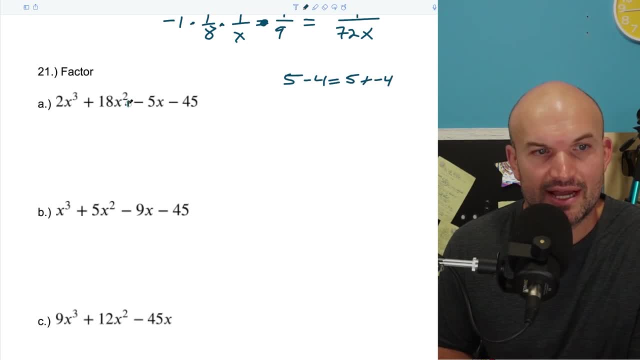 plus a negative four. So what I'm going to do, just to be mathematically correct, I'm going to write this as plus a negative five, X. All right, Then, what you're going to do is you're going to group the first two terms and then group the last two terms. All right, Then what we want to do is: 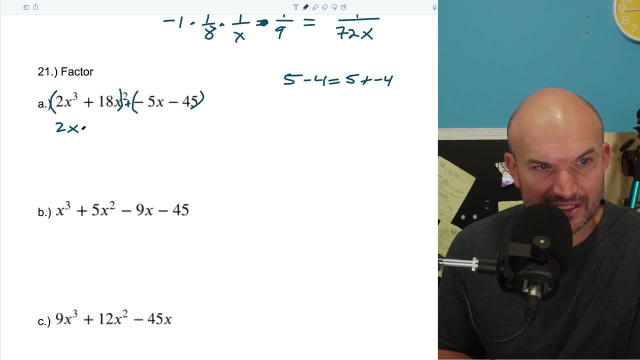 factor out what these have in common. So in this case they have a two X in common. So that's going to leave you with a X squared. So that's going to leave you with a X squared. So that's going to leave. 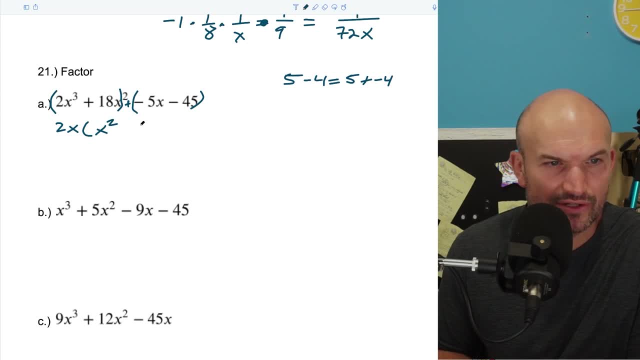 an X squared plus nine, And then over here I can factor out a. that's not an X squared, That's just an X going crazy, Okay. So then over here I can factor out a negative five, and that's going to leave me with an X plus nine. So when factoring by grouping, these two terms have to actually be. 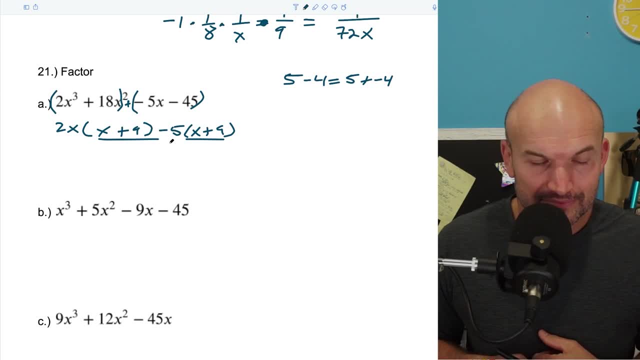 the same, because otherwise then you cannot factor by grouping or it might not be factorable. So, since these are both the same and both these expressions, do you see I have an expression here and then I have an expression here? They're separated by subtraction, So they're. 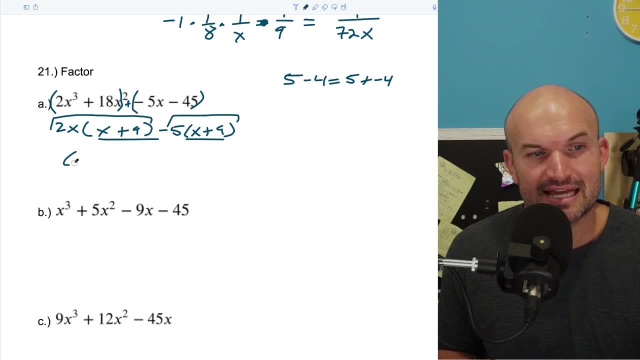 different expressions, but they both share an X plus nine. So what that means is I can factor out an X plus nine and what's going to be left over. What's going to be left over is a two X minus five, And that is going to be your factor form. So let's go ahead and do that again. So in 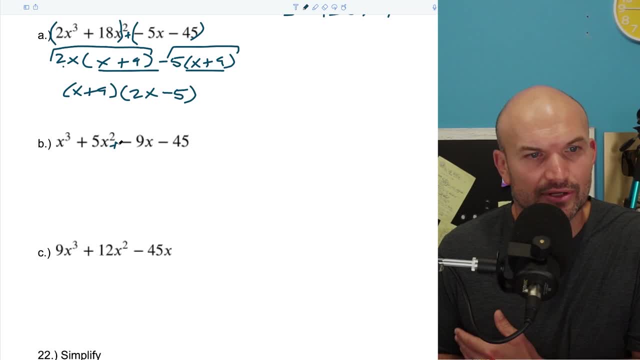 this case I have X, Q plus five, X squared, And I'll just say: put a little plus there, minus the nine, X minus 45. So again, group those, group those. All right. What do these have in common? They both have an X, So that's going to be a X, X plus five. I'm sorry, Yeah, X plus five. 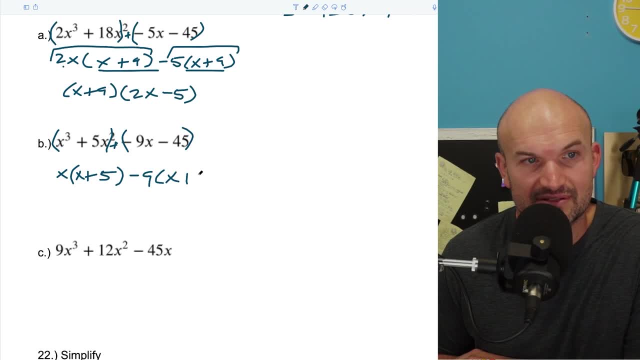 And then over here I can factor out a nine and that's going to leave with an X plus five. Okay, Again, they share the same thing. So you factor out the X plus five and that's going to leave you with a X minus a nine. Now here we have a trinomial right. So again, you always want to. 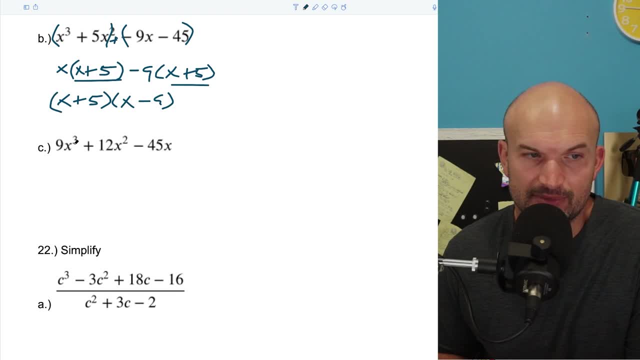 be able to see. what can you factor out? Well, how do you factor out something raised to the third power, Who has it as a trinomial? Well, again, you can factor out this X, and also I can factor out a three. I can't factor out a nine, because nine doesn't even divide in 12. It doesn't go. 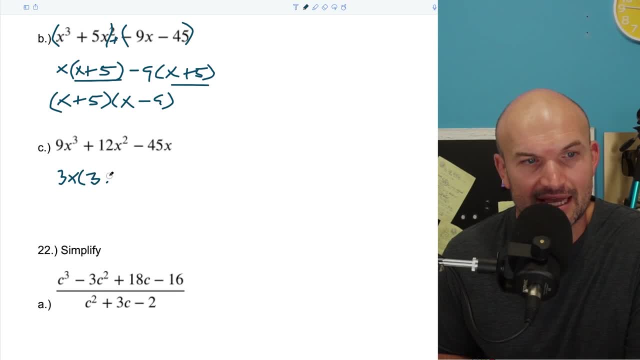 out, I can factor out a three. So by factor on a three X, I'm now going to be left with a three X squared plus a four X, And then let's see that's going to be a minus a 15. Cool, All right, Now we. 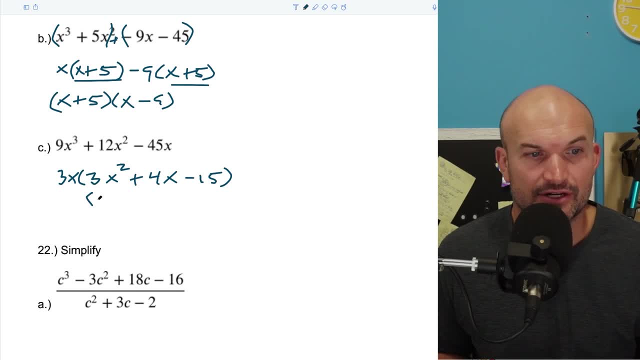 want to see: is this factorable? right Now we want to go back to what we learned in factoring quadratics. So I want to say, all right, I can break this up. do a product, two binomials. 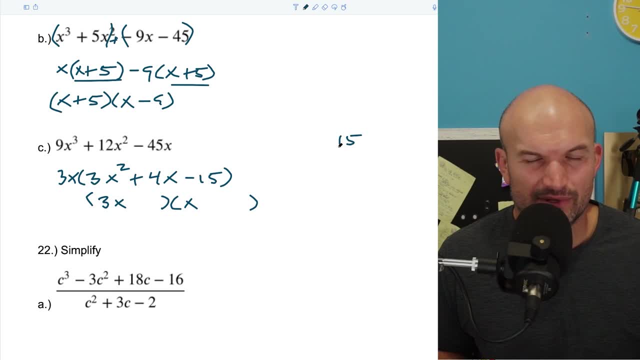 I need two numbers are going to multiply to give me 15.. So we have some options here. I don't want to use 15.. I'm probably going to use five and three, And am I going to get a, a difference of four? Well, if I did three times three, that's nine, And then with five, 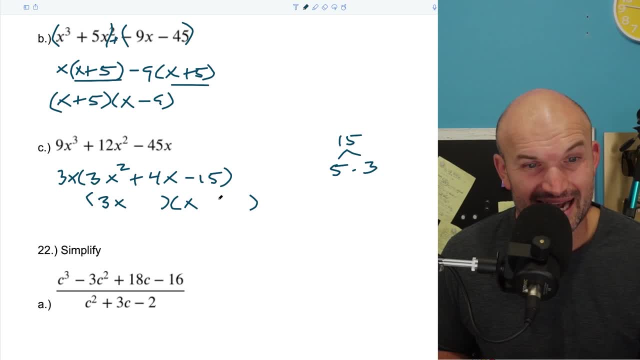 that'd give me a difference of four, right, So I want this to be a positive, and then this would be minus five. So three X times three X is nine X. that works. That's four X. So that's positive. four X, Perfect, And that gives me negative 15.. Cool, And that'd be multiplied by three X, And 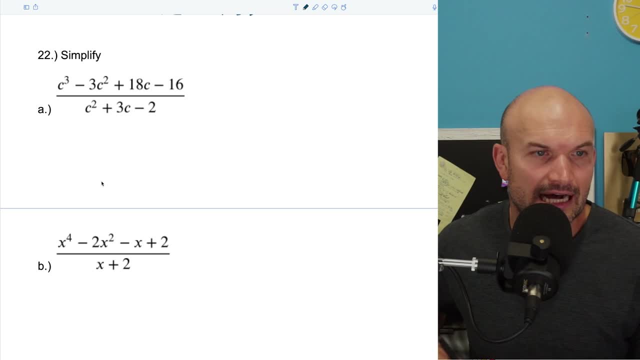 that's going to be my simplified answer. All right, Now we're going to get into long division. So, if you recall or remember, we got to remember how to do division with polynomials. okay, So when we're doing division with polynomials, um, the main thing that the 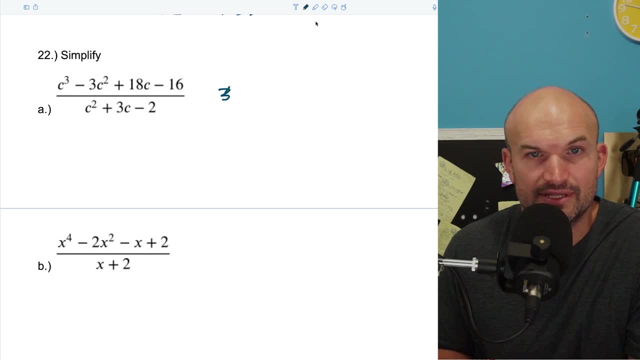 main thing we're going to undo is um set up the long division algorithm. So in this case I'm going to divide here. So I'll do is I'll take a C squared plus a three C minus two, And then I'll have a C squared minus three C squared plus a 18 C minus 16.. Okay, So for long. 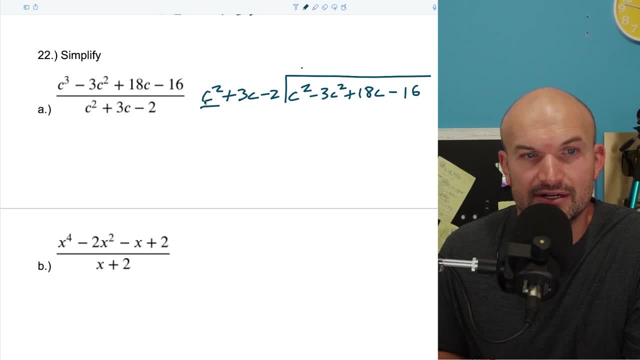 division. we're going to take the first term divided into the first term of our divisor. here C squared goes into C squared. How many times? Um, that's just going to be a one time. So then one times C squared and then one times three C. 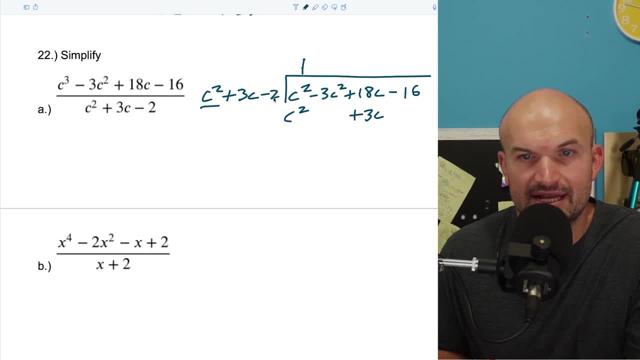 So that's going to be a positive three C, and then a one times negative two, And I'll write that over here. Um, I don't have anything here, so I can just write a zero C squared if I need to Now. 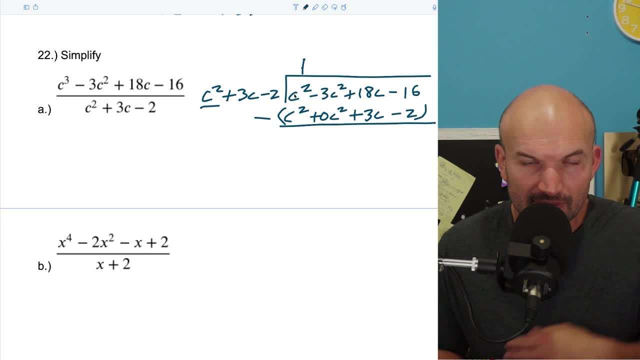 what I'm going to do is go ahead and subtract by two rows Um. so C squared minus C squared, it's just going to be zero C squared, which is zero negative three C minus a zero. So basically you can just bring this down. So that's going to be a negative three C squared Um. 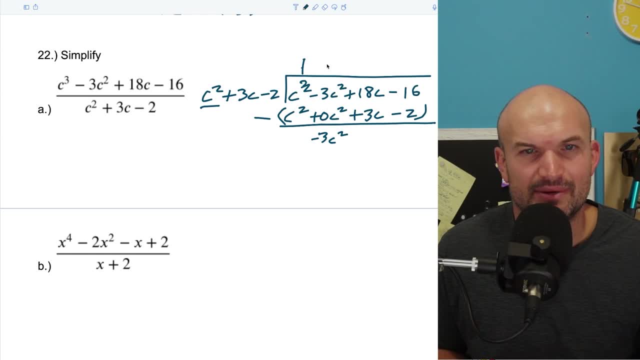 just goes in there. Oh, that was C cubed. No, I was wondering like, why did that not make sense? This is all wrong. Let's go ahead and redo that. Um, it's like not one. that doesn't make sense. 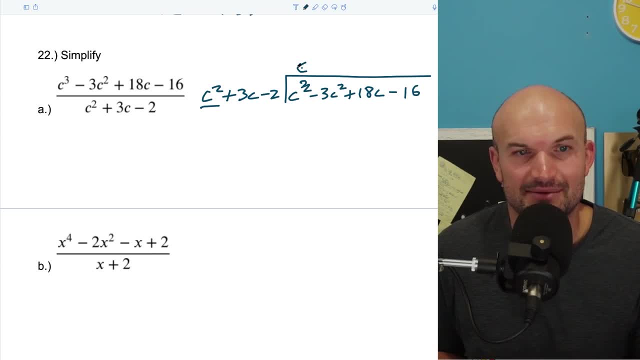 That's C cubed, C squared goes into C cubed a C number of times. So therefore, this gives me C cubed C times a three C is going to be a positive three C squared and C times negative two is going to be a negative um two C. Okay, Now let's bring this down, since there's nothing with the 16. I can. 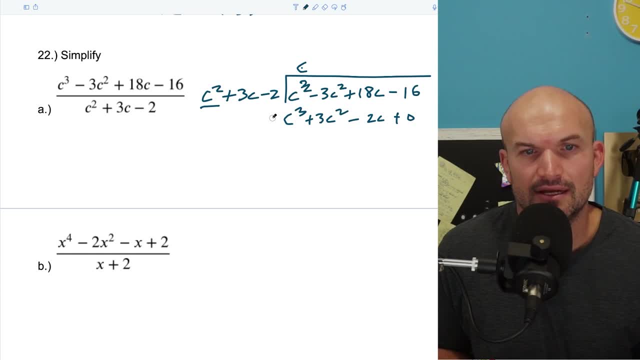 just, uh, I can just put a zero here, um, as a place value. Okay, So now let's go and subtract our rows. So C cubed minus C cubed, it's just gonna be zero negative. three C squared minus a three C squared right, It's going to be a negative six C squared. 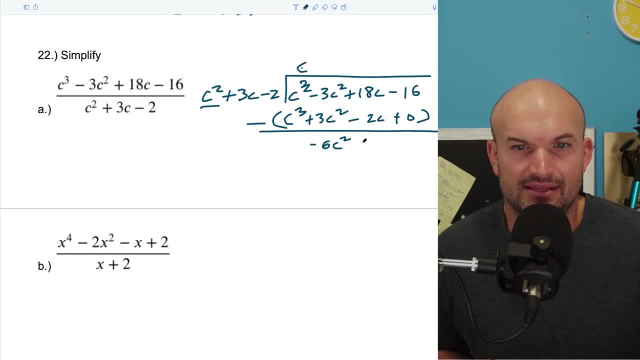 Um 18 C minus a negative two C is going to be a. let's see that's gonna be positive 20 C and negative 16 minus zero. It's just gonna be negative 16.. Okay, So now let's just do it all. 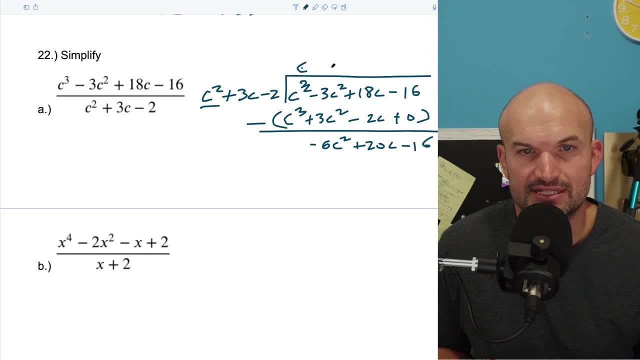 over again. How many times does C squared go into a negative? six C squared, Well, that's just gonna be a negative. six times negative. six times C squared, It's going to be a negative. six C squared: negative six. Six times three is going to be a negative. 18 C and negative six times two is going to be a positive. 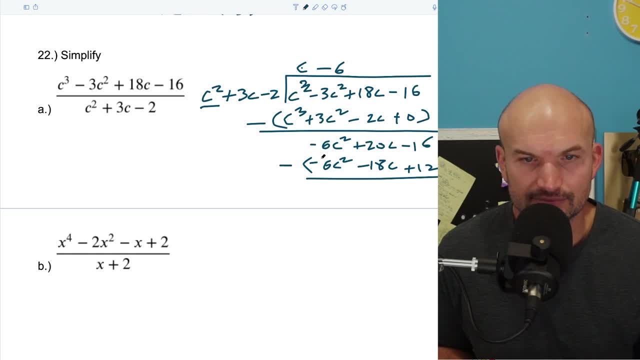 12.. Okay, And again we're just going to subtract our rows here. That goes to zero, that goes to a 38 C and this is negative. 16 minus 12 is going to be a negative 18.. Okay, So that is going to be. 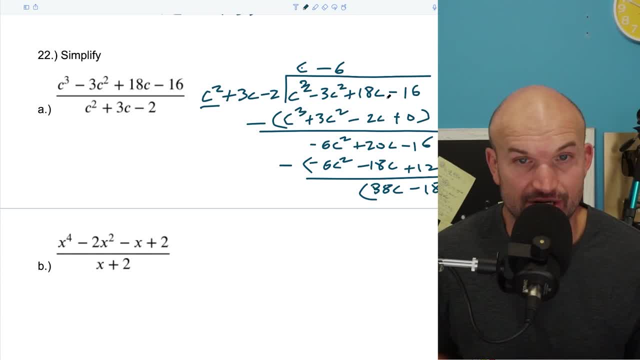 what we call this answer right here is going to be what we'll call our remainder. So here's our, our quotient, So we can write it as a final answer of C minus six plus a 38, C minus 18.. All over your divisor, which is a C squared plus a three, C minus a two. Okay, So that's the long. 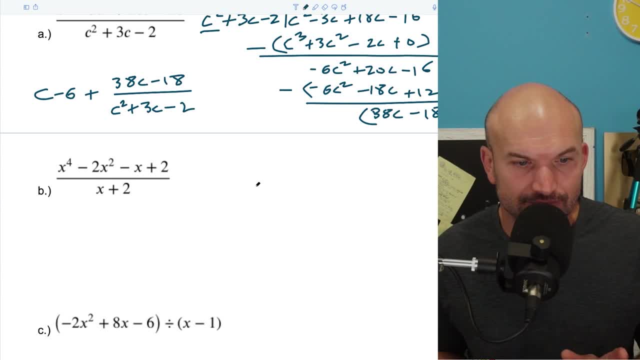 division algorithm. You're going to want to, you're going to need to know the long division algorithm, but you're also going to want to make sure you remember synthetic division, and for synthetic division, basically, all we simply need to do is just take a set, our divisor. 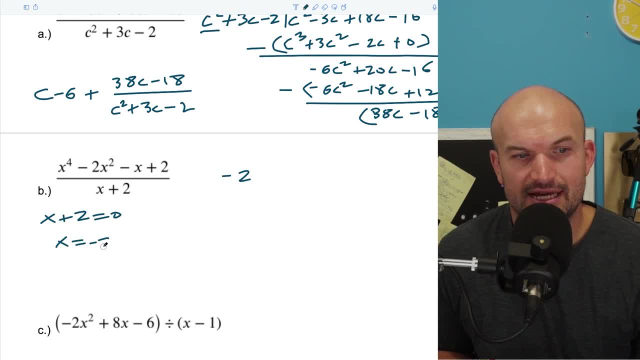 right equals zero, So then X equals a negative two. So now what we're simply going to do is take the coefficients. So we're going to take the coefficients of our dividend here And notice how I don't have a cube right. So when I don't have a cubed, what I'm going to do is use 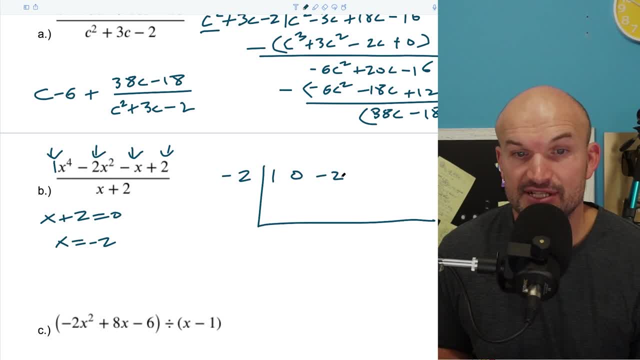 zero as a place value. So I have a one zero or a placeholder negative, two, negative one and two. All right, So now this is part of the synthetic division algorithm. So I bring down the one and then you multiply on the diagonal, add on the vertical. So one times negative, two is a negative. 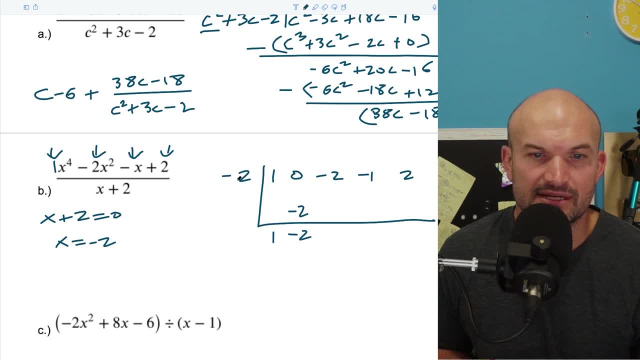 two. Zero plus negative two is going to be a negative two. Negative two times negative two is going to be a four. Negative two plus four is going to be a positive two. Two times negative two is a negative four. Negative one plus negative four is going to be a positive two. 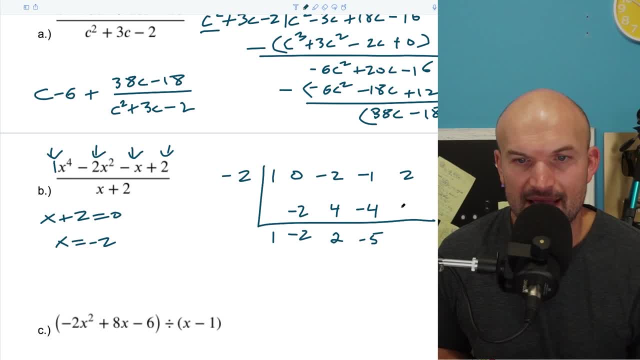 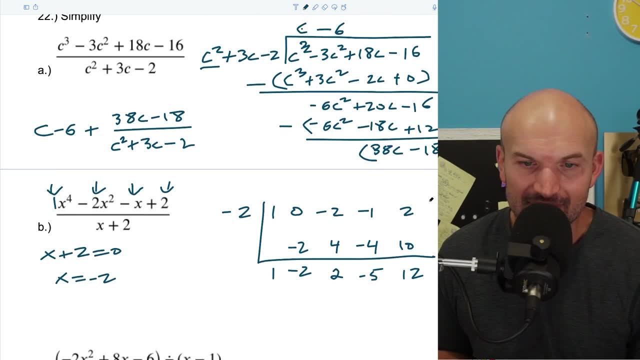 It's going to be a negative five Negative five times negative. two is going to be a positive 10.. Two plus 10 is going to be a 12.. So now this answer looks a little bit different than that answer, right? So what we need to understand is: how do we write this out? Well, that's your. 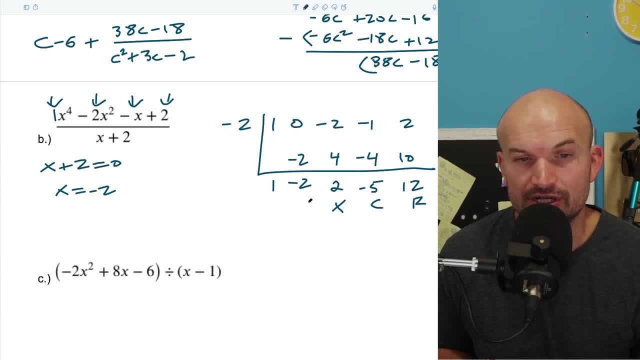 remainder. That's your constant, That is your coefficient of your linear term. This is going to be the coefficient of your quadratic term, And here's the coefficient of your cubic term. All right, So the. so I can write my answer now as a X cubed minus a two. 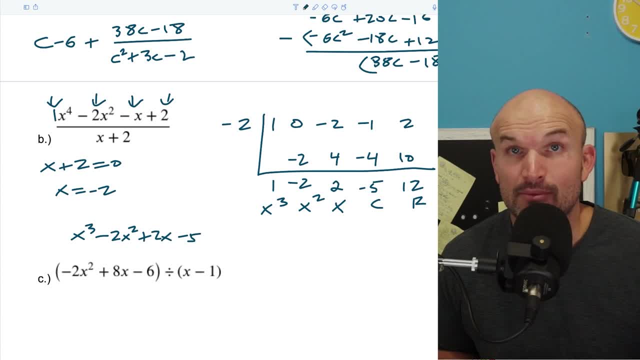 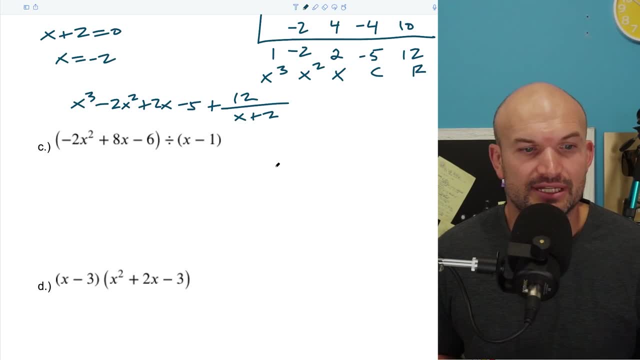 X squared plus a two, X minus five, And remember we have a remainder, right, So that's going to be plus a 12, all over my divisor, which is an X plus two. All right, So let's go and do the exact same. 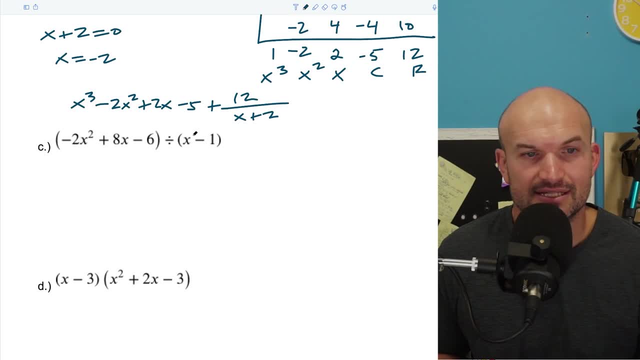 thing again here and just go ahead and set all these up, So again I can set my denominator, set my divisor equal to zero. Hopefully, recognize that's just going to be a one right. And then let's go and take these values here. Let's go and move this over, though just a little bit. 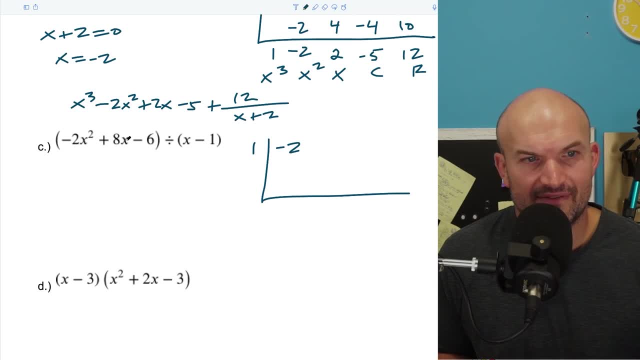 Okay, So what I'll have here is a, a negative two. Um, I have an X and a negative six. That's good, So I'll do an eight and a negative six. Okay, Bring down the negative two. negative two goes times One is going to be a. 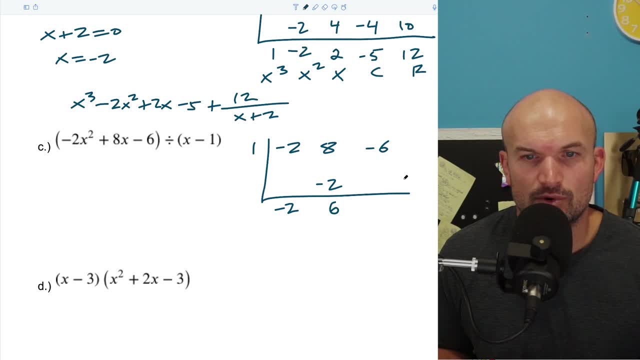 negative two. eight plus negative two, It's going to be a positive six, six times one. It's going to be six. So therefore that zero. So therefore, that's where I'm at my remainder, my constant and my linear term. Therefore, my answer in this case is a negative two, X plus six. Okay, And 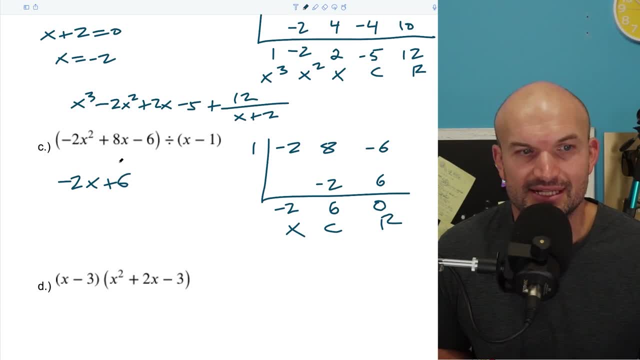 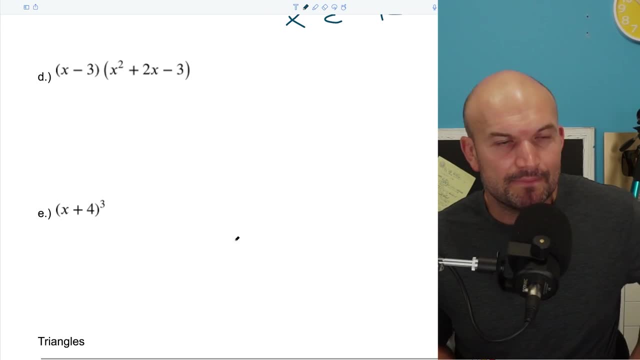 basically what that means again is X minus one times negative two. X plus six is going to equal that right. So that's that understanding of that Um. all right, let's just go through a couple more um, a couple more examples of. 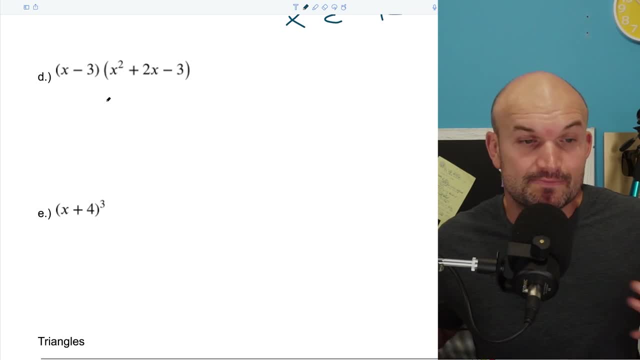 the expanding our binomials, or expanding um polynomials, And because that's going to be something really helpful, um for you to make sure that you can do rather um effectively. So the really the main thing I want you to really understand here is: you know, just apply the. 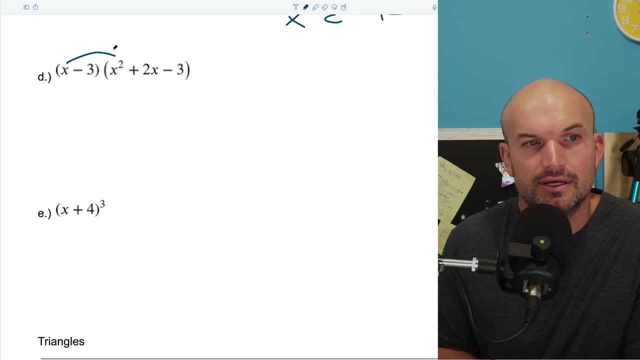 um, just apply- sorry, just apply- distorter property. So you know, you go like this right: Multiply the X times everything, And then you're gonna multiply the negative three times everything. All right, And you can, you know, you can do this using the vertical or the horizontal method. 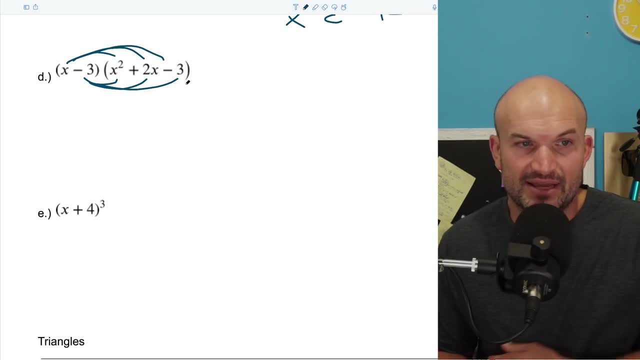 whatever kind of works for you. I usually like to just do the horizontal method, meaning just going to write out all the products and then find my like terms that I can combine. So X times X squared is a X cubed. X times two X is going to be a two X squared. 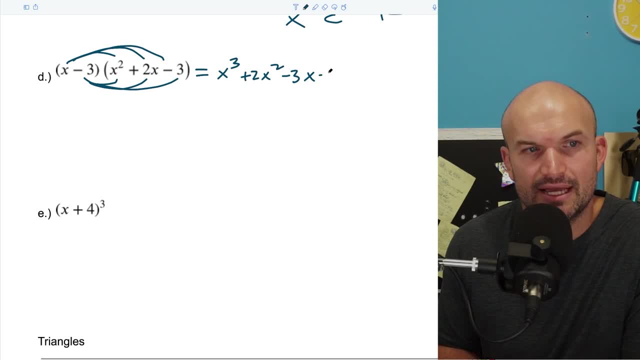 X times negative. three is going to be a negative. three X- Um, this would give me a negative. three times X squared is a negative. three X squared Negative. three times two X is going to be a negative. I'm sorry That's a negative, So I said it but I write it. negative three, That's. 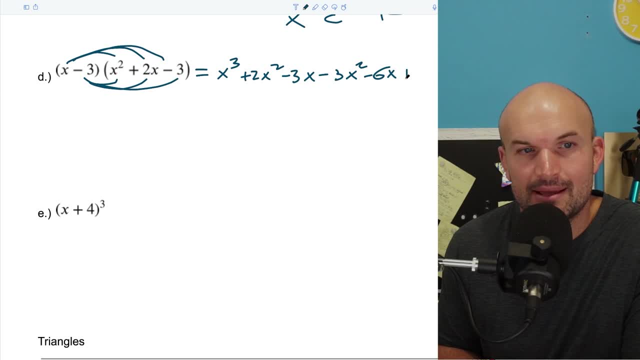 going to be a negative six, So I'm going to write it: negative three times two, X squared, And negative three times negative. three is going to be a positive nine. All right, So that's everything. Now let's just figure out what like terms can I combine? Well, I can. 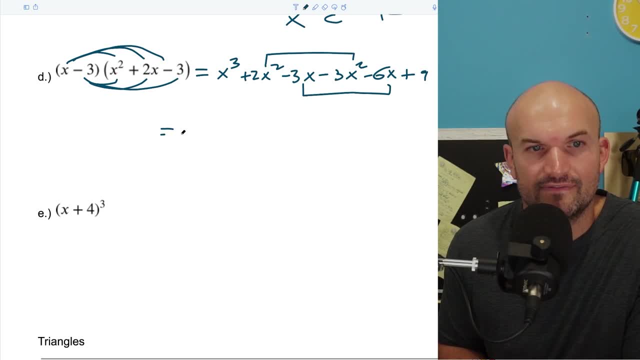 combine my X squared and I can combine my Xs. So therefore I get a final answer here of a X cubed That's going to be an X cubed, X cubed, X cubed, um, an X cubed, and then 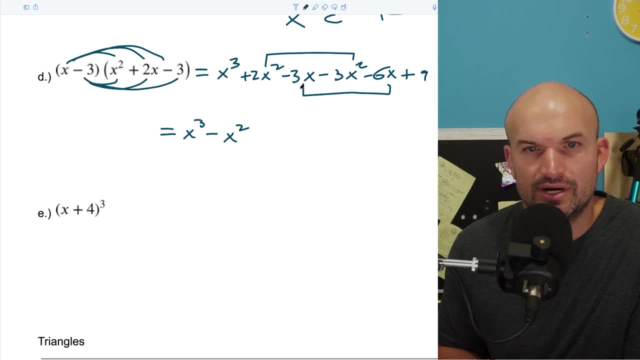 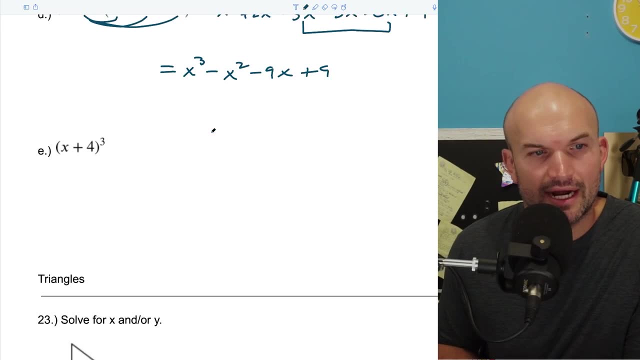 two X minus three X. That's going to be a negative X squared. Um, this is going to be a minus a nine X and then plus a nine. Okay, So, um, yep, it looks good. All right Now in this case. um, there's a couple of different things. I 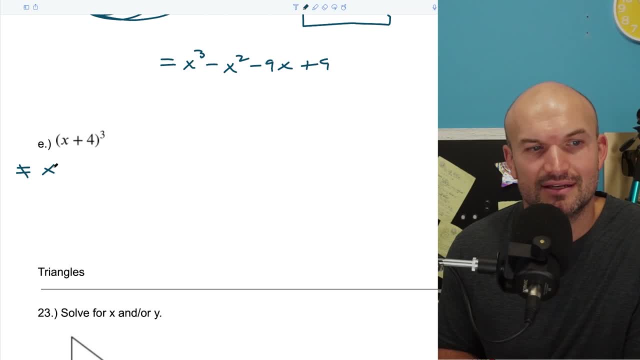 want to do. Please, whatever you do, do not do this X cubed plus four cube. That happens all the time, Happens every year. Don't do that. Remember: X plus four cubed is a X plus four times an X plus. 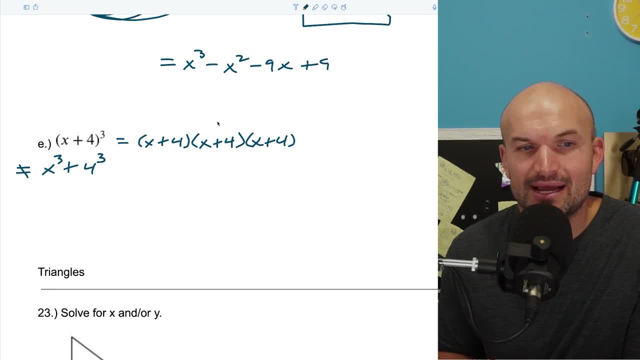 four times an X plus four. Okay, So the way I like to do this is for the first one. I think you can probably do distributed property or foil rather easily. hopefully, Um, and I can go and expand this, Um. so X times X is X squared four times. 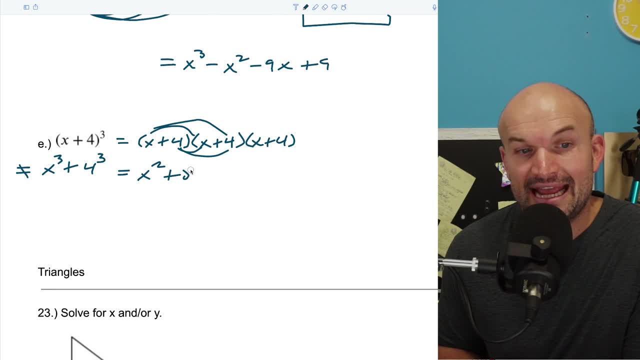 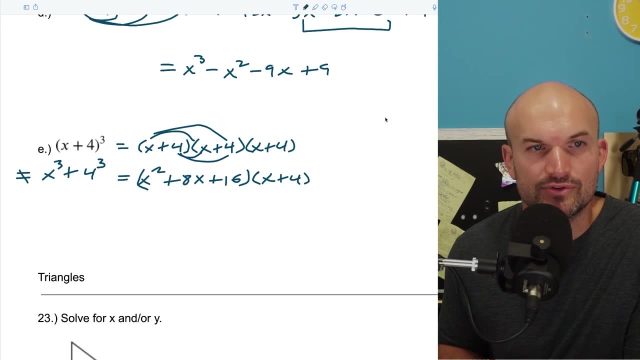 X is four X. four times X is four X. four X plus four X is going to be an eight X and four times four is going to be a positive 16.. Okay, And then X plus four. Now you can do the rest of the problem. 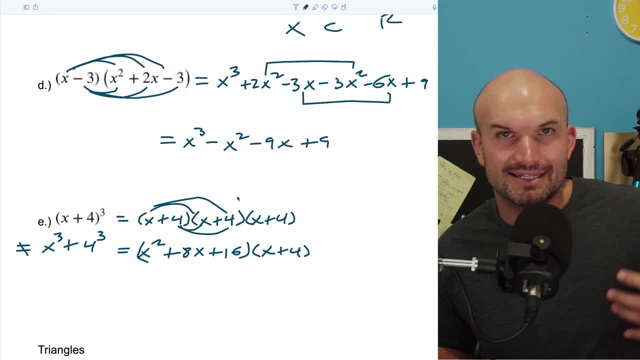 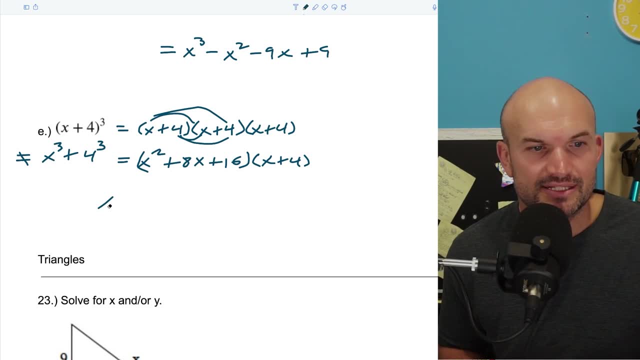 like this. but if you kind of notice there's a lot of things kind of going on, I think sometimes it can be easy to make a mistake. So another technique you can use is use what we call the box method. And the way the box method works is you basically take one product and put it along. 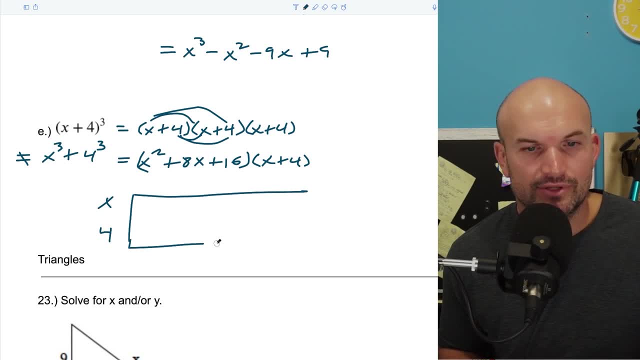 a box And then you take the other product or the other term in your product and you write it along the other side of the box. So that's an X plus four. There's two terms. So I'm going to write two rows. Now this is going to be an X. 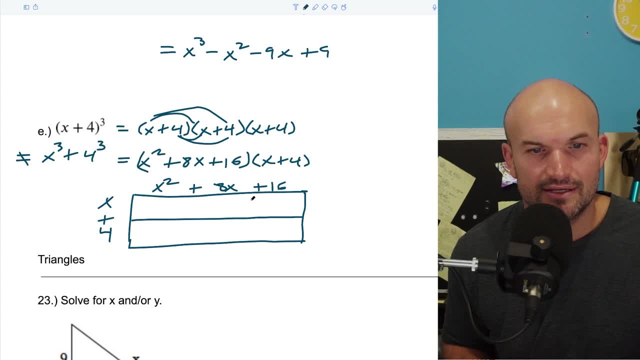 squared plus an eight, X plus a 16, which has three terms. So I'm going to do three columns. Now all you're going to do is basically find the area of each of these boxes. So you're just basically going to multiply length times width. So X times X squared is an X cubed, X times eight. 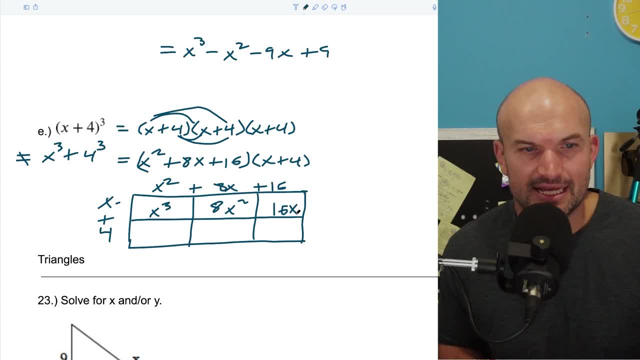 X is an eight. X squared X times 16 is going to be a 16 X. X squared times four is a four. X squared four times eight X is going to be a 32 X, And four times 16 is going to be a four 1632.. That's going to be a 64.. So the thing I like about 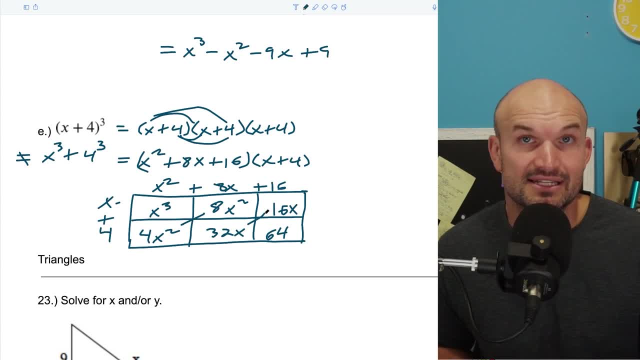 the box method, is it just kind of groups things So you can see as long as everything's on a descending order, everything is kind of grouped on the diagonal. So therefore now I can write my final answer here: as an X cubed, four plus eight is going to be a plus a 12, X squared 32 and 16 is 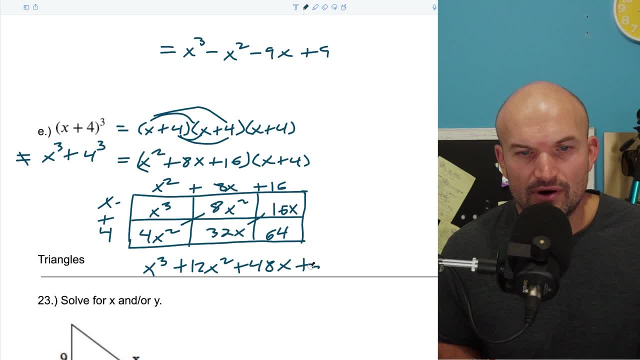 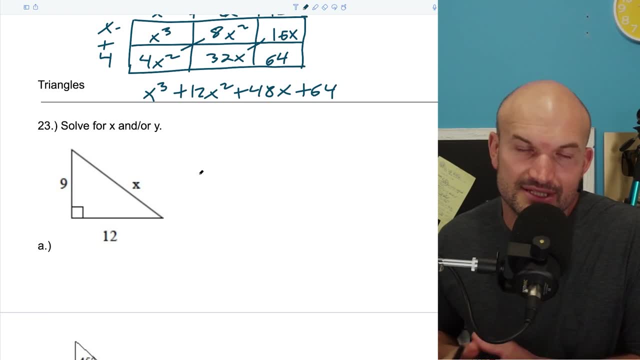 going to be a 48, and then plus 64, and voila, we're all done, All right. So now let's go and do a quick little review of geometry, Because even though precalculus has a ton of the algebra two, there's also a lot of trig and 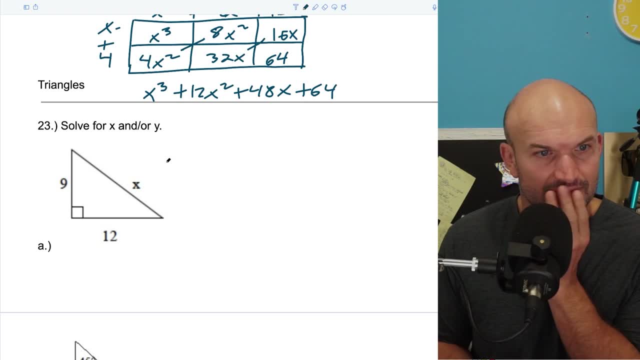 triangles. that's going to be going on So. so if in this case I have solve for X and Y, So in this case, hopefully you recognize the Pythagorean theorem right, Remember: a squared plus B squared equals C squared. So in this case I have a nine squared plus a 12 squared is equal to a X squared. 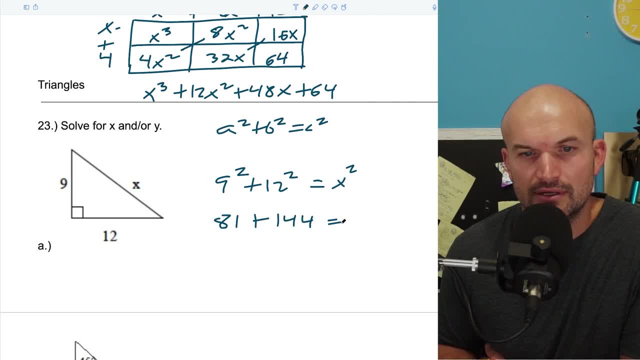 All right. So this is going to be an 81 plus one. 44 equals an X squared. I'm actually that's going to be an 81 plus one: 45 equals a X squared. So take the square root of both sides and you get X. 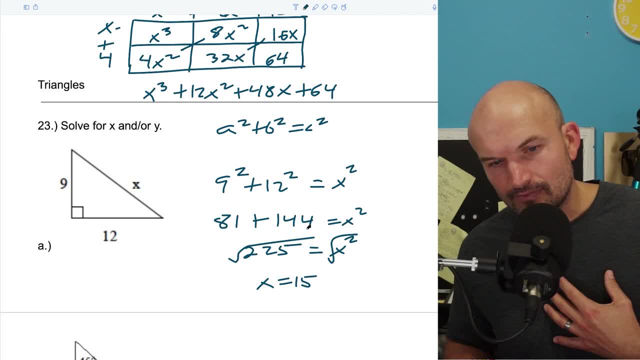 equals a 15. It's not plus or minus in this case, Um, because obviously the sides of a triangle need to be positive, for our example. but hopefully you can recognize here that this is what we call a perfect. I should have known this. a perfect, um, a uh, Pythagorean triple right. So that means: 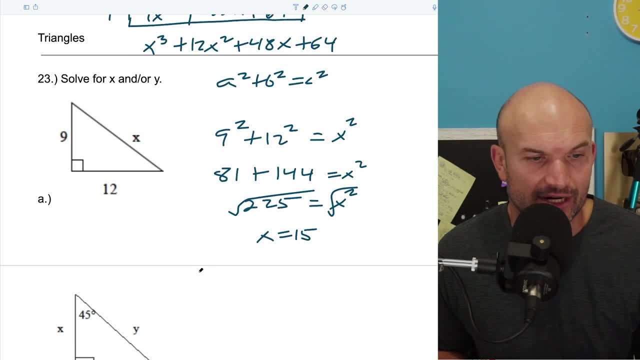 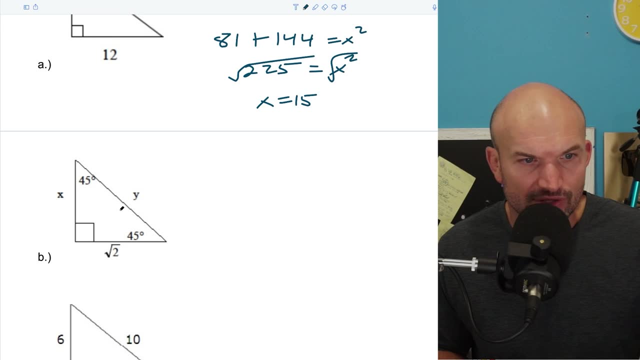 all the side links are going to be an integer, So that's something to remember. is those Pythagorean triples All right? Now let's go and look into our special right Triangles, And so this is a 45,, 45, 90 triangle, So hopefully you need to remember that these are 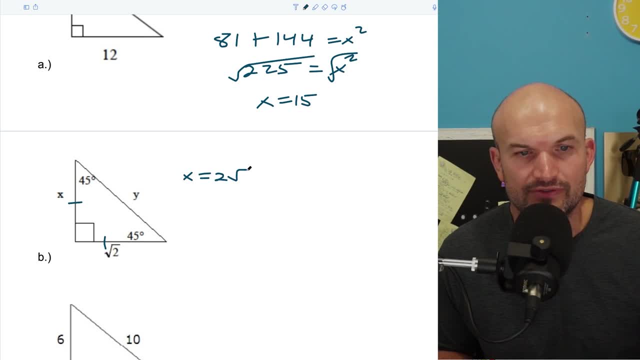 this is an isosceles triangle, So therefore X is going to equal a two square root of two. Now again, you could use the Pythagorean theorem again if you want to, but it's really important to recognize that. um, that, to go from my legs to my hypotenuse, all I need to do is multiply by. 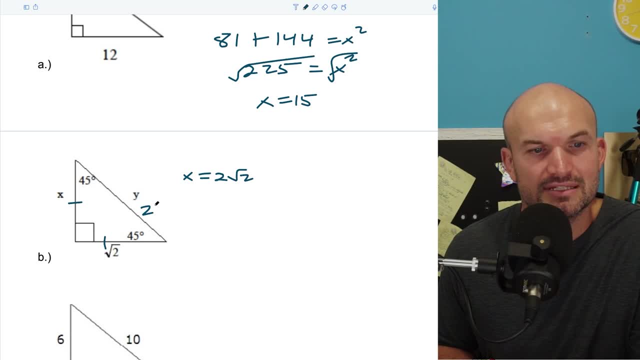 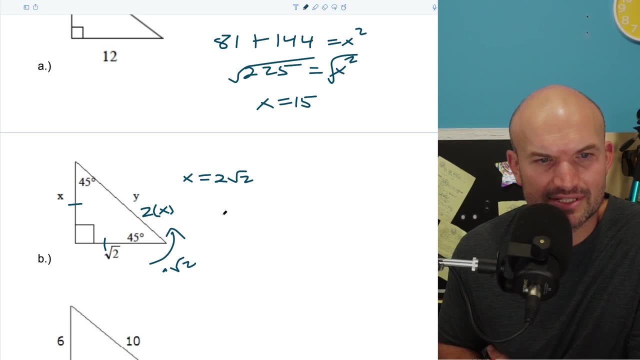 another two. So this is going to be a two times your X, like times, whatever your legs are. So to go from here to here, you multiply by the square root of two. What I'm going to do here is now say Y is equal to a um, two square root of two times a two square root of two. 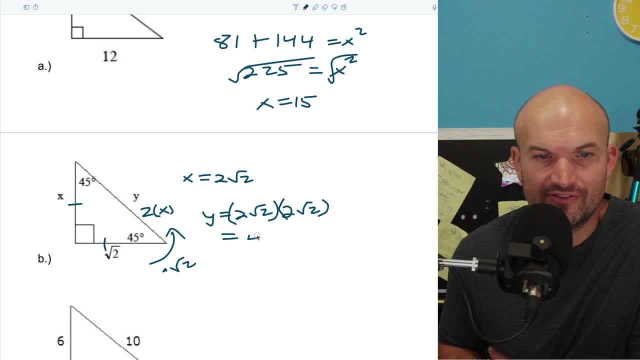 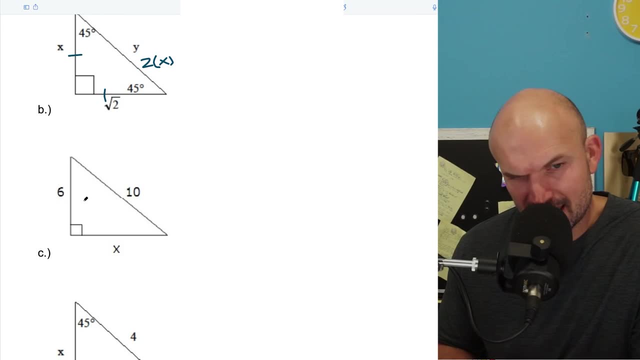 Okay. So two square root of two times two square root of two, that is going to equal a four times square root of two times square root of two, which is two. So therefore that's going to equal an eight over here. Hopefully this is not a Pythagorean triple six, eight, 10.. I think this. 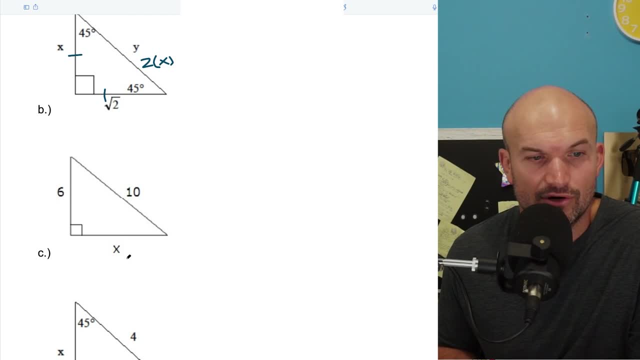 is a Pythagorean triple Um, so hopefully you can recognize that that is going to be 10 or this. sorry, this is going to be an eight. Again, that's really important. See how quickly I did that. Like, that's very, very helpful. You could also use Pythagorean theorem So you could say six. 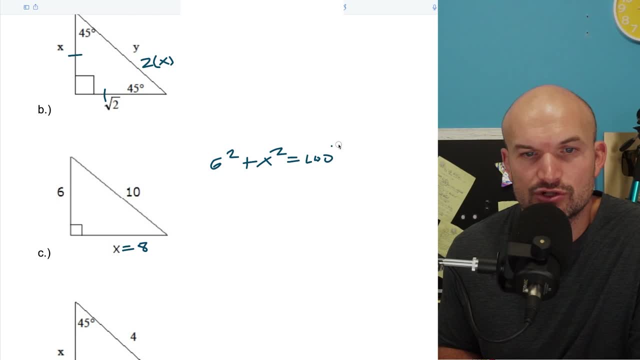 you know, squared plus a X squared equals a hundred squared. Well, that's a 36 plus X squared equals not a hundred squared, That's just going to be a 10 squared, right So? but a 10 squared is obviously a hundred. So 10 squared, which is a hundred, and then you could subtract a 36. 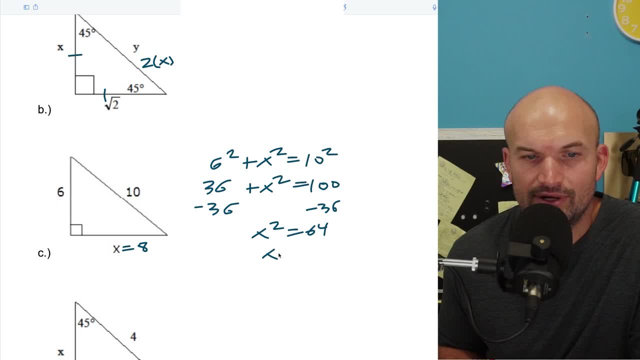 and you get X squared is equal to 64.. And what do you know? Ms McLogan was right. Thank you very much. Okay, Now in this example again, remember to go from here to here- we multiply by the square root of two, So that's going to equal a four times a two. 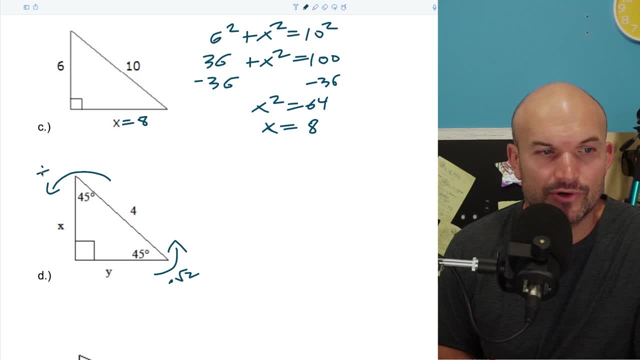 Right. So to go backwards, to go from a hypotenuse to leg, I'm going to divide by the square root of two. So, basically, I just want to know what is four divided by the square root of two. Well, just rationalize your denominator here, And what you'd have is a four times the square root of two. 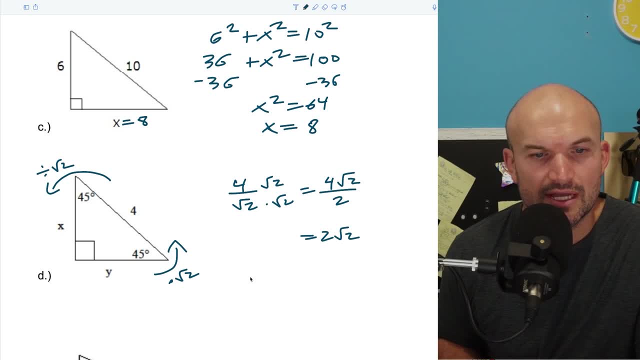 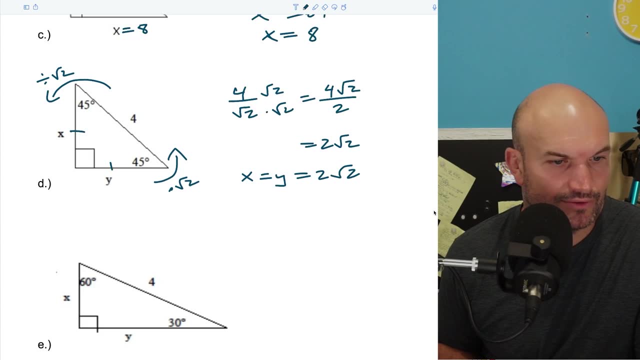 divided by two, which is just going to equal a two square root of two. And remember, X and Y are exactly the same. So therefore, X is equal to Y, which is equal to a two square root of two. Now the relationship between my 30,, 60, 90 triangle is kind of similar, or it's not really. 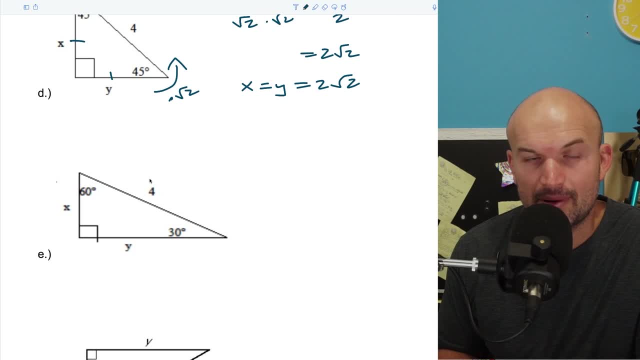 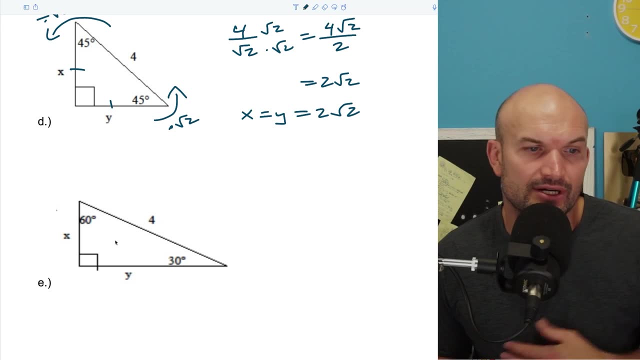 well, it is kind of similar. um, to go from my, I have two legs and a hypotenuse right. So cause, obviously, the legs are not the same like they were for an isosceles triangle. So the relationship here of this triangle is from short leg to hypotenuse. You're going to 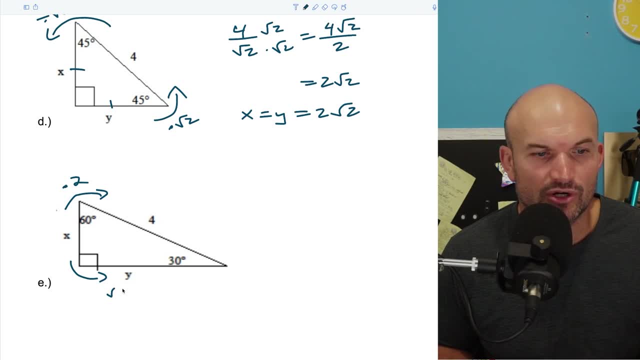 multiply by two, and to go from short leg to long leg, you're going to multiply by the square root of three, And again, if you're going to go backwards, you're just going to divide by these terms. So if I want to find X, that's going to be a four divided by two right, Which is just. 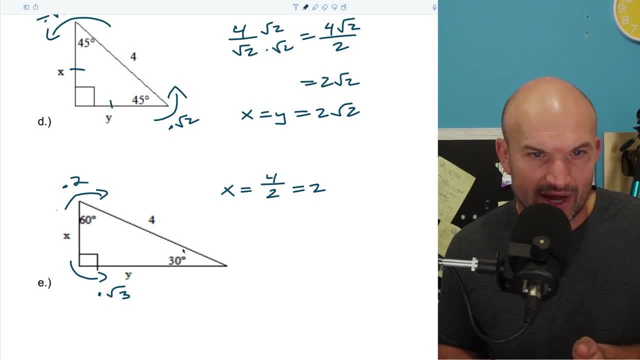 going to equal two. So now, if I want to find X, that's going to be a four divided by two. right Now I know X equals two. to go from X to Y, I multiply by the square root of three, So Y is: 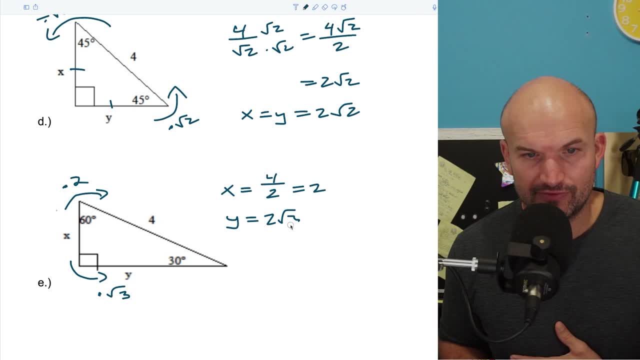 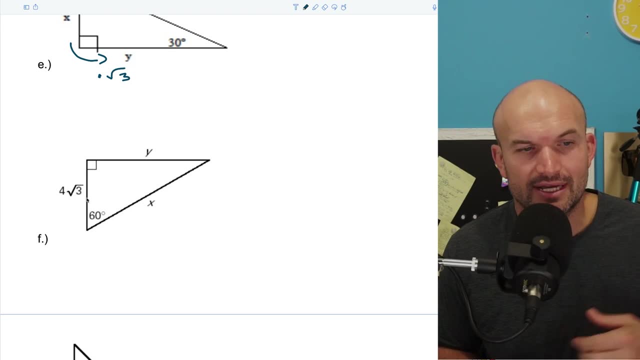 equal to my X, which is two times the square root of three, which is just two square root of three. Um, over here it looks like this is the short leg and that's the long leg, right? So again to go from short leg to hypotenuse, in this case I'm just going to take my short leg, So four. 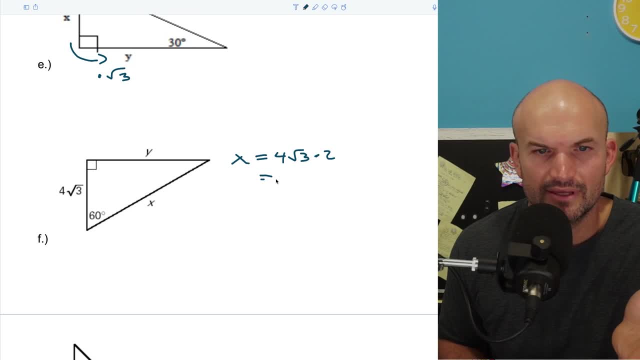 square root of three and I'm just going to multiply that by two. That's going to give me an eight square root of three. to go from short leg to hypotenuse or short leg to long leg, You multiply by the square root of three. So Y is equal to 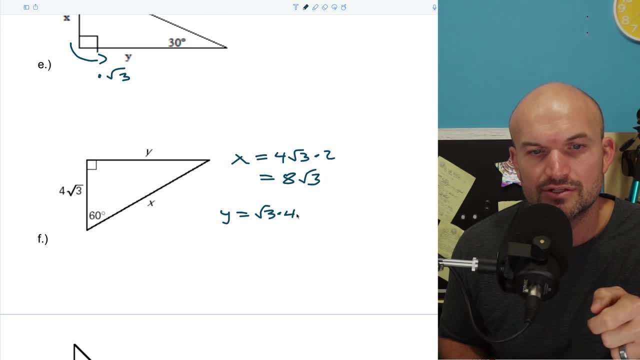 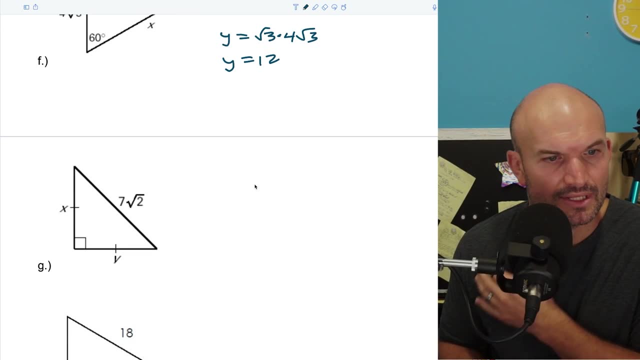 the square root of three times a four, square root of three. Well, I can multiply: square root of three times square root of three. That's going to be three. three times four is going to equal a 12.. Um, over here you're just going to work backwards again. right Again, another 45,. 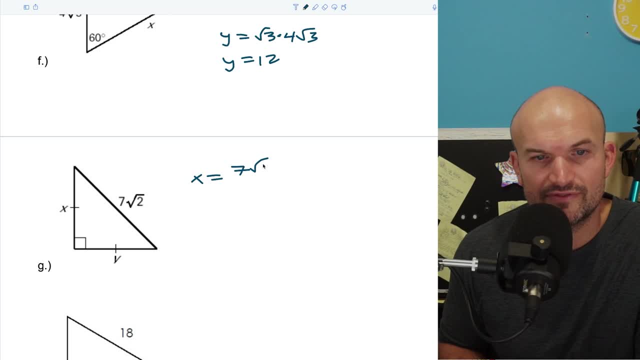 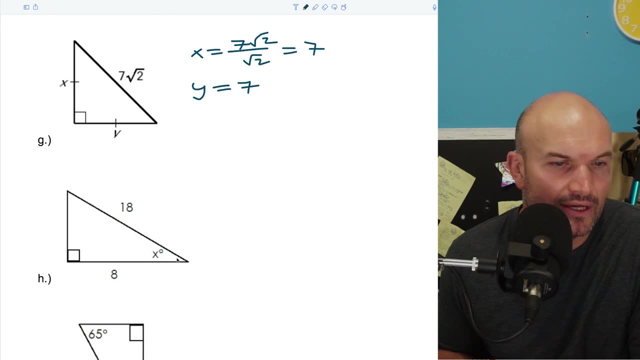 45, nine triangle. So my X equals a seven square root of two divided by square root of two. Well, that's just going to equal a seven, right? And Y, then, is also going to equal a seven. Um, now what we need to do is understand our relationships for trig, because obviously we 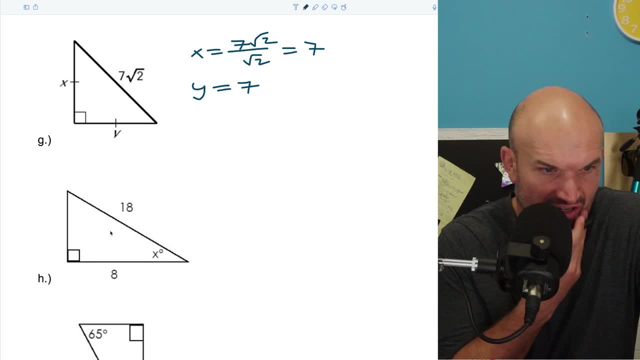 know if this is a special right triangle and we don't have enough information. Um, well, actually we want to find the angle. So the Pythagorean theorem is not going to help us out. So what we need to understand here is: if here's my angle, okay, here is my hypotenuse: the angle between 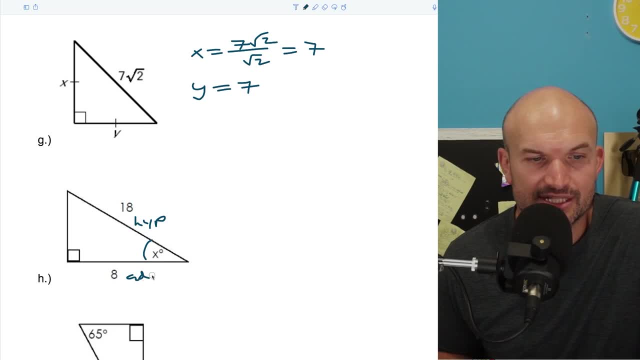 the right triangle, the right angle And my angle is what we call the adjacent side, And the side on the other side is what we call the opposite side. All right, So when I have the hypotenuse and the adjacent, we need to understand our trigonometric functions. So I have the hypotenuse. 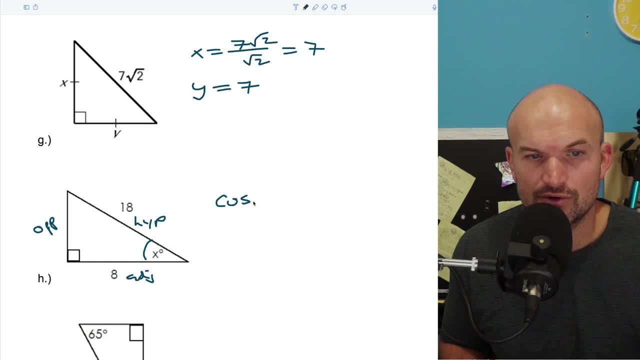 and the adjacent side. So I'm going to use the cosine function. So what I can say is the cosine of X, right, Which is my angle, is going to equal to my adjacent, which is eight, over my hypotenuse, which is 18.. So therefore, X equals the cosine inverse of eight. 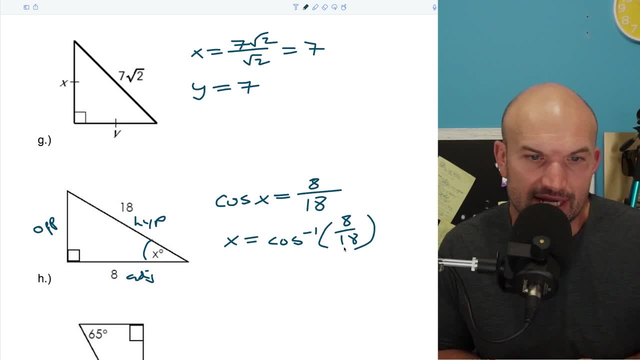 over 18.. So if I want to undo cosine, I want to find out the value of that cosine. I need to use the inverse function. Uh, make sure your mode is in degree mode. When you're go ahead and type in your calculator and you just do cosine inverse of eight over 18, you 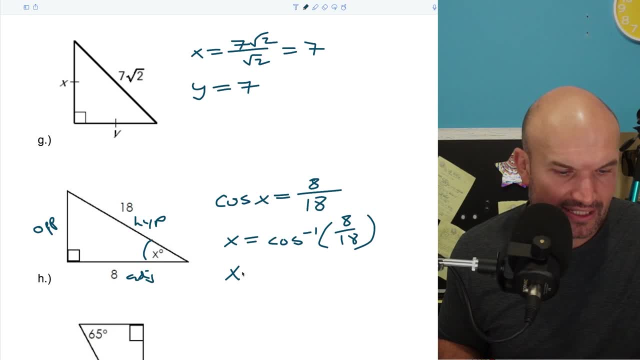 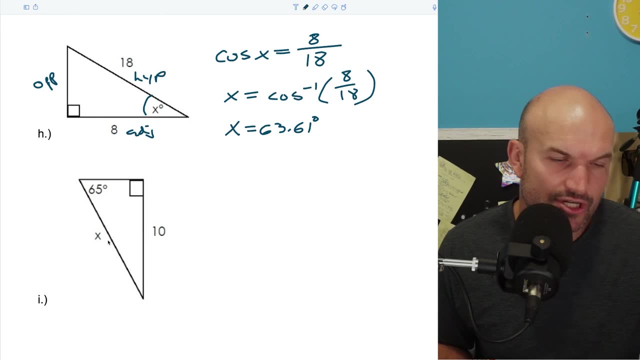 don't need to simplify it to one ninth. You can just leave it exactly as it is, And in this case, X is going to equal a 63.5.. And I'll just run it to the nearest hundredth degree. So now let's go and do another one. 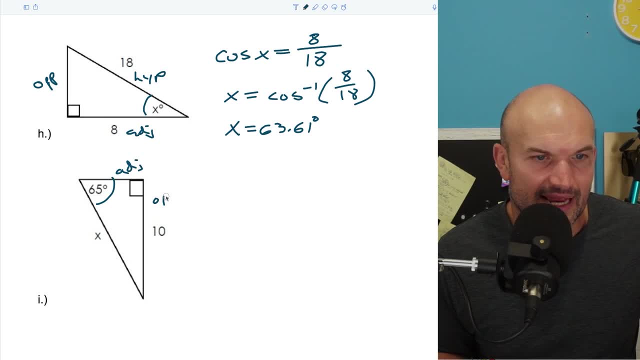 So now we have an angle right. So this, that means that's my adjacent side, This is my opposite side. Okay, So, um, in this case, where you have the opposite and the adjacent, so now we're going to use the tangent function So I can say the tangent of X. I guess I should. 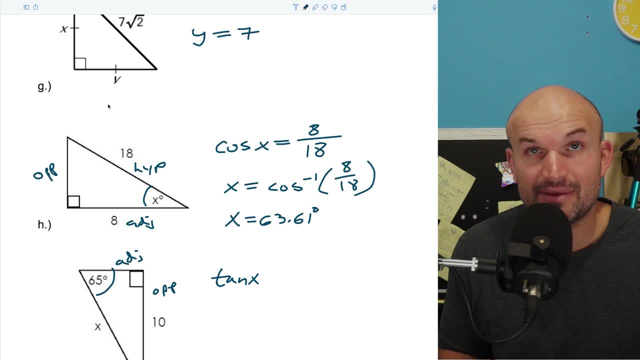 probably like review all the functions right. So, um, we have three main trigonometric functions. The sign of a angle X is equal to the opposite, And we have the hypotenuse over the hypotenuse. The cosine of X is equal to the adjacent over. 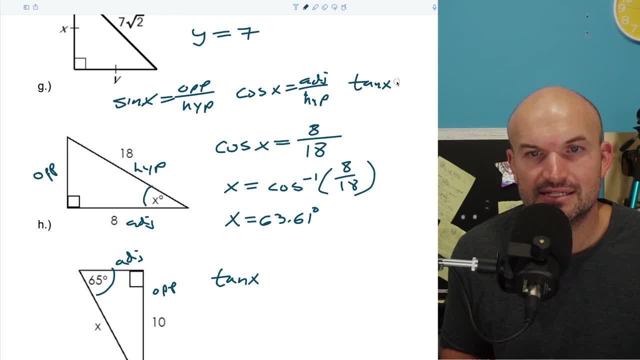 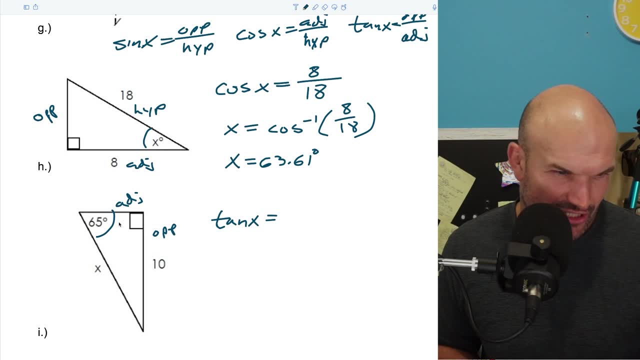 the hypotenuse And the tangent of X is equal to the opposite. over the adjacent. All right, So now I'm going to have. tangent of X is equal to a. actually I don't have enough information. That's sorry. I don't have a wrote adjacent, but we don't have anything for the Jason. 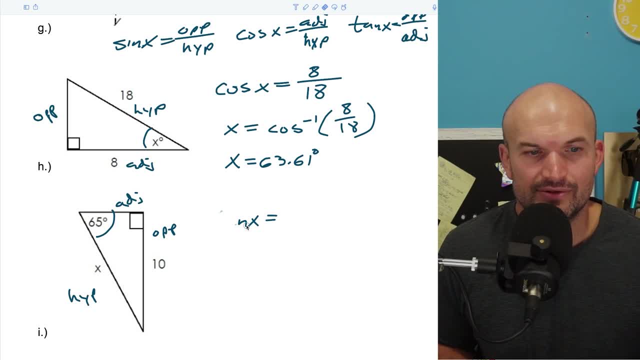 We have the hypotenuse, so we're not going to use tangent. We're going to use the opposite over the hypothese. Speaker 1, we're going to use sign. In this case the cosine is equal to the opposite over. 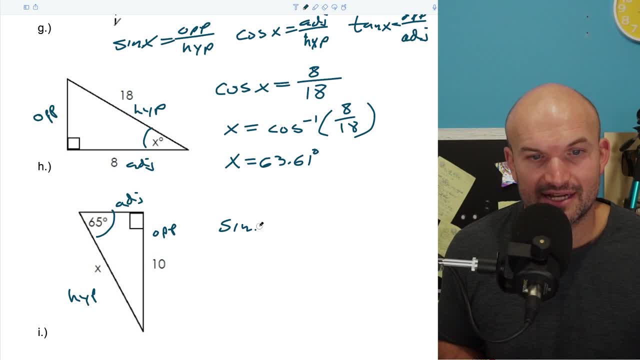 case. So therefore, let's rewrite this So I'll have a sine. of X is equal to opposite over the hypotenuse right. So that's going to be a 10, or? I'm sorry, I'm losing my mind. We know what the 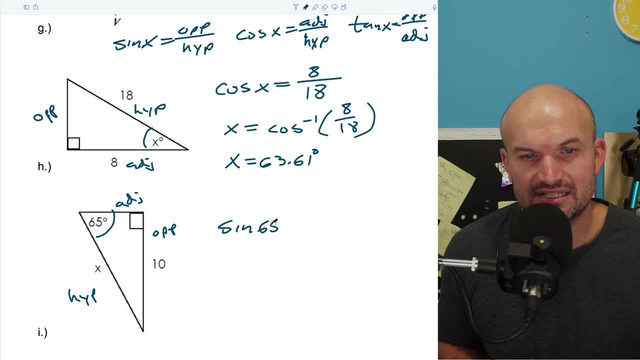 angle is right. So I can say: the sine of 65 degrees is equal to the opposite over the hypotenuse. So that's going to be a 10 over an X pool. Now I need to solve for X. Well, obviously, to solve for. 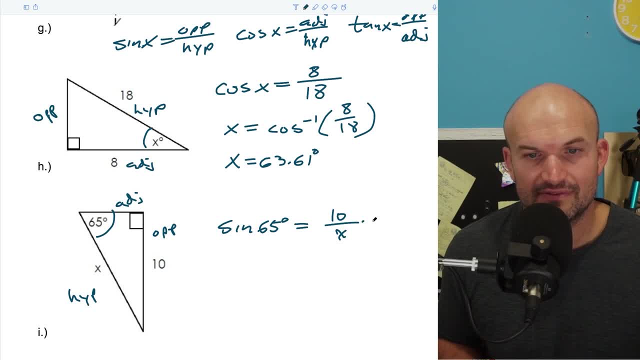 X. you need to multiply by an X on both sides and then divide by sine of 65, right? So multiply by an X on both sides, you get X times a sine of 65 degrees equals 10.. And then to solve, you need to: 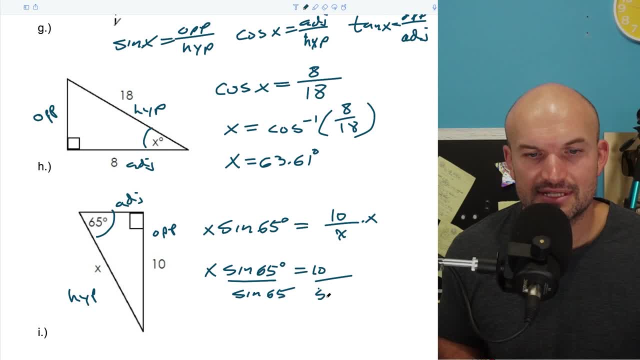 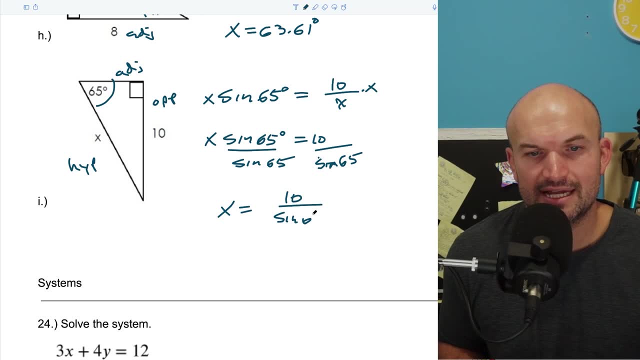 divide by the sine of 65 on both sides. So sine of 65.. So now what I'm going to have is X equals a 10 over the sine of 65 degrees. Now what I simply need to do is again plug that in. So I'll just. 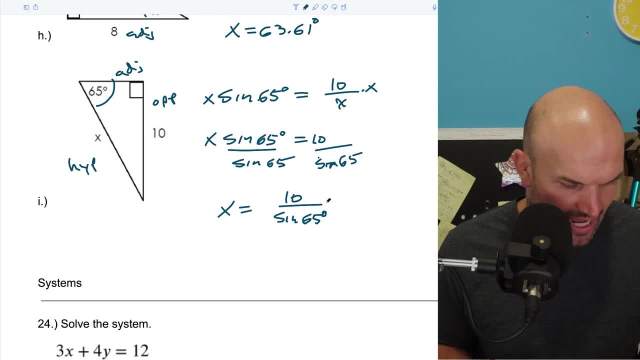 do a 10 divided by the sine of 65 degrees, And now I get a X equals 11.03.. I know that again, I'll just use that to the hundredth. All right, Um, last but not least, here is doing some. 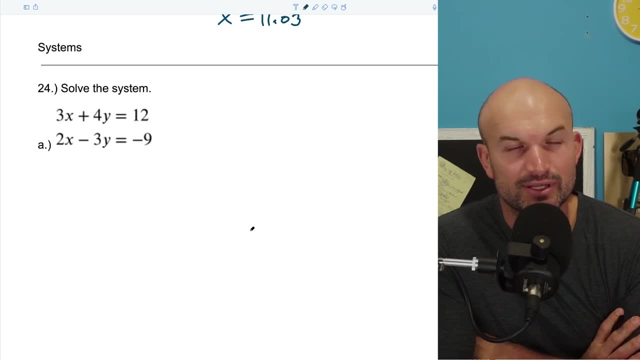 systems of equations. So let's just practice solving. Remember? you could graph it, You could use substitution, You could use elimination. Um, in this case, it actually doesn't tell me what to do, So as long as, unless I have a variable that's already isolated, I'm just going to use 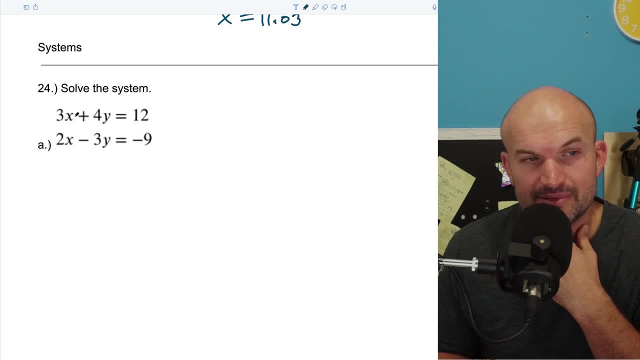 elimination. So the main thing we want to do, to remember, is get the coefficients to be exactly the same Um. so what we want to do is find the LCD. Now, typically you can find the LCD for the negative Um, but I usually like to find. I usually, like you know, you want one to be. 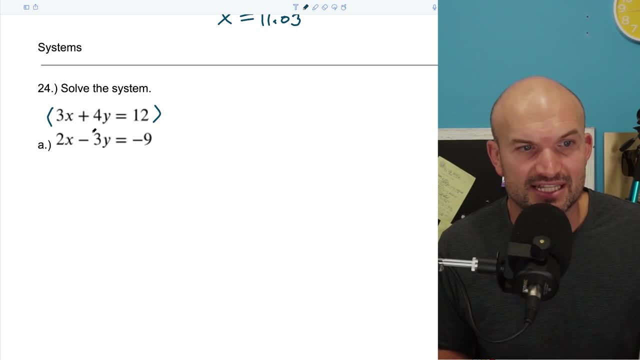 positive, one to be negative. Well, since here these coefficients are already ones positive, aren't already ones negative? Um, I'm just going. I'm not going to choose that one, though, because actually the LCD of three and four is 12.. The LCD of here is six, So I prefer to find the 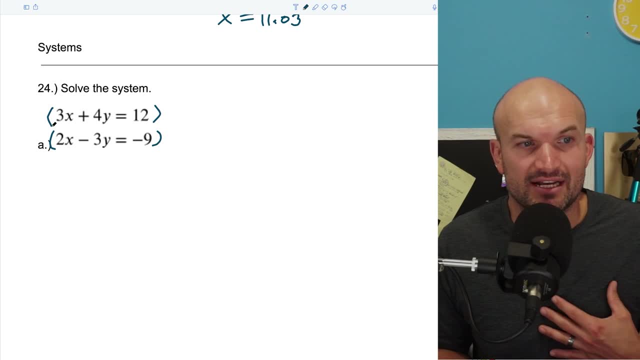 LCD of the smaller number. but since I want one to be positive, one to be negative, I'm going to make one of my scalars be negative and I'll just make the top two to be a negative two, And then I'll multiply by three. So now I need to multiply everything, times everything, Cause you have to. 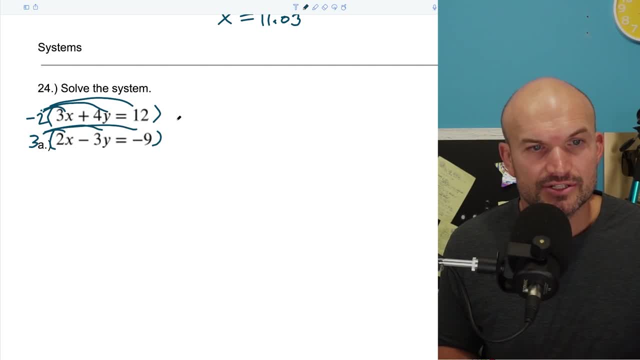 produce what we call Equivalent equations. All right, So now let's get a new system. So my new system now is a negative six X, um plus- or that's actually not plus, that's going to be a minus eight Y equals a negative 24.. And then over here I'm going to have a positive six X. 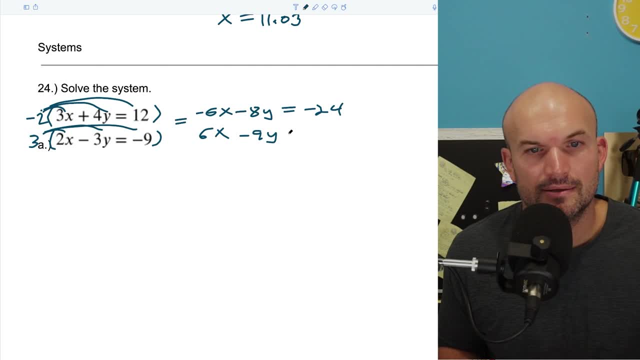 minus a nine Y equals a negative 27.. Okay, Now I have these up. Now I can just go ahead and add them vertically And what's going to happen is I'm going to get rid of my axis. So therefore, this will be a negative 17 Y. Um, this is going to equal a negative 51.. No, sorry, 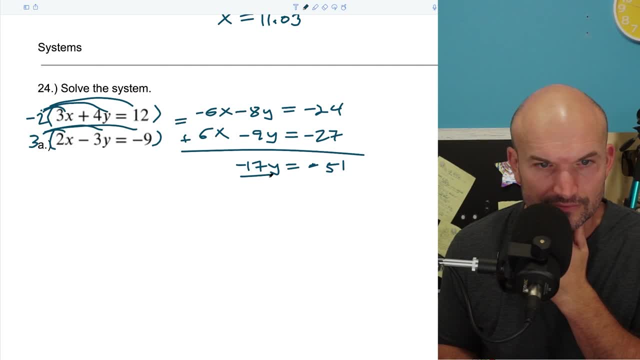 That's yeah, Negative 51. So it'd be a negative 51 divided by negative 17 divided by negative 17.. Y is going to equal. It looks like a positive three. Now I just need to go ahead and solve for X. So remember, just plug it back into one of those equations, It doesn't matter which one you. 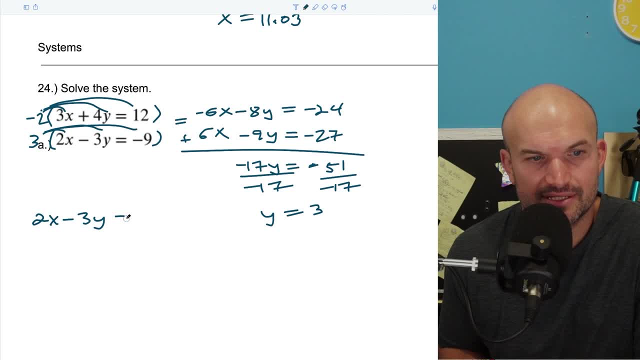 do it in. I'll just choose the bottom equation. Um, because I don't know. I'll choose the bottom equation. So, therefore, I have a two X minus a three times three Equals a negative nine, right. So that's a two X minus um minus nine equals negative nine. 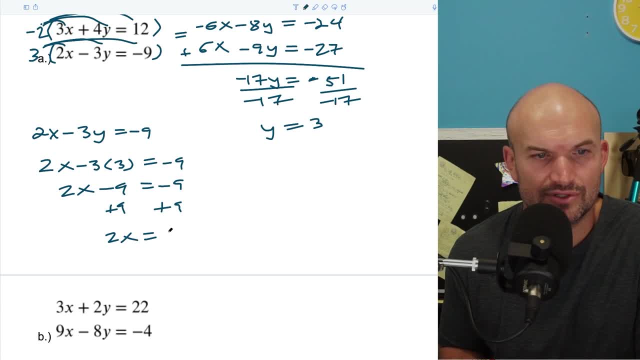 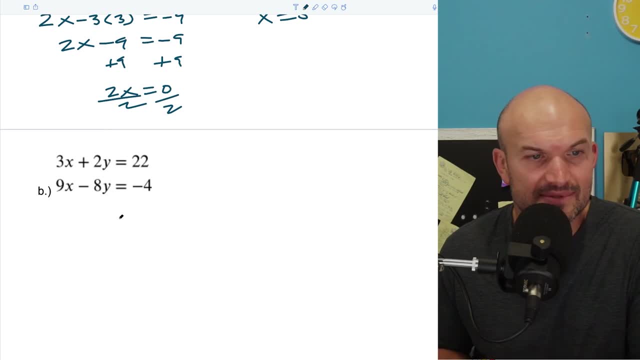 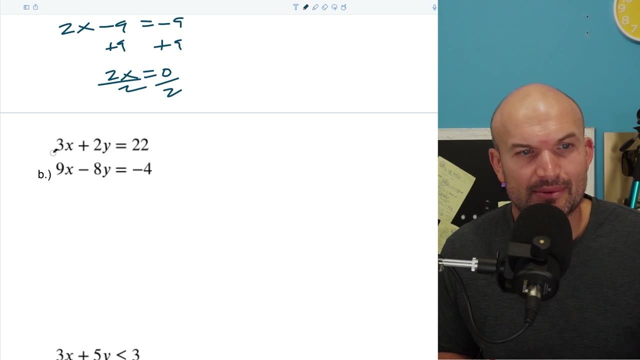 And then I'll just add a nine to both sides. Two X equals a zero. So therefore, divide by two, divide by two X is also going to equal zero Um. so now this one is already nicely kind of created for us, right? So for this one um to go from, all you need to do is multiply by three. 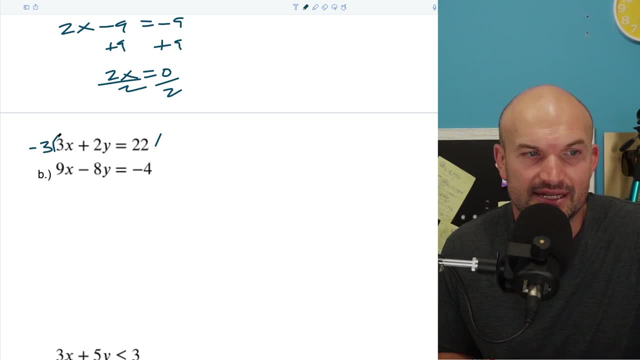 on one equation, But again I want it to be one positive, one negative. So I'm going to make this all right. So when I do that, I get a negative nine X, um, minus a six Y, and then therefore, 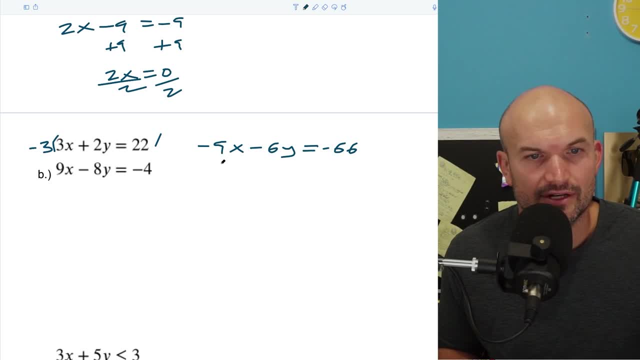 that's going to equal a negative 66.. Then over here I have a positive nine, X. Um, this is gonna be minus eight. Y equals a negative four. Okay, So now I have the same coefficients, One's negative, one's positive. I can add them up vertically. That's going to eliminate those, That's going. 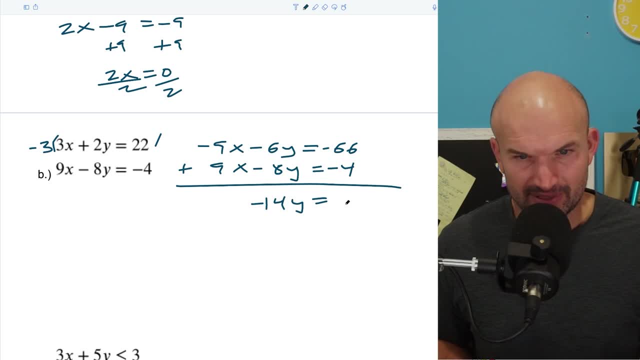 to give me a negative 14 Y And therefore this is going to be a negative 70.. Right, I'm assuming I didn't do anything correct? That's going to be negative six Y, That's being negative six six, Okay, Um, I don't think that is going to be there, but it's. 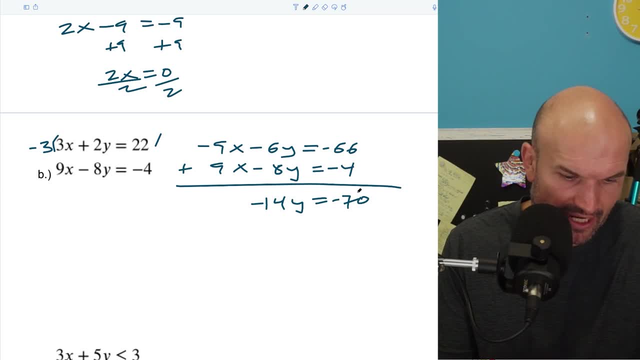 I guess we can use a fraction here, So I'll do a 70 divided by a 14.. Oh, that equals five. I guess I probably should have checked my work here. Um, so I divide by negative 14 on both sides. 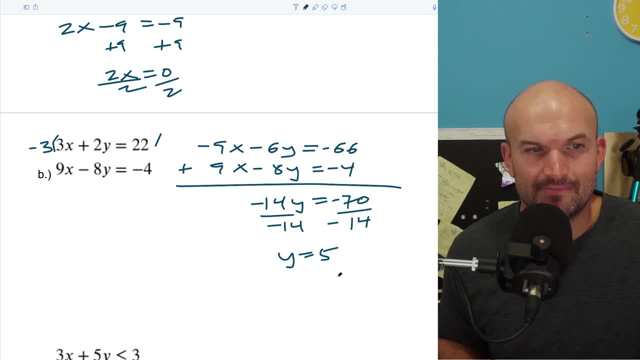 and I get Y equals five. Okay, And again, just to go ahead and solve for X, in this case I'll go ahead and plug it into the top equation. So I'll do: a three X plus a two times five equals a 22.. So three X plus, let's see that's going to be a 10 equals 22.. 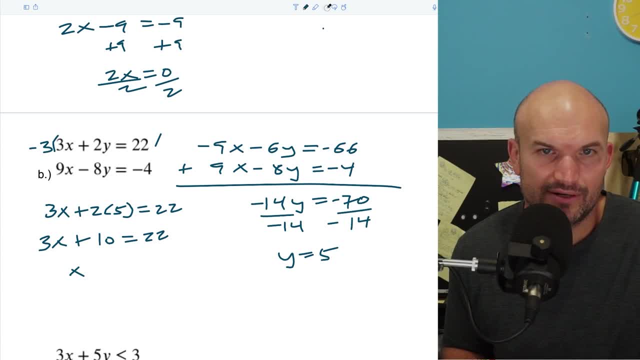 And then subtract 10 divided by three. Um, I'll just do my work. I was like showing my work. I don't like doing mental math. because when I'm doing mental math, what happens? I make mistakes. or then students always ask the question like Hey, where'd this number come from? Or how do 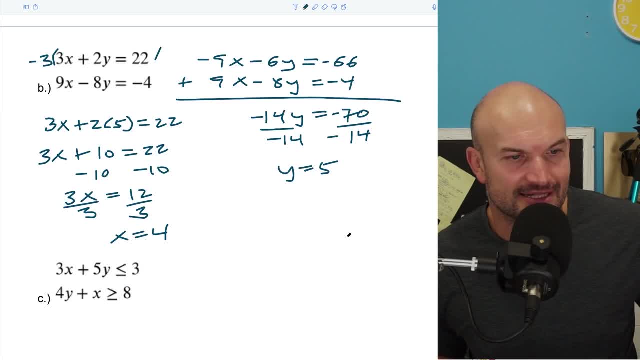 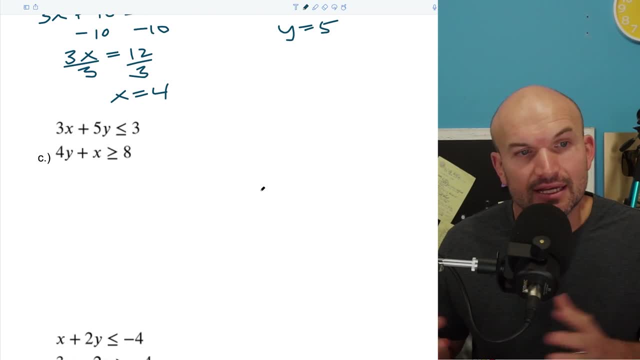 you do this, So X equals four. All right, Um. now, last but not least, I just want to cover inequalities and graphing inequalities. Remember, we need to worry about this, like with the shading: you know the test points and where everything's going to be at. So, um, in this first example, 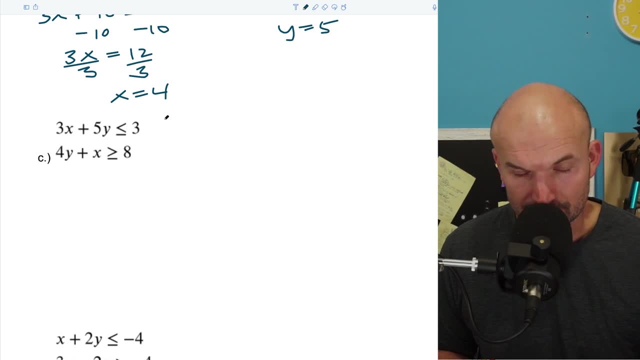 what we want to do is basically just kind of rewrite these as um in in our slope intercept form. So I'm just going to do a three X plus five- Y is less than or equal to a three, And then I'll do a four Y plus X square and equal to an eight. Okay, So, by putting this into slope intercept form, 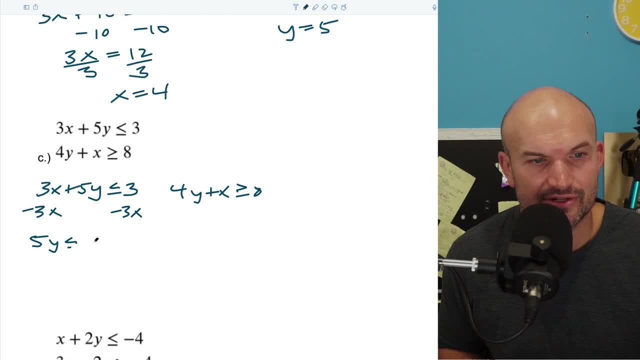 I'm going to subtract a three X on both sides, So I get a five. Y is less than or equal to a negative three X, um negative three X plus three. Okay, Then I'm going to divide by five on both sides. 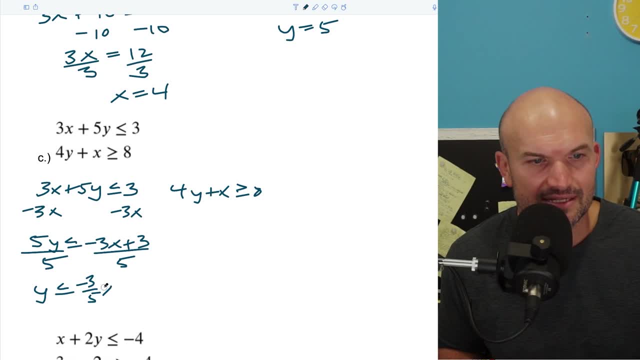 So Y is less than or equal to a negative three X plus three. So I'm going to divide by five on X and then plus a three fifths, which is going to be, like you know, close to like 0.5, right, Or? 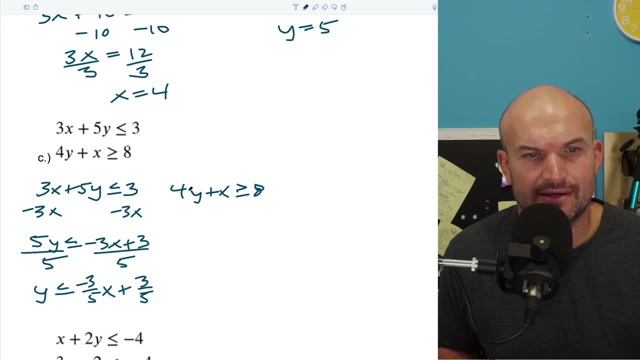 that's roughly 0.6.. Um, that's equal to an eight. Okay, So then over here I'm going to kind of do the exact same thing. Just subtract the X, Now I have a four. Y is going to be greater or equal to. 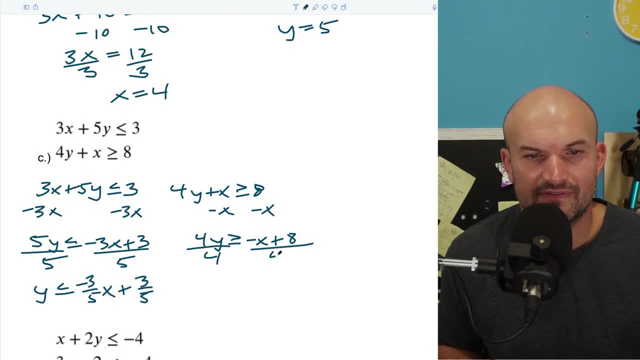 a negative X plus eight. divide by four, divide by four, Y is greater or equal to a negative one. fourth, X plus two. Okay, So now let's go ahead and graph this And again the graph. I'm not perfect here, ladies and gentlemen. I am just trying to get an idea of what this graph is going. 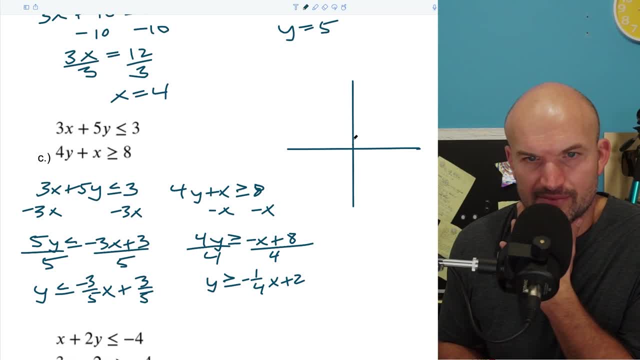 to look like. So three fifths is going to be like some, you know. let's say one, two, three, Let's say I can just do three, um, four, five. one, two, three, four, five, one, two, three. 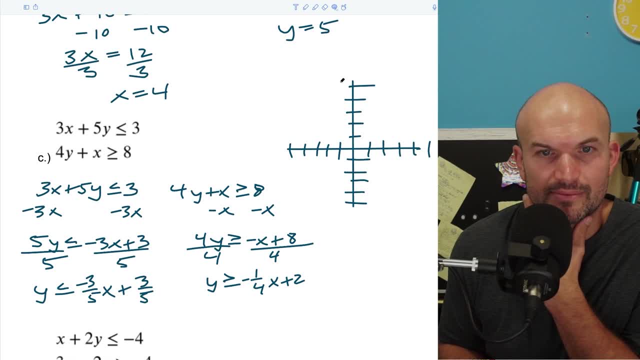 four, five. one, two, three, four, five, And actually what I'm going to do is I'm going to copy this, cause we have one more problem to do, So I want to use it again. All right, So let's go ahead and graph this. So three fifths is going to be like roughly somewhere there. 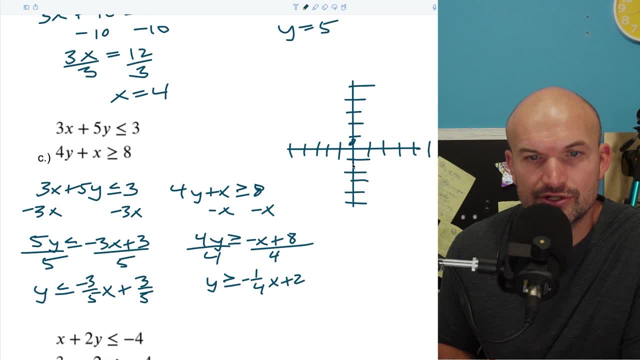 And then I'm going to go down three to the right five. So down one, two, three to the right five. one, two, three, four, five. Cool, Okay, Now this is less than or equal to, so therefore it's going. 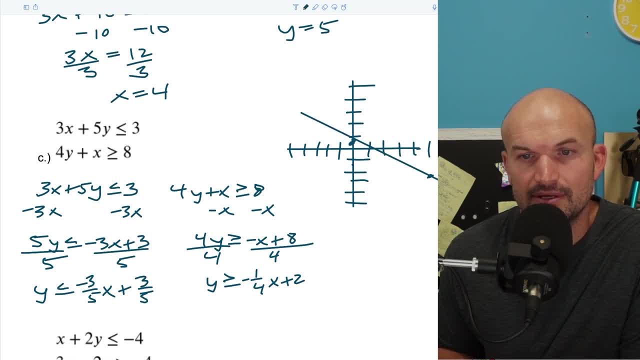 to be that line. This boundary line is going to be included, All right, And then what we need to do is just kind of use a test point. So let's choose zero. zero. Does that work? Zero right Is less than or equal to zero plus three fifths. So zero is less than or equal to three fifths. 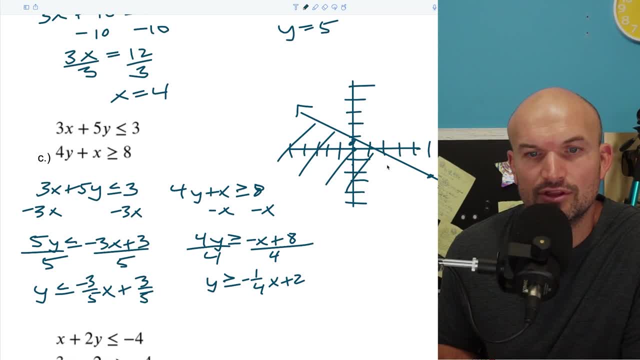 That is true. So therefore we can say: this is, all the points that are below the boundary line are going to be true. Now let's graph. Y is greater than or equal to negative one. fourth, X plus two. So go up two, one, two, And then now I'm going to go down one over four. So one, two, three, four. 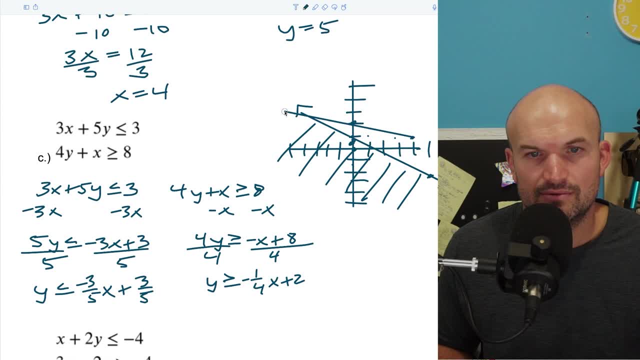 So it looks like that It's going to have a slope That's going to go like this: Okay, So it looks like we're going to have to extend this a little bit farther to kind of see: Okay, And then here, that's what. 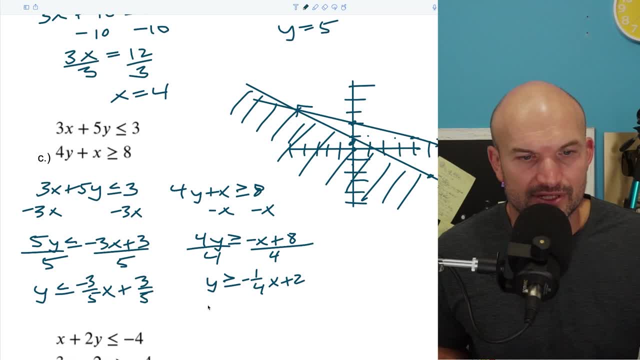 my graph looks like there, And now what I want to do is use my test point. So this one says zero is greater than or equal to two, right, When you plug zero in there. And so my test point here is false. So therefore that means everything up here is going to be true. So if you kind of see, 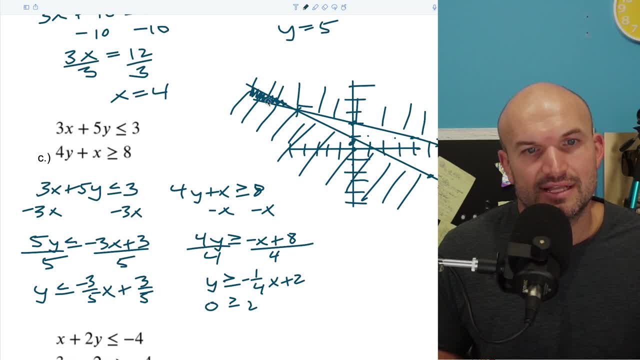 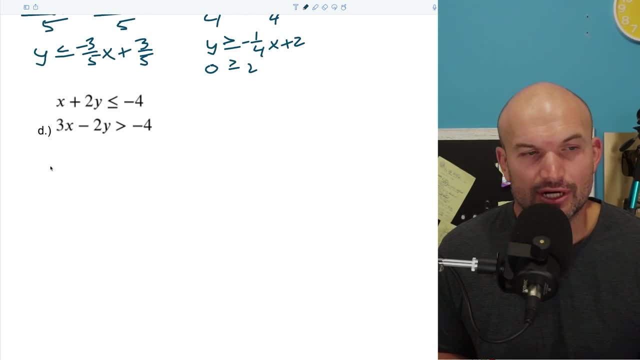 where do they intersect? they intersect in this little region right there. So that's going to be the solution to the system. All right, let's just do this one more time, Just to kind of get a good, just to get a good idea. So we have X plus a two Y. 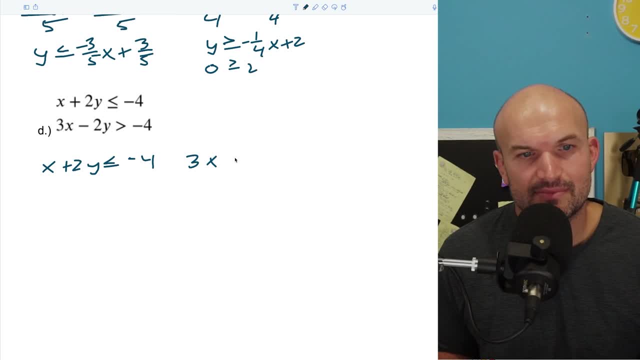 is less than or equal to a negative four. And then here I have a three X minus a two: Y is greater than a negative four. Okay, So let's go ahead and solve for Y And then so we can go and graph them. 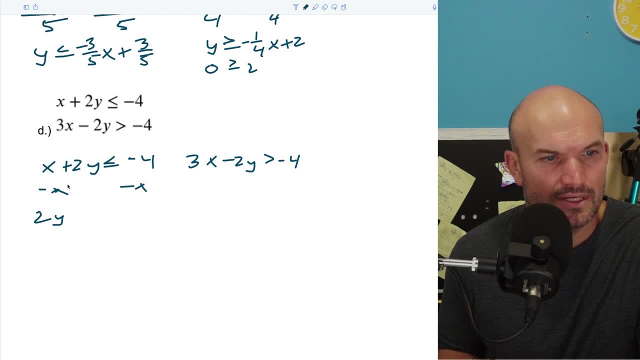 So subtract X, subtract X. So two Y is less than or equal to a negative X minus four. divide by two: divide by two Y is less than or equal to a negative one. half X minus two. All right, And then over here we're going to subtract a three X. I'll have a negative two Y. 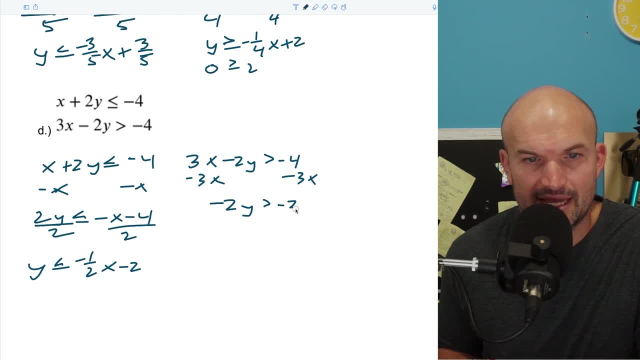 It's going to be greater than or equal to a negative one: half X minus two, Which was greater than a negative three X minus four. divide by negative two. divide by negative two, So Y. remember, when we divide, though, we have to flip the sign right, So that's Y is. 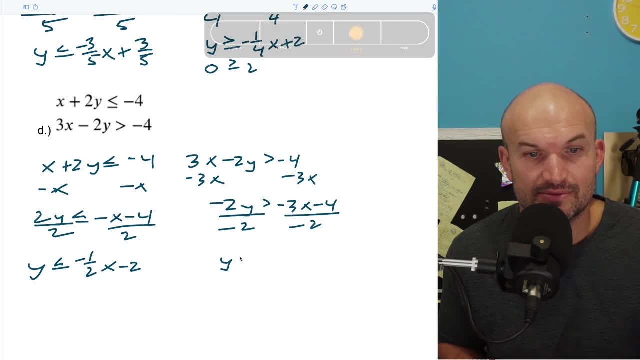 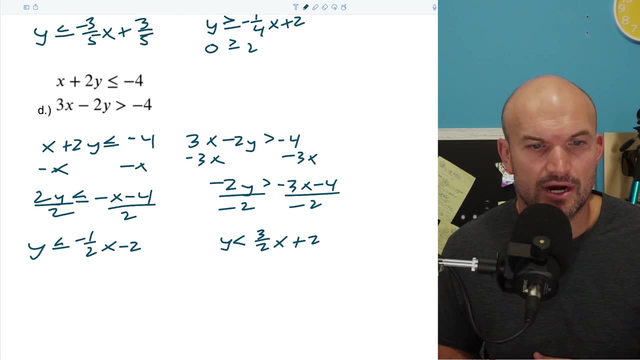 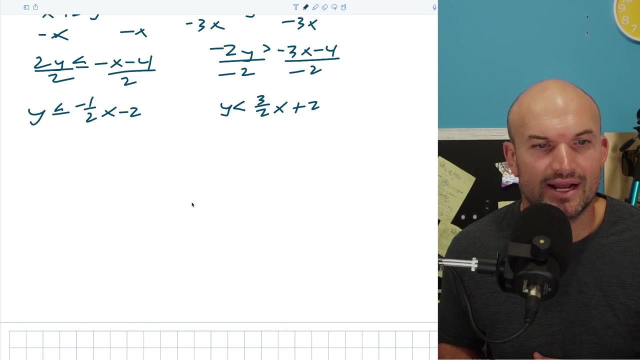 less than not. that way, Y is going to be a less than. let's see. this would be positive. three halves X and negative. four divided by negative two is going to be a positive two. All right, So let's go ahead and copy and paste that right there. Perfect, All right, Let's see. 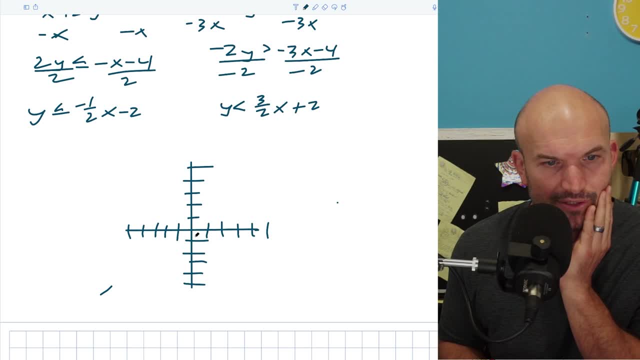 how this looks. So I have a negative two, So I'm going to go down negative two and then down one over two. So down one over two, Okay. So my graph is going to look something like that: Just try to mimic the slope as best as possible. And that is less than or equal to, So therefore,